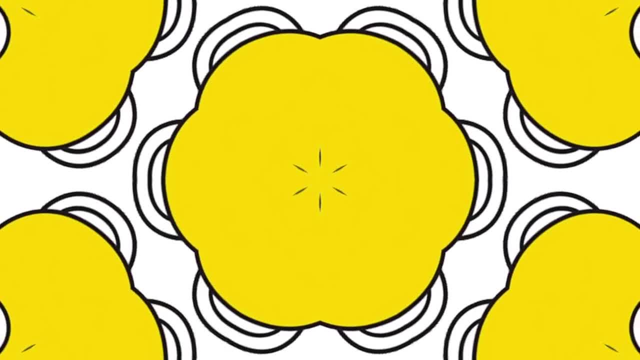 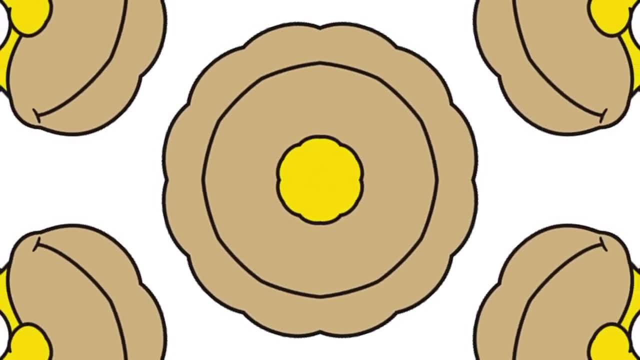 I have no idea. No idea at all. I'm pretty excited about it too. So every so often we change our money and I think there's a big push at the moment for plastic money in order to increase security, And I guess with the £50 note you want a really secure £50 note. 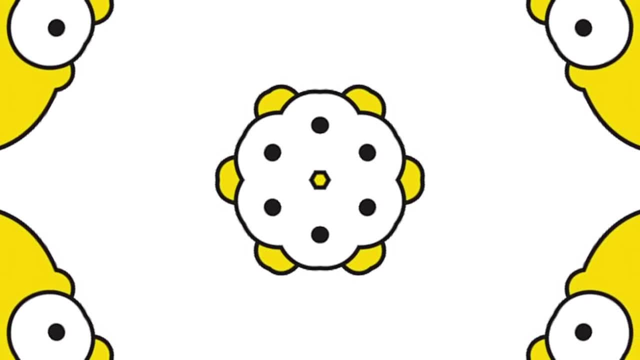 And so they've decided it's going to be a science-y type person. And there are a few of us. It's been brought together. I'm hugely honoured to be part of that committee and it's going to be fun and interesting. 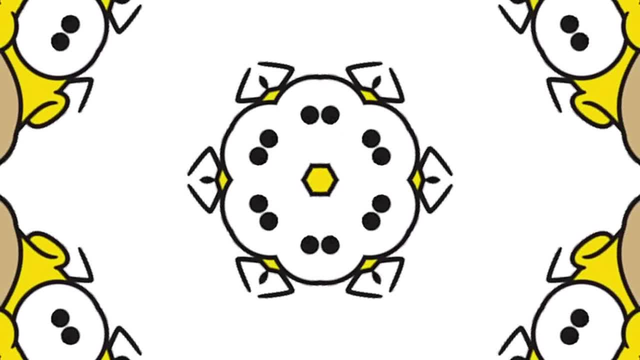 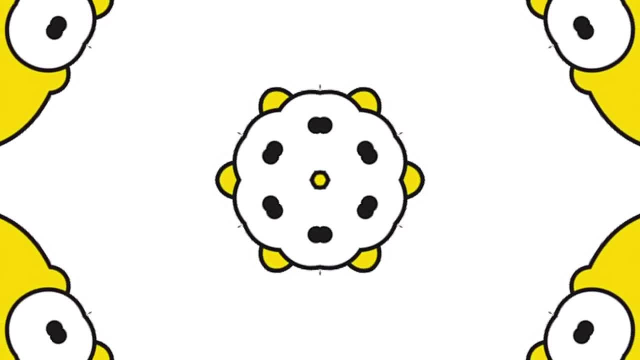 And I think we've had a record number of suggestions from the public, of scientists from the past right up to people who've recently passed away, like Stephen Hawking, To be on the £50 note. you need to be deceased and you need to be a real person. 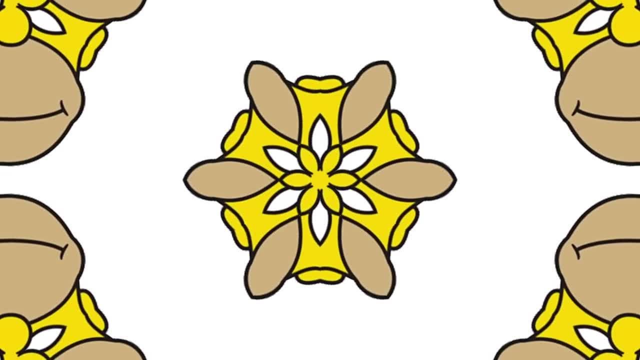 Yes, And a scientist, So Doctor Who does not count. I know I saw the governor of the Bank of England had to specifically rule out Doctor Who. That's right, But yeah, we've had. I think the people have nominated everyone from Margaret. 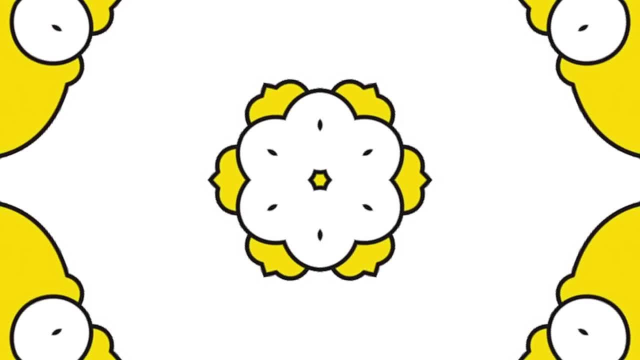 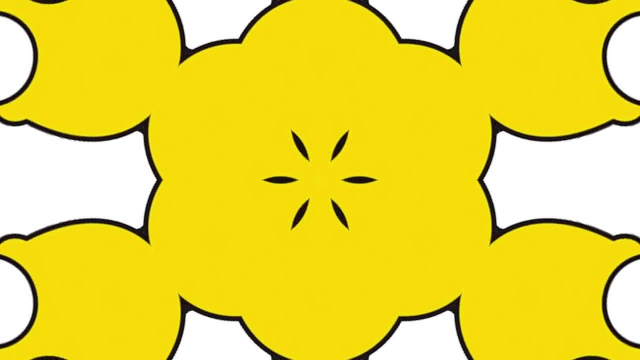 Thatcher, who was a chemist and may or may not have invented the Mr Whippy ice cream, going back to, yeah, all sorts of incredible people. So it's going to be great fun. We sit down next month to go through the list and to come up with a short list. 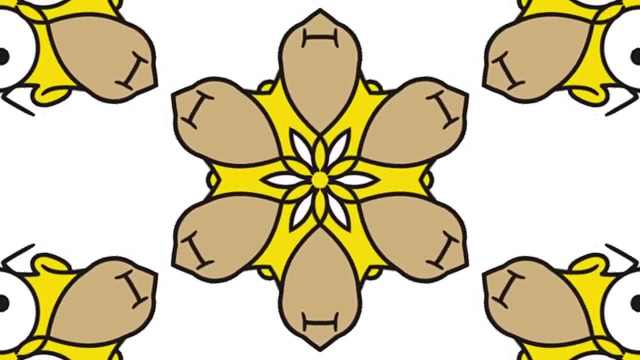 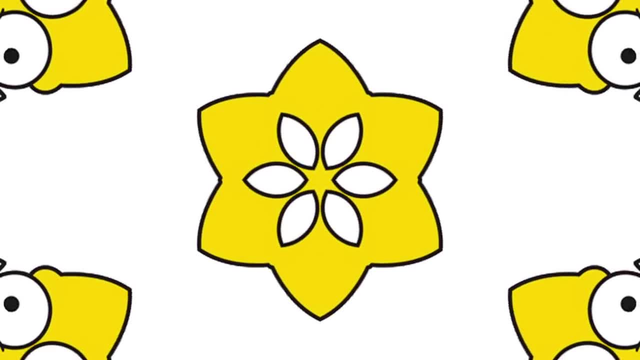 and then we'll argue about that And then I think ultimately Mark Carney, the governor of the Bank of England, will choose, But hopefully he'll go with whoever we think is the best person I've seen in the publicity and the articles about it. there are three or four people that seem to be emerging as the bookmakers. 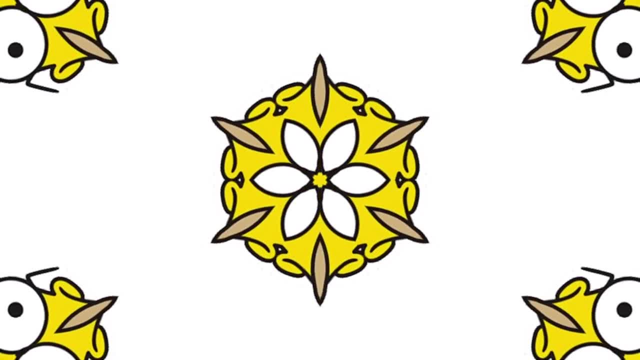 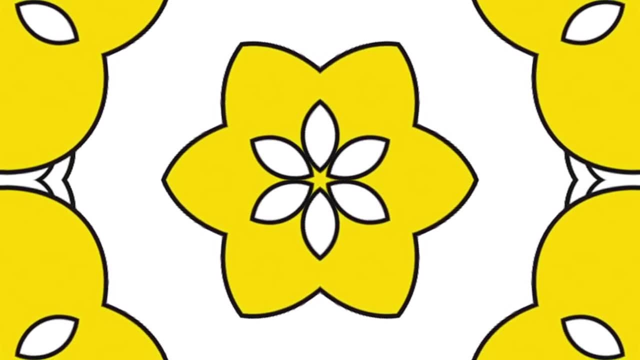 as favourites, As someone who's on the committee that will then decide. do you feel swayed by that? Or do you feel like this resistance? Oh no, let's choose someone unexpected, Let's surprise the public. Or do you feel, no, let's go with what the public wants. 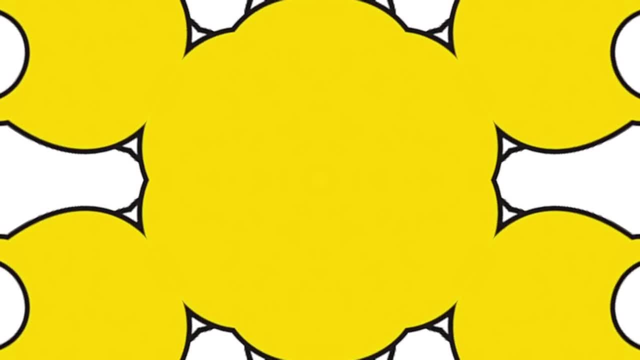 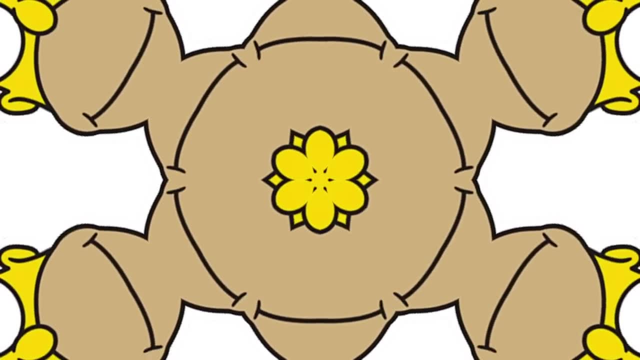 How does that work? What's your instinct? It's really frustrating because I can't say anything, Because if I say to you, you know what, I've heard some of those names and they were on my list too. Or if I say to you, actually I've got a completely different name. 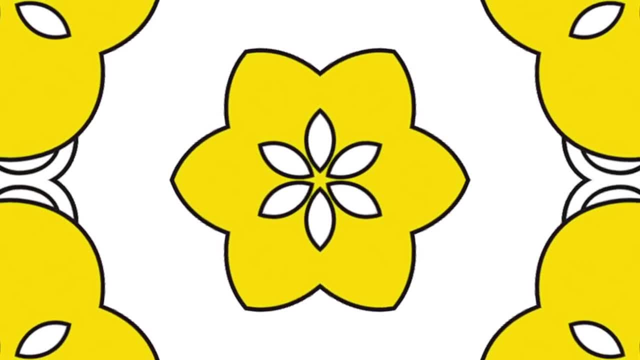 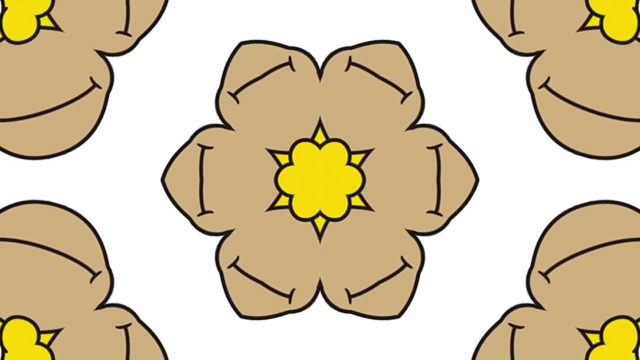 We can't really voice an opinion until we've come up with our final person. So I've just found it wonderful. The names have come up who I hadn't thought of, And there are other names that are obviously much more familiar. And there are people like Newton has already been on the one pound note, I think. 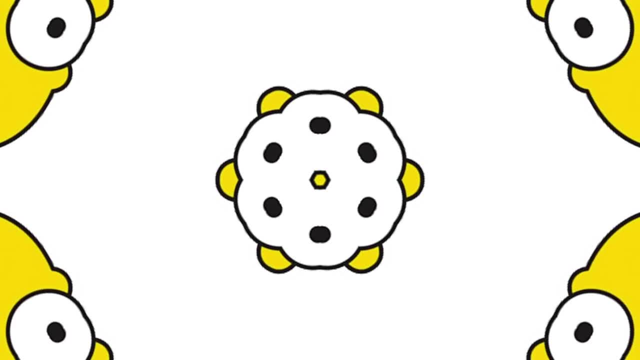 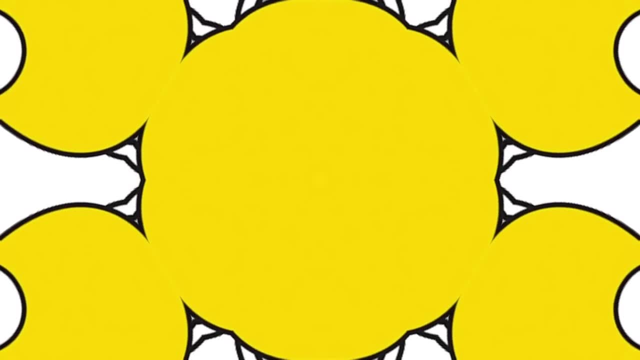 And has also commemorated on the pound coin because he was secretary to the Royal Mint. Yeah, he ran the Mint, He ran the Mint, yeah. And so I think he may have been the person who came up with the idea of milling around coins, so you couldn't chip away at them. 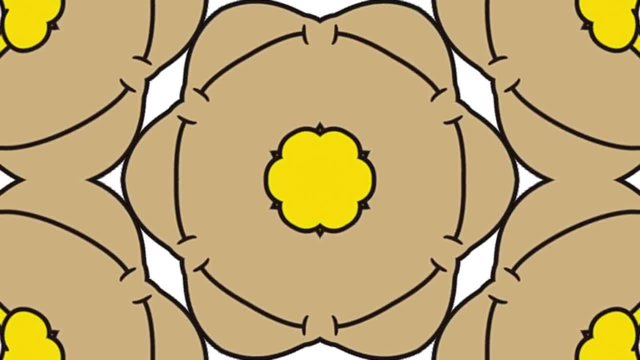 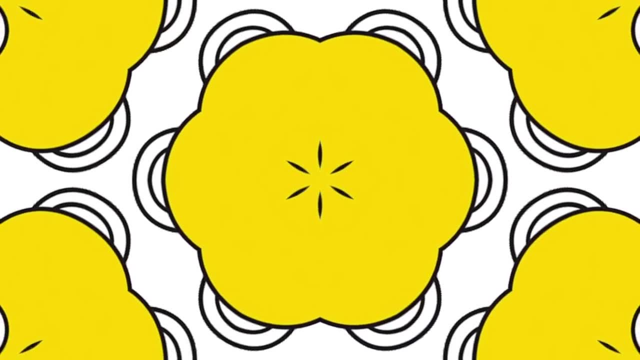 So he's been commemorated. Darwin's been there. There have been engineers like Watt and Bolton. I think, Faraday, Faraday, Faraday, Faraday, Fantastic to see him there standing in front of the bench at the Royal Institution. 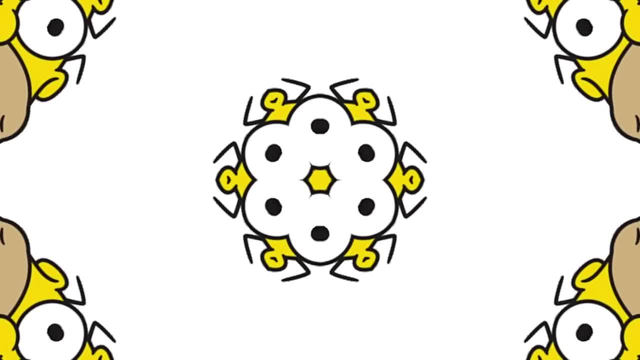 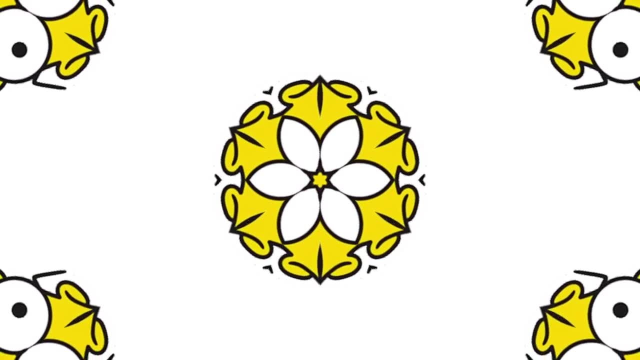 So there have been many great scientists and we just need one more for the new 50 pound note. Have you been getting like emails or phone calls or people wanting to give you their two cents worth? Or have you been like? have people been like leaving you alone and realizing that you're like, quarantined from being influenced? 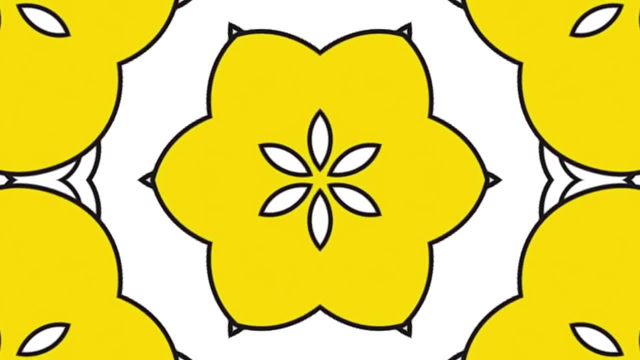 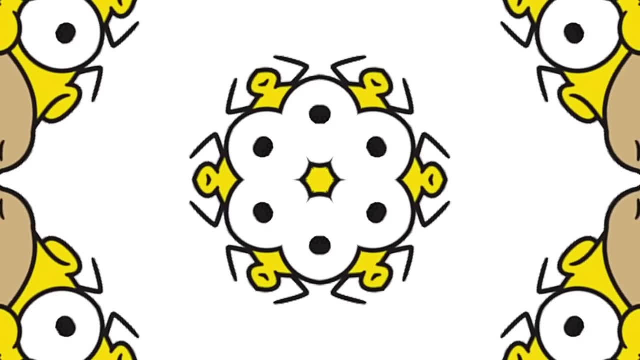 No, no, I've had a few suggestions. My own son came along with me to the when it was all announced at the Science Museum. Yeah, I took him along as well. So he's had a good think about it and he's got a definite, strong suggestion which I will. 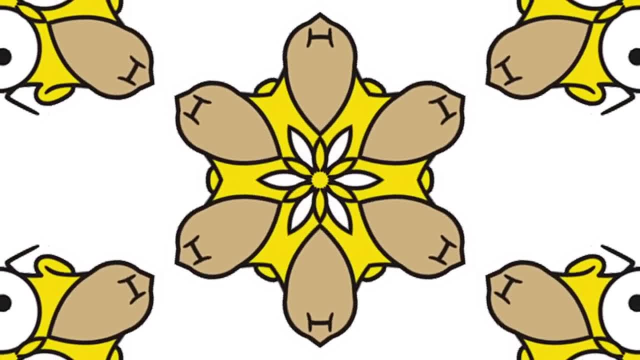 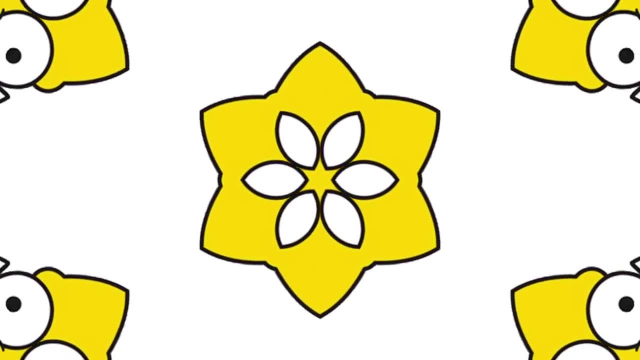 I will not reveal either, Oh no, But I've also encouraged teachers. you know, get the classrooms talking about this, Get them to figure out who they think should be on the 50 pound note and run your own poll and let us know as well, because we'll take all of those into consideration. 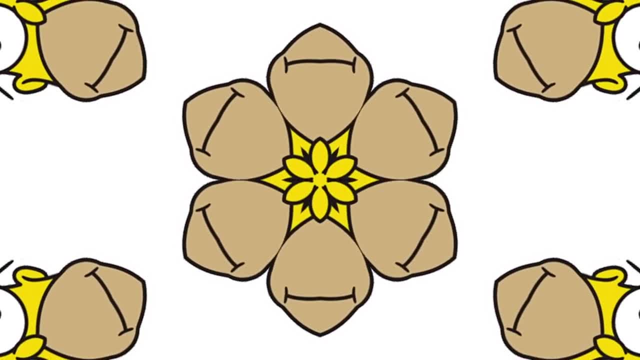 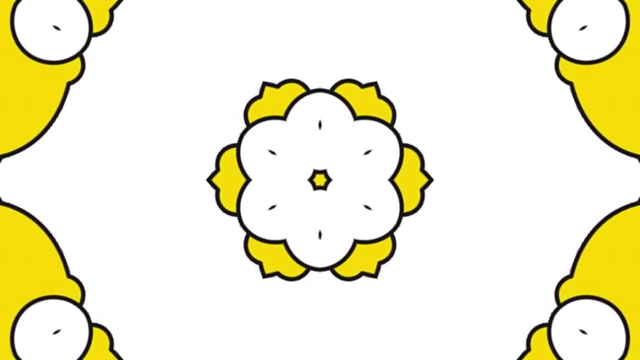 Okay, We made a video on one of my YouTube channels where we made some suggestions, So I'll send you the video as well. Oh, excellent, Great, You can see what you think. All right, then, Starting properly. then I was reading up and I didn't realize that you are from Somerset. which is where I live. Yeah, Yeah, Yeah, The West country. Yeah, That's it. You were born there. I was born in Wellington, which is a very small town not very far from where Thomas Young was born. Thomas Young was born in Milverton, just down the road from where I was born. 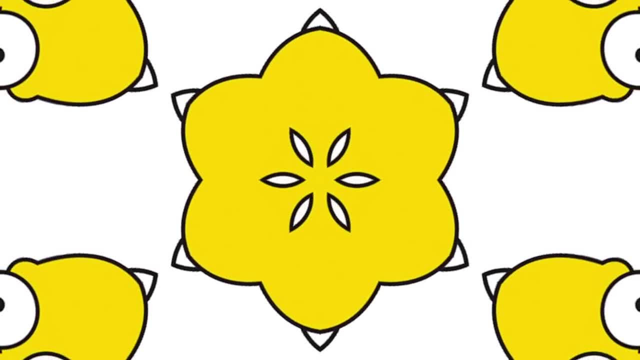 And he went to Emanuel College and I went to Emanuel College And he's a great, brilliant scientist and I'm not. That's where the similarities end. The powers had to diverge at some point. So yeah, no, very, very proud. 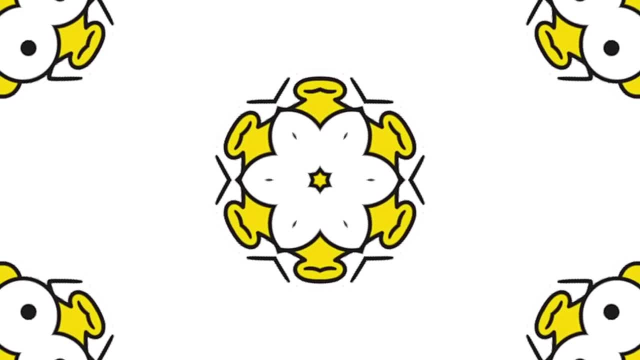 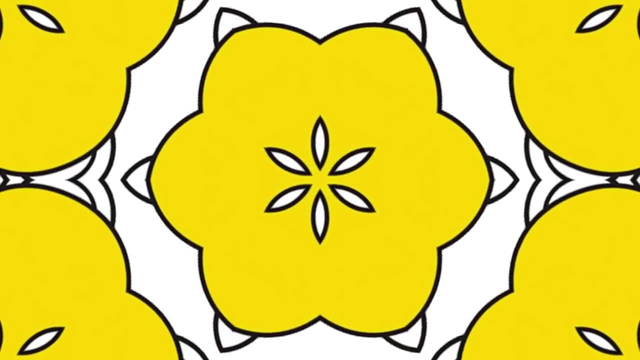 And my family for some very odd reason. well, they're from the Punjab originally And for some very odd reason, back in the 1930s, So they were among the very first wave of immigrants from India settled in the West. country. So when I was growing up in the 60s and 70s everybody West of Bristol who was brown was from my village. So if you go to a place like South Malton and Tiverton and Barnstable and Taunton and 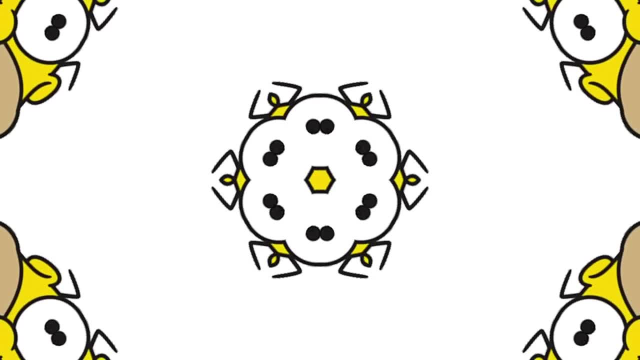 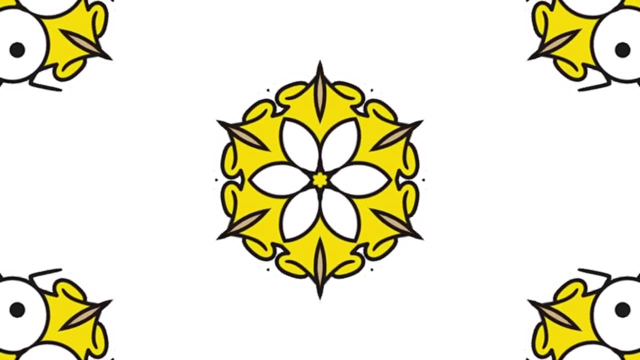 Exeter. anybody there who was Indian, was related to me or was a next door neighbor back in the home village. And I remember the first person I ever met who wasn't from our village, who was sort of of Indian descent. when Idi Amin expelled the Asians from Uganda we had a family settled. 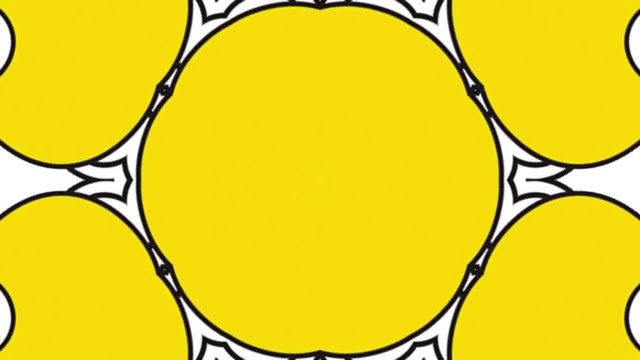 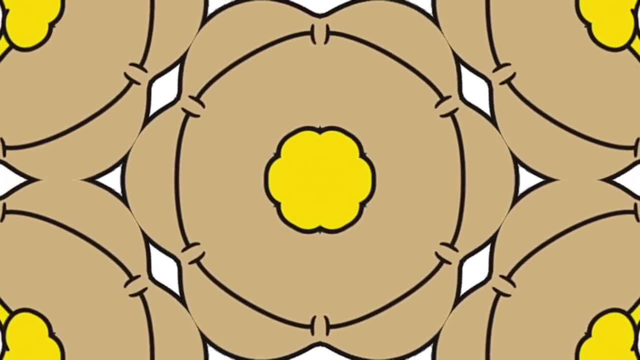 in our town. But yeah, so a very happy childhood. loved being in the West country, still very, very fond of Somerset and always enjoy going back. Did you ever find out why your parents chose like a village in the West country as opposed? to London or the other places or I think if you go back to 1938, you know late 30s, there was kind of no obvious place to go. There wasn't an Indian community in Somerset, There wasn't an Indian community in places like Gravesend or Southall or Birmingham or Wolverhampton like there is now. So there was no obvious place to go, And I think there had been some people from our village who'd gone to the West country and who'd sold sort of door to door And that's sort of what our family did as well. 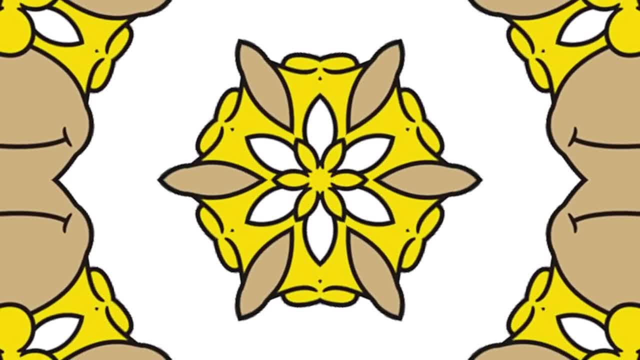 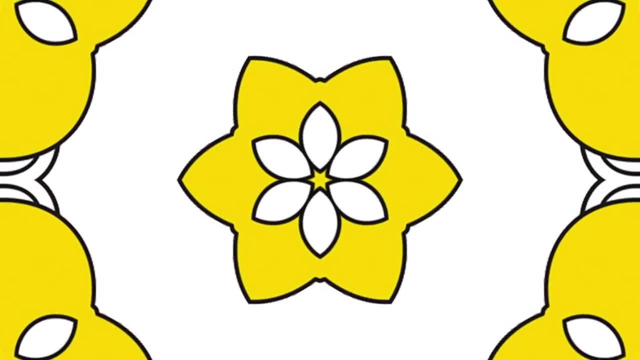 They would sell things to local farmhouses. you know Wellington boots, overalls. I remember my grandfather passed away. I wrote a little story for the local newspaper and got letters from people who'd remembered him because you know, you remember a big brown. 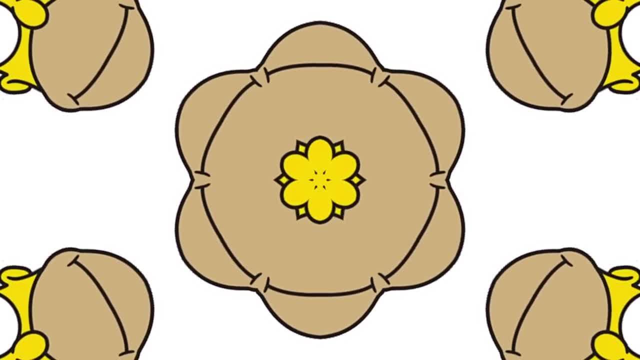 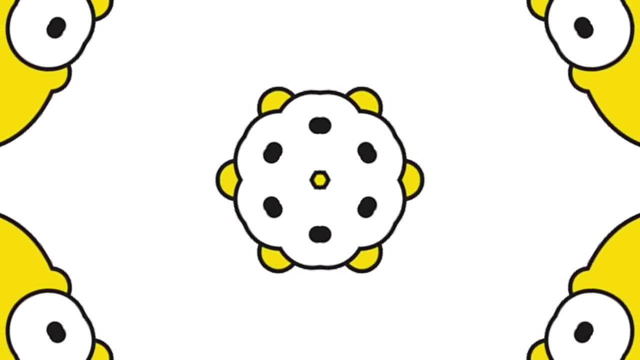 guy turns up your door in the 1940s, by that stage you'd remember him, And so I remember a woman who said she just distinctly remembers getting a pair of socks when she was about five or six, because getting a new pair of socks was a big deal. 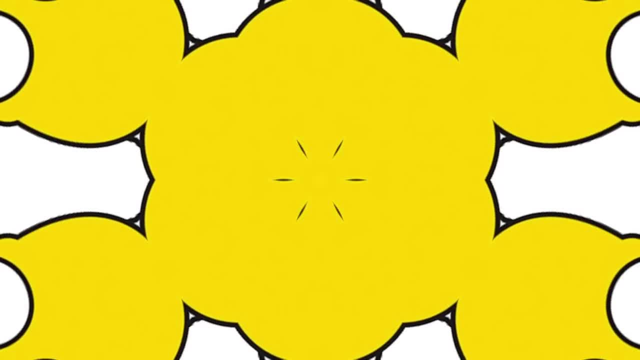 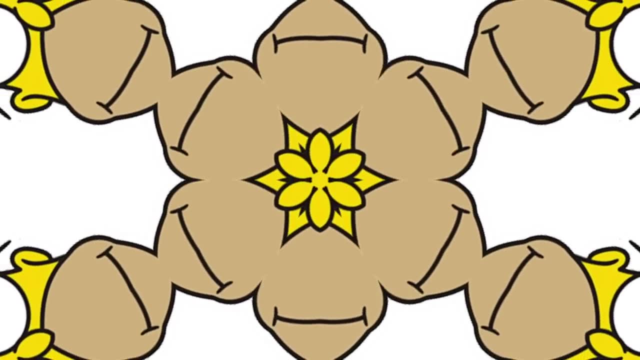 And it was my grandfather who'd kind of knocked on their door and sold them. So yeah, there'd been sort of tinkers selling from door to door just prior to my family's arrival. Yeah, And I thought, well, okay, that's where we'll go. 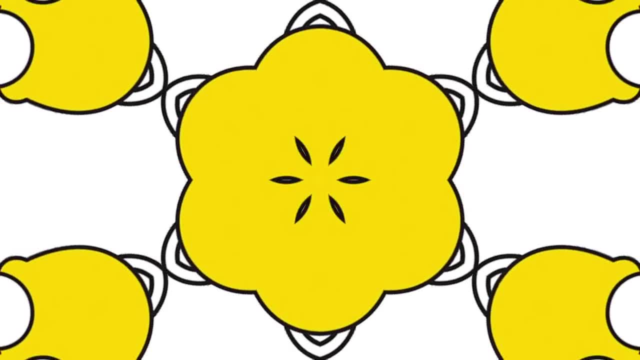 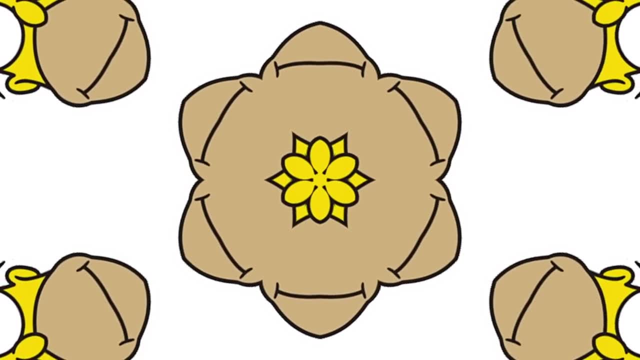 It was fairly random, to be honest, I think. What were you like as a boy For a start? were you like, were you a science and math geeky kid, or were you like into sports or what was what? I've guessed you were going to be who you became. 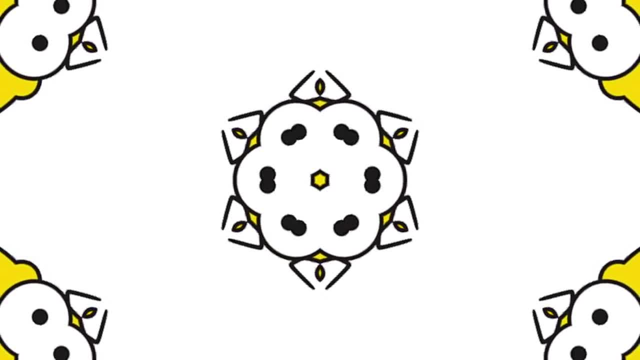 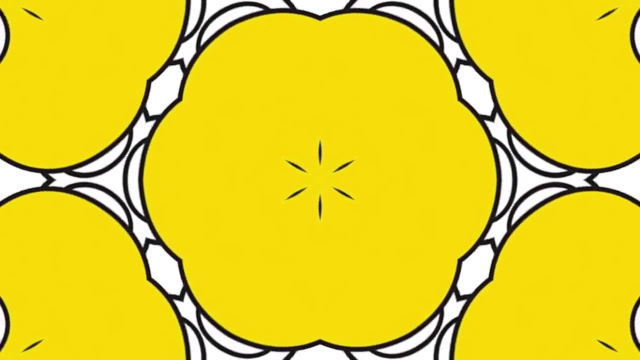 I loved football. I used to collect all the cards and kind of name all the players in the first division at the time. What was your team? Derby County, Nice, Very local to Somerset. Yeah, How did you end up with them? I had cousins who lived in Derby, So that was the reason for that And it was a good time to be a Derby fan, because they won the league a couple of times and it was through the Brian Clough era and many other great things. 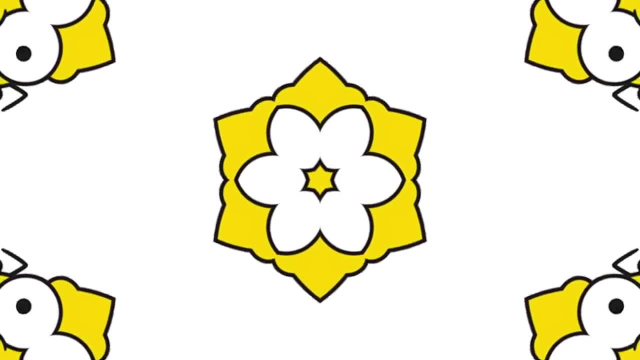 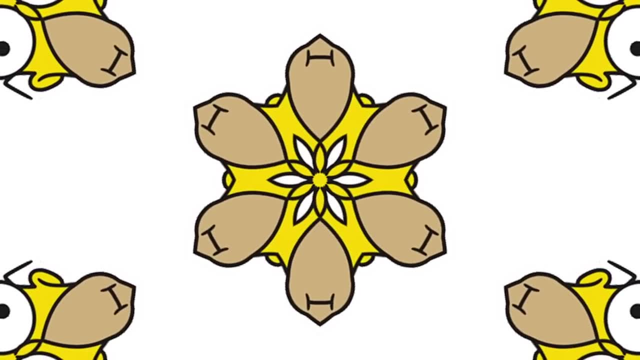 So I loved football and I loved television. I used to watch television, you know. at any point TV was on I'd be watching it Like wholesome good TV, or just like fluff, Just anything, You know. when I was a bit older, I used to love watching Tiz Wars. 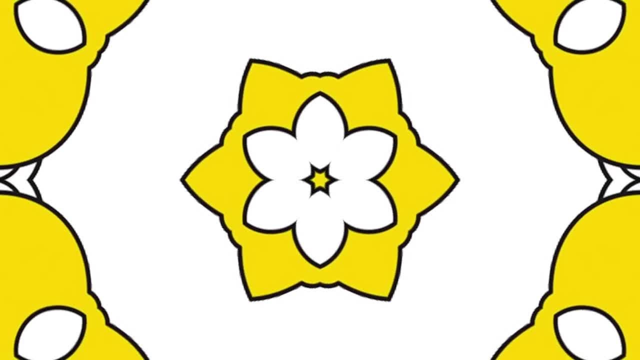 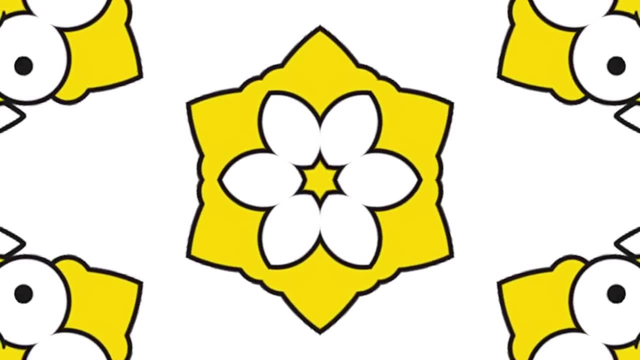 Do you remember Tiz Wars? Today is Saturday. watch and see. it was kind of an anarchic TV show with people like Chris Tarrant. And then when the video recorder came in, you know, I would just watch even more television. 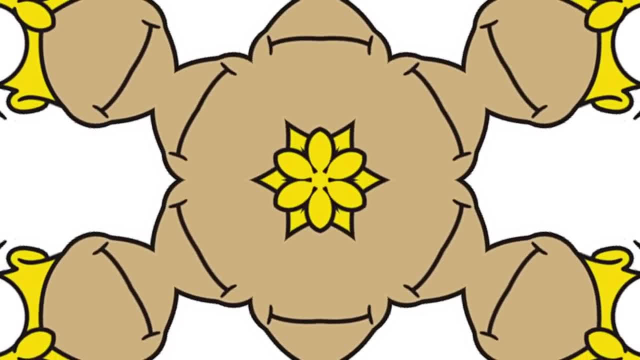 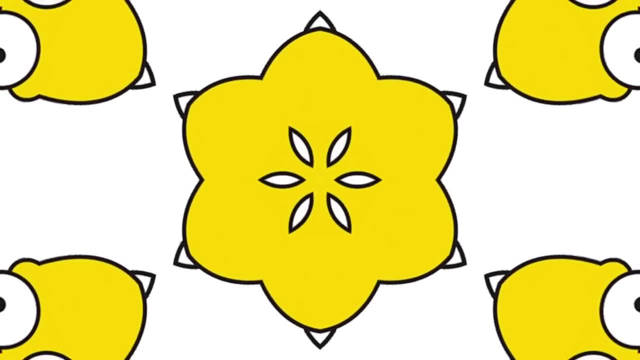 So I love TV. I love junk TV. I loved football. Were you good at football? Yeah, I was. I was pretty good. Yeah, I played football late into the evening until the sunset and then I'd get home eventually. But I also love science. 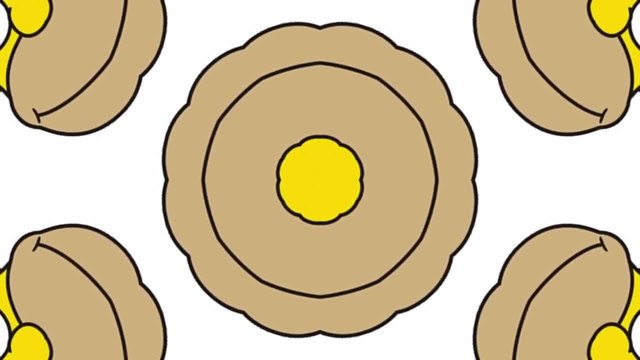 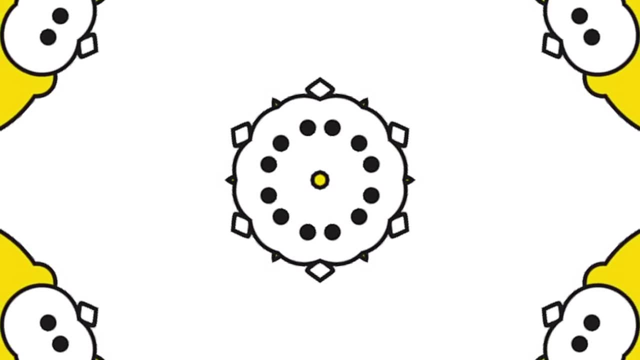 So science was the thing I did at school and I loved math and you know people were landing on the moon. I can't quite remember the first man on the moon landing, but I can remember a lot of what followed in the early seventies. 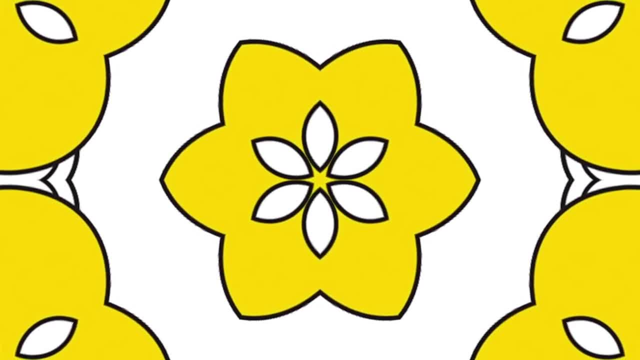 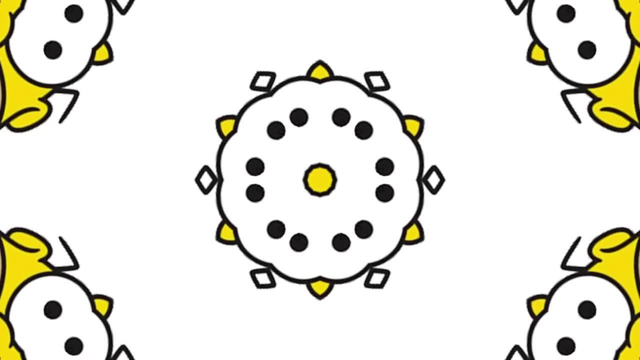 And so, yeah, That was who I was And I kind of just knew that physics is what I loved. I grew up watching Tomorrow's World and people like Patrick Moore and James Burke and Magnus Pike. One of my books I sort of dedicated to all those heroes that I grew up watching on television. 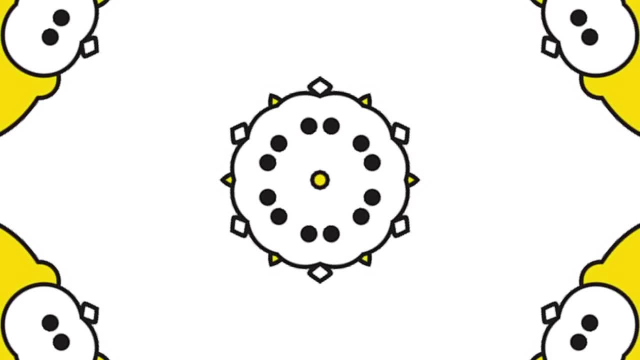 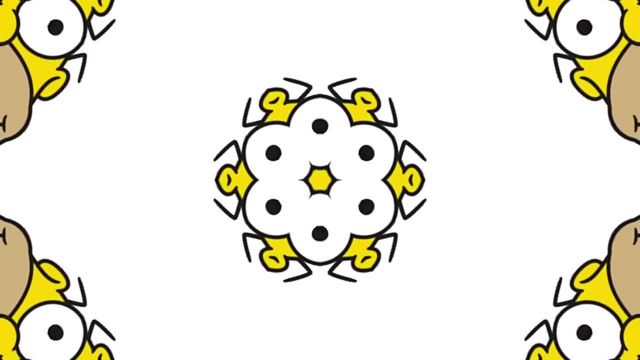 Yeah, Physics, the universe, Einstein- where did it all come from? was just the thing. that was always what I was going to do. It just seemed like the most fascinating thing in the world. I had fantastic math teachers, had a great physics teacher, and then I went to university. 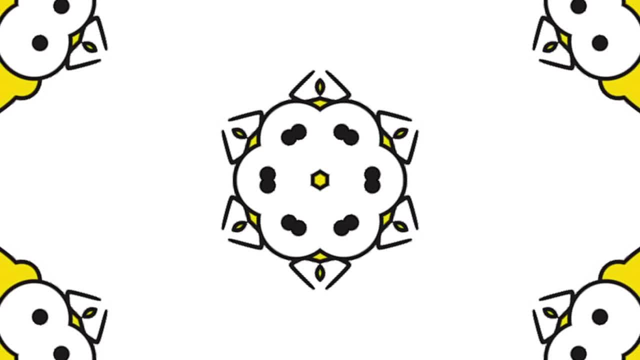 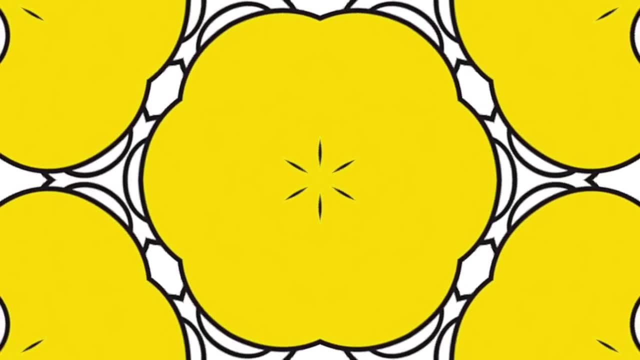 and did physics, and that was it Just still while you're young. one last thing I have to ask because of your Indian background. you said you're really into football. Were you into cricket A little bit? Yeah, I mean being at Somerset- Joel Garner, Viv Richards, you know, occasionally going out. 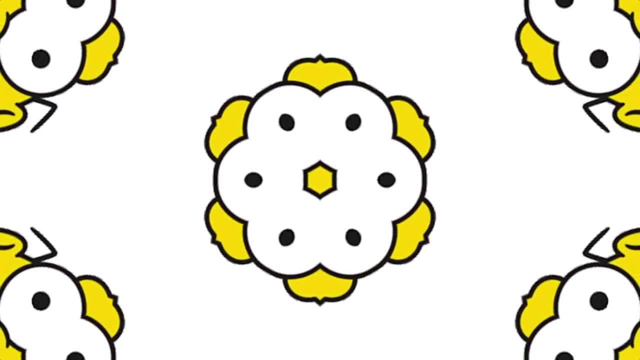 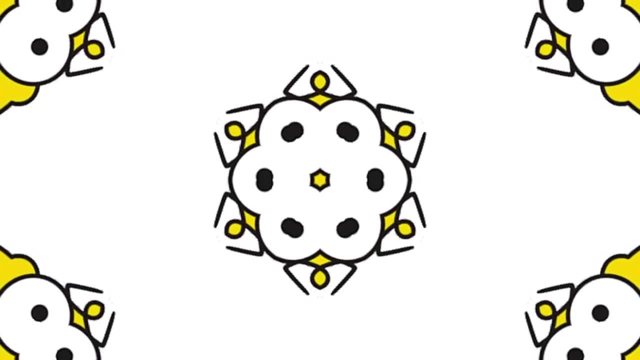 to Taunton and watch Somerset play. So I enjoyed cricket as well, but football was my real passion. It sounds like, compared to a lot of other people who I speak to who have become scientists and mathematicians, you sound like you were quite well rounded. 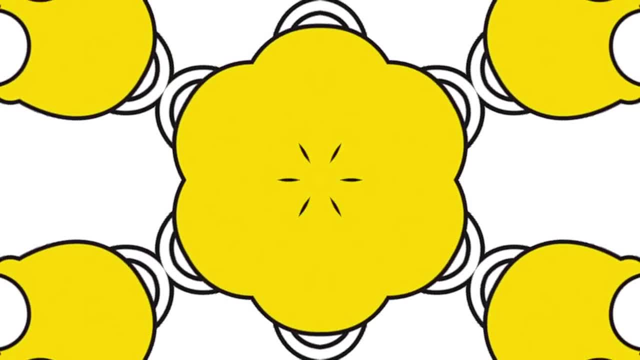 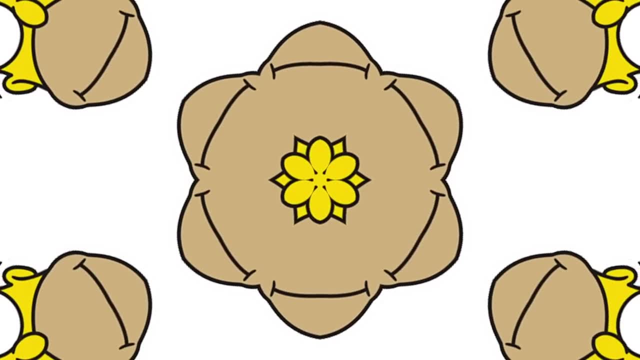 You weren't just like this total math nerd. You know you were liking your sport and popular culture and it sounds like you were like pretty normal. It's slightly different to some of the other people you've spoken to, because I'm more of a journalist now than a mathematician or a scientist and never ever was a mathematician. 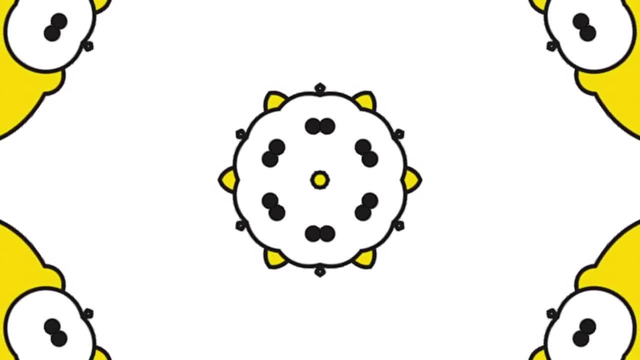 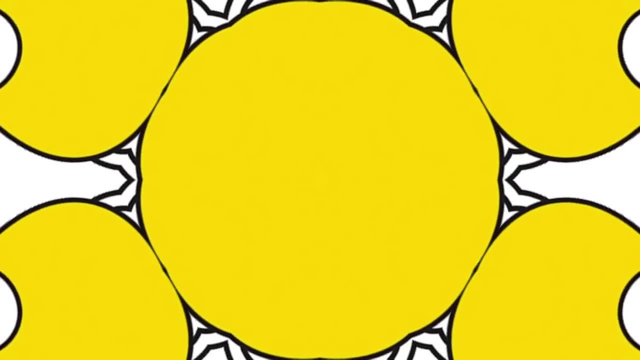 really, It sounds as though I'm going to say: well, I may be not typical to your usual interviewee because I do something different to your usual interviewee, But actually what I'm going to say is that I also interview mathematicians a lot, and have worked with physicists and others and I tend to find that they're hugely well rounded. So when I was at CERN, you know, physicists would run the local marathon. they go skiing, they do extreme sports. They'd be very accomplished musicians. 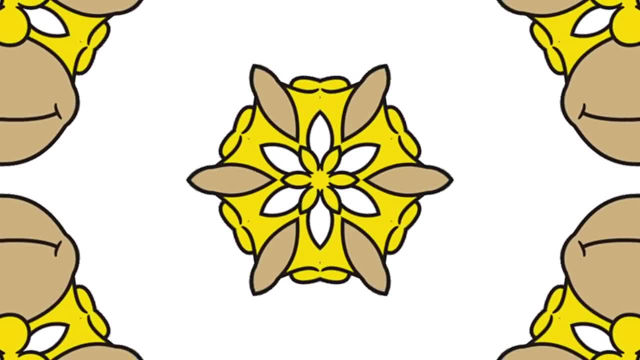 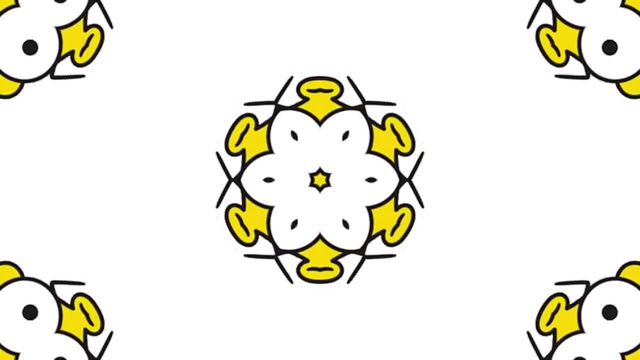 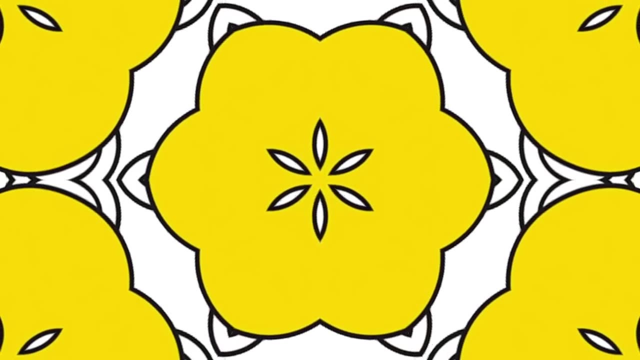 So I tend to find that mathematicians are passionate about many, many things. They're curious about anything and everything. That's my impression, Whereas if I tend to meet an artist, they tend to be scared of science, Whereas scientists, I think, aren't scared of very much. 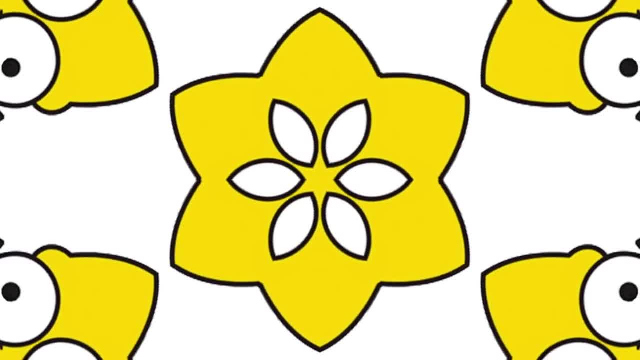 I agree with you when it comes to adult scientists and mathematicians, But when I hear them describe their childhood, I mean they could be, just like you know, people who are very, very good at math. They're very, very good at math. 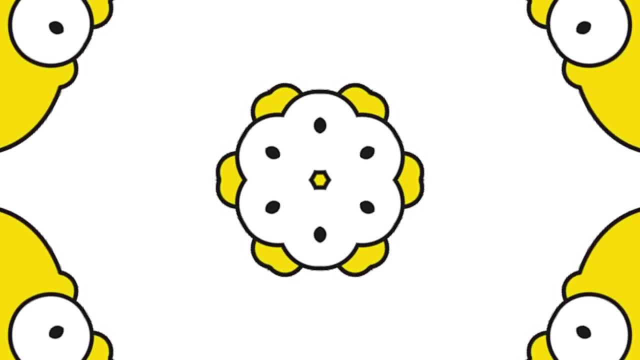 They're very good at being humble, But they always describe themselves as quite nerdy as a kid. They grow up to become quite well rounded people, I agree with you, but they always say, oh yeah, I was always the nerdy kid at school. 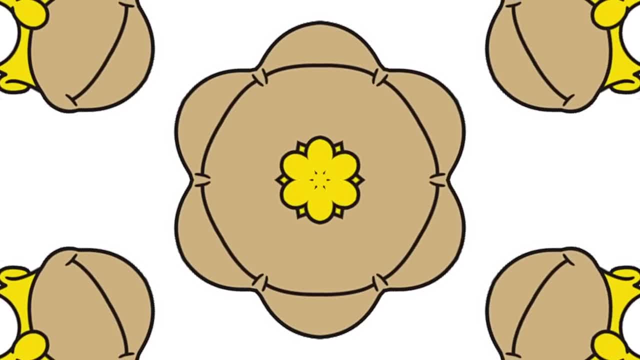 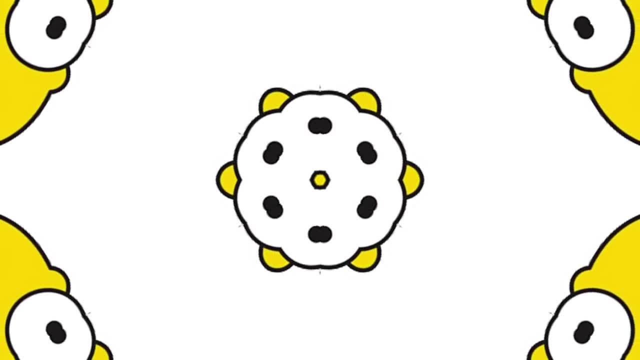 They're still the nerdy person there, but they're nerdy surrounded by all the other nerds. So I don't think they've changed really. It's just that they've become part of a bigger community of concentrated nerdity. Coming back to your story then, were you being influenced by your parents? 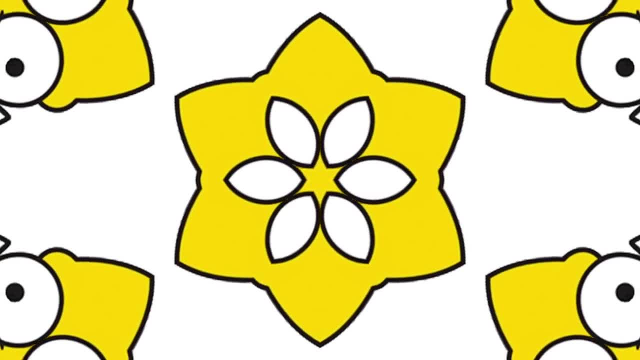 Did they say, yeah, you should be a physicist, that's a good path for you. Or were they saying, no, no, you should be a doctor. No, So my mother never went to school, so she can't read or write. 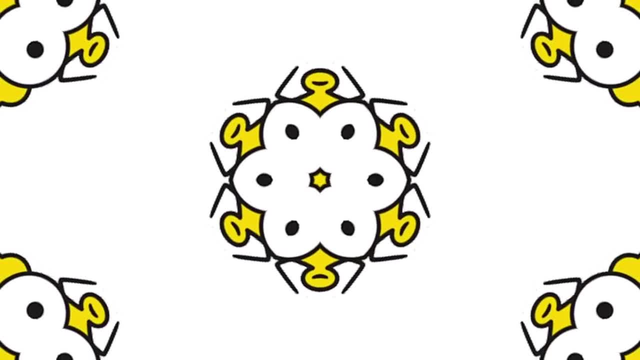 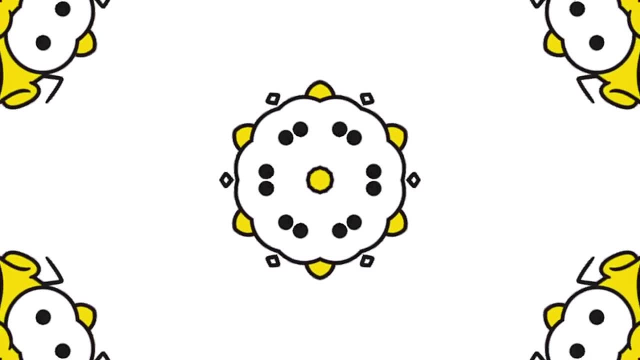 And my dad can sort of read a newspaper, but that sort of struggles as well. So when they came to this country, they're both very bright but they're not educated, So they just worked incredibly hard to build security for themselves and also, obviously, 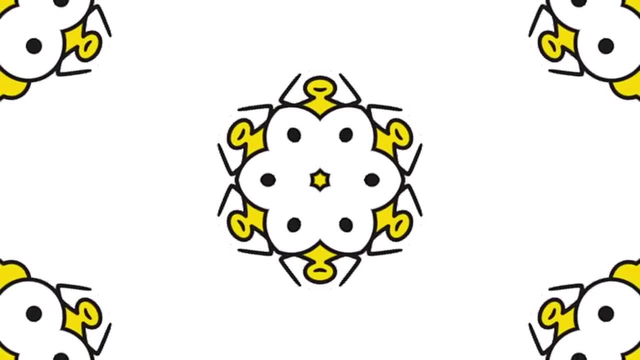 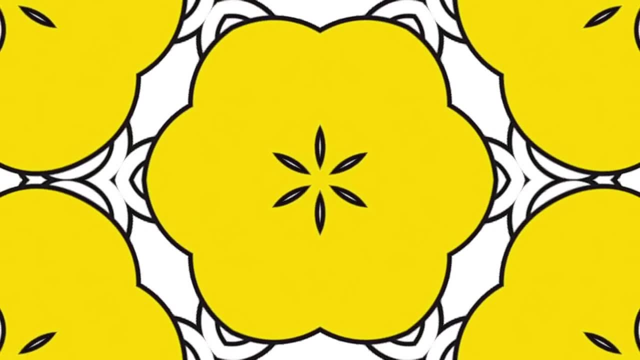 for their children. So when my mum left India she never saw her parents again. She never even spoke to them again because even a phone call would be impossible. So I think for my siblings and myself the goal was to continue that security. 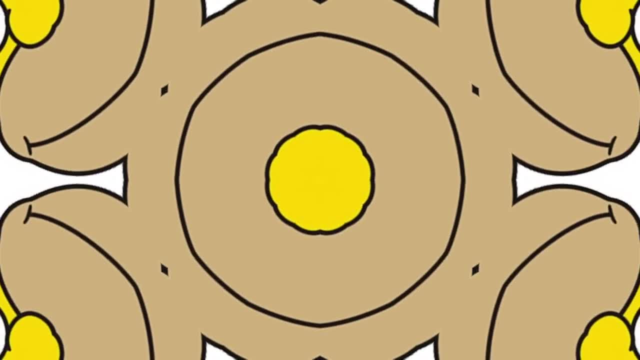 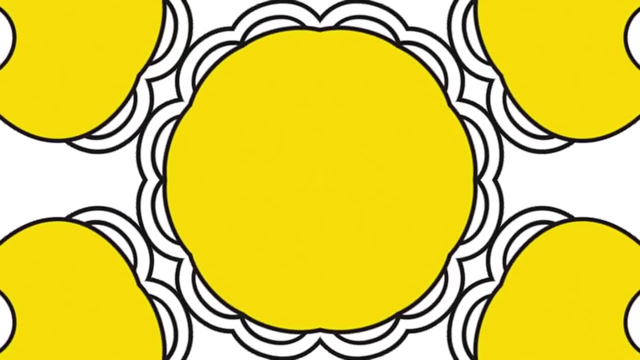 To go into business or to become a doctor would have been a dream scenario for my parents, But that was it. The things that they were comfortable with, the things that they were familiar with, the things that they knew would bring security to all of our lives. My two brothers and sister went into business as well, as well as my parents. But because I was the youngest, and I was the youngest by quite a long way- my sister's about eight, nine years older than me. I was the youngest. I think I was cut a bit of slack and they always thought, oh, eventually he'll come into the family business and he'll work and do something sensible. But I kind of just did what I did And I still think my parents don't quite understand what a physicist is and probably don't even. 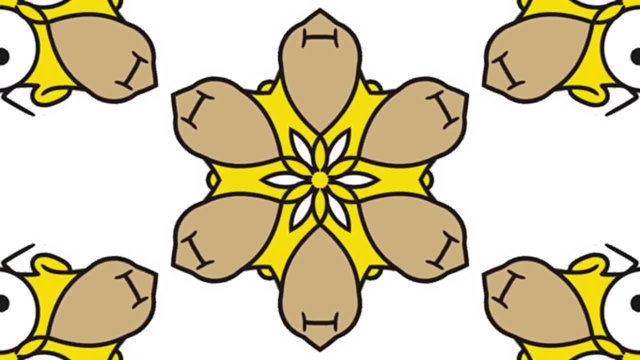 quite remember that that was the degree I did. So I kind of just did that. I just knew it was the right thing for me and I just knew it's what I loved And I think, what clicked. so I did a degree in physics. 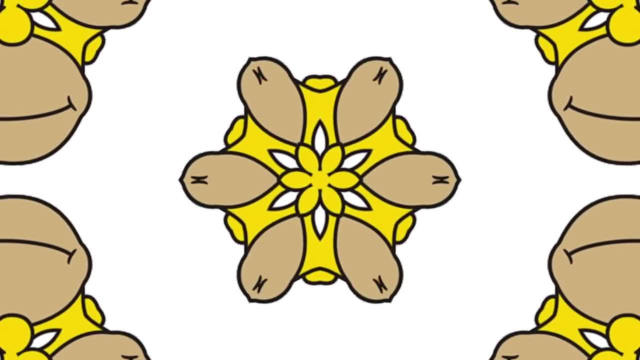 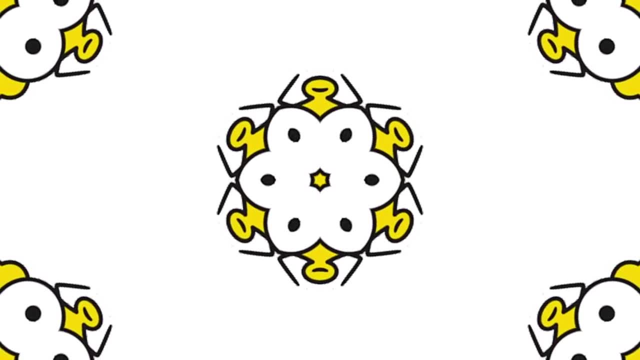 I did a PhD in physics, They were probably even more confused about what that was all about. And then I went to work for the BBC And I got a job on Tomorrow's World. And that was the point at which they think, oh okay, he makes programs about science. 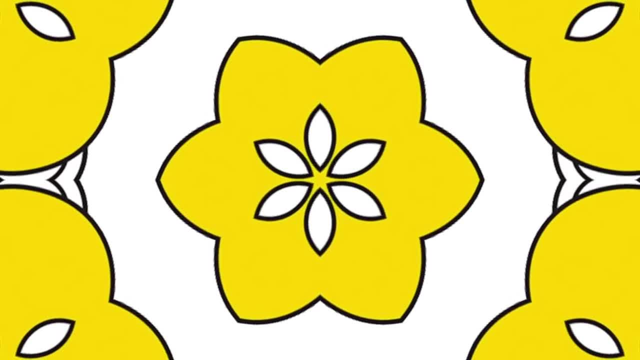 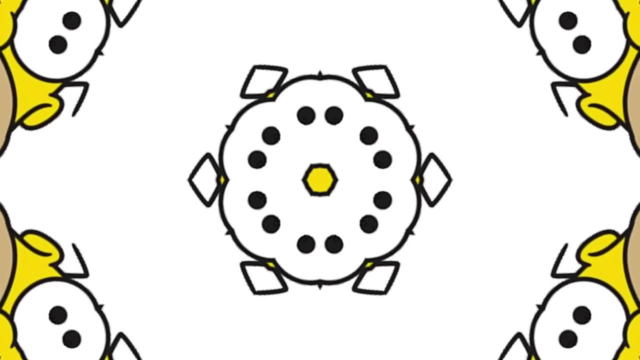 for TV. Okay, we can understand what that's all about, So that was a point at which they could explain to their relatives- our relatives- what I actually did for a living, which was to make science programs on television. Like me using the 50 pound note to describe it. 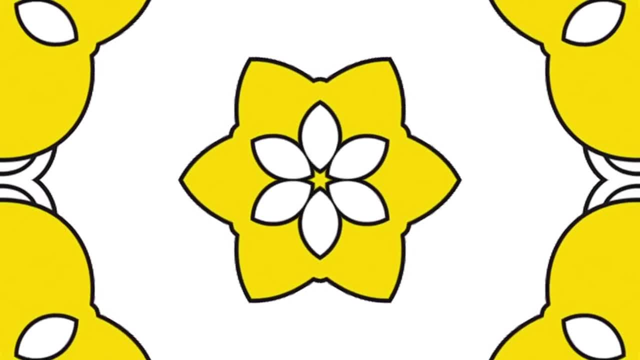 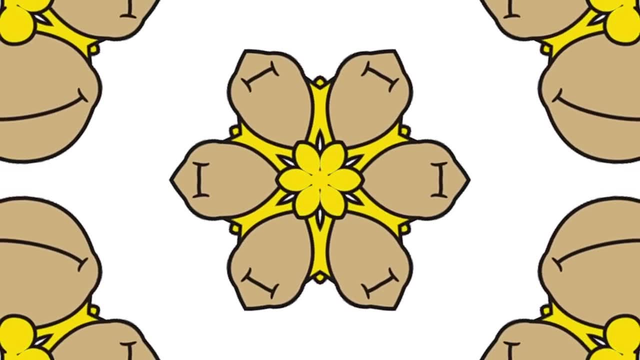 Yeah, exactly, And they could see that I was happy doing what I was doing and they could see that I was successful and they could see I had a secure future, I could pay my own way, and so on. So at that point there was no need to try and entice me back into the family business. When I was a kid, I used to work in the markets. Again, we used to sell places like Glastonbury Market. I remember when there was the incredible England comeback against Australia with Botham and Willis. How have you wedged that into a number five podcast? 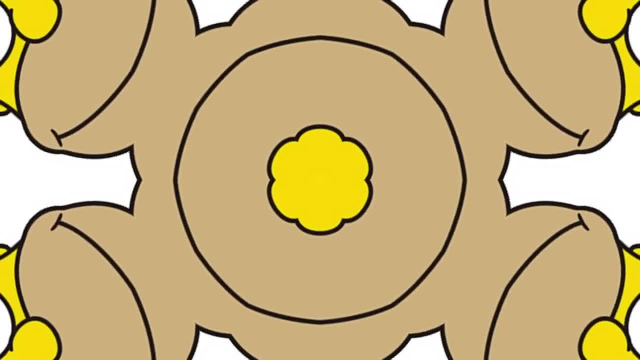 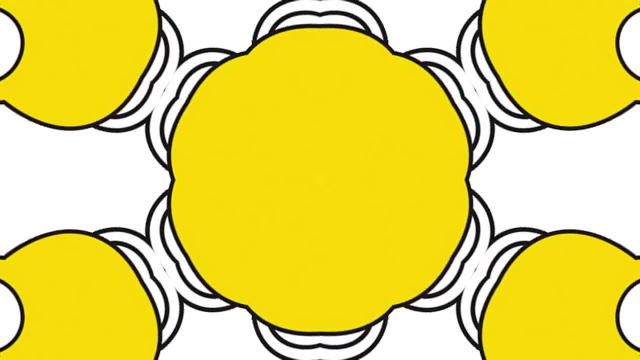 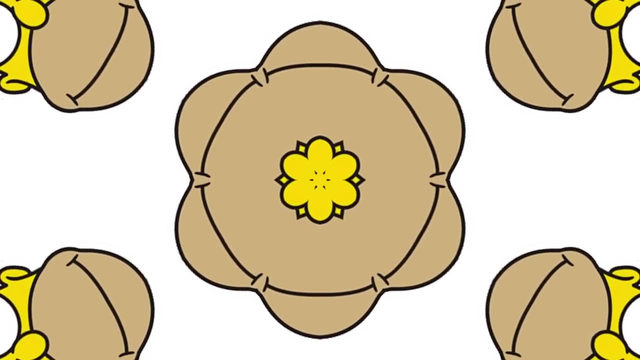 My lasting memory of markets is getting up on freezing cold days and building these little stalls. Yeah, I remember building these little stalls with big, heavy iron pipes and pulling the canvas over it and getting up at five in the morning. All of that was a misery, but that sunny summer's day in Glastonbury when England were coming. 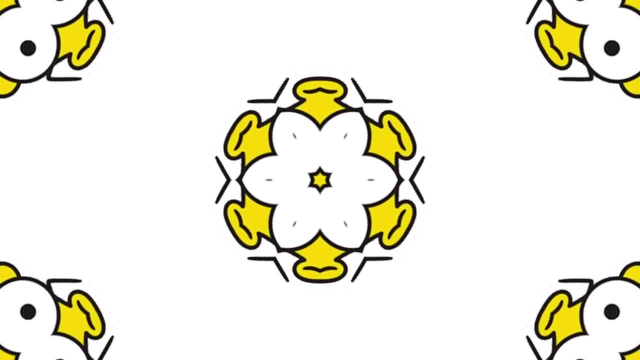 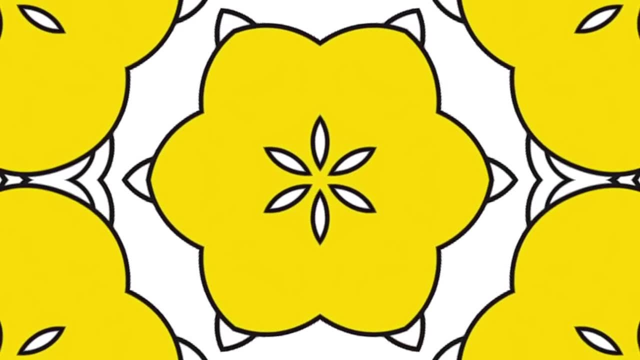 back was amazing. So I used to work in the shops and I'd run summer stalls and Westman Supermare. So I did all of those things And when we got our first computer to run the business, I remember trying to program that and getting that working and doing stock takes. 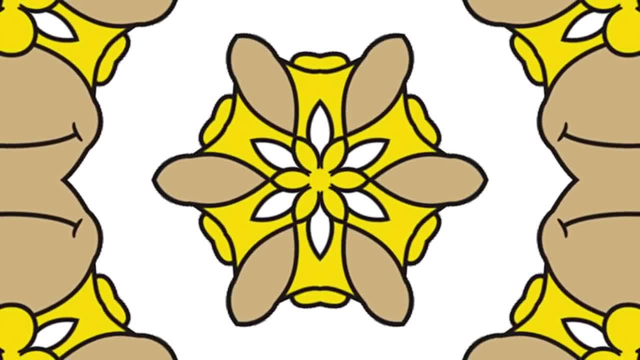 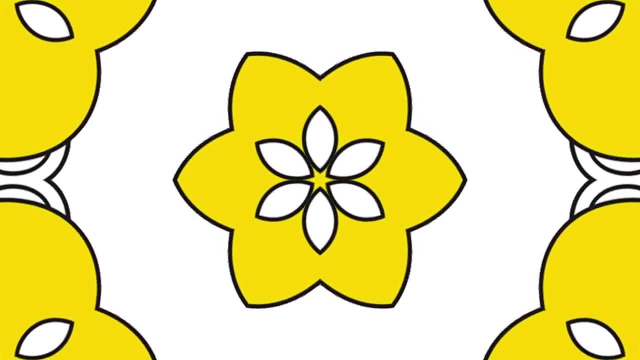 So I did all of those things and I even remember when we had decimalization I could do the translations between shillings, pounds and pence to new money and I could help the customers do that and so on. So that was kind of one of the first times I actually found math useful. 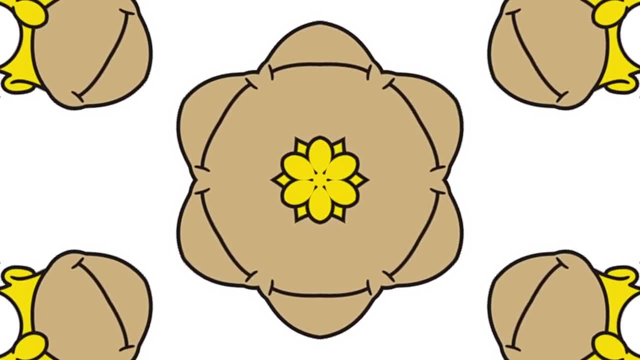 So I did my time in the family business. I learned a huge amount, I'm sure, but ultimately that's not what I was going to do And you can tell from my dress sense I didn't learn anything about fashion from that business. 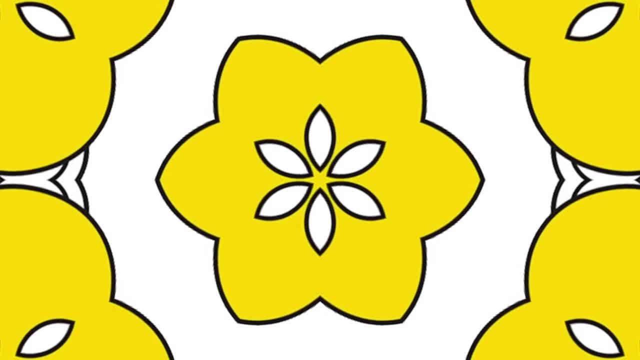 which was women's fashion clothing retail. What was your PhD? It was in particle physics. So, again, that's the kind of physics I love. That's what I wanted to do. So I did my PhD in particle physics. That's the kind of physics I love. 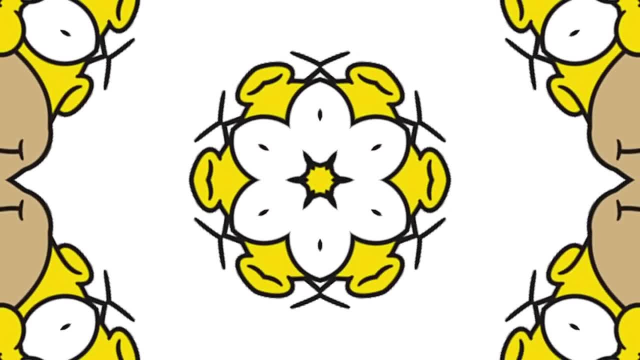 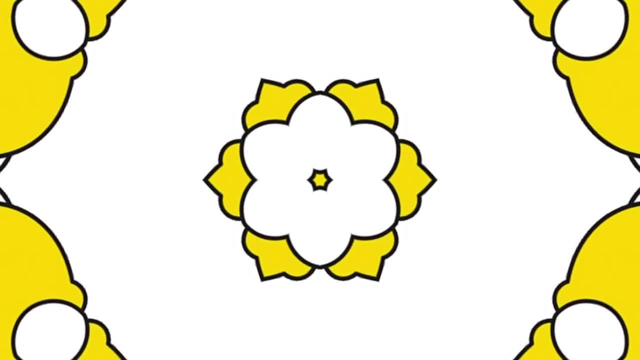 It's what I wanted to do. We have the Large Hadron Collider today, which is a super massive ring that accelerates hadrons. Yeah, Beams of protons against beams of protons. that's what it does. One of its feeder rings, one of the rings that accelerate stuff before it gets injected. 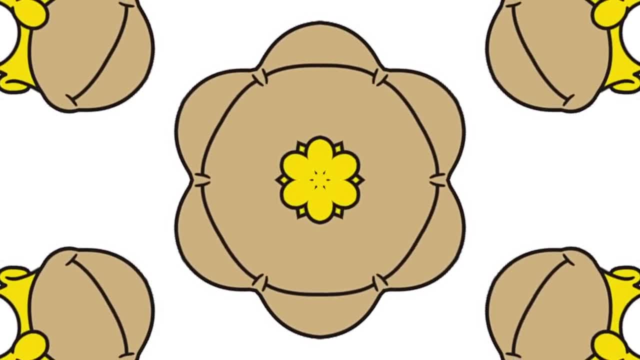 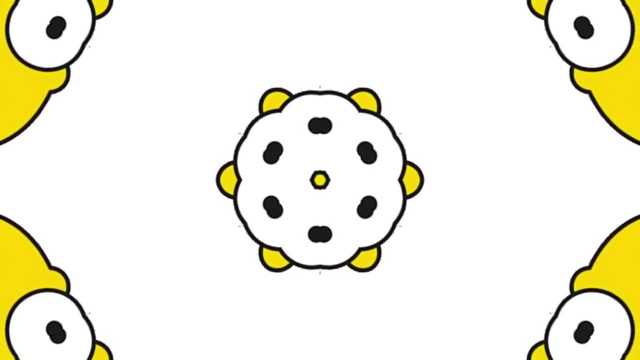 into the Large Hadron Collider is called the Super Proton Synchrotron, the SPS, And that's what I worked on when I was doing my PhD. I had two experiments, UA1 and UA2, underground area one and underground area two. 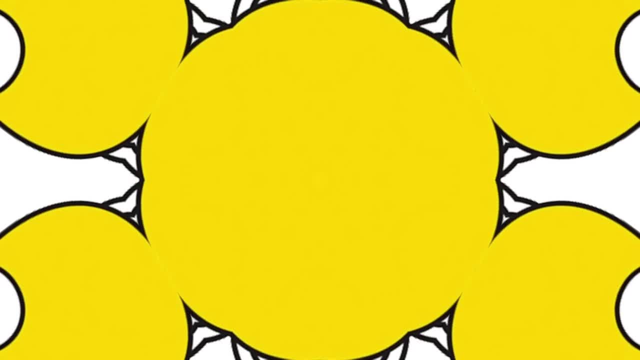 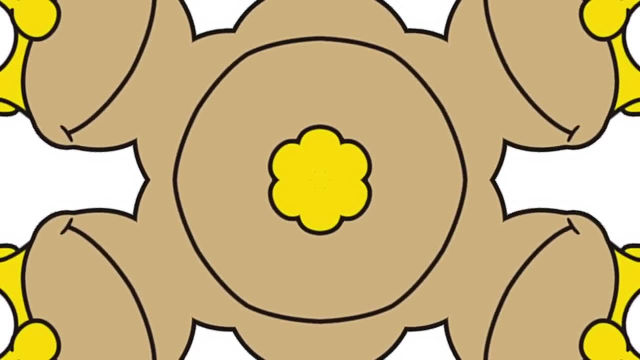 And prior to my arrival, they'd won the Nobel Prize for discovering the W and the Z boson, which are these large particles responsible for the weak nuclear force? And so, when I joined the experiment UA2, we were probing the W and the Z in more detail. 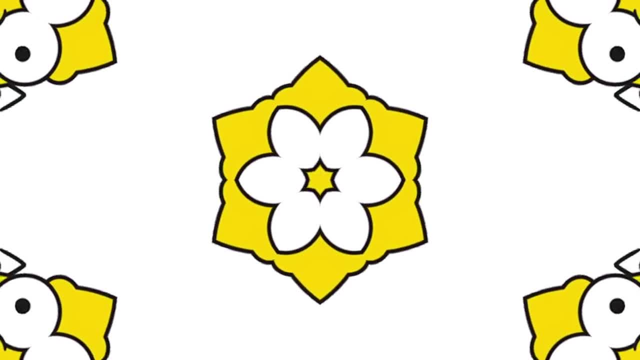 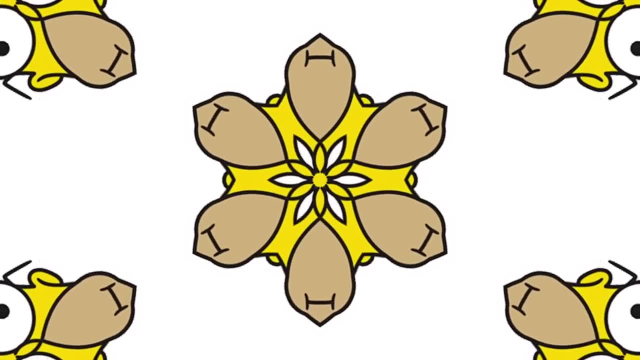 but the little group I was working on was trying to find the top quark. The five other quarks had been discovered. There wasn't a seventh and eighth one. There wasn't a fourth generation, so to speak, But there was a third generation. 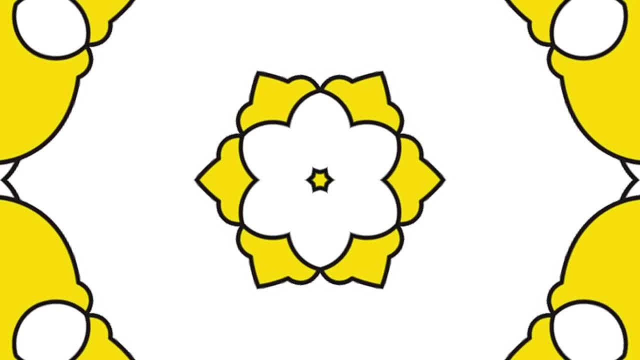 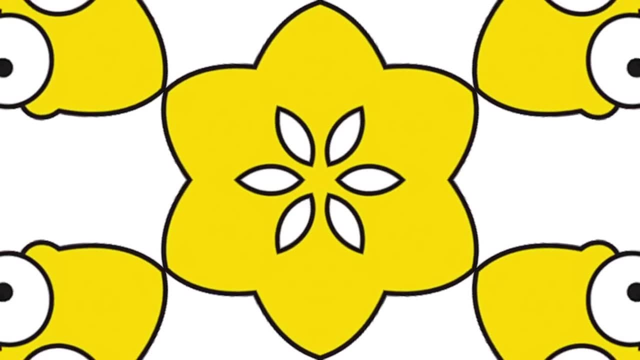 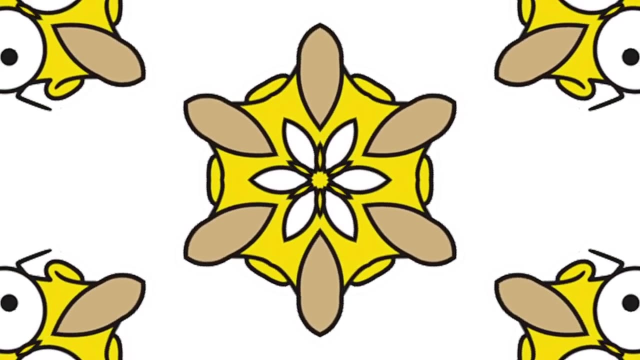 And the other half of that third generation. the top quark was missing. We looked for it, We couldn't find it. Ultimately, our accelerator wasn't powerful enough to create that top quark. So my PhD was all about saying the top quark must be heavier than a certain mass, otherwise 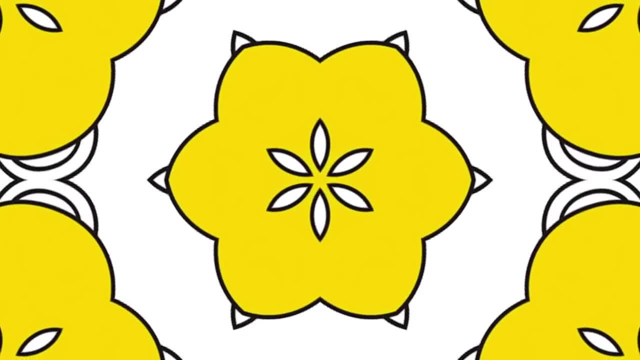 we'd have seen it. So you can put constraints on what the top quark can do. And that was sort of the bulk of my PhD was. I built a bit of the detector as well. Essentially, that's kind of what you do. 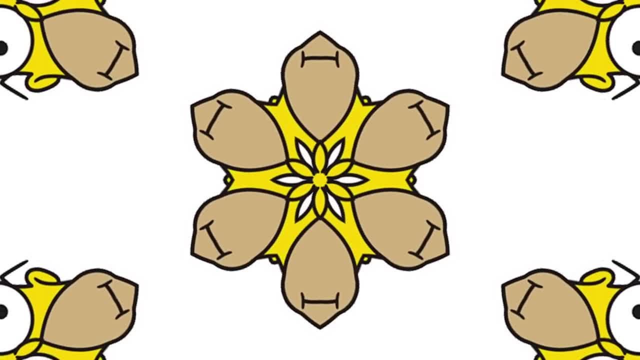 You build a bit of the detector, You do some physics and you write up what you've learned. And I loved it. I loved every minute of it. It's what I wanted to do. That's what I'd always dreamed of doing. 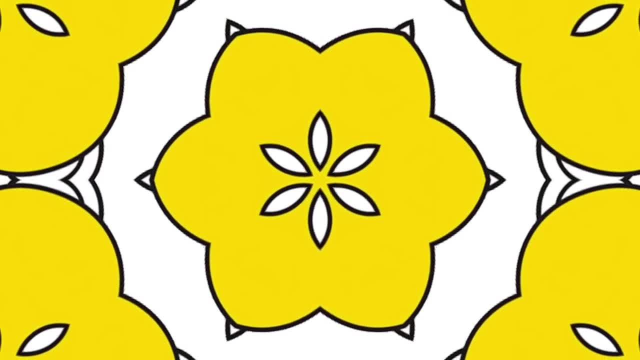 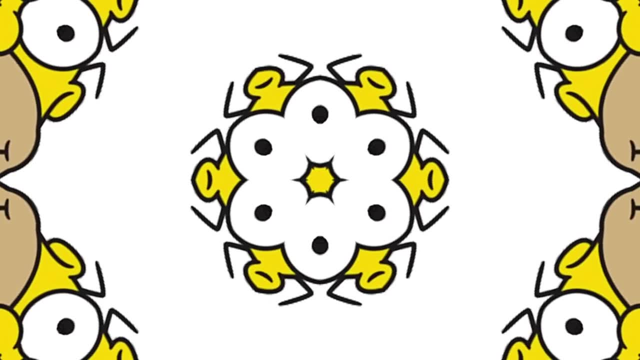 It's an incredibly exhilarating, exciting place. It's fantastic And I loved every minute of it. But by the time I was writing up, I could just see other people who were better than me, much better than me, quicker, brighter, and that they were the people who would go. 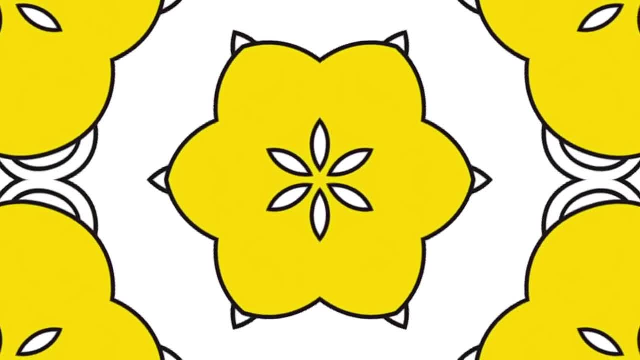 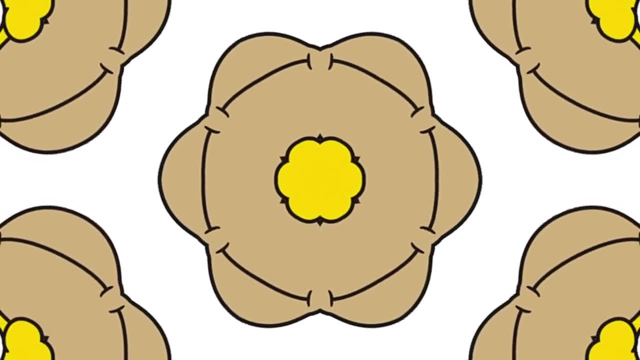 on to make great discoveries. Some of the people in my group have gone off to become director general of CERN and do other incredible things, And so then I thought in those final six months I'd actually applied for a couple of postdocs. 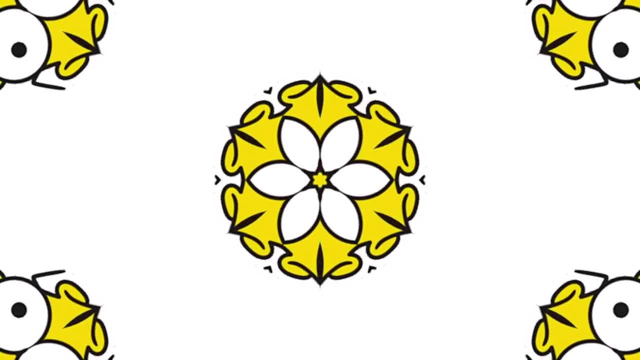 So I was in the process of saying, well, from here I go on and carry on to do more physics. But I just had this realization that what else could I do? What else should I do? What else am I good at? 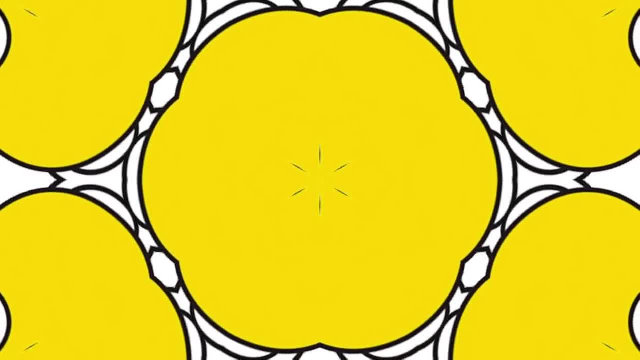 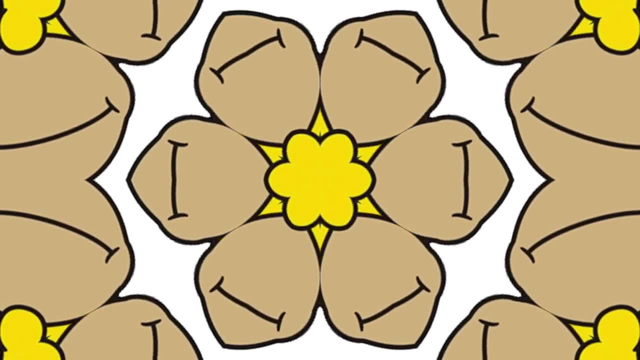 And then that's what took me back to television and thinking: I loved television when I was a kid. I love science. I love teaching and talking about science. Just before my PhD, before I started, I'd spent some time teaching in India. so teaching- 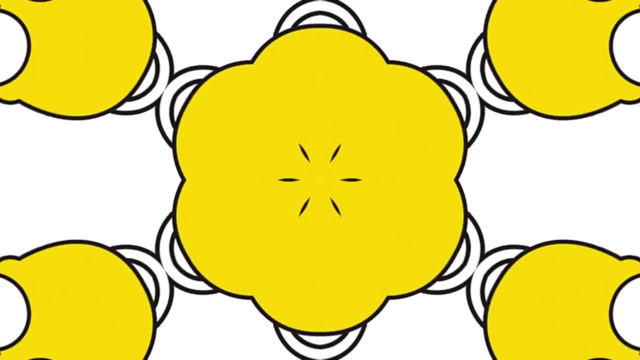 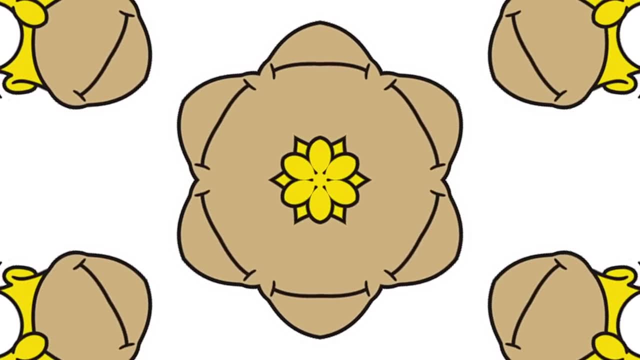 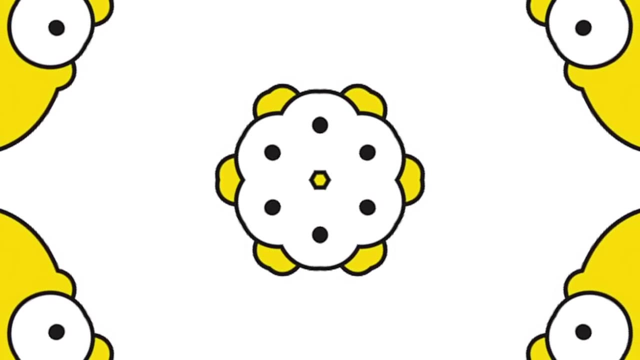 talking about science, watching science on television. Why don't I try and become a TV producer or TV director? So that was the next step. I was lucky enough to get a traineeship at the BBC for just six months. You say that so casually, but I mean. lots of people dream of working in TV and think 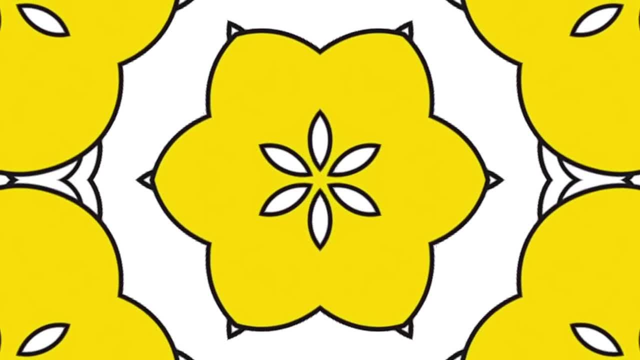 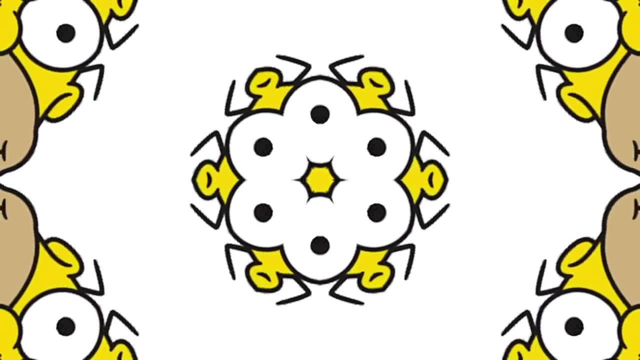 oh, I'd be good at TV, but not many people get to do it. And you sound like you just said: hmm, think I'll try TV now. What did you have that they saw, or how did you get in? So I remember applying for a job in radio, for a start. 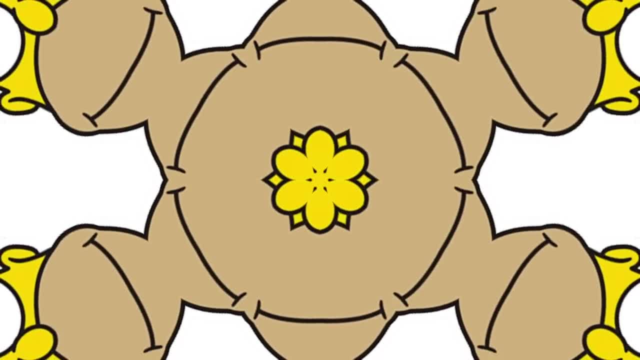 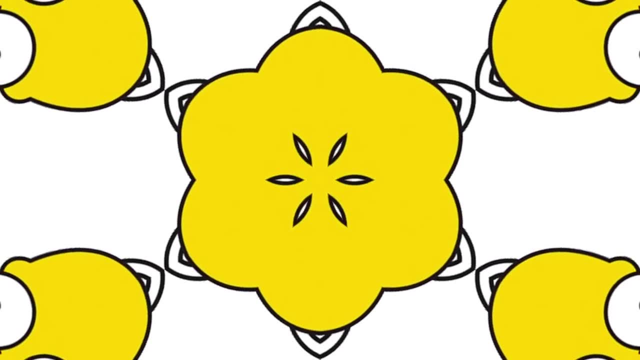 And I turned up for the interview. I was like, oh, I'm going to do this. And they said: so tell us about what radio you've listened to this morning. And I hadn't listened to much radio because I didn't really love radio with the same passion. 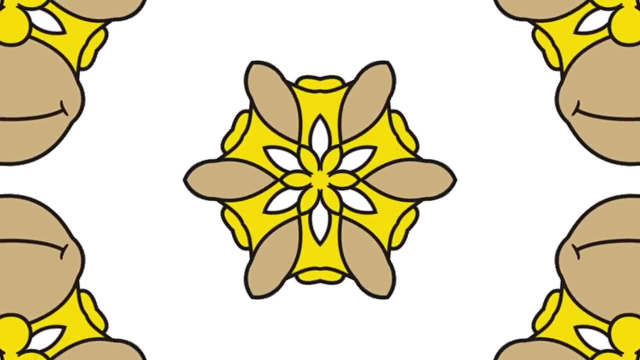 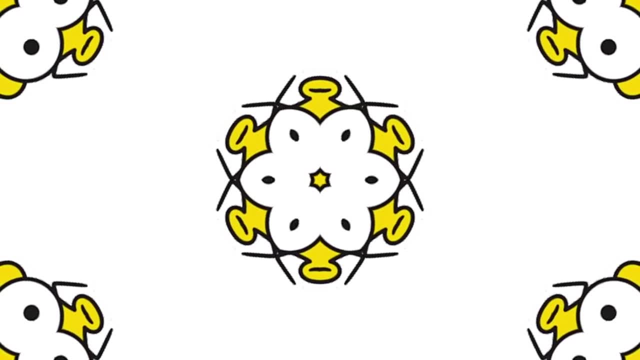 that I love television And so that was the end of that interview. But when it came to the TV interview- and it was with the science department- I knew TV inside out, I knew the history of science, television broadcasting. I could critique programs. 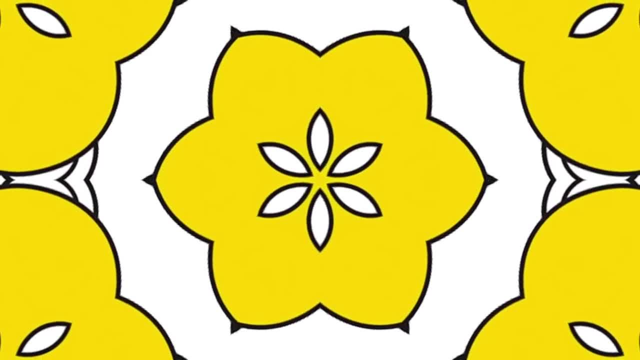 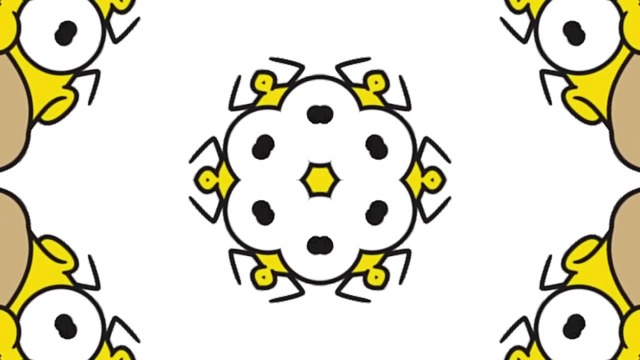 I had a PhD in physics which made me. I think that meant they said we've got to interview him at least because this is interesting and a bit different. You see, the difference now is that if somebody applies for a job in television, they better. 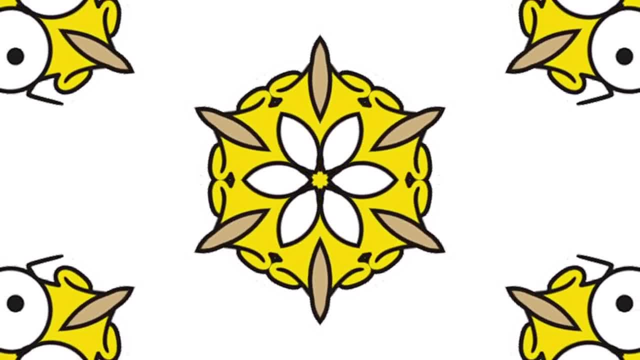 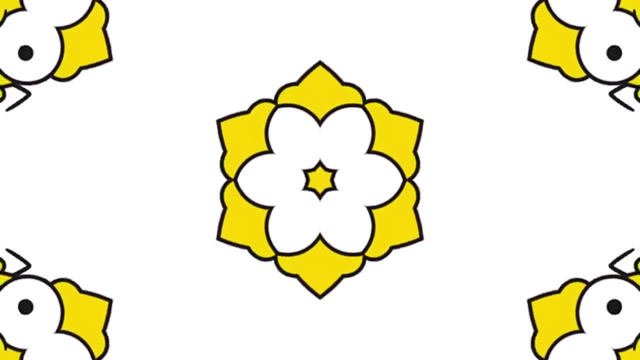 have a portfolio. They better have edited stuff at home on their PC. They better have their own podcast. There is no reason today for anybody not to have done the groundwork themselves before they start going to their interviews and so on. Back then you couldn't really do that. 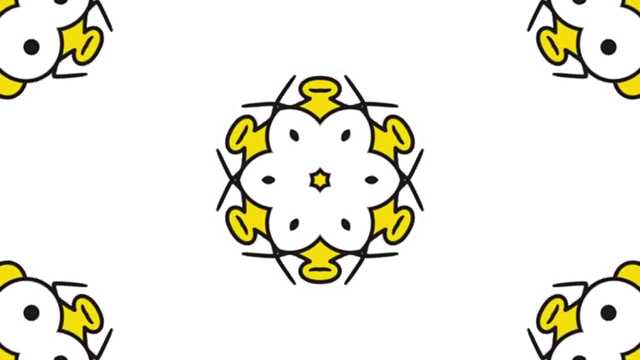 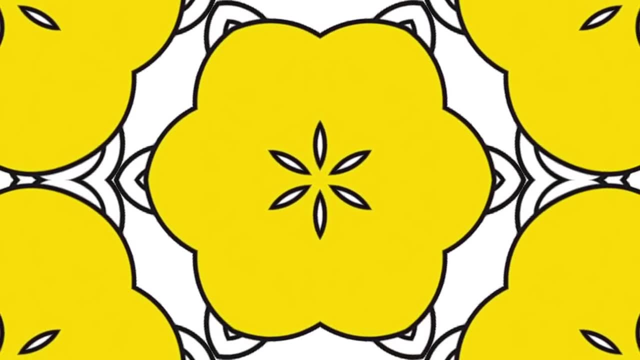 So I had to kind of cook up as much as I possibly could in terms of anything media related I'd ever done at university. I'd edited, I started a physical, I did a physics newsletter, I contributed to university magazines, I'd made a couple of videos for the student union. 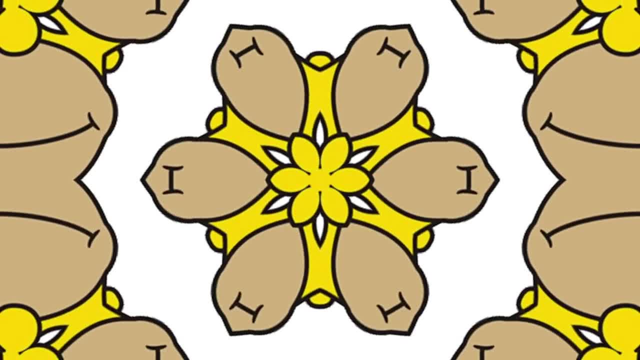 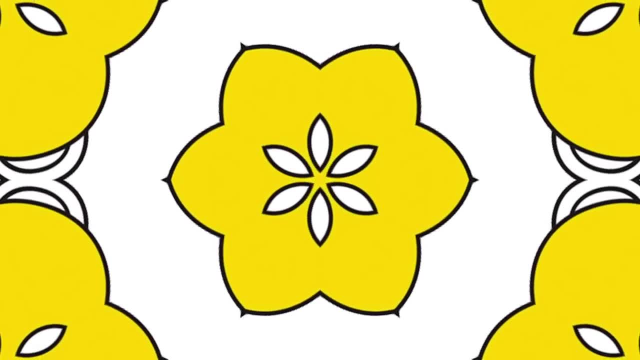 I'd done a bit of student radio at Cambridge, but in a way that was only done because I knew I wanted to apply to the BBC. Try to make my CV look as good as possible. Had this PhD in my back pocket to say, look, you've at least got to interview me. 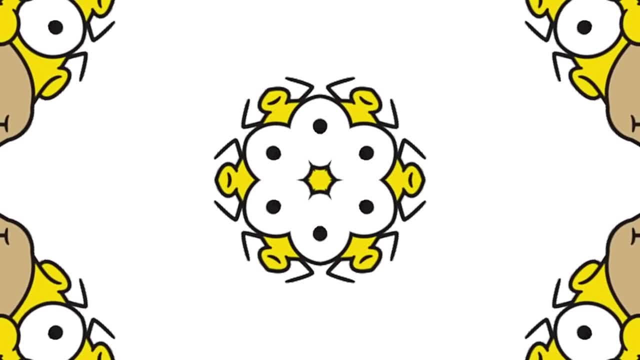 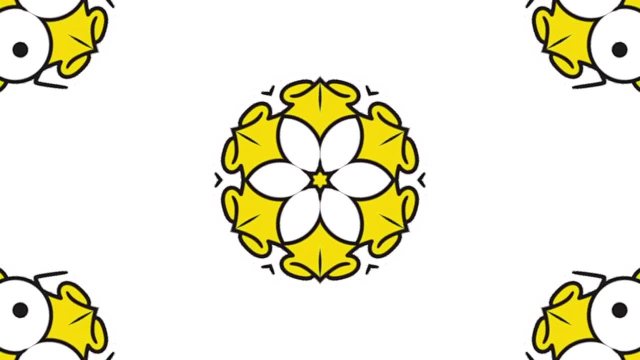 Got on well with the people who were there at Tomorrow's World who interviewed me, And then it's a case of you've got six months to prove yourself and if you can do it, great, If not, goodbye. And the turnover is huge. 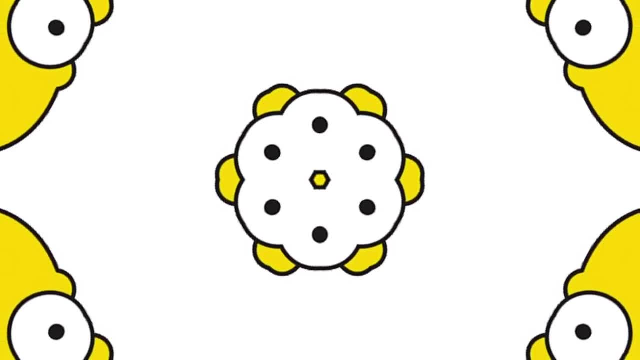 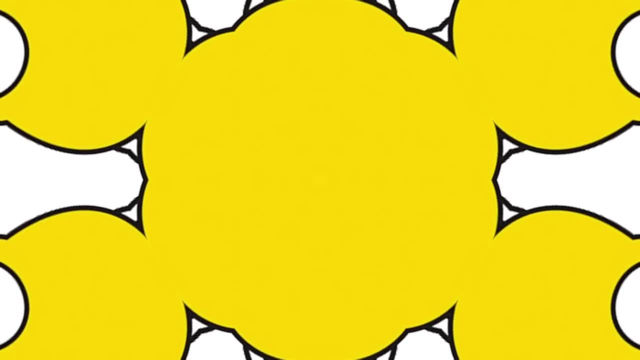 Even when you get a job, it used to be only a one-year contract and if you didn't deliver then you were out. So it was a pretty tough environment, but I could do it, I could make films, I could find. 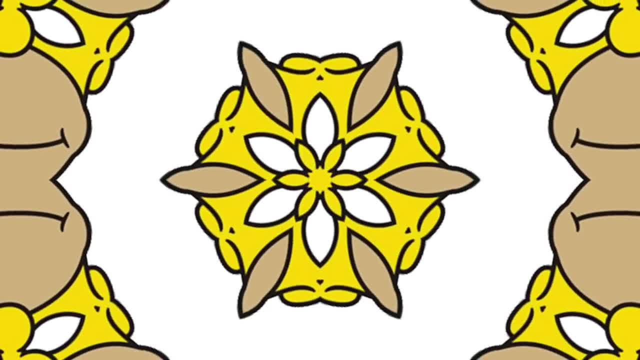 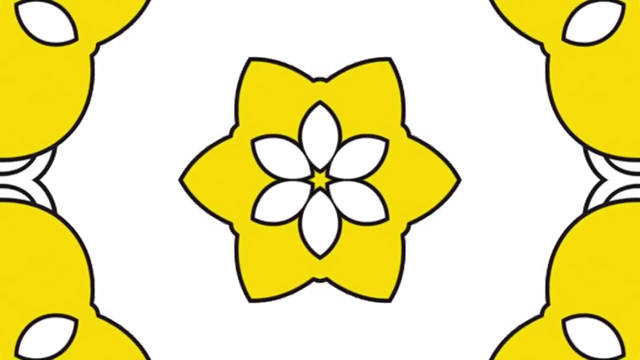 Again, people say: how do I become a good filmmaker? But first you've got to find the stories, and that's really tough. It's the same with writing a book: First you've got to find what you're going to write about. 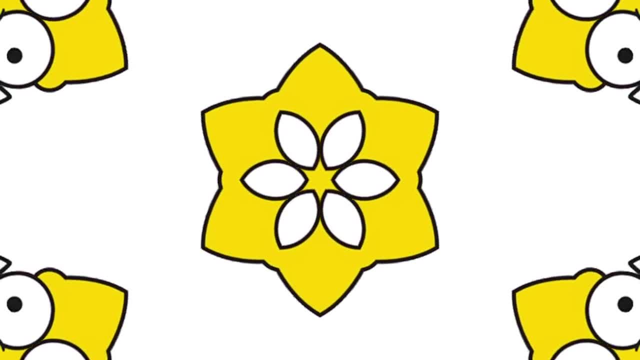 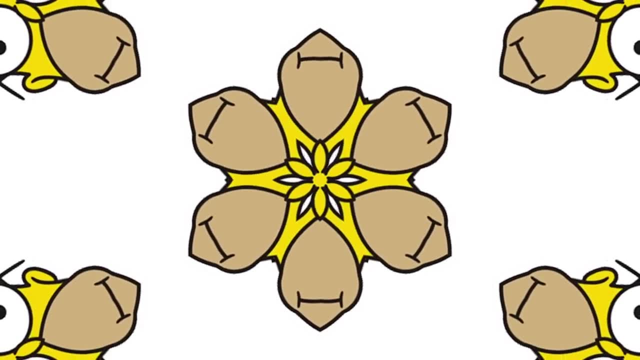 Then you've got to convince somebody else that this is worth writing about or making a film about. Then you've actually got to go away and make it. And that's only the final stage. And if you can find great things, If you can find great stories, turning them into great films is pretty easy, especially. 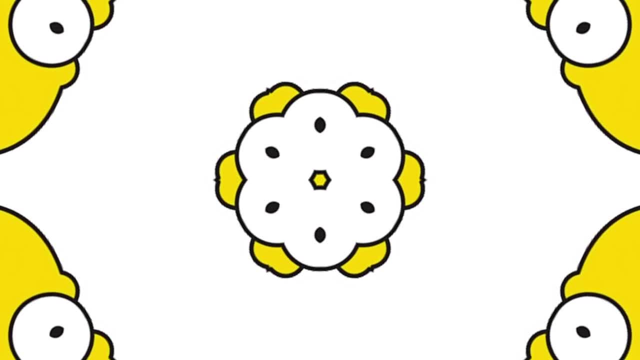 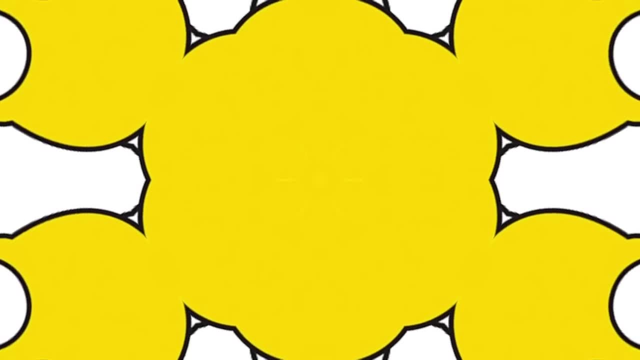 if you just let people do their jobs. So I would just say to the cameraman: make this look good. And say to the sound person: look, just make sure I'm not doing anything stupid here. And if you work with good people and give them the opportunity to make you look good. 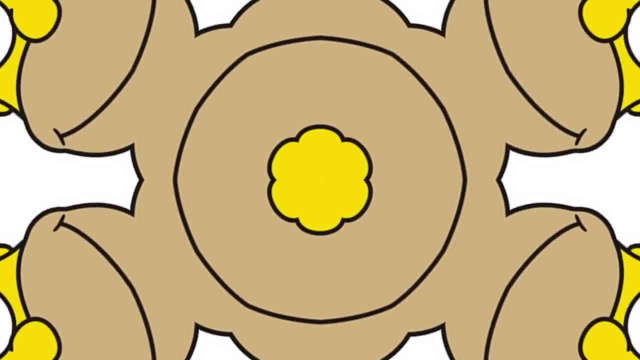 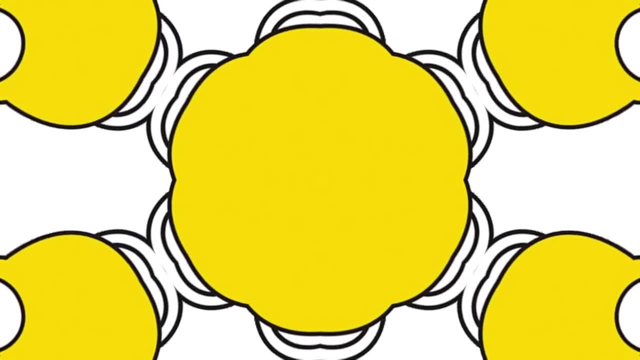 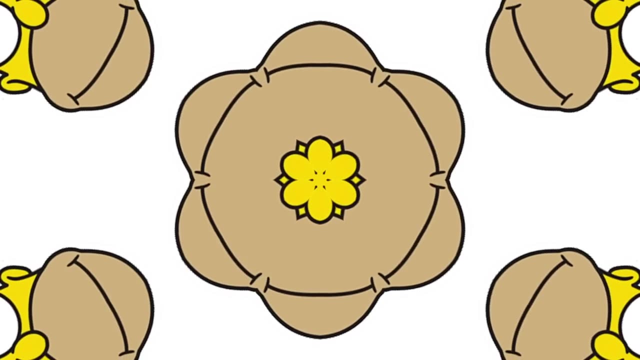 as a director, then you end up making interesting films, And I loved my time at Tomorrow's World. I made dozens and dozens of films about all sorts of subjects, from debunking miracles, government to anti-snoring surgery, to going back to CERN and making films, making films. 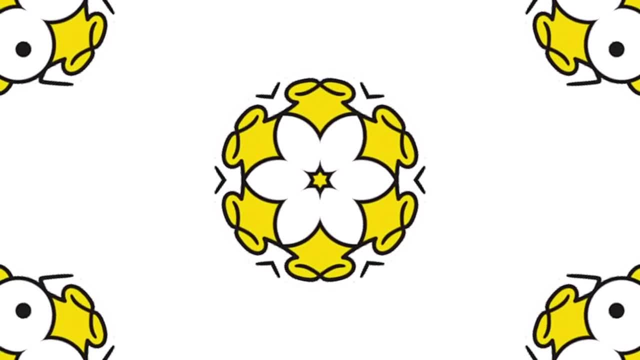 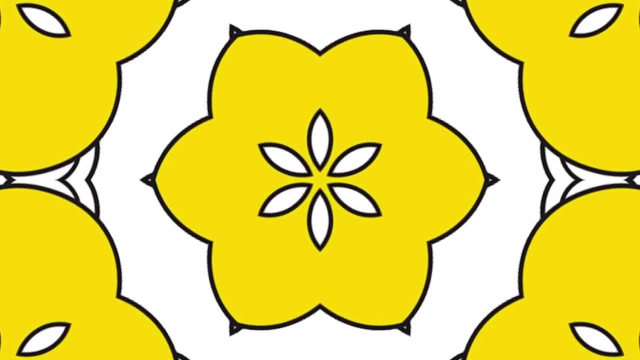 about artificial intelligence. I got to interview Garry Kasparov. time travel got to interview Stephen Hawking- Just extraordinary opportunity to go out there and play. And I did find what I'm supposed to do. You know, I loved physics and I couldn't have gone through my life without doing my PhD. 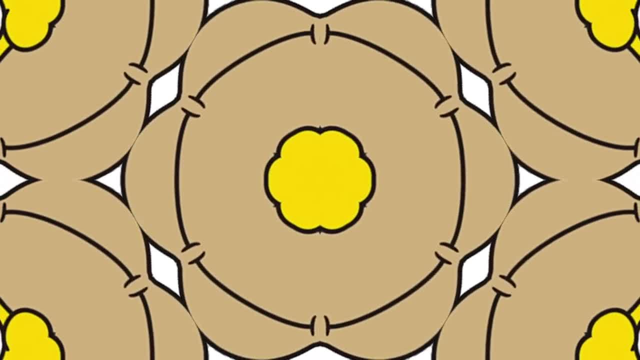 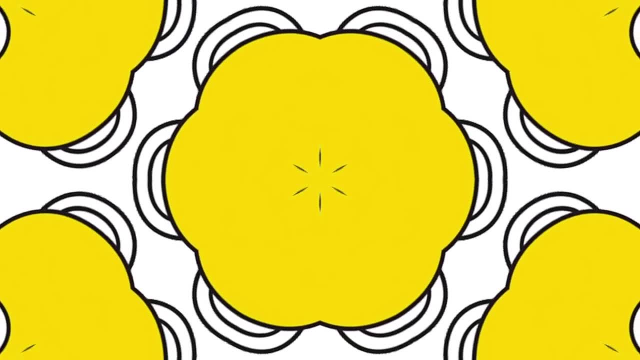 But ultimately that sort of media side of science is where I've thrived, I think Do you, I imagine also having the PhD and the- Yeah, The degree of strict credibility in science helps when you're approaching those scientists and saying I wanna make a book or I wanna make a film. 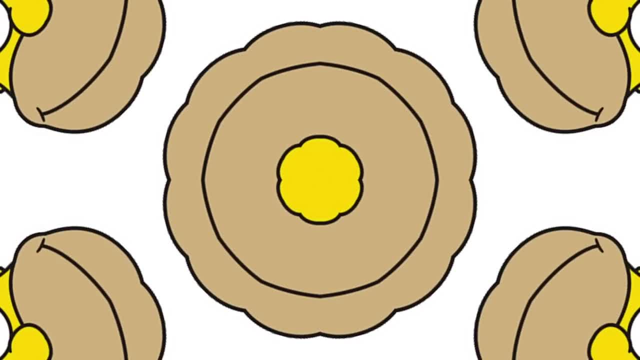 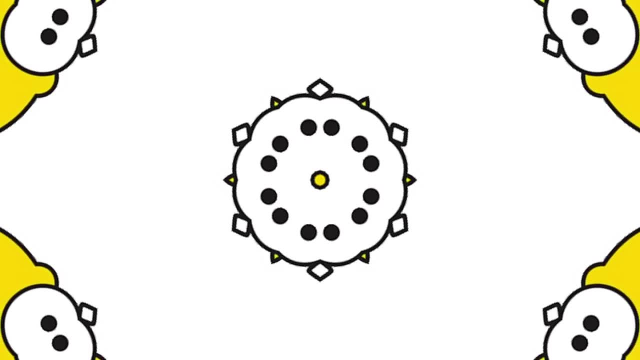 You know you're like, I'm one of you. That must help, at least at the start. It works two ways. So there were some people in the BBC science department who have virtually no scientific background. They can quite rightly argue that when they go in to see a story they're seeing it from. 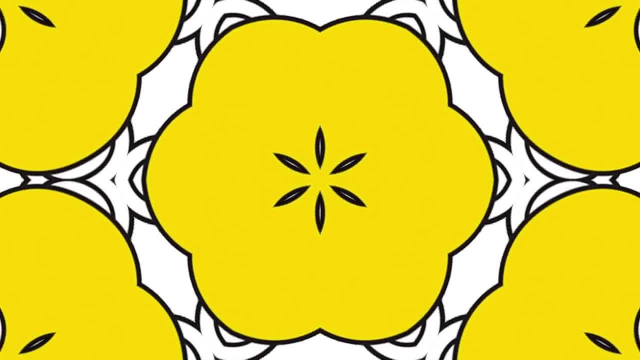 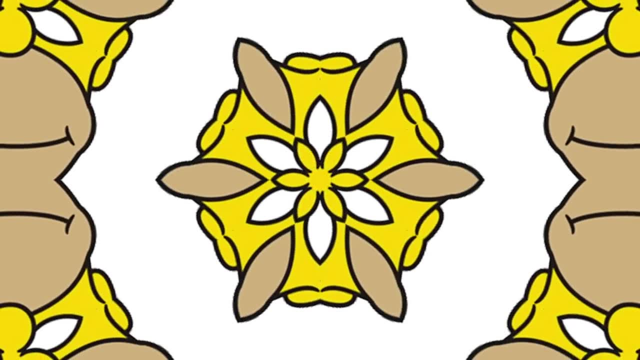 the perspective of the non-scientist, and that's fine. When I go into a story, I can build those relationships. I know about peer review. I know how research works. I know about the frustrations of research. I can perhaps win people over. 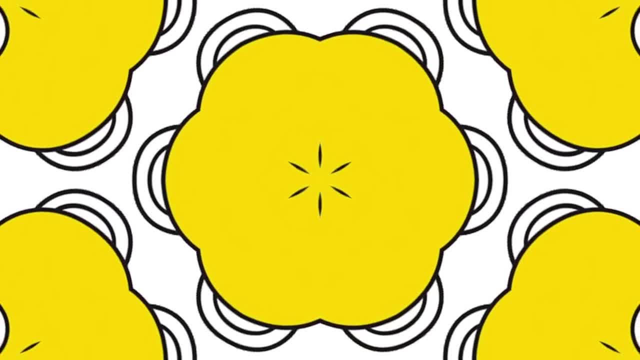 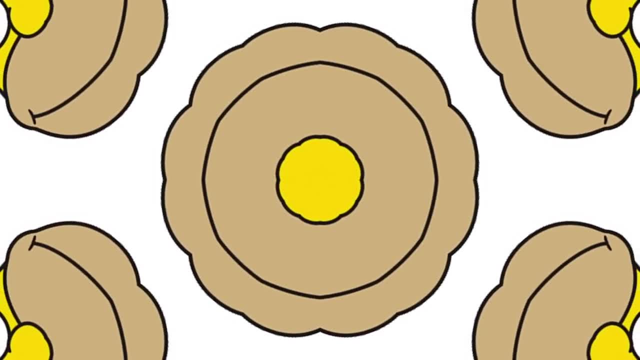 And I would say that's all the advantages of when I tell a story. But I think ultimately you just have to be a good storyteller. That's the main thing. Whether you're a non-scientist or a scientist, you go into it and you just find those stories. 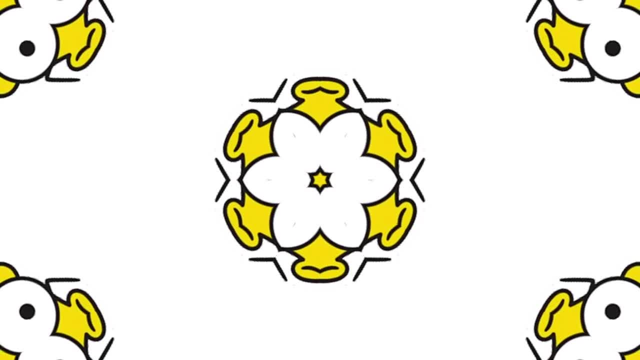 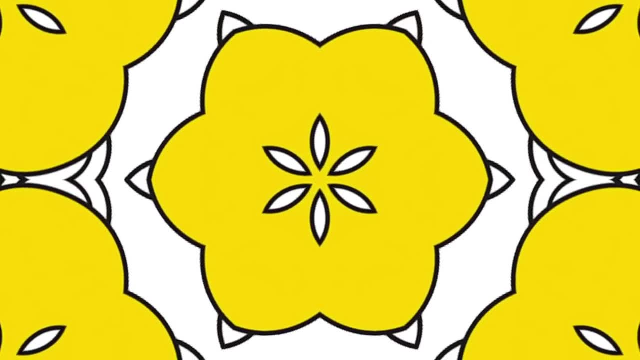 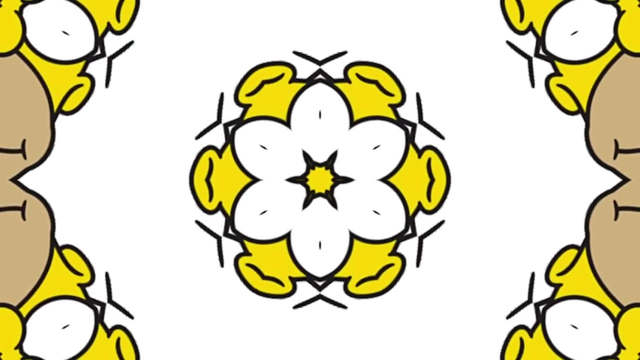 get on with people well and then tell those stories. When you finally became an actual practicing physicist, you know working at an amazing place like CERN- how did that compare to what you imagined being a physicist would be like when you were like a schoolboy who said: this is what I want to do. I want to be a physicist. When you actually did the real thing and met the reality of funding and the grind and the ups and the downs of it, was it very different to what you had dreamt Or was it exactly what you dreamt? 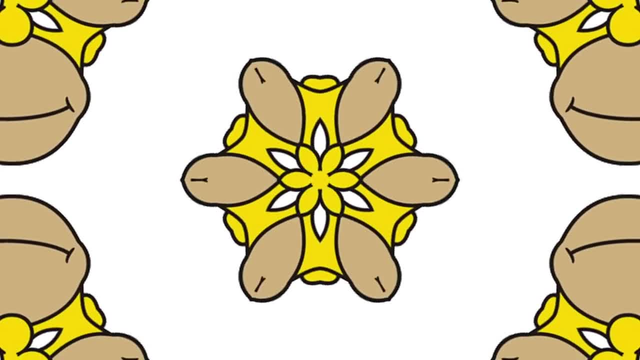 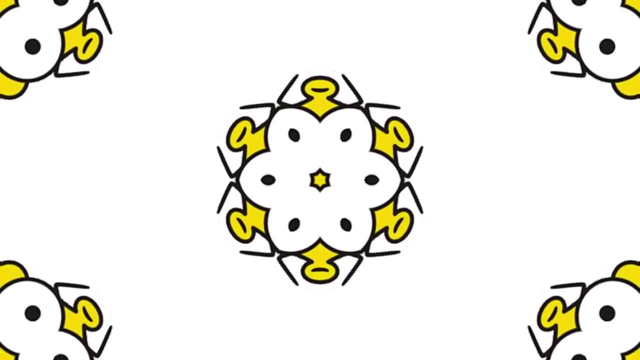 It was pretty much how I'd expected. You know, CERN's a pretty glamorous place. I was living in France, I was crossing the border. Lake Geneva was just down the road. It's this huge facility. You know shiny metal stuff everywhere, famous physicists wandering around. 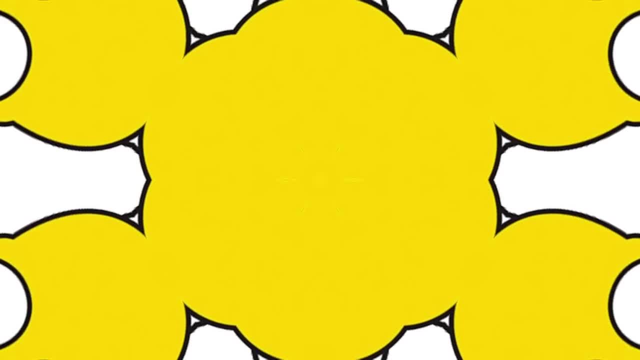 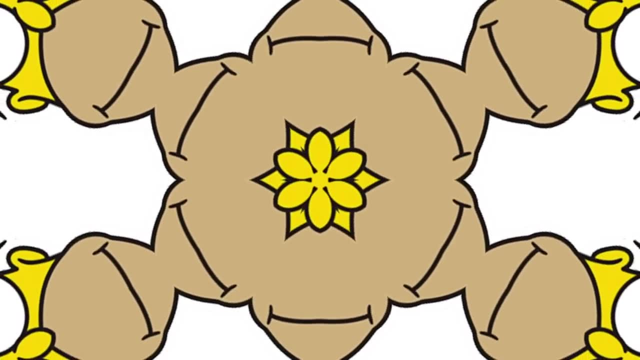 It was brilliant, You know. incredible seminars by people visiting from all over the world, Nobel laureates speaking. You know, maybe I'm looking back at it and roasting two glasses, But I do remember the first three months being terrifying because it depends when you join. 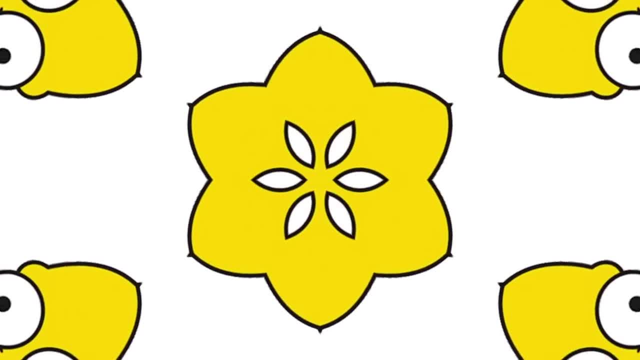 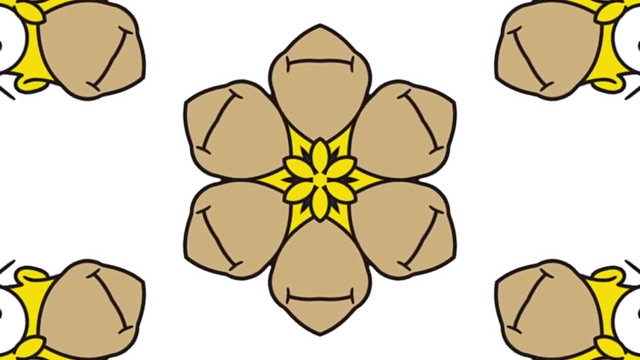 the experiment. But I joined the experiment at a sort of critical phase where we needed to start building this detector and get on with it quickly. So I just got sent straight out to CERN. I didn't know what to do. I didn't know much particle physics that was going to be relevant. 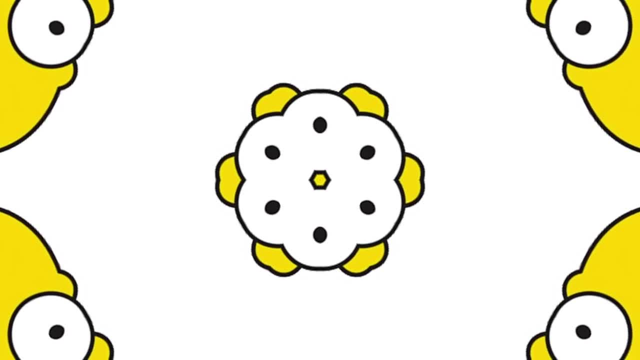 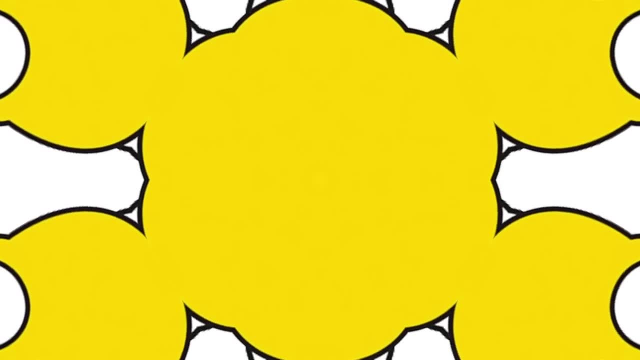 I didn't know much about the technology that I was going to be using to build this bit of the detector And I felt really lonely, So those first three months were super, super tough. Getting through that was hard, but I survived it. 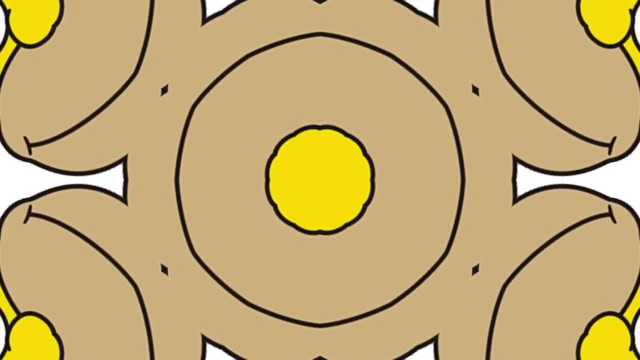 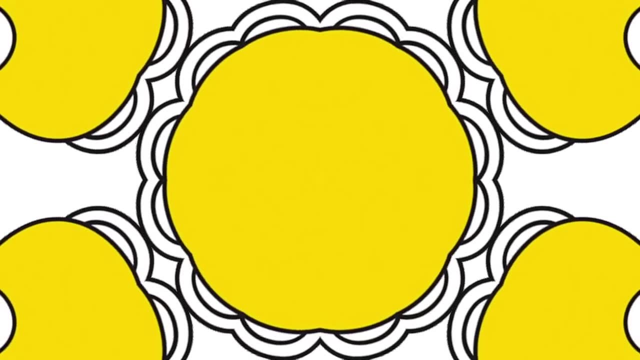 And I think literally I just about survived it. You know, it was probably one of those phases where you probably throw the towel in, or what doesn't kill you makes you stronger. And then I got back to Cambridge after Christmas, managed to kind of take a bit of a breather. 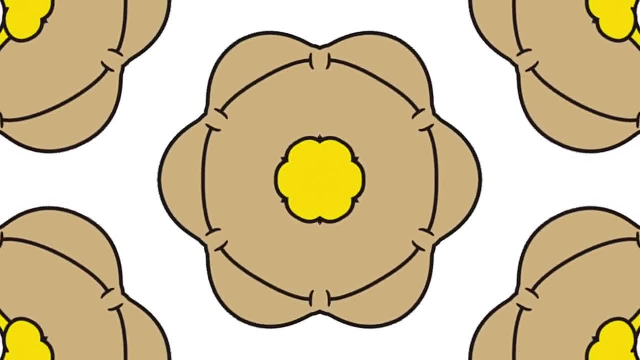 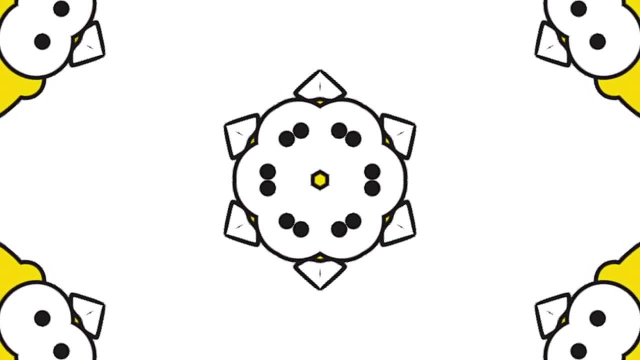 consolidate some of my understanding of particle physics, build on my knowledge of the technology we were trying to build, take a deep breath and begin to really enjoy my PhD, which is what I did for the rest of the two and a half years. You talk about this realisation that you weren't as good as some of the others. 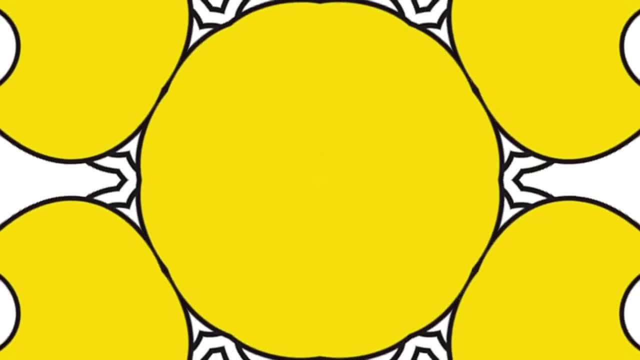 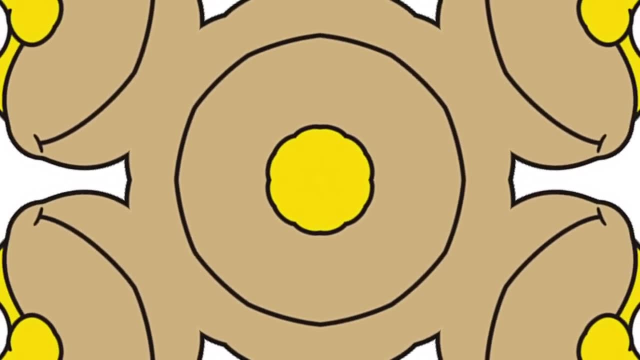 You weren't going to be the superstar and thinking: maybe I need to be doing something else. I don't often hear people say that It sounds like it was a difficult decision. Was it forced upon you? Was it easy? Was it courageous? 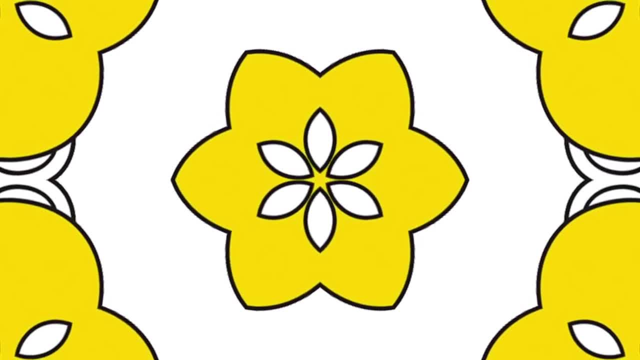 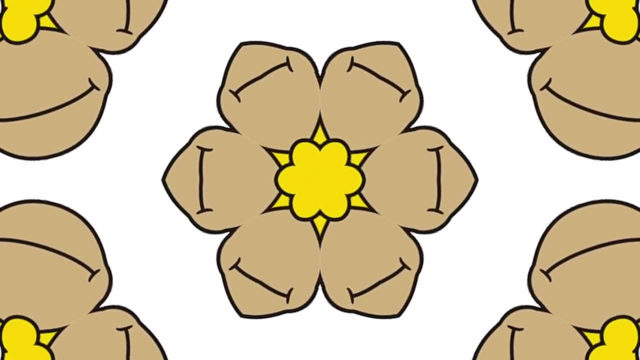 I think the people you talk to In general are successful mathematicians, And so they've got to be professor of what's at University of Doudar And to get from age 10 to professor at wherever you've pretty flawlessly got to leap every. 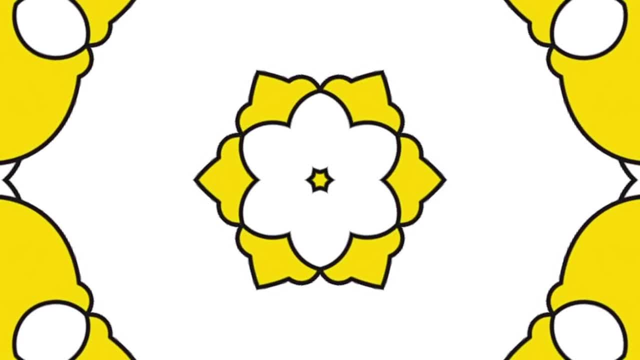 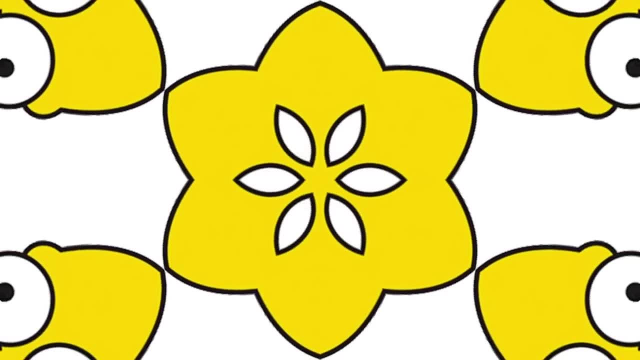 hurdle. I would imagine I'm trivialising here, because it's clearly a struggle all the way through And unless you really strive and work hard, you don't get to those places. And there will have been moments of self-doubt for all of those people. 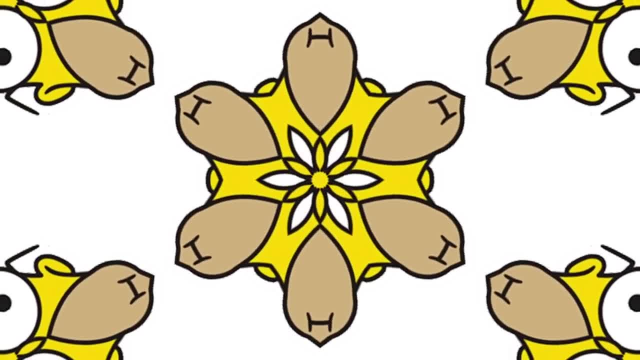 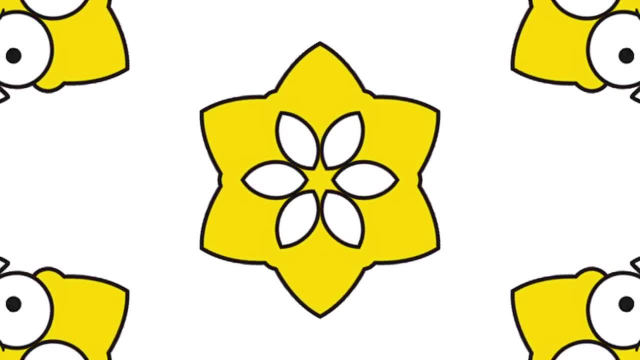 But clearly they They've got to where they needed to be and where they deserve to be. So for me, it was just a case of thinking: you know, what else can I do, What else should I do, What else would make me happy? 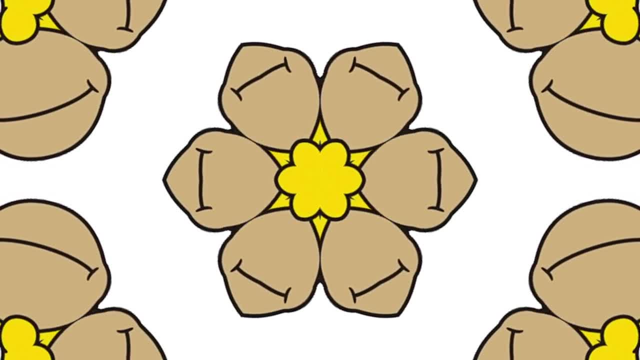 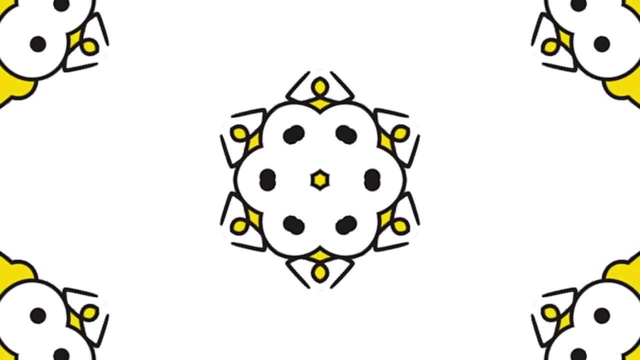 What else? When I talk to sixth formers, I also say what makes you different and special. What can you do that other people can't do? I remember somebody once said: you know, when you're looking for a good job for the rest of your life, what can you do? 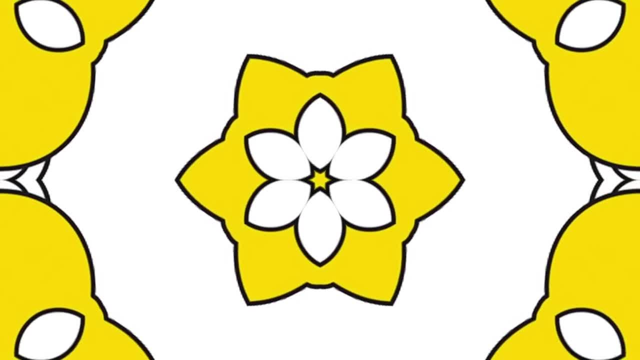 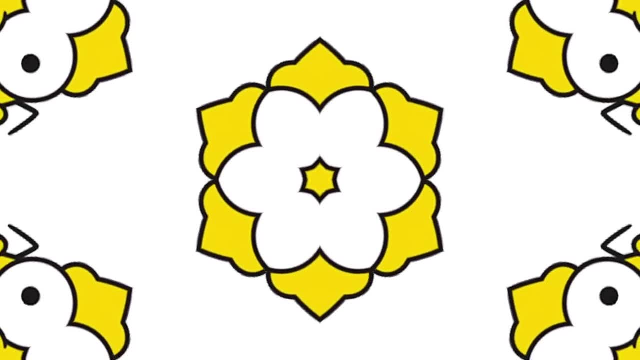 What do you enjoy doing And what will somebody pay you to do? So you might be good at lying on the beach. You might like lying on the beach, but you might not get paid for it, And there are various other combinations, So I just had to find something that I really would be good at. And which you know some. If I could have taken a postdoc position at the University of Toronto- I think that's one of the places I was applying to And that would have been fine, I think I would have got the position, maybe, and carried on quite happily. 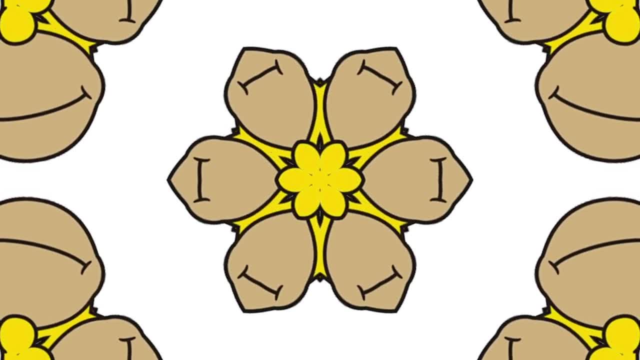 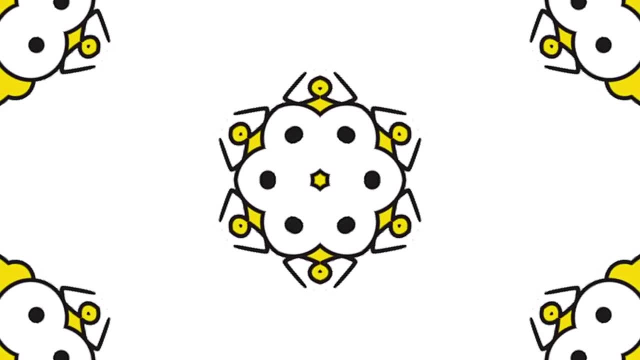 But so could 10 other people have done that job. So also, what makes you different? What would you do that nobody else would do And find that maybe odd combination of skills that you have. So there were lots of other people who were good at physics. 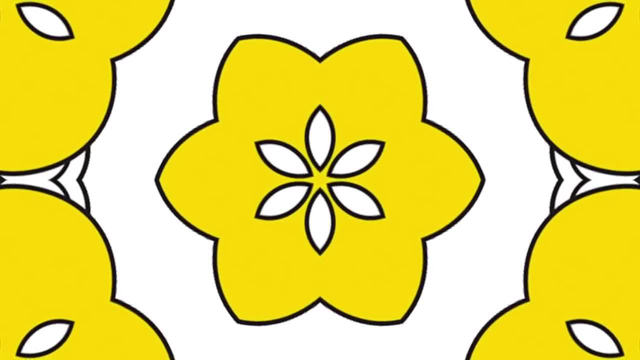 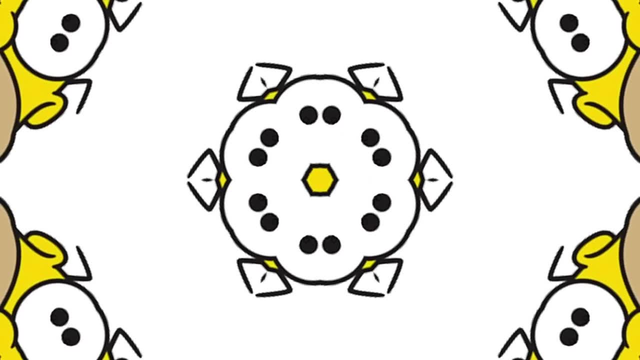 And there were lots of people who were better at physics than me, But they didn't. They didn't love junk TV And they didn't necessarily enjoy teaching And they didn't necessarily enjoy talking about their work as much as I do. So all of those skills are what makes me a bit different from those people. 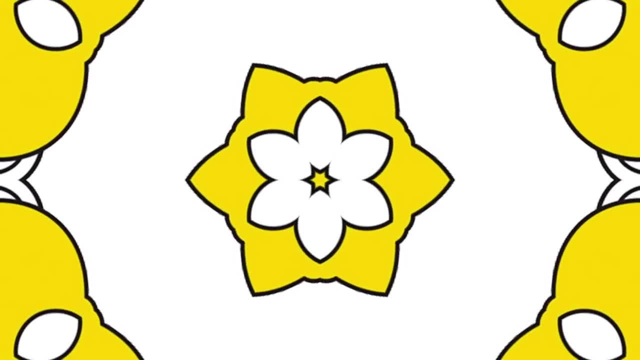 And then I think there's maybe a pattern here that when I was at the BBC and I was there for sort of six or seven years and I think I did really well, I think I made some great films, And then I just left. 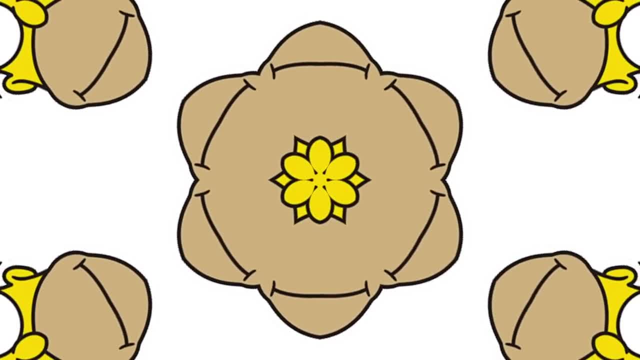 I just said: right, that's it. I've kind of made enough films. I could make more films, but I'm not sure how life would be different. So I'm going to go off and write a book. In fact, I actually said I'm going to leave. 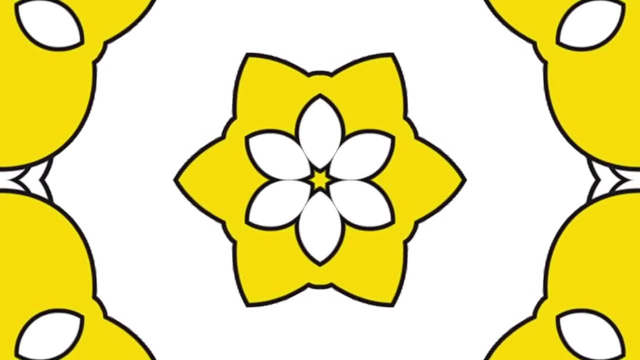 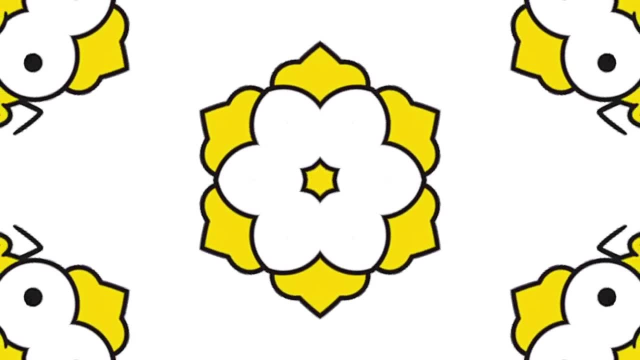 And then a few months later I thought: oh, hang on, I should write a book. I haven't written a book now since 2013.. So it's been five years And that's it. I can't imagine writing another book because I want to do something different. 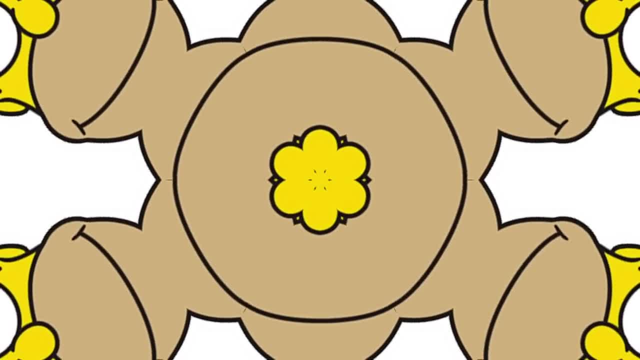 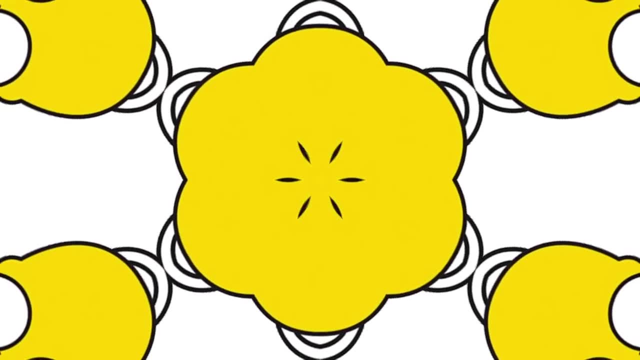 So there's a kind of a pattern there of leaving something behind and moving on, but then using all those skills that you've picked up from a previous. So the reason I write books in a certain way is because of the way I used to make television. 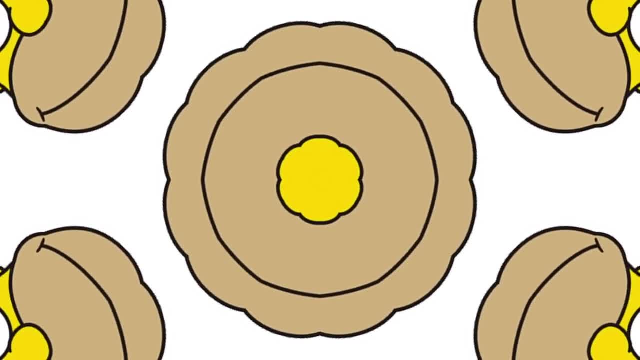 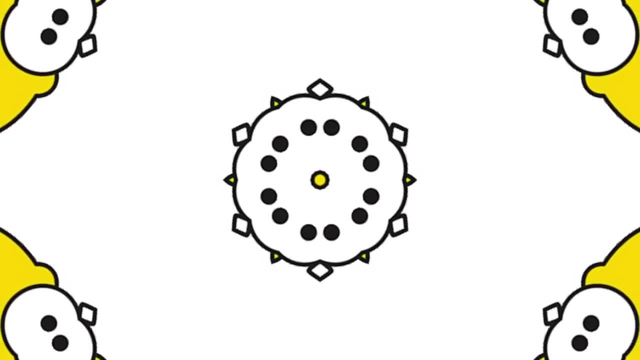 The way I make television has been hugely informed by the fact I've done a PhD in particle physics. So even Even though you abandon things and move on, they're all science related and all those experiences and skills feed into whatever you do next. 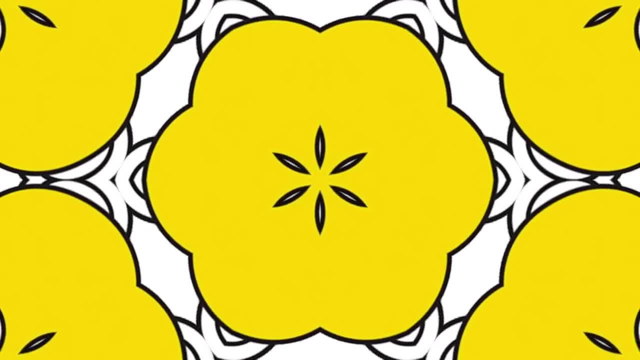 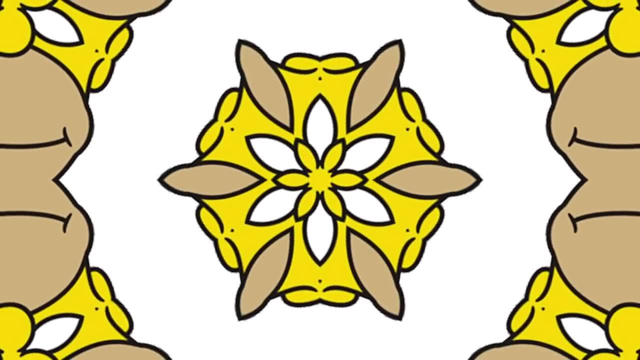 Are you someone who has always had the next step, secure and safe, before you let go of the branch? It sounds like a couple of these times you take the plunge, you just let go. Yeah, you know, I suppose I still have my postdoc application in the pipeline. 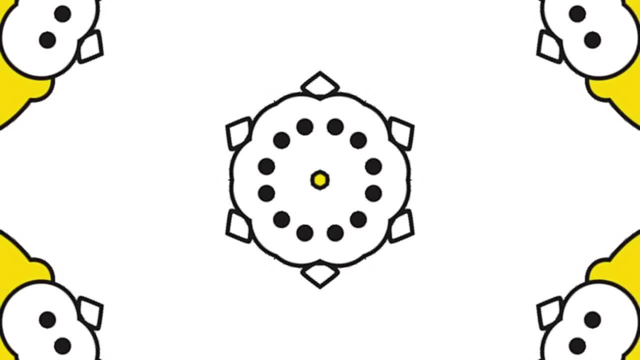 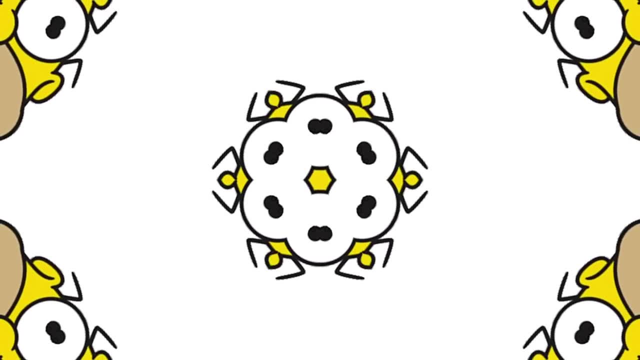 while I was applying to the BBC, but I definitely left the BBC before I knew what I was going to do next. I just said, right when this project's over, I'm off, And I had no idea really where I was going to go. Something we'll come to shortly, that we're going to talk about, like some of the things you're working on now, but now I very much think of you as someone who is like a bit of like a campaigner and someone who wants to make a difference and change the world for the better. 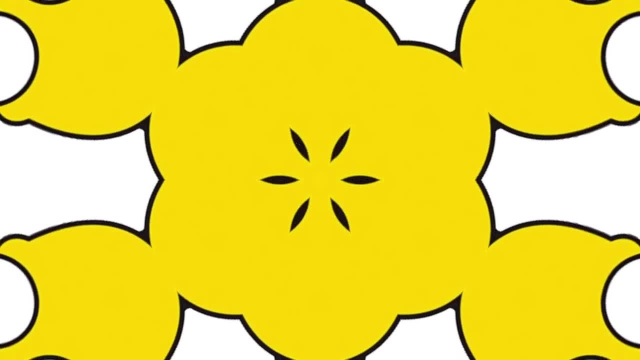 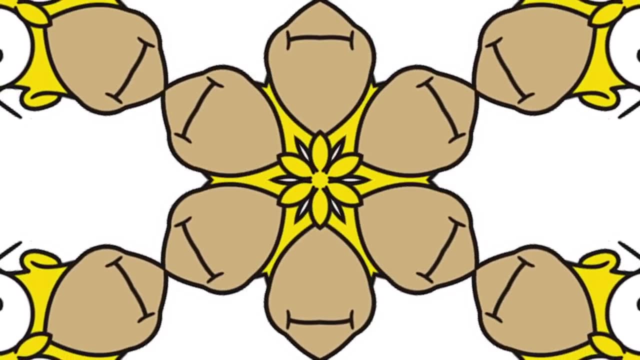 like you know, in a kind of crusade-y type way. But were you like that when you were at the BBC? Were you thinking these films are going to make the difference and make the world a better place? Or were you just like you know, this is my job and I'm a storyteller and I like TV? 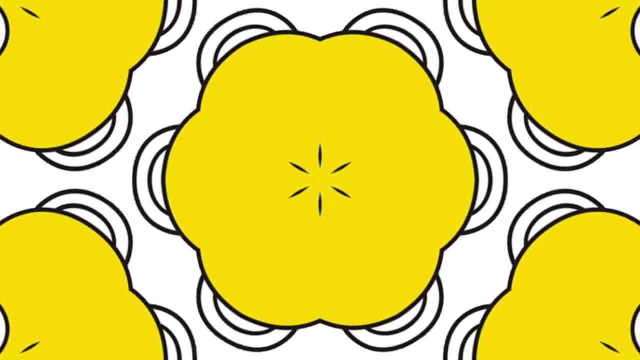 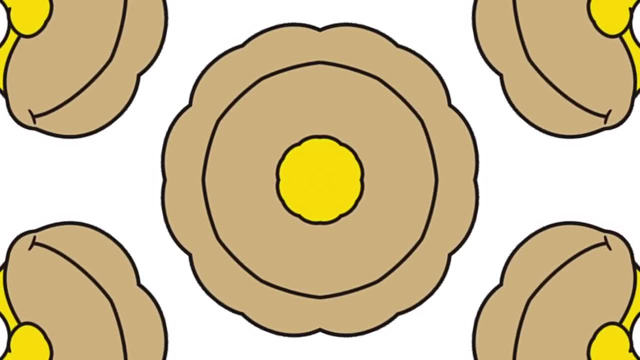 Or was that sort of streak already Running through you, that I must make this film because the people must know and the world must be made a better place? I think there are a lot of people who joined the BBC Science Department with that mentality, And I was one of them as well. 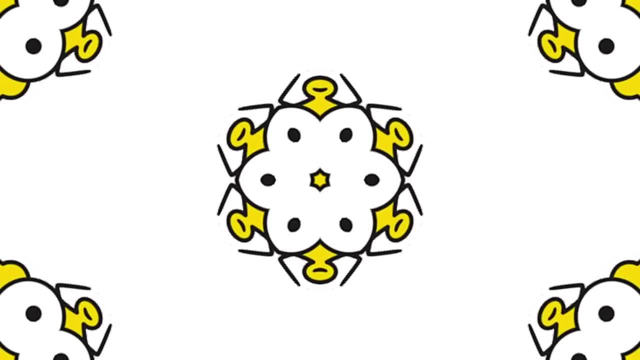 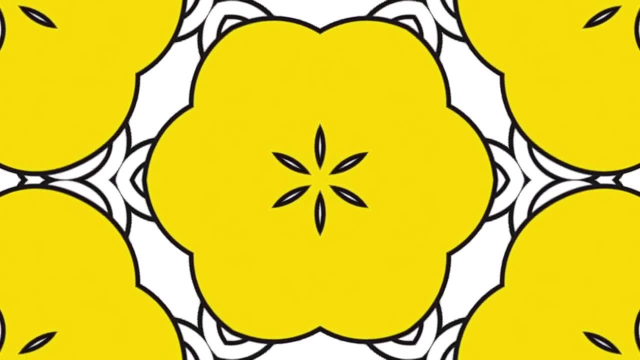 And I think it's a great thing that you are passionate about science and you want other people to see that passion, that passionate side of science. You want to inspire that next generation, And I think that's true, for whether you make political films or films about history, you want to bring on that next generation. 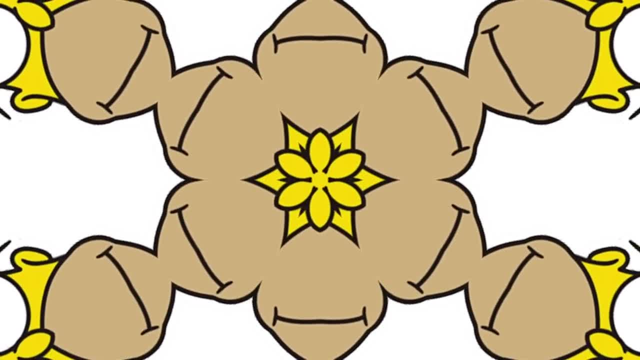 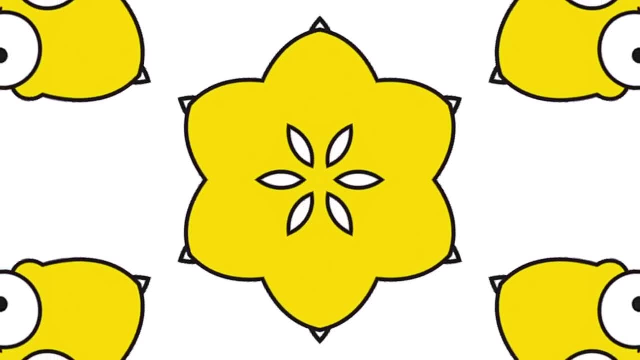 You want to excite them, You want to tell those great stories. So I wouldn't say it's campaigning, I would say it's just trying to share the joy of science. Yeah, in a very kind of obvious way that I think many people 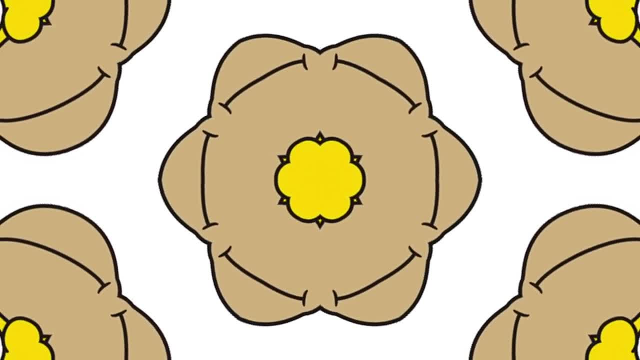 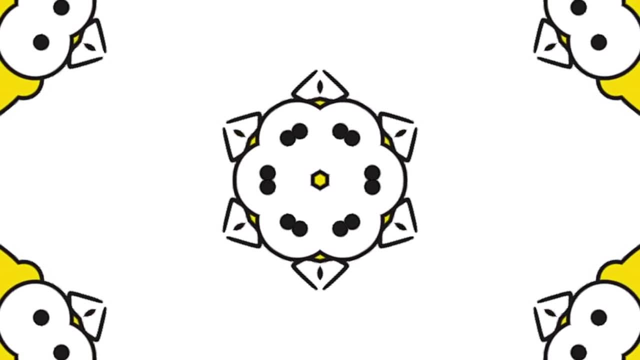 are going to television want to do So. when you left the BBC, you went through the book phase then, of writing a series of very successful books. How does one decide? okay, this is a good idea and this is a good newspaper article. 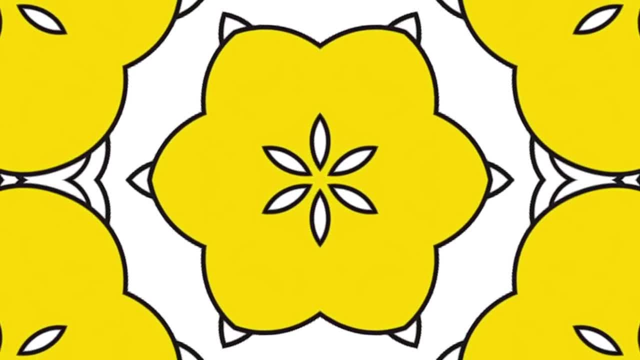 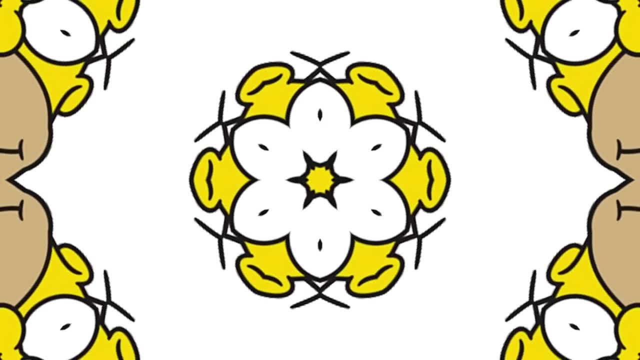 This one, this is book worthy. This one, this one's a book. So Fermat's Last Theory. I'd made a film about it for the BBC and the idea there was that the film had been hugely successful. And it's just as soon as you hear the story. 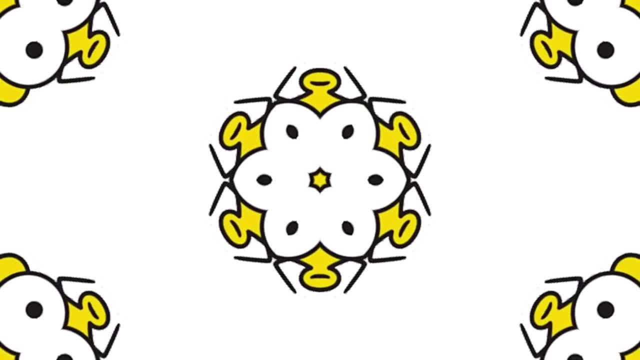 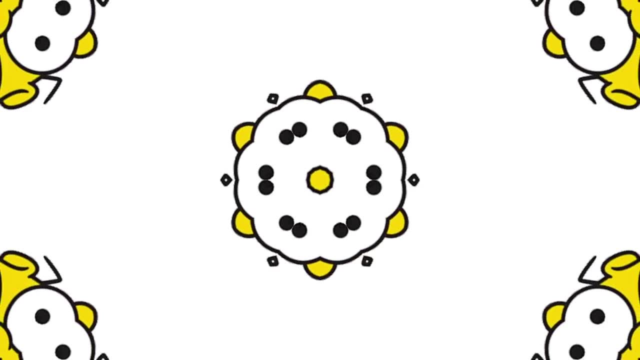 you realise it's a terrific story. This is the story, of course, of Andrew Wiles. Yeah, Professor, Andrew Wiles and Pierre de Fermat and this 350-year-old problem. It's just full of wonderful little stories along the way. 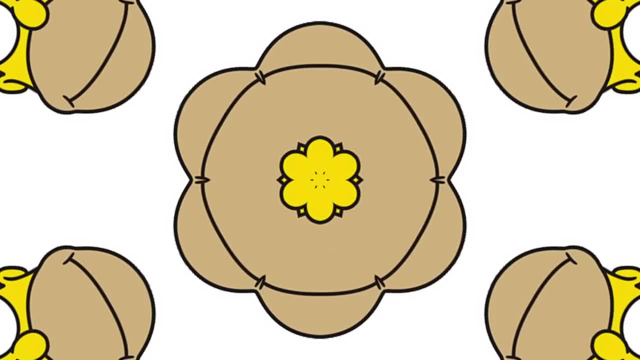 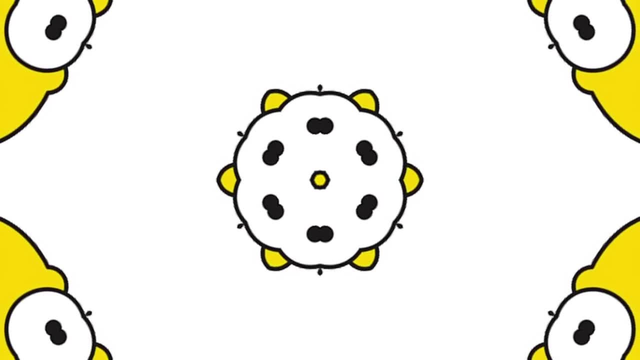 and sort of terrific beginning and an even better end. So you made this film, which is still a great film that people love watching, but then a book. Is it because you felt like the film hadn't told the story? Yeah, so I'd left the BBC and 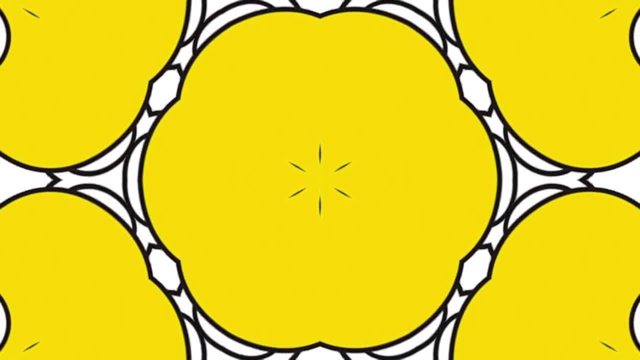 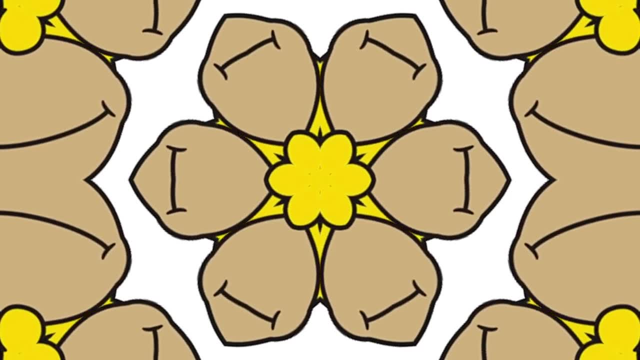 or was in the process of leaving the BBC, And then you realise that a 50-minute documentary- which is what that Horizon documentary was- is about 6,000 words. Okay, now a pitch is worth 1,000 words and all of those things. 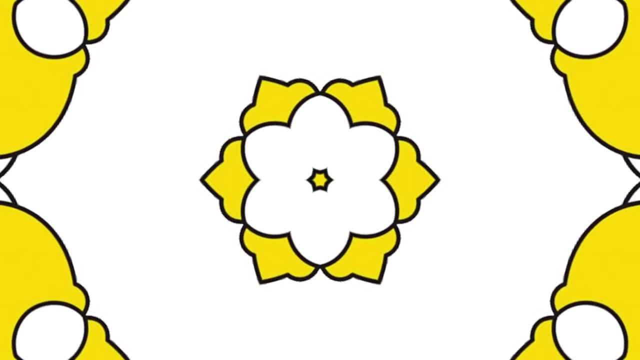 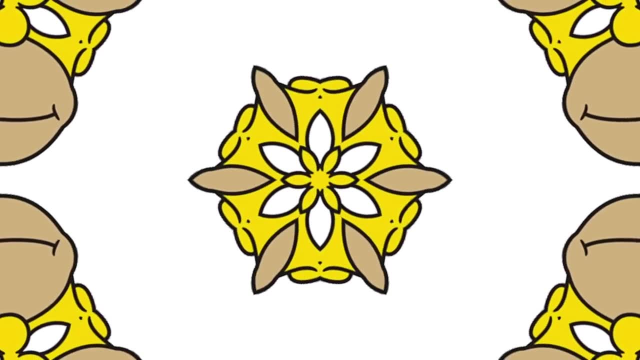 and I wouldn't change anything about that film. I'm hugely proud of it, But in 6,000 words you cannot go through all of the history of Fermat's Last Theorem. The mathematicians in that film were so eloquent. 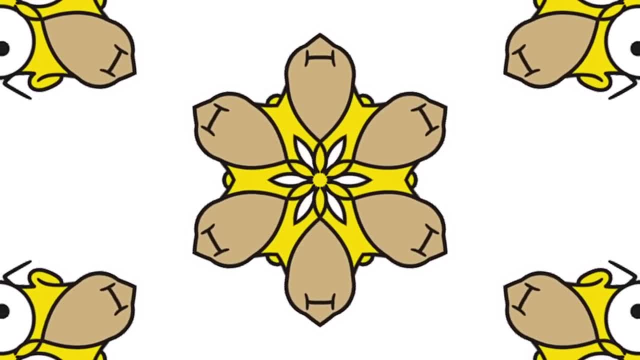 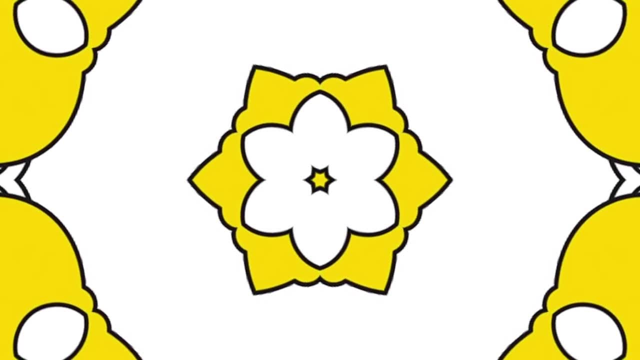 that all the history really went out the window, because we wanted to hear about the mathematicians alive today. So why not write a book that's got all that history in it? Television is not a great medium for explaining maths, So we got some of the core concepts in. 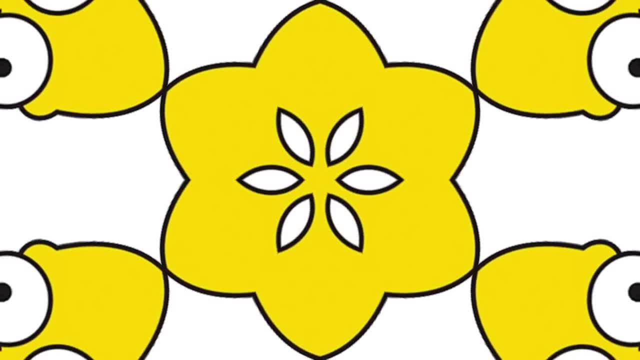 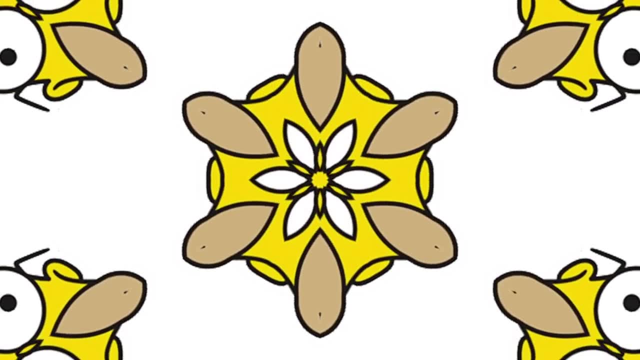 but not much beyond that. So let's explain more of the maths in the book as well. So that's where the book came from. Let's tell the full story of Fermat's Last Theorem, And then in that book there was a little bit about Alan Turing. 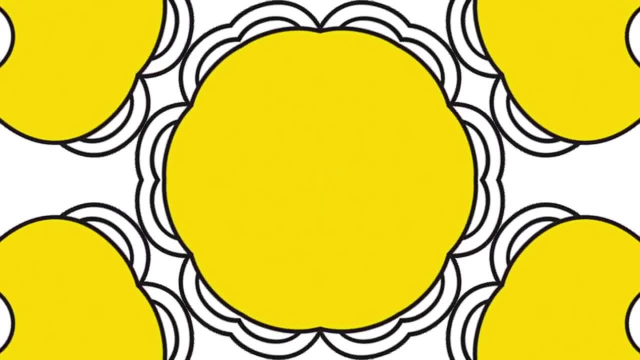 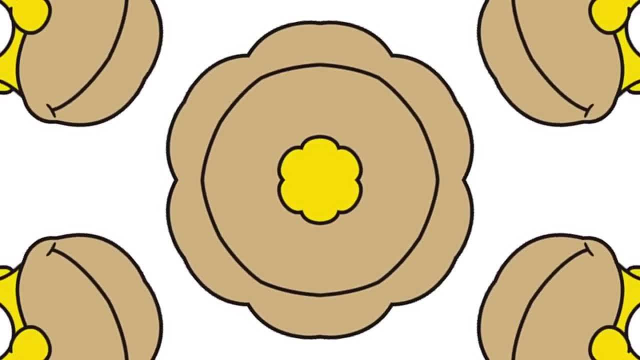 and a little bit about Bletchley Park and Colossus and computing. That's sort of where the code book came from. I probably had a much bigger section about Alan Turing and Enigma, Which inevitably got squeezed right down, So it then got blown up again into a huge book called The Code Book. 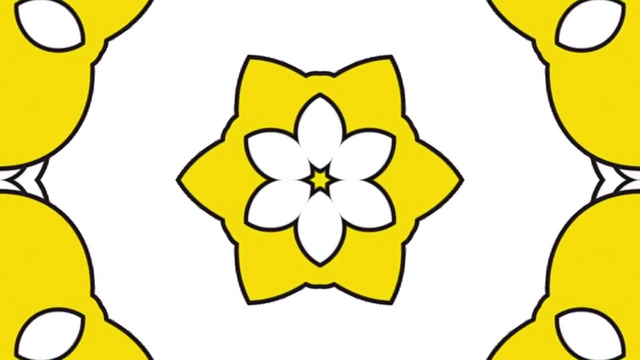 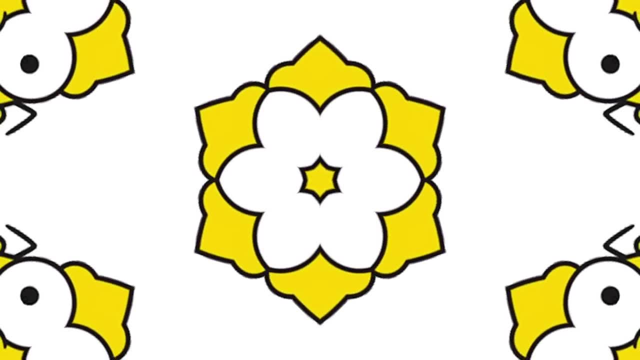 And when I was at Tomorrow's World, I had a whole file of stories about cryptography, because it was a really fascinating area of technology but not very televisual, So I never ever made a film about it with the BBC, but I had all these stories. 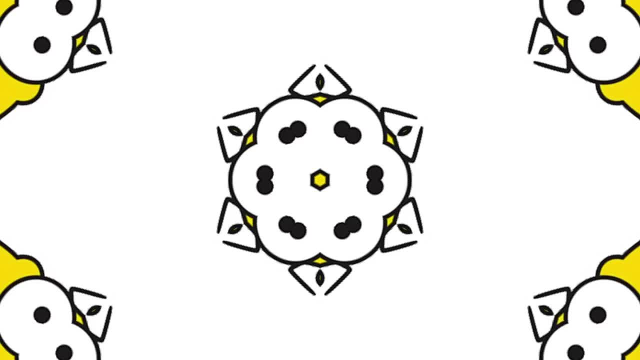 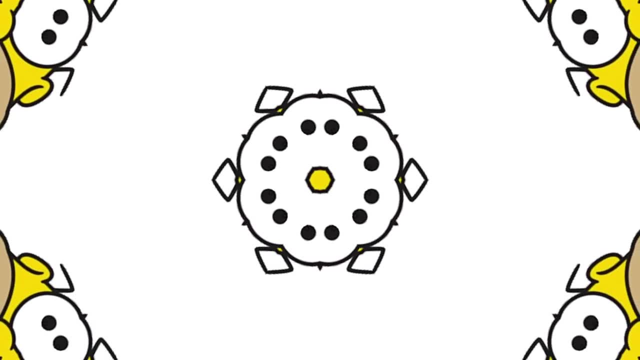 And I knew it was very relevant today. I knew there was a great history And I knew there was the story of Alan Turing and Enigma, So that's where the code book came from. Nobody had really written about cryptography. Cryptography since the late 1960s is a great book by David Kahn. 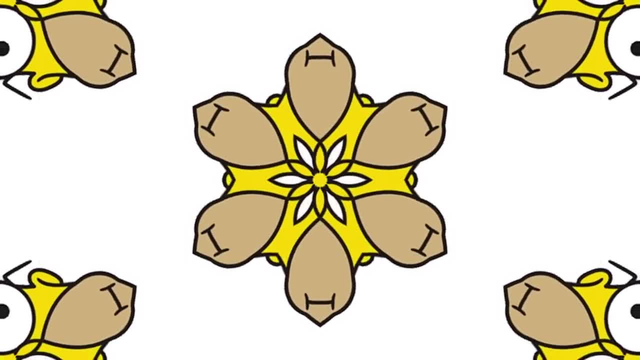 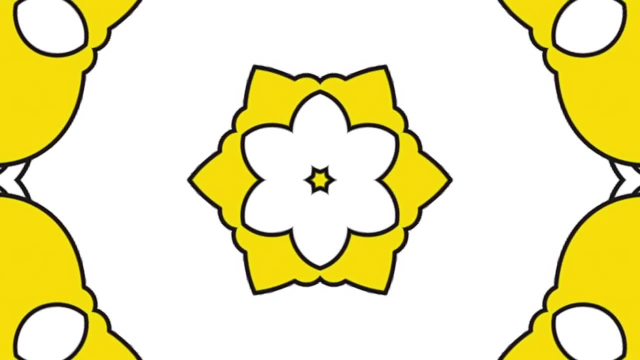 which is about 1500 pages long. It's huge, but it hadn't been updated And it wasn't the book that I wanted to write, even though it is a great, great book. And then I was on a plane once talking to somebody about CERN. 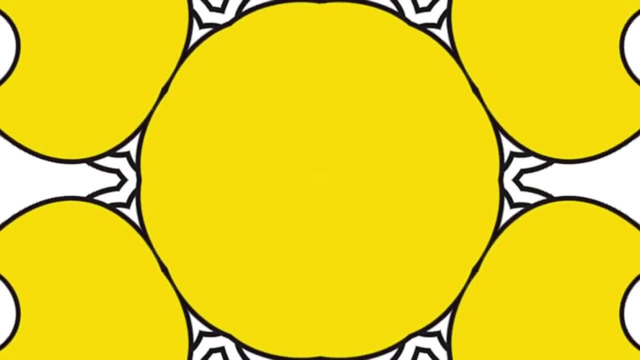 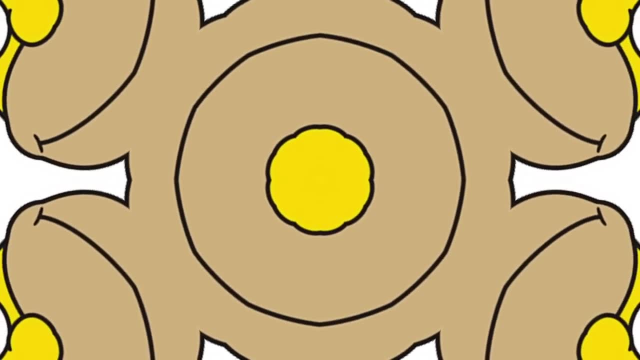 and particle physics and the Big Bang. And it was quite clear that this perfectly pleasant person had no idea, really, what the Big Bang theory was, or how much evidence we had for it or where it came from, And I thought, well, this is extraordinary. 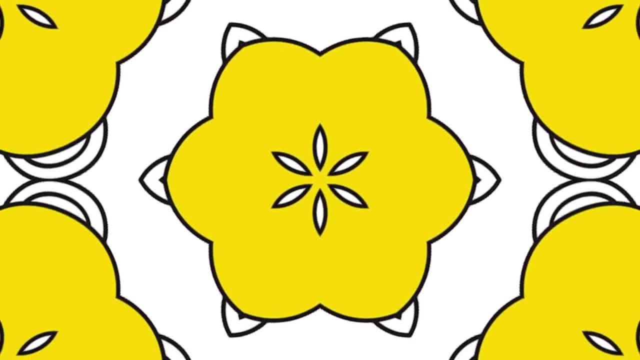 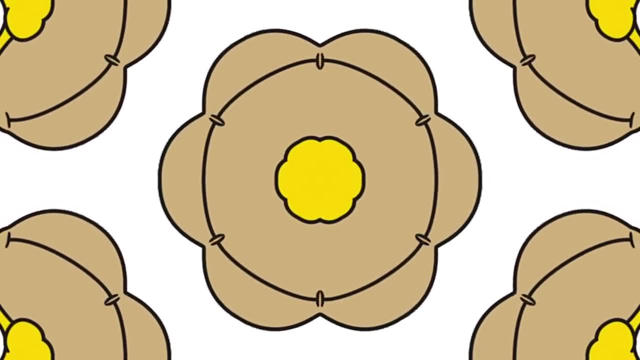 We're part of a unique generation. We're the first generation really to have a theory of the universe and its evolution and its origins, So everybody should know this story And that's where Big Bang came from. I think I wrote the proposal for that book on the plane. and faxed it back to my agent and said: look, this is it, And I've got the scrap somewhere of barely 50 words. And by the time I got back to England about a week later, that was it. The contract was signed and that was Big Bang, ready to write. 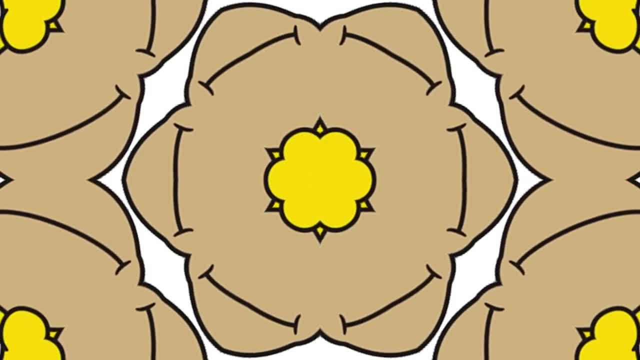 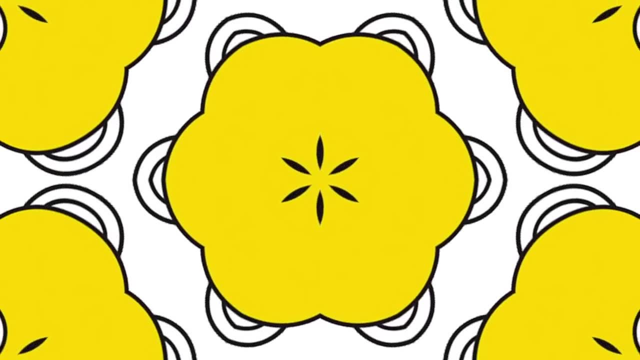 It helps when you've already had two pretty successful books. That's true. Yeah, Then I was going to write The Simpsons book, And that's just a great. that's just a fantastic idea When you realize that there's maths in The Simpsons. 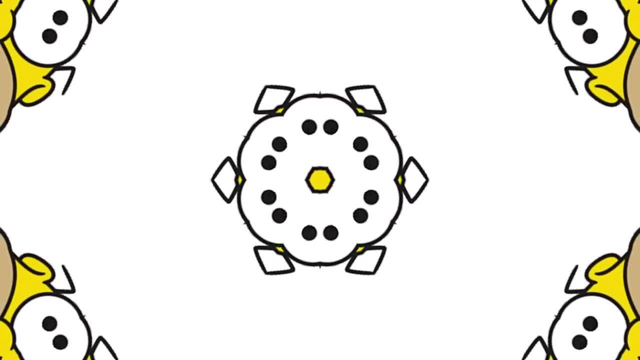 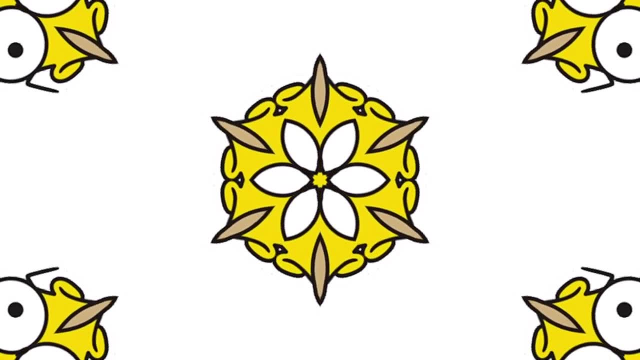 great stories are very few and far between. They're very hard to find, especially if it's a book story or a book idea that's got to last hundreds of pages and it's going to take up years of your life. It's got to be a really compelling idea for a book. 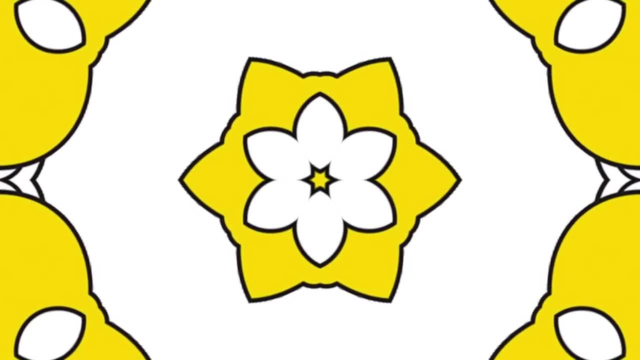 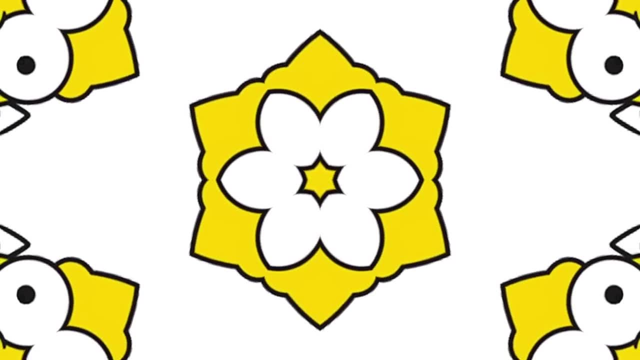 And The Simpsons is just absolutely a gift of an idea, And so once I'd realized it was there, that was a very obvious book to write. But then I got annoyed and angry about alternative medicine and I thought that was a more important book to write. 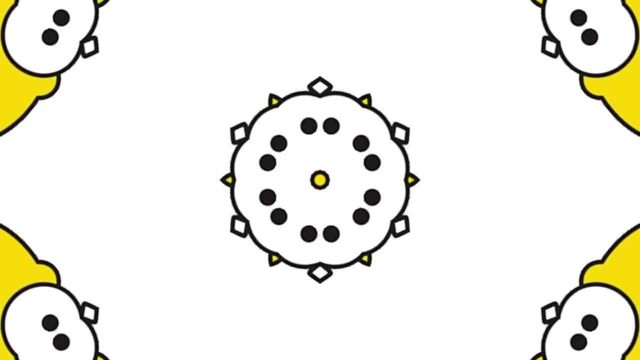 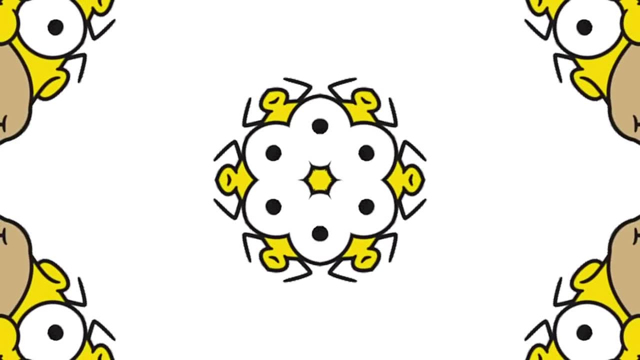 And I think this is where the campaigning side I think maybe starts- is. The Simpsons book was set to one side and I wrote a book with Professor Edzard Ernst, all about alternative medicine called Trickle Treatment. Our book is very critical of alternative medicine, but I think it's also very, very fair. 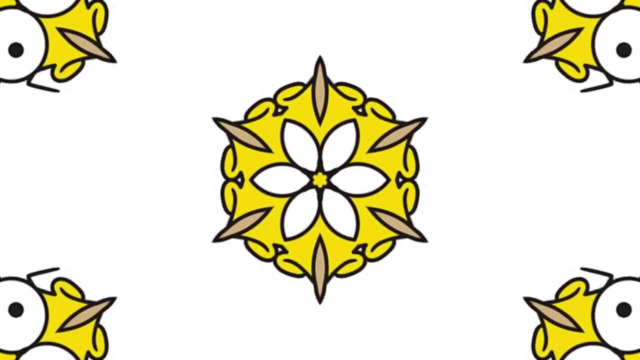 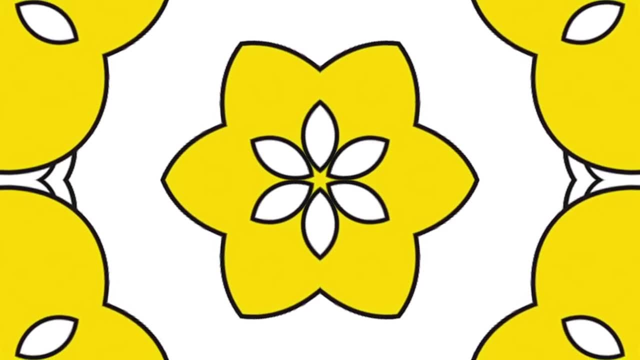 It's based entirely on the facts and the evidence. Where an alternative therapy works, we say it works. And then I got sued for libel, and that's where more campaigning stuff happens. Yeah, And then eventually, when that case ended, I got back to writing The Simpsons book. 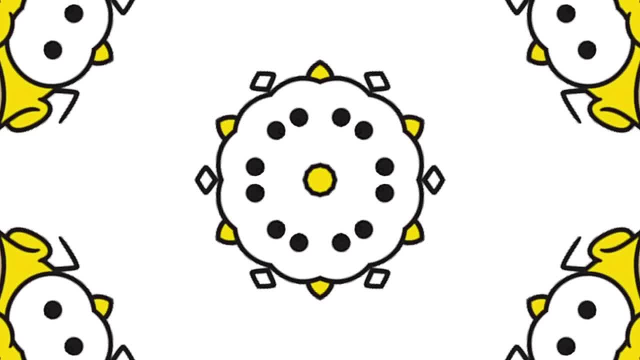 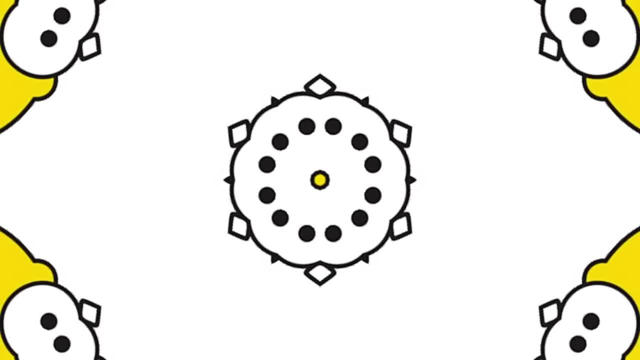 Yeah, That's where those five book ideas have come from. I have to ask you about the libel stuff, seeing you brought it up, because it's so fascinating to me as a journalist as well For people who don't know this story, because outside the UK it's obviously probably not. 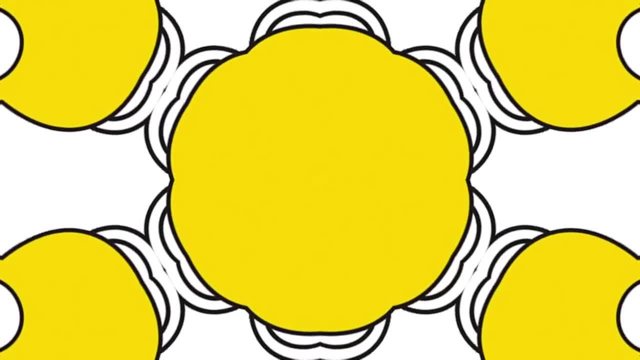 quite as well known. can you give them an executive summary of what happened? Sure, So I'd- It wasn't the book that got you sued. No, no. So when you write a book, you write articles to promote the book. 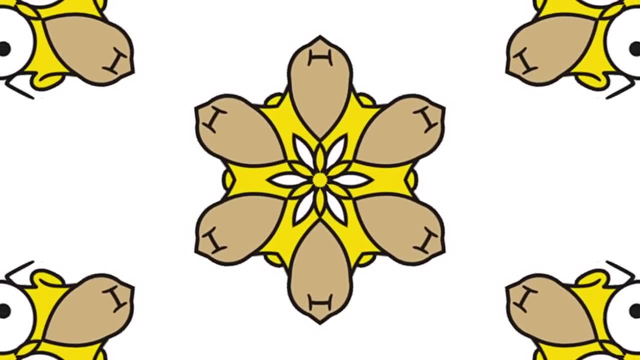 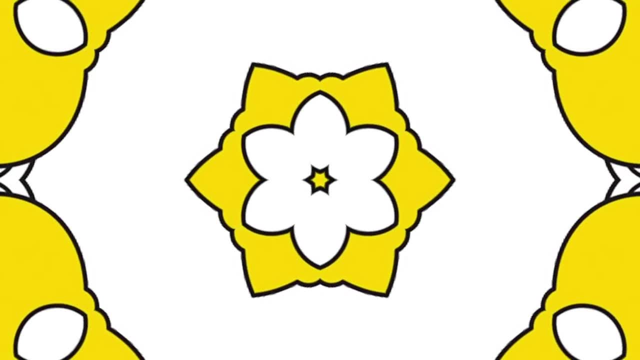 And I'd written an article for The Guardian about chiropractic. when I started writing the book with Edzard, I didn't know much about chiropractic. I thought they were just sort of physios that focused on your back. Turns out, chiropractors have a very, very odd history. 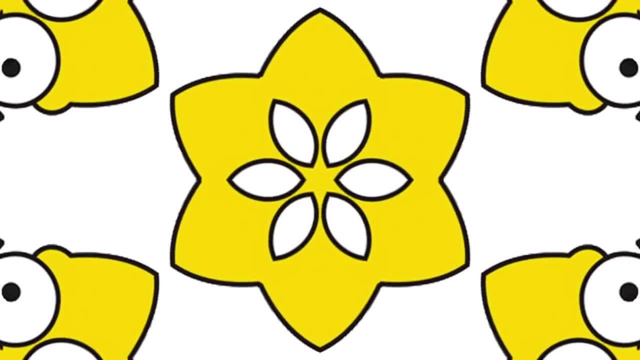 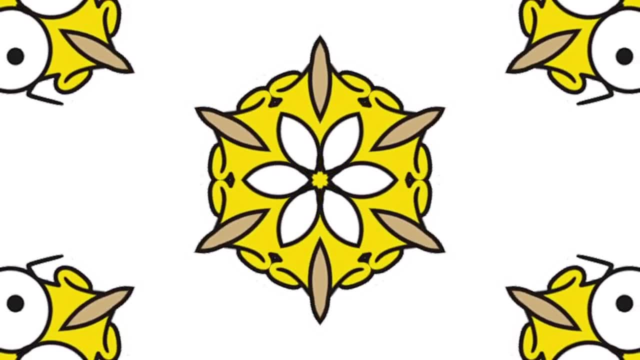 There are some good chiropractors who will just focus on your back and they will do some perhaps good things, but it's all a little bit questionable and some of it's very, very questionable: Manipulating babies that are just a day or two old, giving very dodgy advice about vaccines. 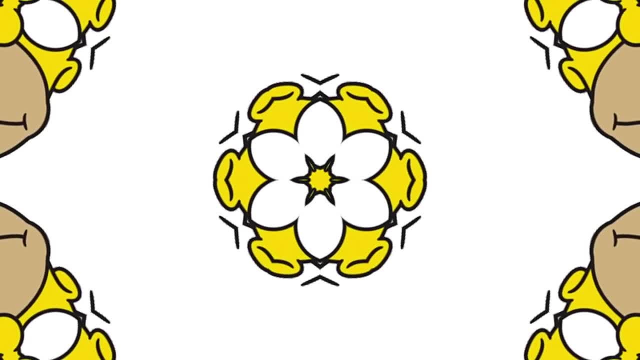 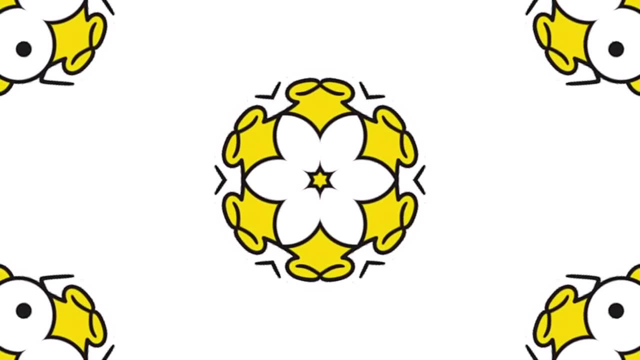 just really some disturbing things happening in chiropractic in general around the world. Yeah, So I wrote this article saying: if you want to see a chiropractor about your back, yeah, fair enough, Not for me, but you may want to do it. When it comes to other conditions. don't go near a chiropractor, was my advice, Because you'd already written a book. Yeah, When you wrote this article, did you feel like you were stepping on a landmine, or just feel like it felt like grist to the mill, sort of? 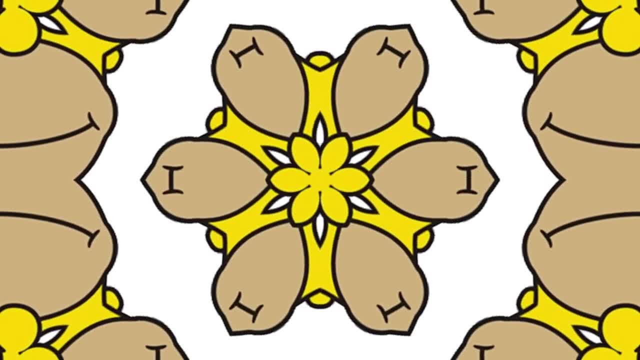 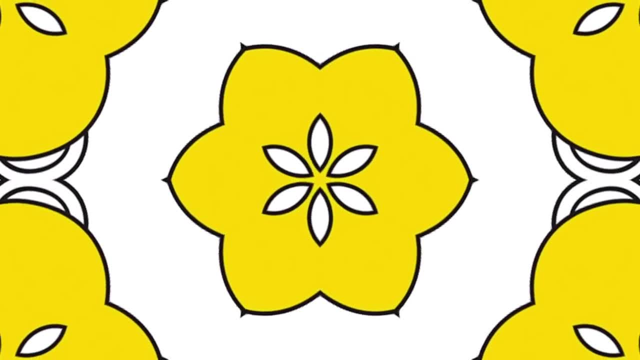 No, it was just I'd written it. I probably said to Edzard: Edzard, do you want to have a look at this? Any thoughts before I submit it? The editor at The Guardian would have read it. They may have run it past their legal team. if I don't think they did, because there. was nothing really contentious there as far as anybody could see. But a month later a letter arrives through the door and I still remember being sat there on the steps reading this letter, feeling nauseous immediately because it's a letter from a firm of solicitors saying that the British Chiropractic Association is threatening. to sue me for defamation? The paper or you, Just me? You'd think they'd go for the paper with all their money. You would think so. Never really thought about that before. Why would they just go for me? There are a couple of sentences in the article. 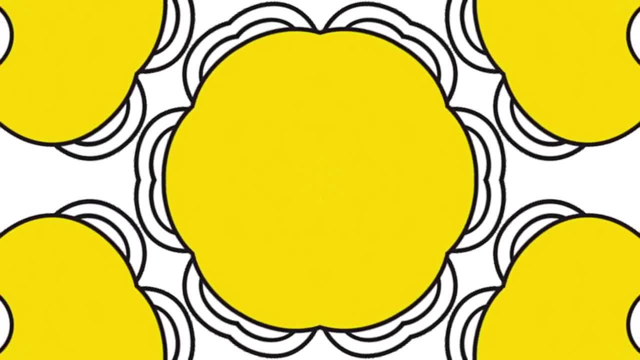 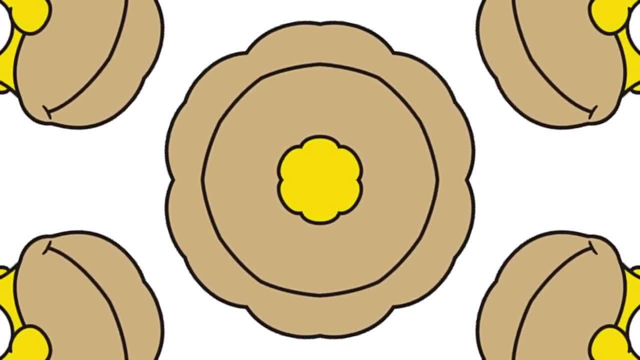 There's an article where I talk about they happily promote bogus therapies. There is a reading of that. There is an interpretation of that which says My interpretation was they're promoting stuff that just doesn't work, kind of blithely doing it. 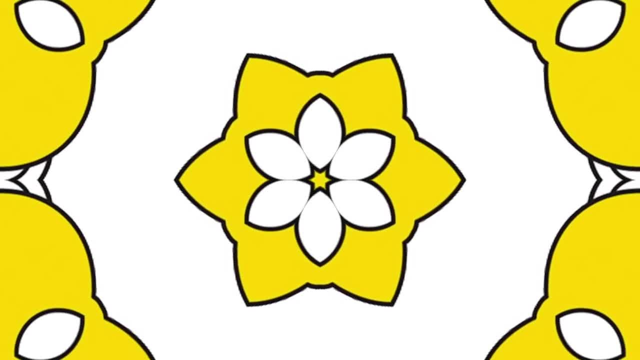 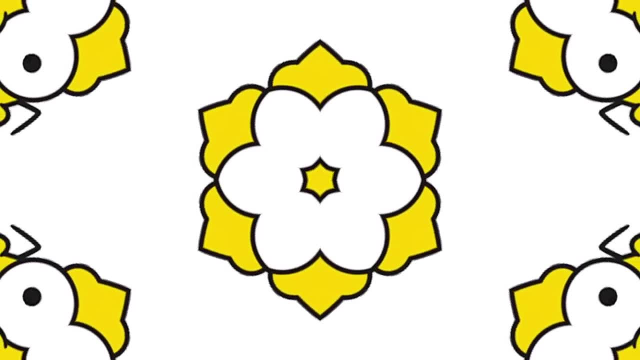 Their interpretation was that they are deliberate fraudsters who know their therapies don't work, and yet they do it anyway in order to get money out of the public. Now, there are things in my article that I think make it clear that's not the case. 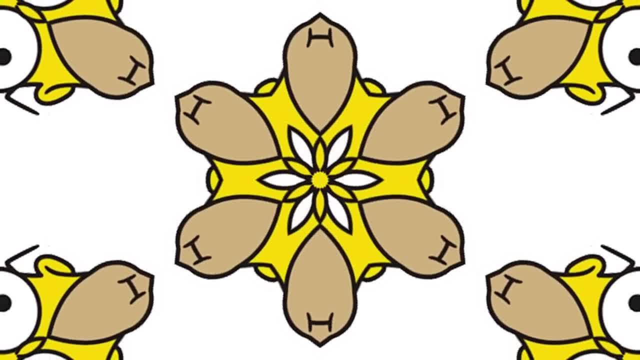 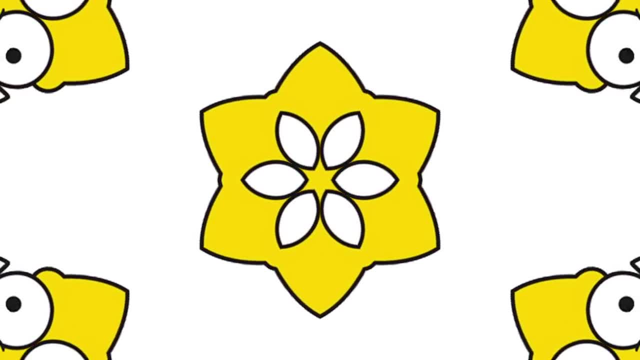 I call them fundamentalists. If you're a fundamentalist, you're not defrauding anybody. You have a deeply honestly held belief. but you may be wrong. So I thought there was a very different spin on it. They disagreed. 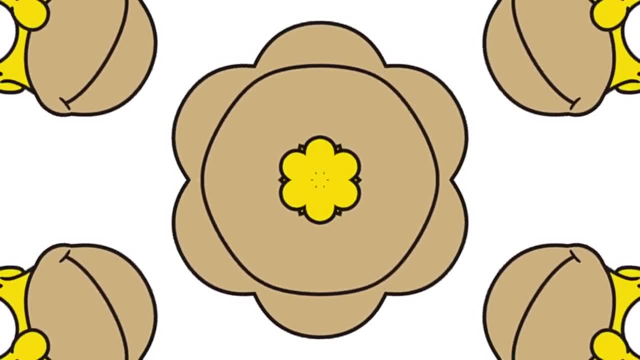 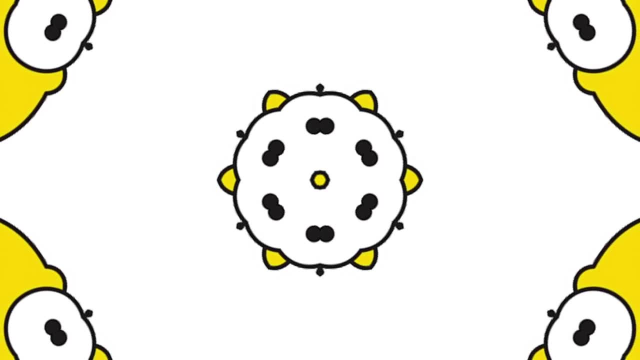 They threatened to sue me. The Guardian just said: look, we can't be involved because English libel law is so expensive and it's so one-sided. English libel law used to be horrendously anti-free speech, anti-journalist. And the Guardian said we're going to lose this case. People just lose libel cases all the time because the law is stacked against the writer And I quite accept that the Guardian couldn't stand by me because if they'd have lost it. 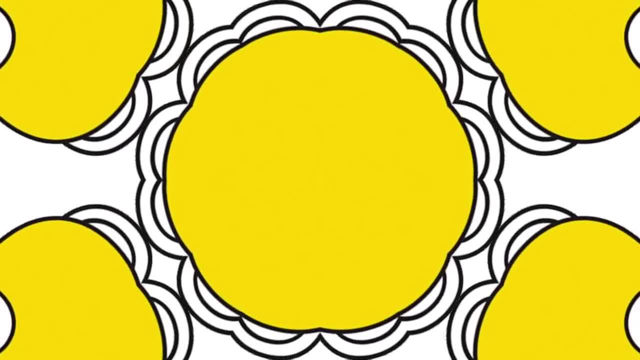 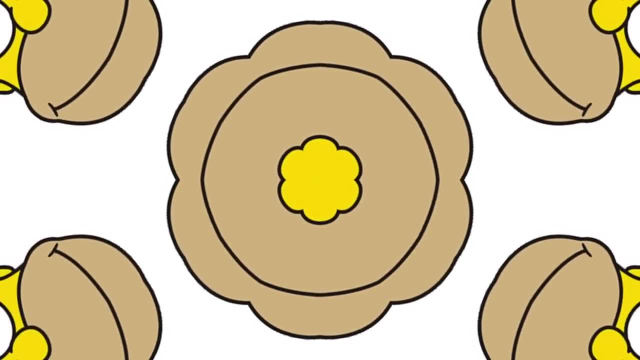 would have cost them, say, a quarter of a million pounds, and they would probably have had to lose two journalists. So it's not right for them to put the journalist's necks on the line for one little article by me. So I went to speak to a lawyer and he told me the same thing. 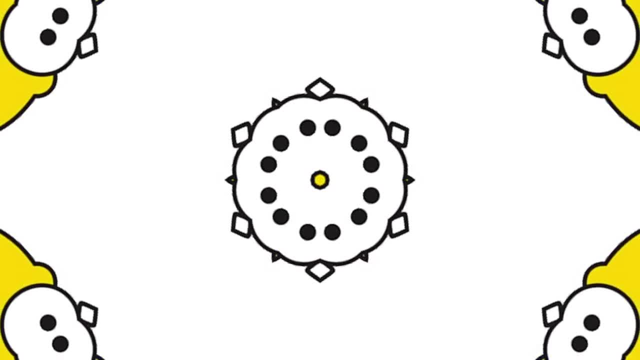 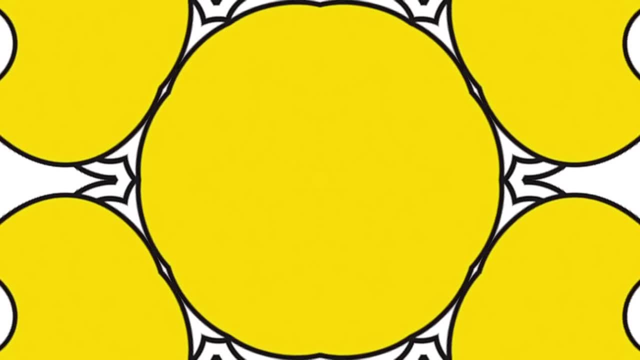 He said: oh, just settle, just write a nice apology, pay them a small amount of damages, Everything will go away. And I just couldn't. It just didn't make sense to me. How on earth could this be the right thing to do? 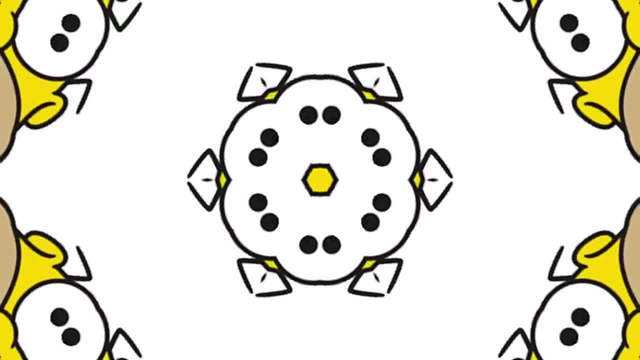 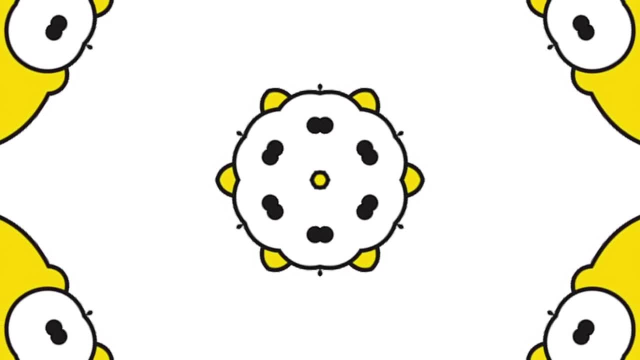 How on earth can anybody in the future, if they look at my Wiki page, how could they ever trust my writing again? Simon Singh, who was found guilty of libel. So that wasn't going to happen, And so I just said: look, we'll just rebuttal the claims and we'll see what they do. 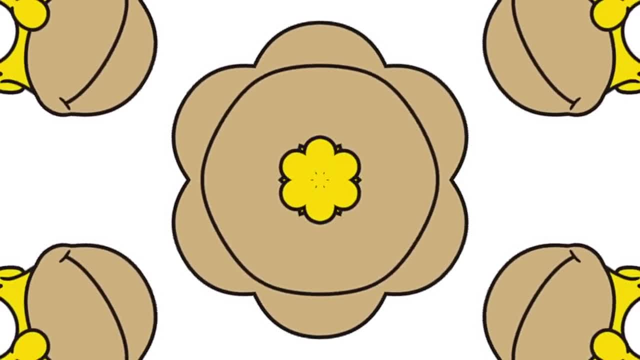 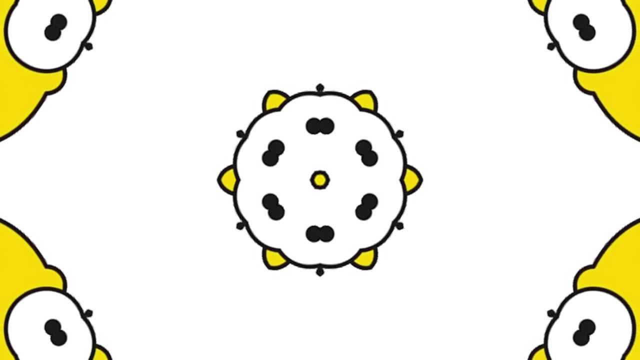 And I just assumed they would back down, but they didn't. It became a right old mess, didn't it? Yeah, There was something called a preliminary hearing, where you say, before we go to court, let's agree what these words mean. 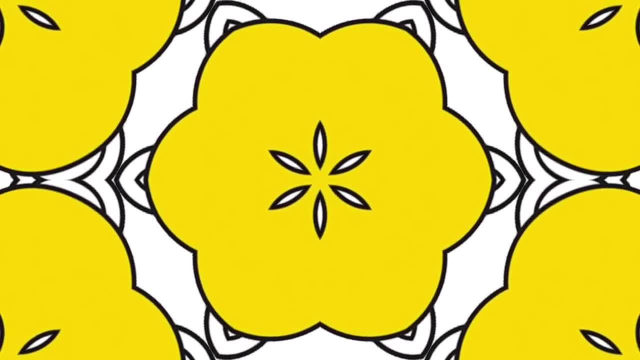 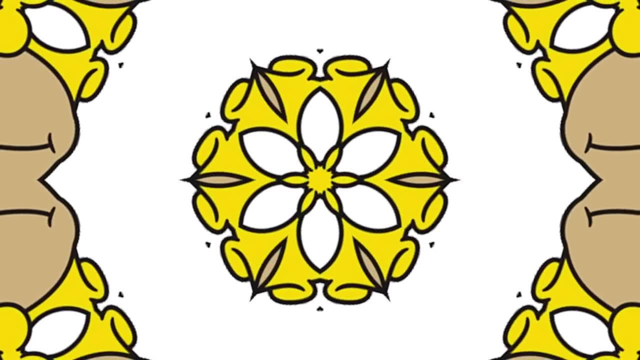 Do they really mean that I'm calling you a fraud or do they just mean I don't think that what you do works? And the judge at the time, Justice Eadie, sided with the chiropractors and said it was plain as a pike staff that I was defaming them, that I was calling them fraudulent. 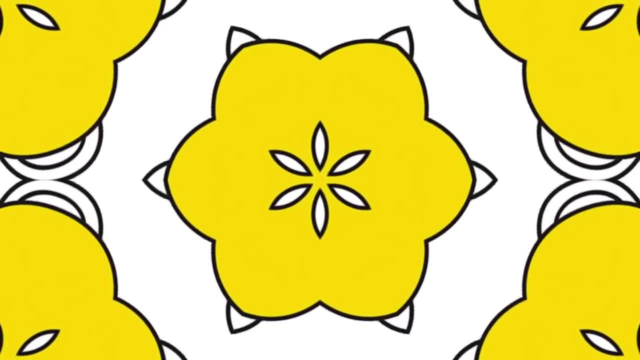 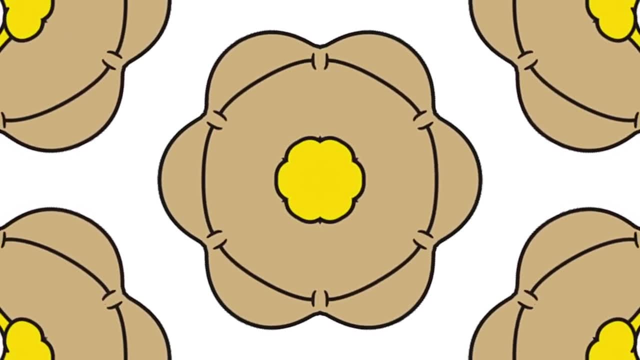 And at that point it looked like we'd lost, there was no point carrying on. And what I did at every stage was I just kind of did a cost benefit analysis That by that stage I think it had already cost me sort of 50,, 60,, 70,000 pounds. 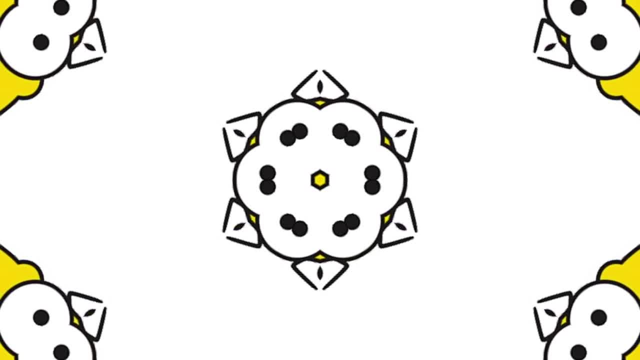 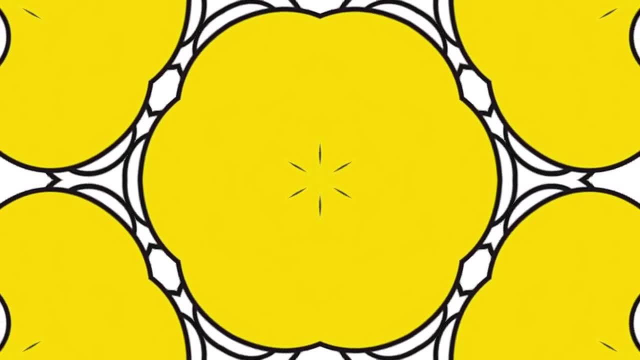 And I said, look, if I lose now, it's goodbye to that money. Now I was lucky because, as you said, I had three or four successful books by that stage, And so I could afford to take that loss. It would have been painful, but my wife is a journalist as well, so she was standing 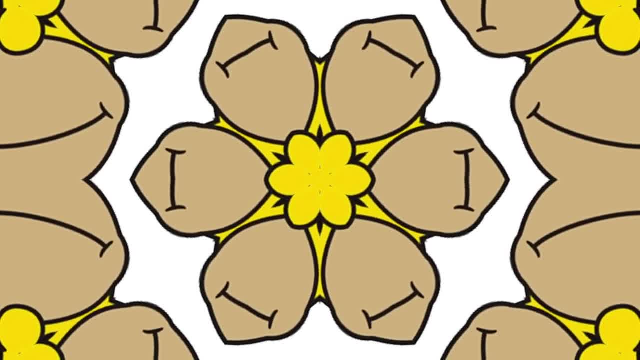 right by me. I had her support. I had a bit of a financial cushion that I could rely on, And when I looked at the cost benefit analysis, it was a case of if I spend another 20,000, I'm going to lose. 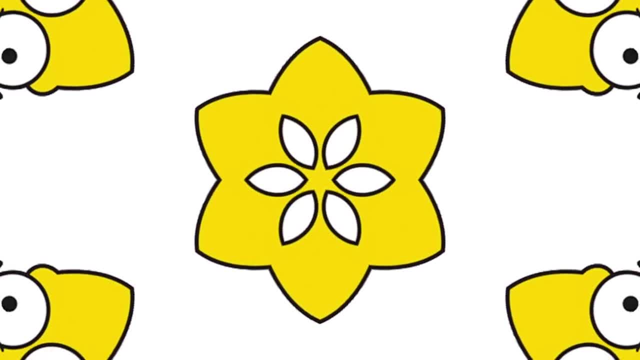 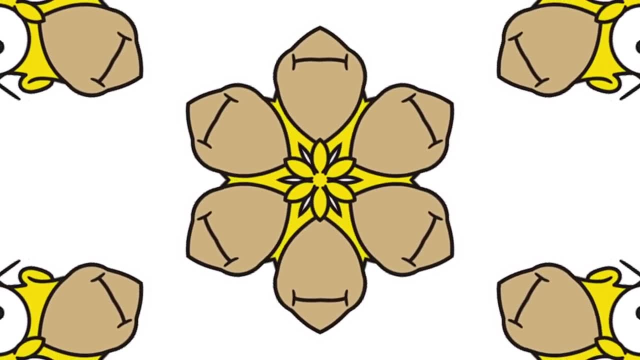 If I lose another 20,000, let's take this to appeal. I could lose another 20,000 pounds, but I could hopefully save a lot of money, save my reputation and prove that I'm in the right. We were refused the permission to appeal. We appealed again for permission to appeal. Eventually, they allowed us to go to the Court of Appeal, which was a really big deal Because by this stage- and this was two years later- the Court of Appeal had the master of the roles and the law chief justice on it. So they brought out some of their really big guns, Because by this stage lots of people were writing about it. It had become a bit of a core celeb, hadn't it? for the whole issue I was getting support from Norway and America and Australia because there was this other problem that our libel laws were so one-sided that it encouraged libel tourism. People would come to London to sue because this is where you'd win. Russian oligarchs would sue in London. Ukrainian newspapers would end up getting sued in London. 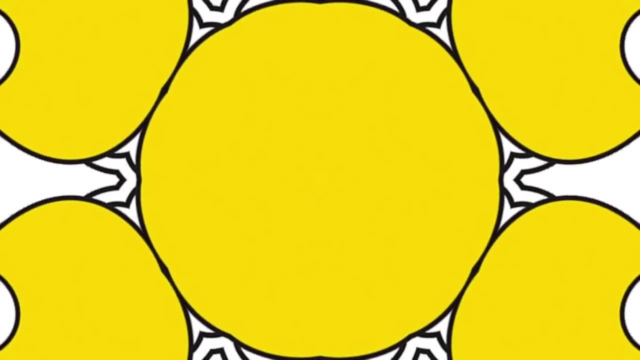 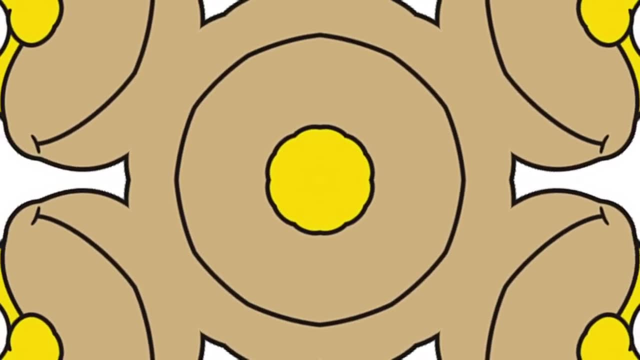 And so that's why I think the Court of Appeal was so powerful in its members And, luckily Well, luckily, Yeah, Whatever it was- they could see the sense of it And they said: look, when discussing scientific medical health issues, issues that are seriously, 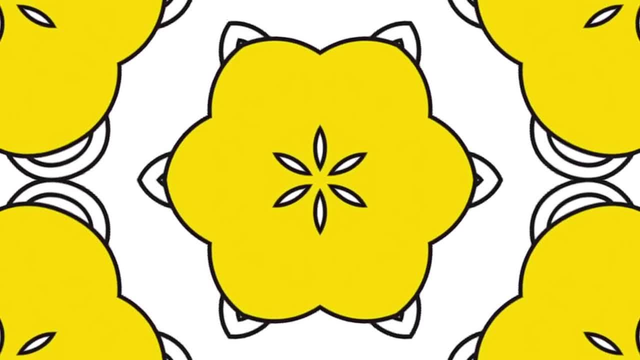 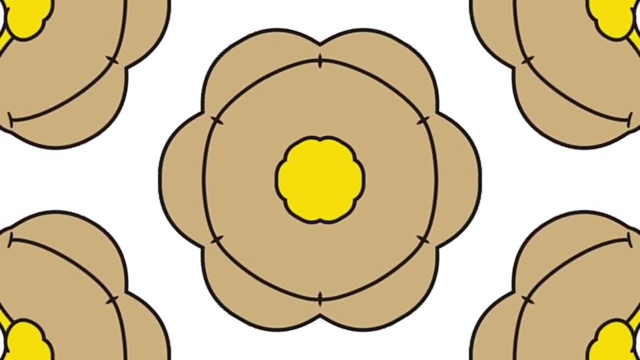 in the public interest. we must allow journalists to be able to speak up reasonably and fairly, Not maliciously and not recklessly, but we have to allow people to speak their minds and not to have them treading on eggshells in fear of libel threats. 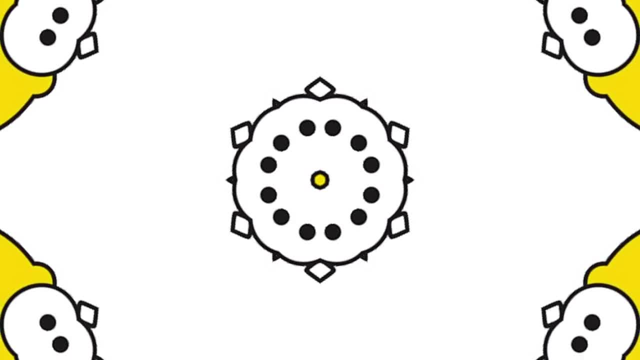 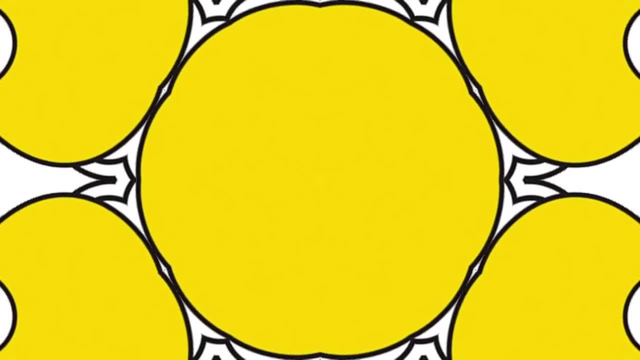 There was this thing called the libel chill, which is that you didn't even write certain things because you were scared of what the repercussions might be. So they had to remove that. So that was the end of my case. But then lots of other people, as I say not just in the UK, but also from around the world- human rights groups, charities all banded together, A lot of skeptics, a lot of rationalists, a lot of scientists, a lot of bloggers, a huge community on the internet who'd been threatened with libel. They all came forward and we worked together on trying to change the libel law, the defamation. law And that resulted in the Defamation Act 2013,, which now means we have a much fairer libel, And I think that's what we need to do. I think that's what we need to do. I think that's what we need to do. 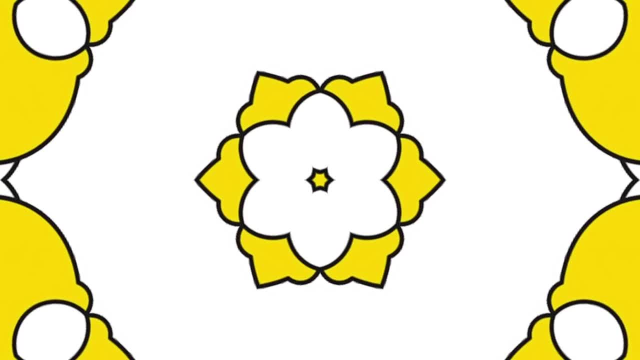 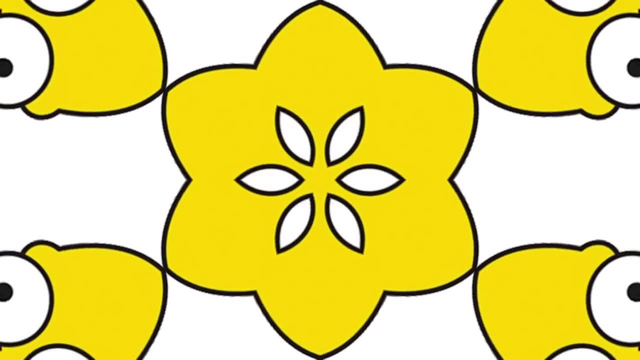 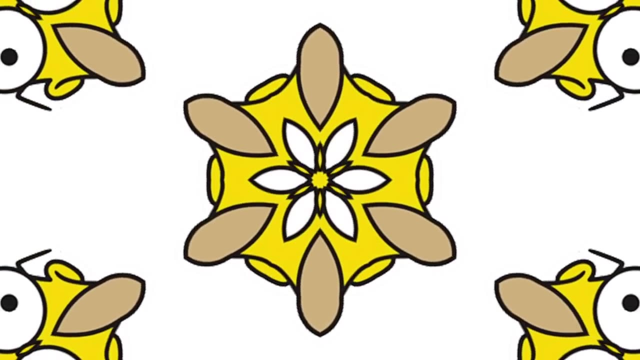 We need to have a much fairer libel law in this country And the experience over the last five years suggests that we've not had those high profile scary cases where people say: how ridiculous is that? How could that possibly happen? Academic journals have a huge amount of protection now. 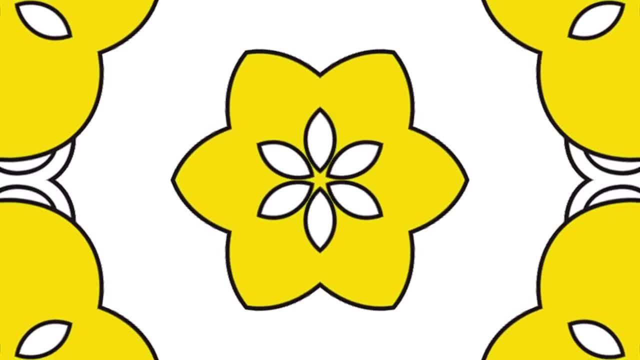 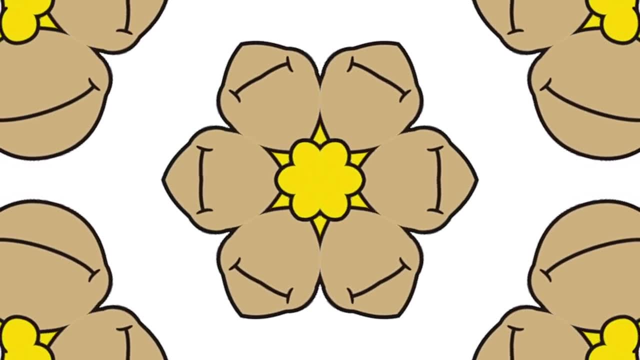 Scientists have much more protection. The law is still there. If somebody says something nasty about you, then you should be able to defend your reputation as an individual. That's really important. Nobody wants to get rid of libel, But the big, powerful body. 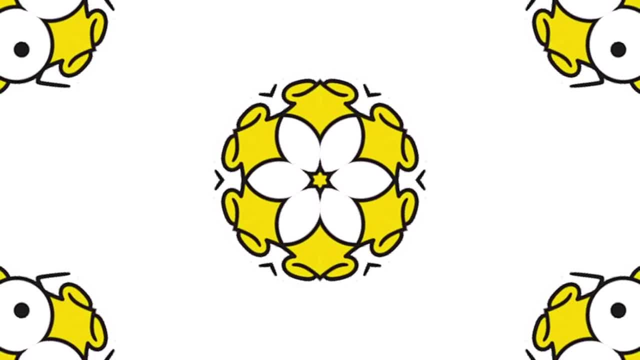 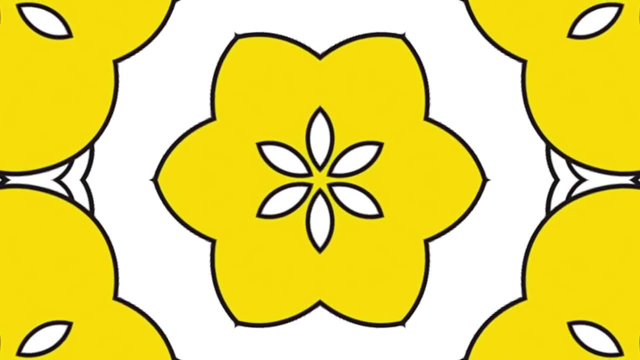 Everybody should not be able to use libel to bully journalists. That's where that change has happened, And there are people like David Alan Green, who is now quite a well-known blogger on legal issues, And he was one of those people right there at the very beginning who started blogging. 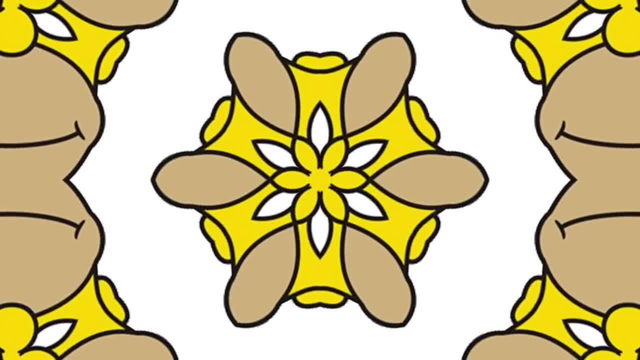 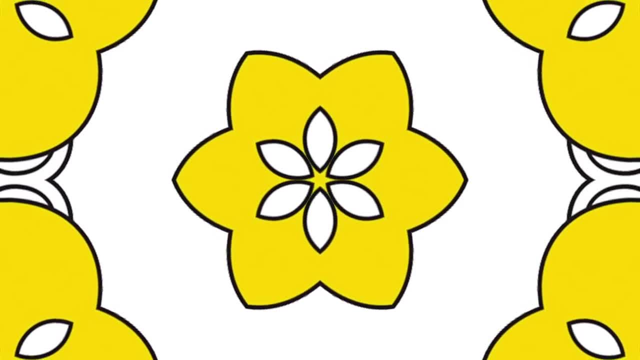 about my case and helping me with my case and beginning to build this campaign. Organizations like Cents About Science that people may know about. absolutely at the heart of this campaign. Index on Censorship: English Pen, Global Witness. large numbers of people worked on this. 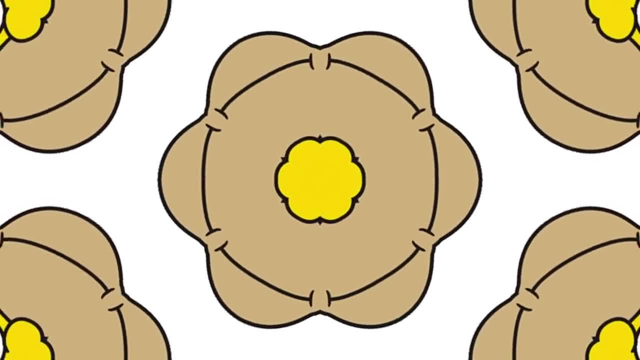 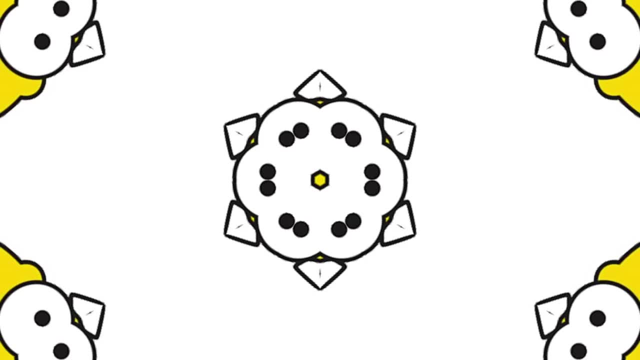 And yeah, so now we're in a much better position. How close did you come to packing it in Taking the loss? How many times Were you ever teetering right on the edge, or It was always a consideration. It was always a case of right on the one side. this is what could happen. 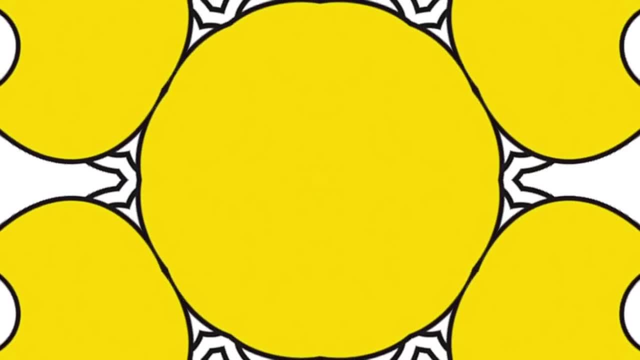 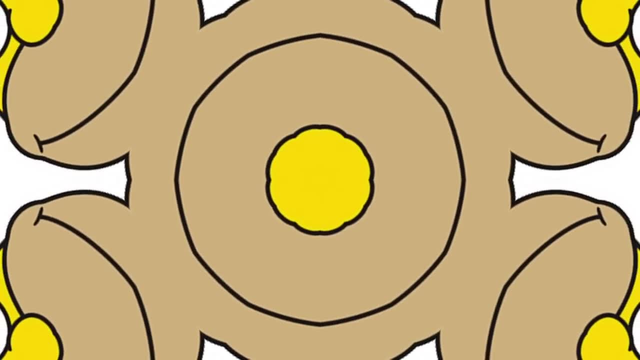 On the other side. this is what could happen, So it was always a consideration, But there was never a day when a pen was hovering over the page and thinking: ah, I'll just write this off. The day when we lost the preliminary hearing was disastrous. 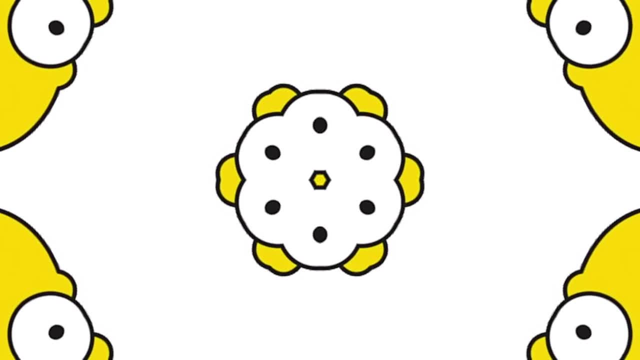 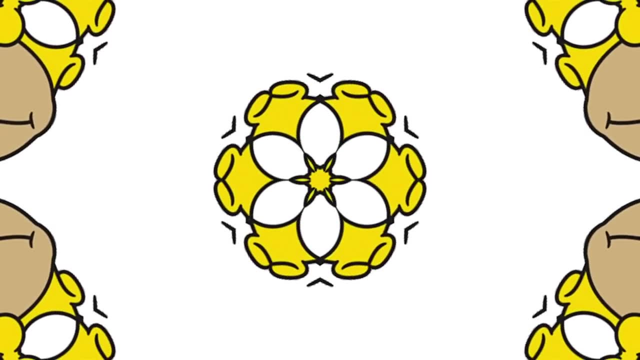 I remember Robert Dugans from Brian Cave was my solicitor And we just sat across the table from each other and just said: what do we do? There's nowhere to go here. The judge has just told me that I've accused them of fraud. 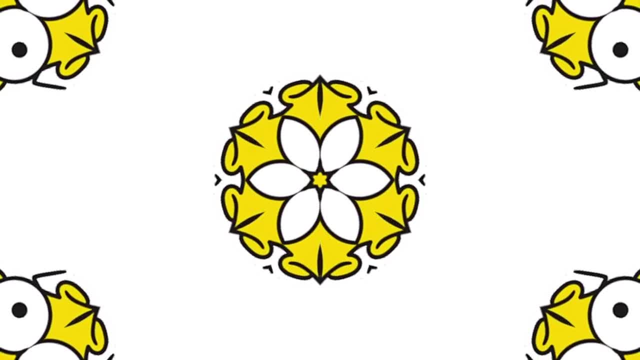 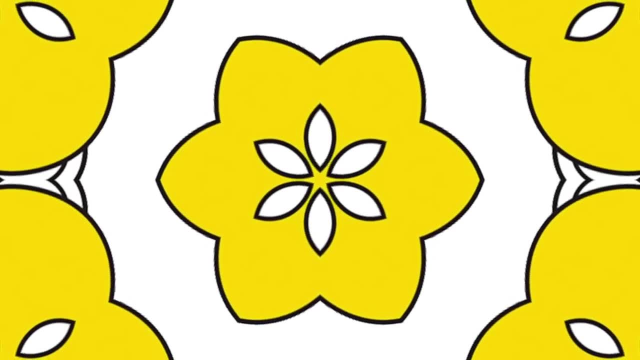 That's not what I meant And that's not a statement I can defend. How do we go? Where do we go from here? So there was a point there where it was a case of how do we write the apology letters. How do we get out of this as quickly as possible? 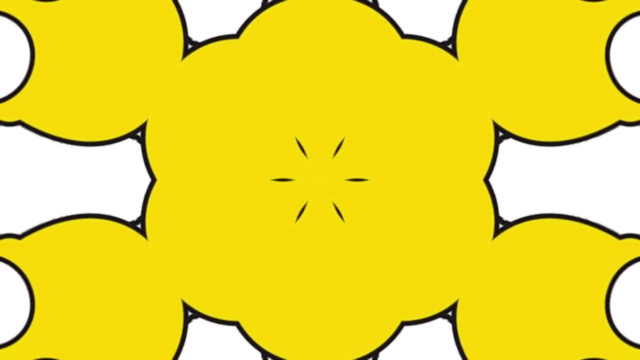 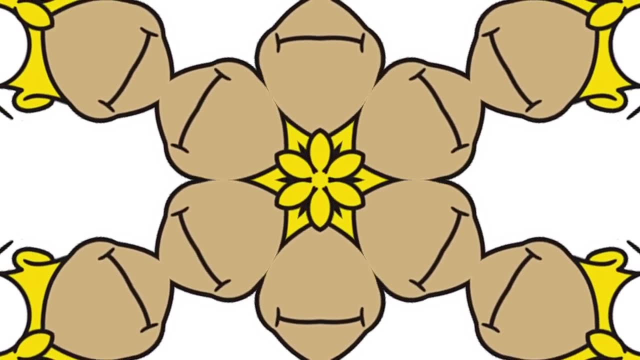 Are you glad you wrote the article Because of the good that came? If you could go back in time, would you rewrite the article and keep yourself out of trouble? No, It's. a great number of The libel reform came out of that article. 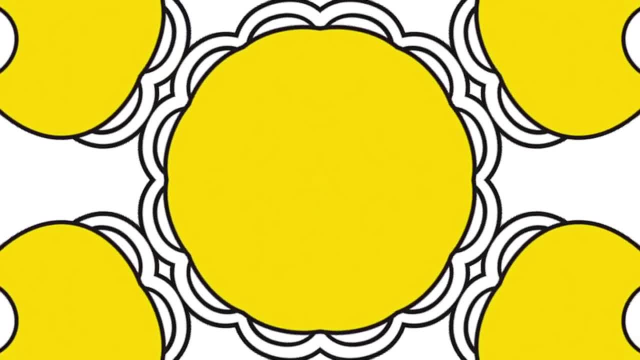 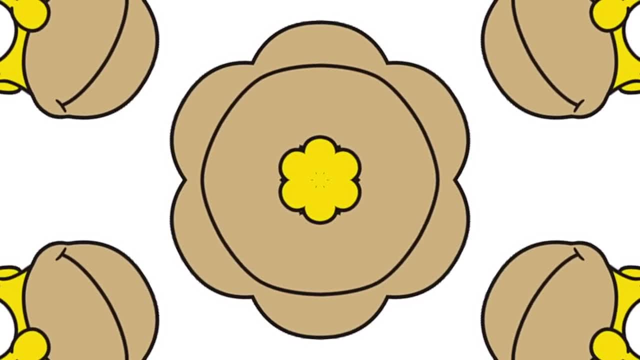 Also, Ben Goldacre was sued. at the same time David Colquhoun was being sued. It was a great thing And again, it probably The first time I'd ever gone to see my MP. I'd never done that before. 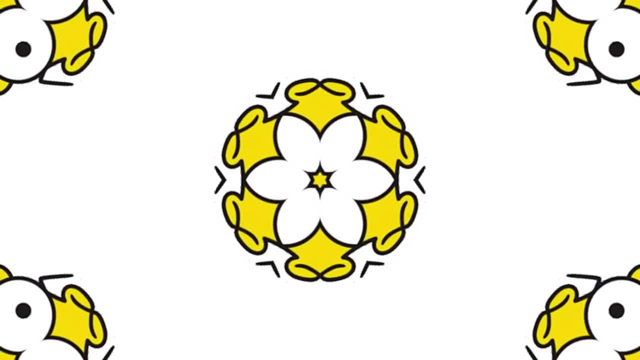 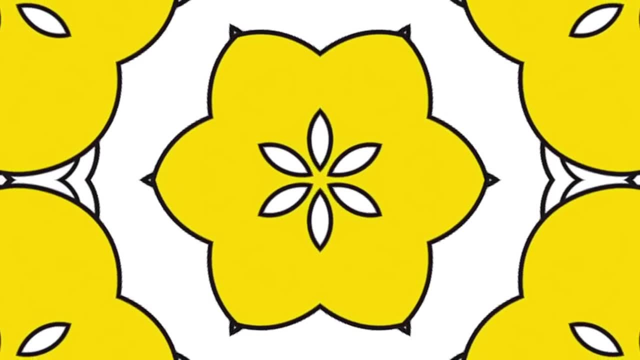 And I think other people who were involved in the campaign went to see their MPs, And so I learned about how you can begin to change things, how parliament works. One of the things we wanted to do early on- we wanted to get this on the parliamentary. 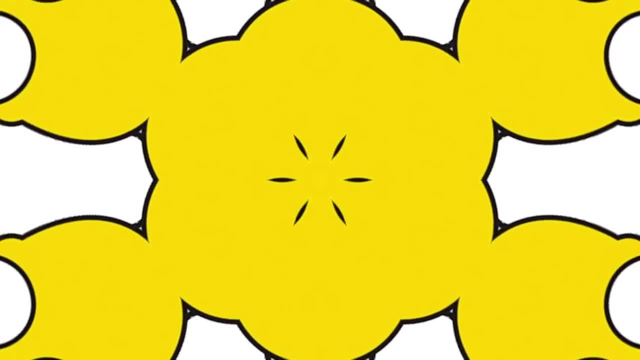 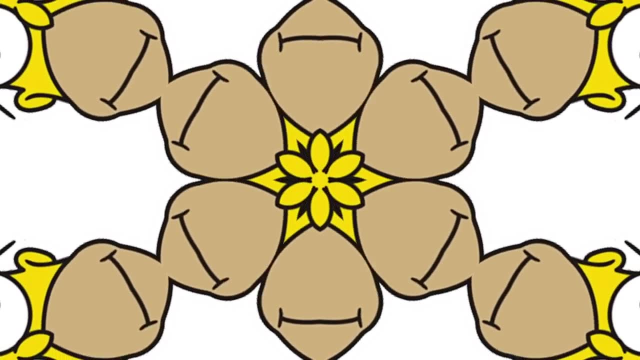 agenda, So we had to. One of the ways to do that is to have an early day motion. So I think any MP can put something down in a book and if other MPs support it and it gets enough support, then the government has to consider it as something that they need. 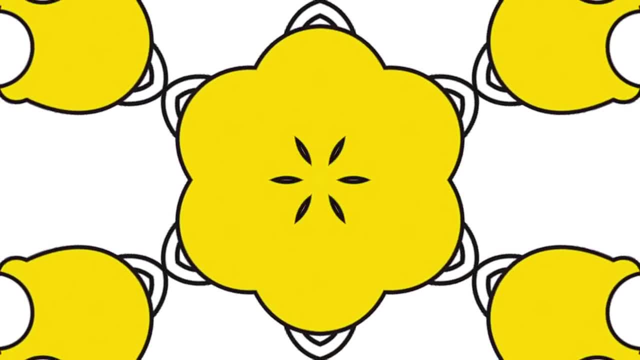 to take on board. And so we said, great, we'll get an early day motion. Who's our MP, Who's going to put this forward? And then we said we can't do that, because what will happen is that we'll encourage everybody. 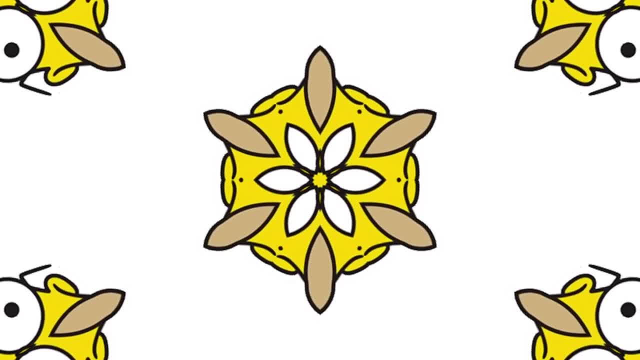 to write to their MPs. Their MPs will look at this early day motion. They won't know what to do. They'll go and see their party officer. The party officer will say: we don't know anything about this, Don't bother signing it. 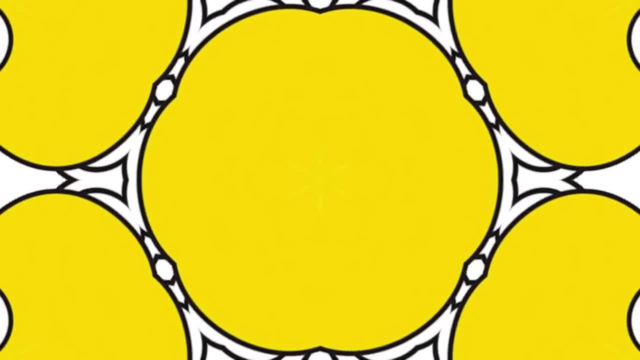 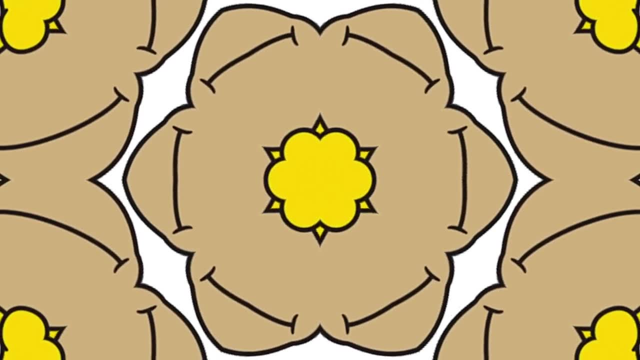 And once an MP said they're not going to sign it, they're reluctant to change their mind. Instead of doing it that way round first, we need to spend three months lobbying all the MPs, first informing them, bringing them up to speed. 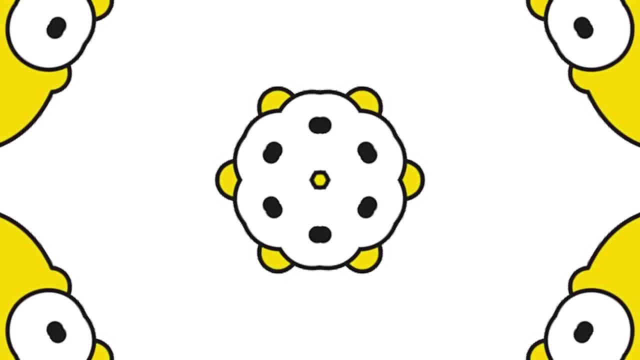 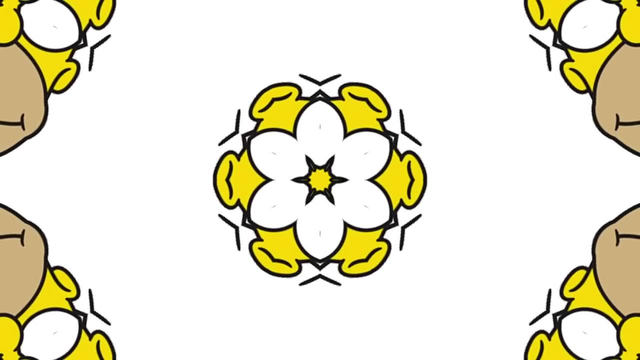 Then we put down the early day motion, Then we get people to write to their MPs, Then the MPs know what to do and they will back it And it was the biggest early day motion of that parliamentary session. So learning about the levers of government and how you make change, how you work with 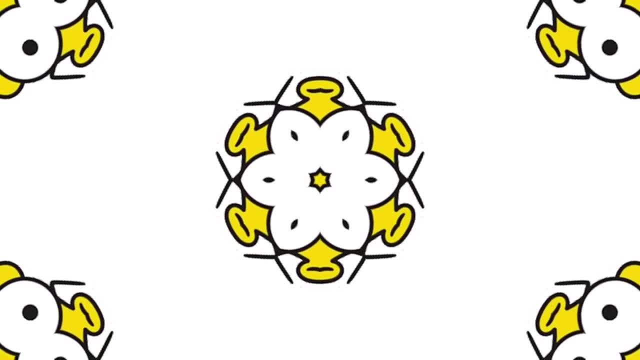 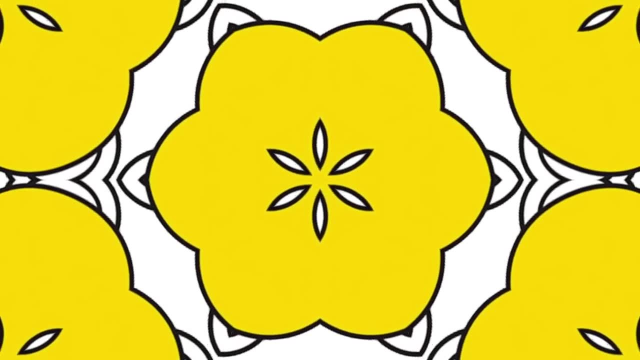 the party conferences to bring the parties on board, How you sometimes play one party off against another. All of those things were for a kid who was doing a PhD at CERN and was only interested in quarks and so on. This was a whole new world and I'm very happy to have published that article and happy to have survived it? Did you end up seriously out of pocket or did you end up, like you know, you weren't on the bread line? I'm trying to think what the costs were in the end- The costs in the end, my costs. I'm thinking about 200,000 pounds. Yeah, I was presented with a legal bill at the end of 200,000 pounds From your lawyers and people who'd helped you and all that sort of stuff. Yeah, So all the people I was responsible for paying for, Yeah, And they had a legal bill probably of about- let's call it- 200,000 pounds as well. Possibly. yeah, The other side, The other side as well. Yeah, So had I lost, I would have had to pay the whole lot, Right? So that's why it was terrifying amounts of money. Yeah, Now, because they lost, they have to pay their own bills. That's the end of that. But you still had to pay yours. No, no, I can claim my money back from them, Right? But they will argue every single line. So they will say, hang on, you had a meeting here with your senior barrister. 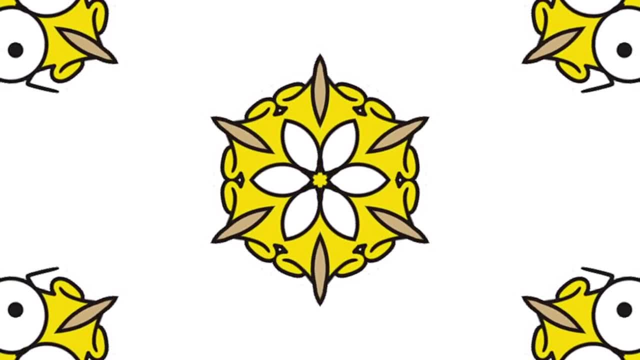 Why didn't you only have a meeting with the junior barrister? Look, you had two meetings here in three days. Why couldn't that have been consolidated into one meeting? Okay, They will argue about every single point, And so you only get back about two thirds of your money. 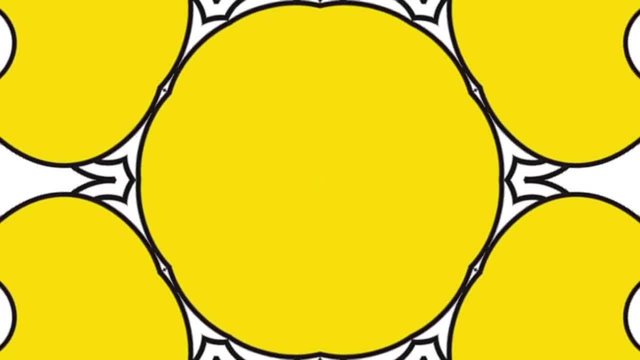 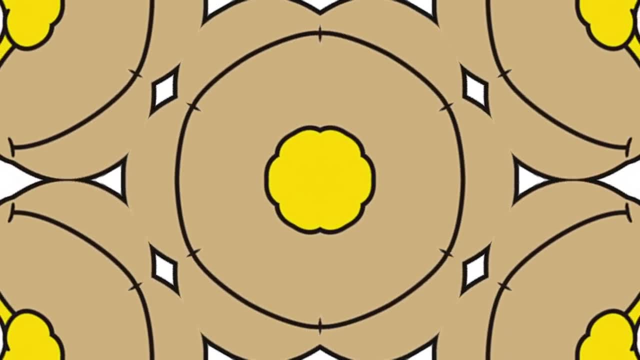 Right. So I was still 70,000 pounds out of pocket And the Guardian. these numbers are not quite right, but at the end of the day, whatever the shortfall was, the Guardian was very, very helpful in bridging that. 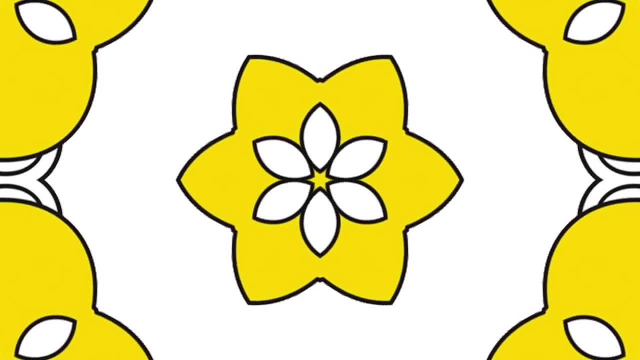 Okay. So I absolutely understand why they weren't there at the beginning, but I'm very grateful that they were there at the end. And also, I mean, the other cost was that during those two years I wasn't writing a book. 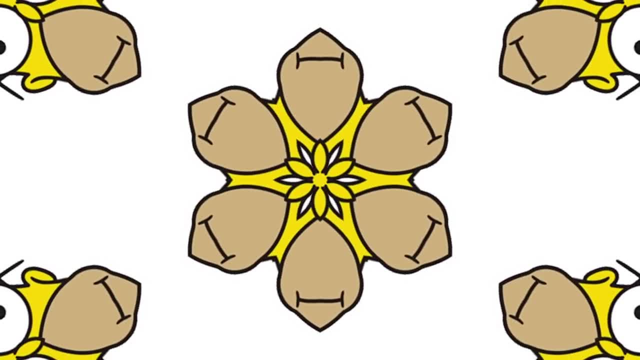 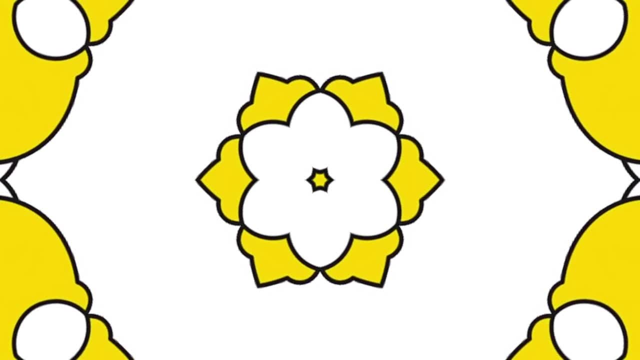 I wasn't really traveling or lecturing, So you're not doing any work either. How has Simon Sink not written the definitive libel book? This sounds like an amazing story. You talk about meeting Andrew Wiles and the compelling human story of that. 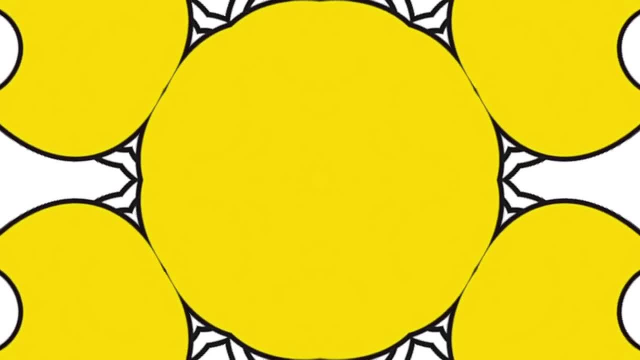 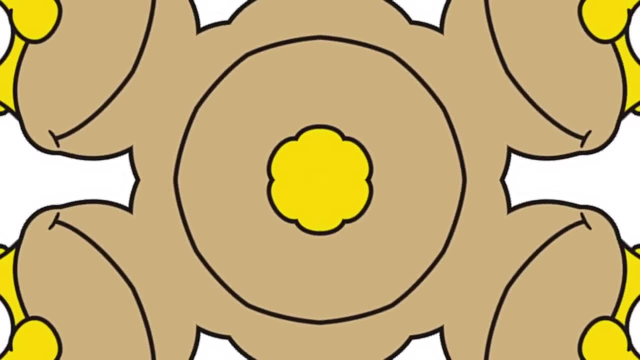 You sitting on the steps feeling sick with that letter sounds like a great opening to a book. Yeah, maybe, Maybe It'd be interesting listening back to this. One of the things I don't like doing is talking about how I feel, Right. 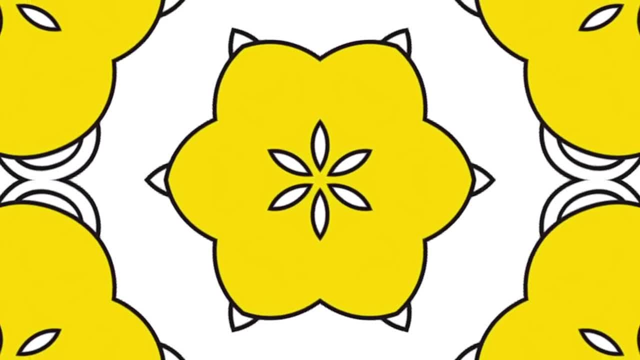 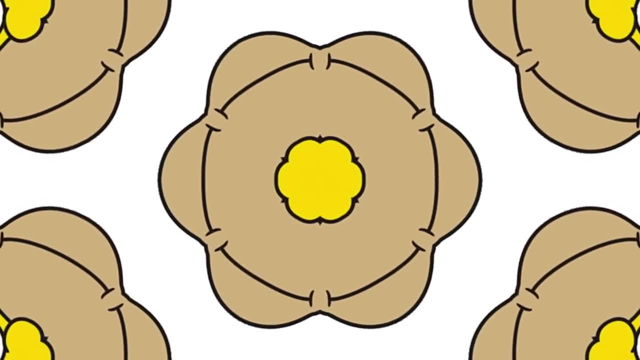 And so I can tell you facts. I can tell you there was this libel case and there was that libel case and there was David Allen Green and there was Facts. I can tell you- And I can probably even do quite a good job of this- is how they felt and this is how. they felt and so on. But in terms of how I feel about things I tend not to be very good at. So I think if you're going to write that sort of book, you need to be very open with how you felt. 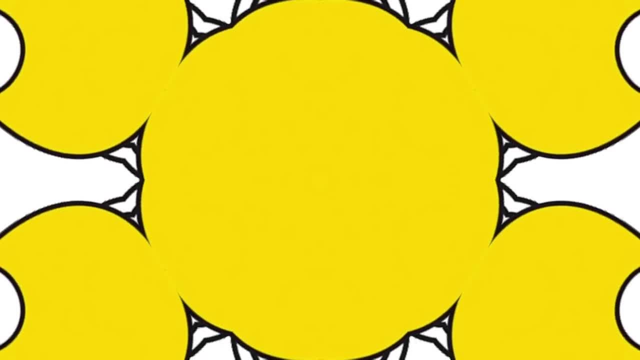 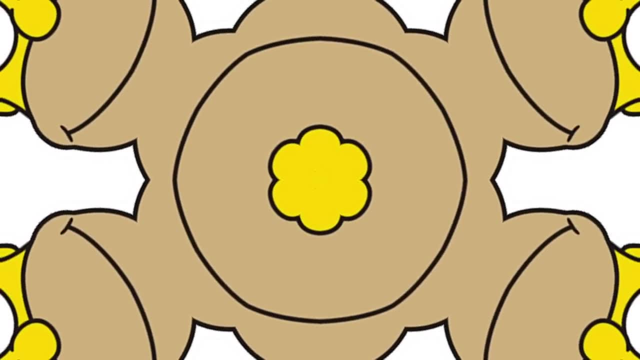 I can imagine the family conversations over the breakfast table During that period. it would have been compelling. Yeah, Yeah, It was, But we So. my first son was born. My wife was pregnant, actually during the final Court of Appeal and I think she was trying. 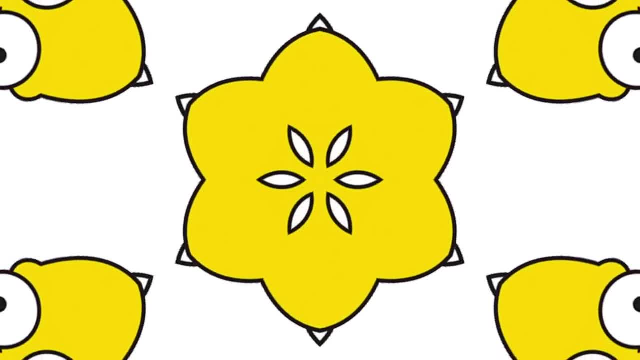 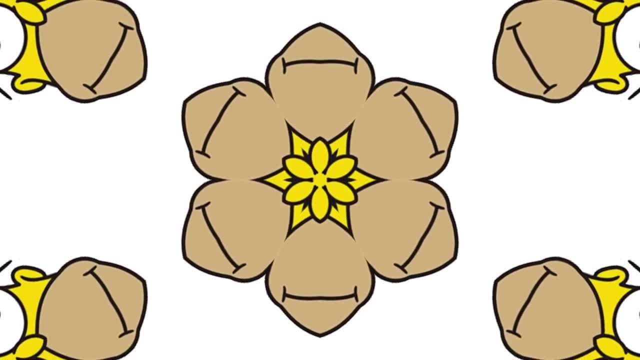 to catch the judge's eyes to try and gain some sympathy. But I was saying the bulk of it happened when we didn't have children and this sort of dominated our lives And, as I said, my wife's a journalist, so she was absolutely there every step of the. 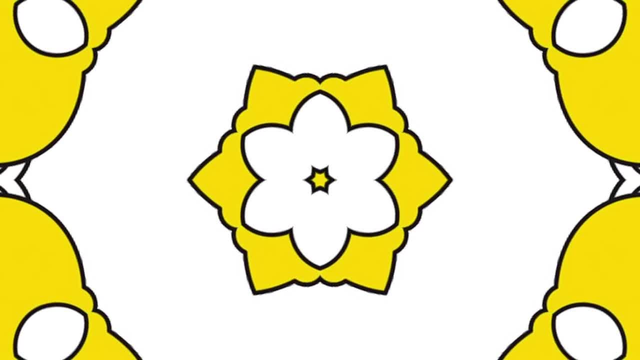 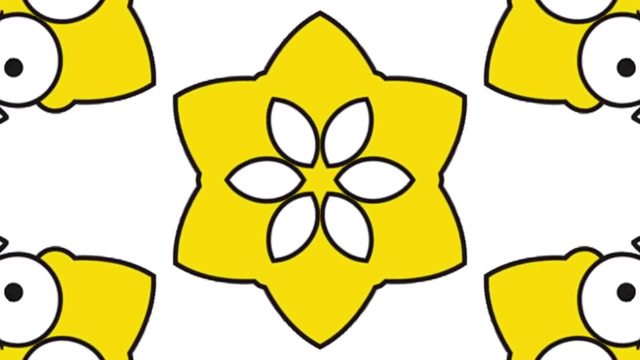 way, And all those people out there, All the people that Listening to this and who followed that campaign and who wrote to their MPs or who tweeted about it or who blogged about it or who mentioned it to their mates in the 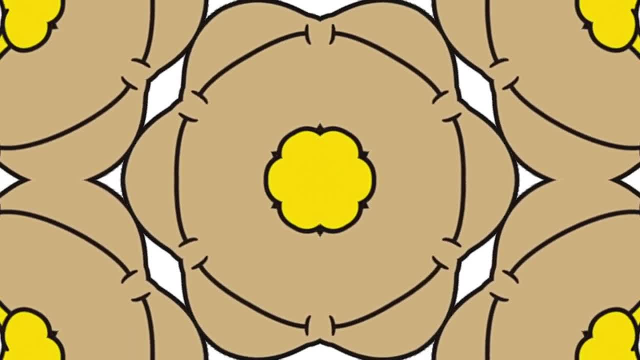 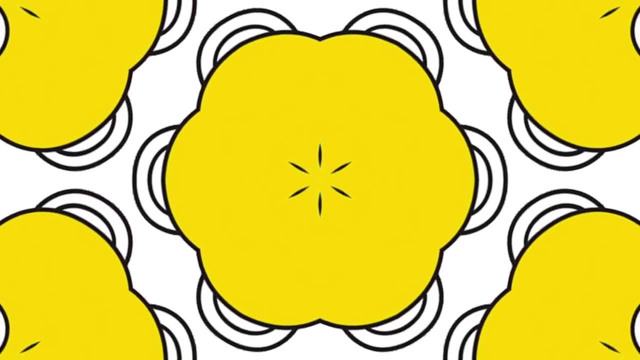 pub, All of those people saying that I wasn't the crazy one, that the law was crazy- That made a huge difference, absolutely. Had I just been left high and dry, I would have then just thrown in the towel, But had I been high and dry, I wouldn't have needed a towel. 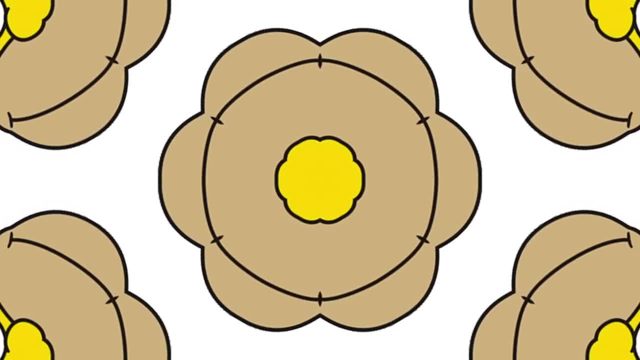 So there we go, For all the successful things you do: television, books and other things you're doing now that we'll talk about in a moment. how much do you think the liable thing will be like? well, one of your real legacies. 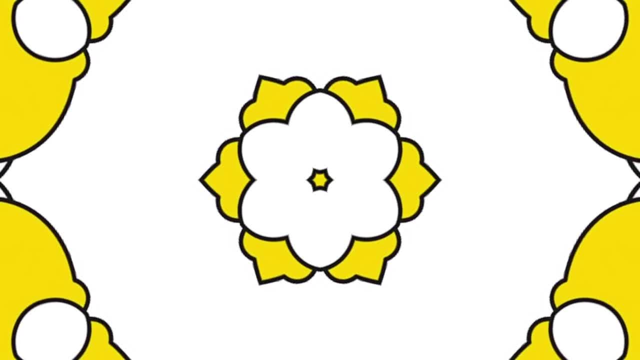 I mean, that's how I first heard of you was. oh, Simon Singh, he's the liable guy. Oh yeah, I know that story. It's amazing. But I mean, maybe that just Does it still follow you around. 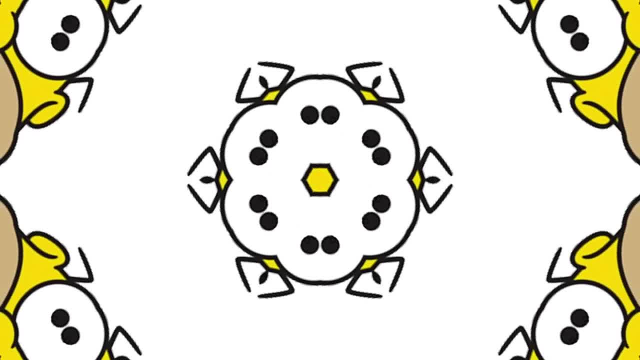 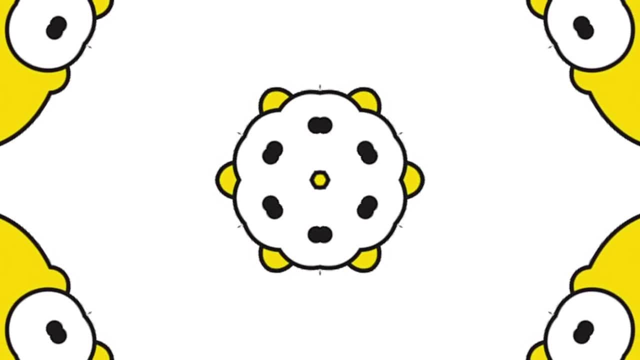 Occasionally- yeah, it does. I met somebody in the cafe the other day and said: oh, I'm teaching you today in our journalism class And it was very odd to think that your case is being discussed with journalists to help them understand the pitfalls of libel. 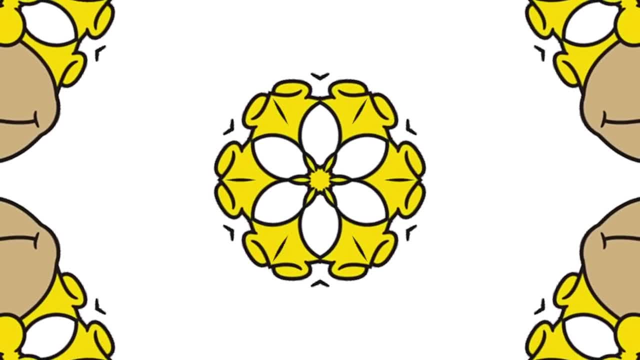 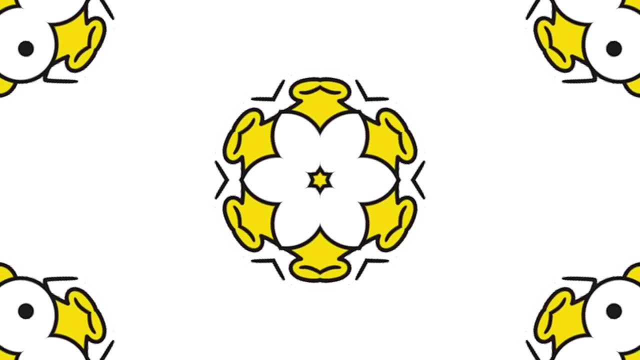 So that's great, I mean absolutely so exciting to know that that legacy is there. Yeah, Yeah, Yeah, Yeah, Yeah. That legacy is still there And that many others- I say Ben Goldacre in particular, and many others- fought for. 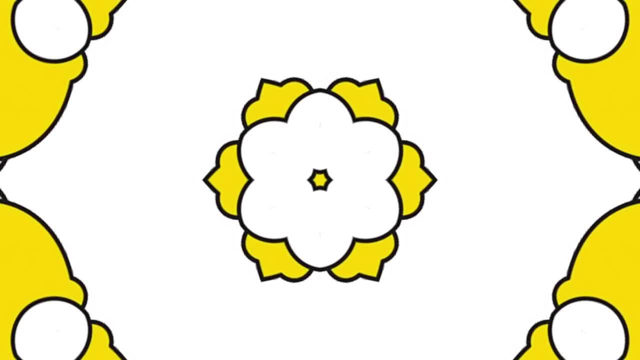 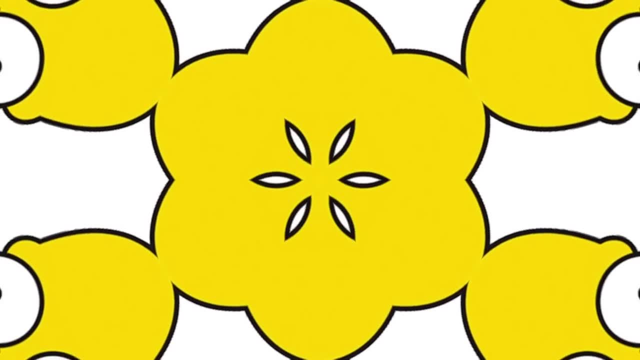 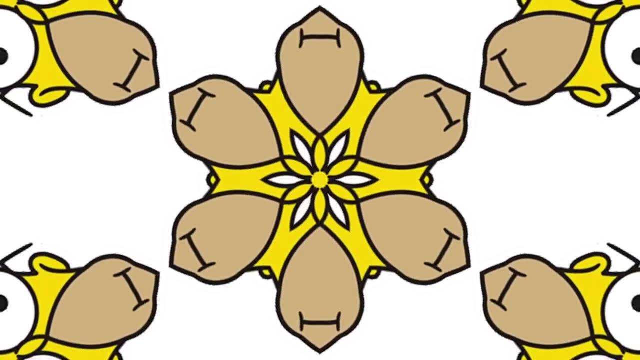 that change- But it also just goes back to my PhD- is utterly forgettable. Whatever was in there has been superseded within six months by many other people. So had I gone on and stayed in physics, I don't think I'd have done a great deal that. 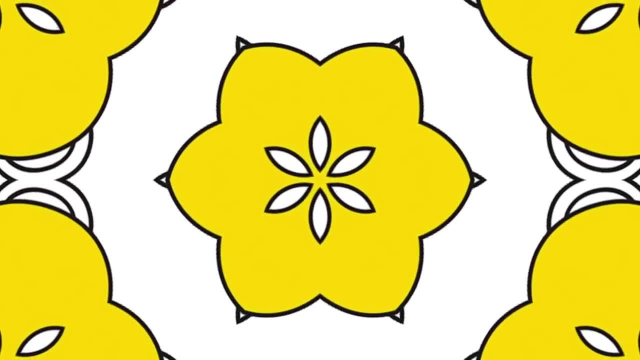 would have been very memorable But the libel law. I'm very proud of that and very proud that people still remember it and still teach it in lecture theatres. All it took was a couple of loose sentences in a Guardian article. They weren't loose. 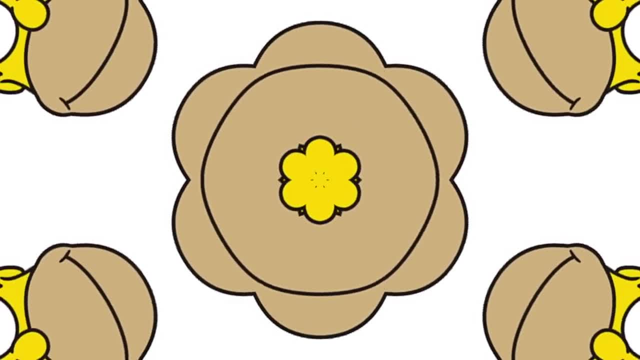 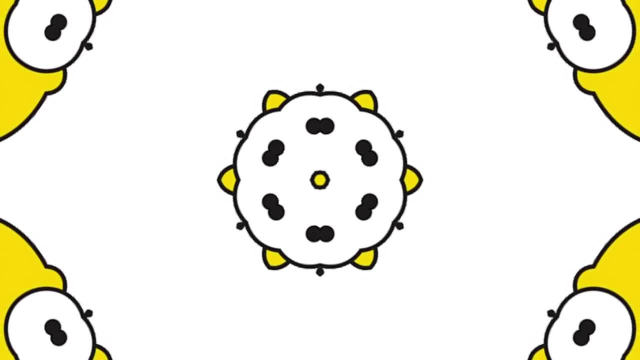 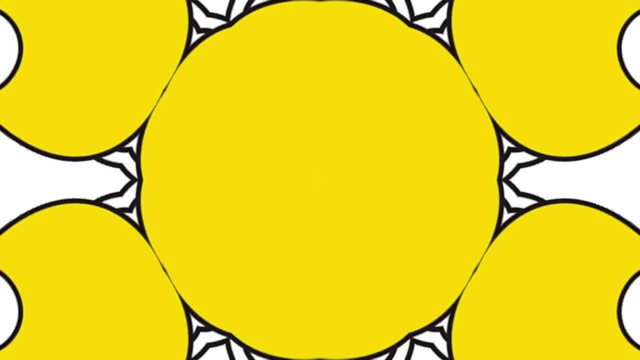 There was nothing wrong with those sentences. No, Obviously. the court decided So quickly on some of the books. then I will ask you a couple of quick things about books. One is: it seems like over the course of these five books, this is where you're turning from. 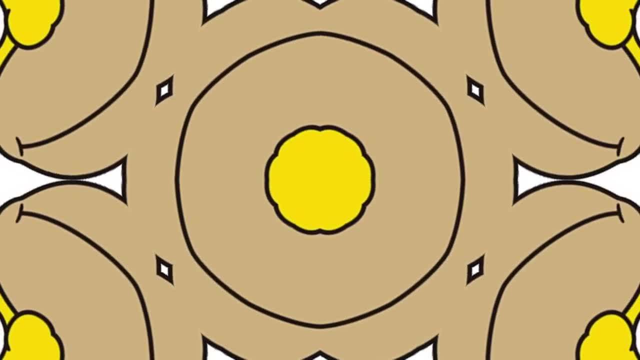 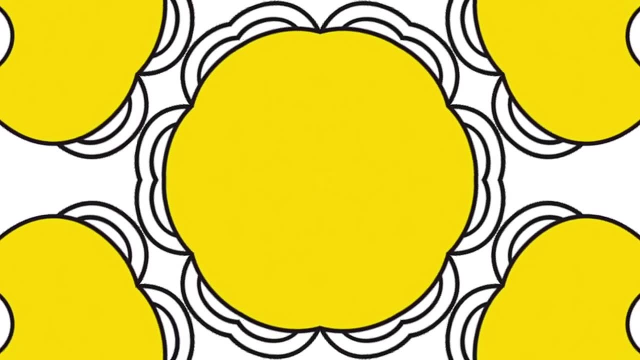 Simon Singh the physics guy into Simon Singh the math guy, Because you seem to start Like three of them I think are the same. Three of the five certainly I would describe as math books rather than science or physics books. 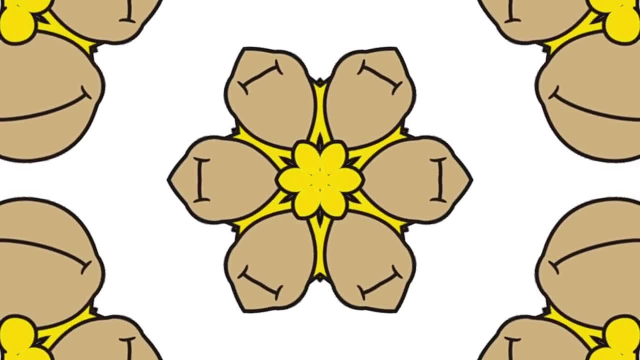 Yeah. So when I was on Tomorrow's World, you just look for any story. You look for any good story. I couldn't have had a career at the BBC just doing physics. I would have thought math would be the last place you'd look for those stories. 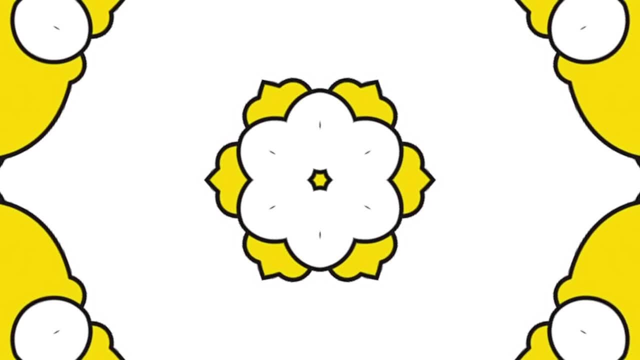 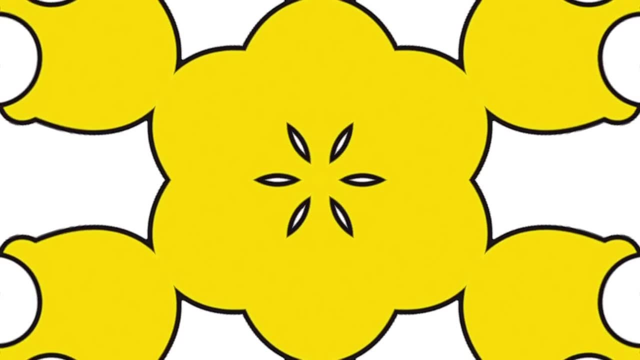 Well, Fermat's Last Theorem was there from the get go. That was the first story, So you have a maths head start. when your first book is Fermat's Last Theorem, Then the code book is a maths book. I agree. 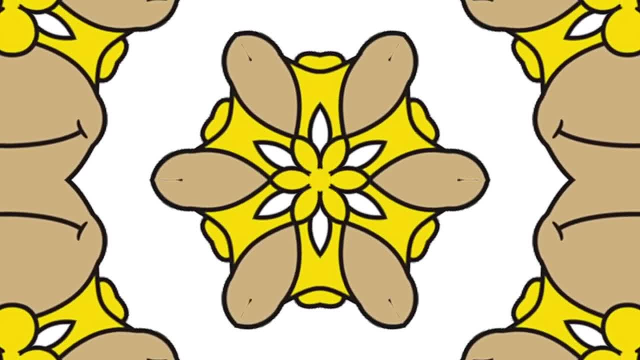 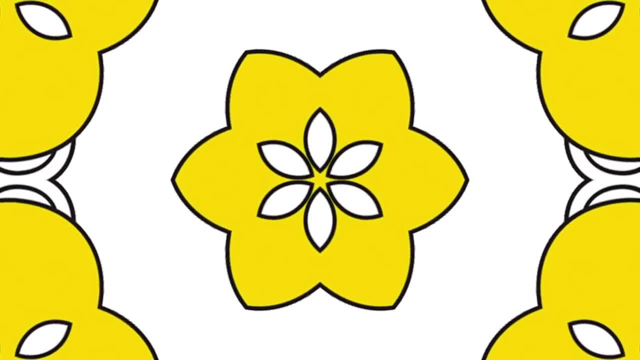 But it's also a book about history. But it's also a book about history and technology and many other things and linguistics and so on. So it's not a physics book, I agree, but it's only a little bit of a maths book. 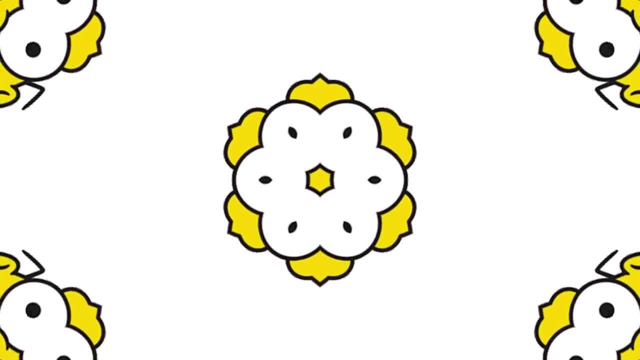 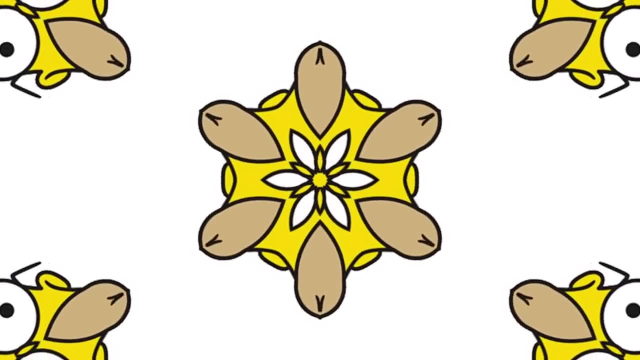 A big bang is physics through and through trickle treatments, completely outside of my area of expertise and could only have written that book if I hadn't coauthored it with Edzard Ernst And then the symptoms book. I was absolutely probably deliberately avoiding writing any. maths books. So the Riemann hypothesis, the Poincare conjecture: People send you ideas for maths books all the time. It was just deliberately not going to write about any of those things, But the Simpsons maths book was just irresistible. 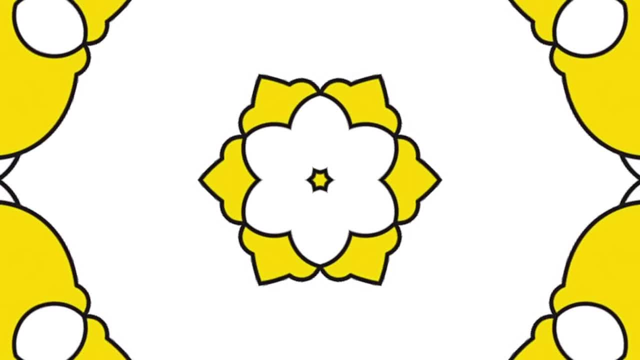 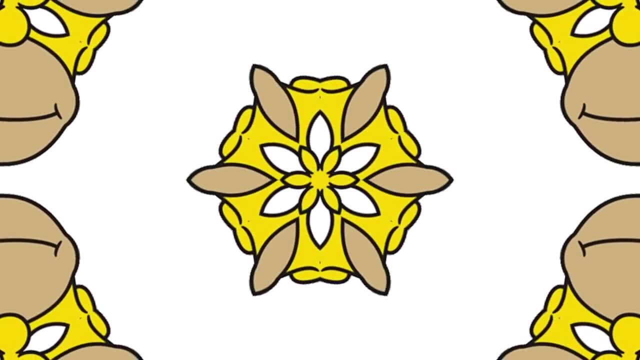 The Simpsons maths book seems like the odd man out in that collection to me, though It seems more frivolous than the other ones. It is, It is, And I think when I started writing it I wrote it in a different way. I had six big chapters, because all of my books kind of have six or seven big chapters. 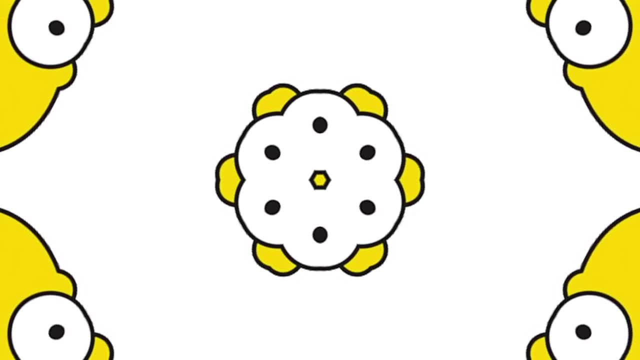 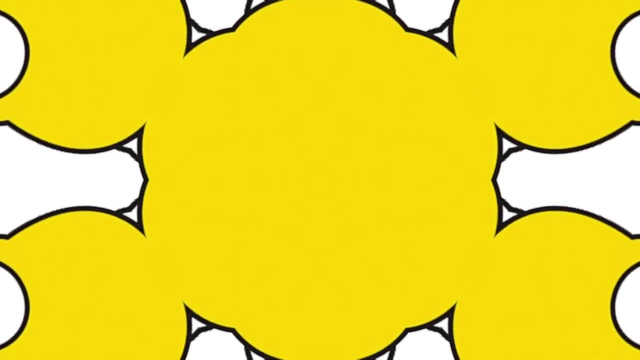 When I was flying over to meet the writers for the first time. for the first time I rewrote the whole book between London and Los Angeles and I smashed it up into 17 little chapters. So each little chapter is just: you kind of come in, you learn a bit of maths, you learn. 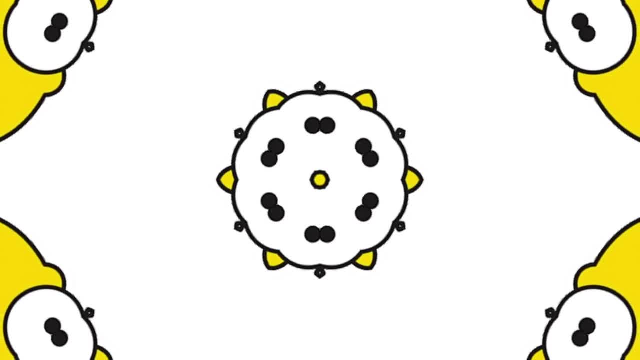 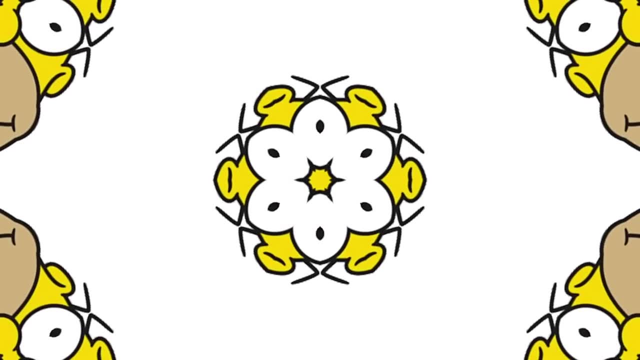 about that Simpsons episode. The maths begins to get a bit difficult and bang, we're out into a new chapter, a new idea, a new writer and so on. So it's a much more bite-sized book, Yeah, And the flow of it and the pace of it and the lightness of it is more akin to the Simpsons. 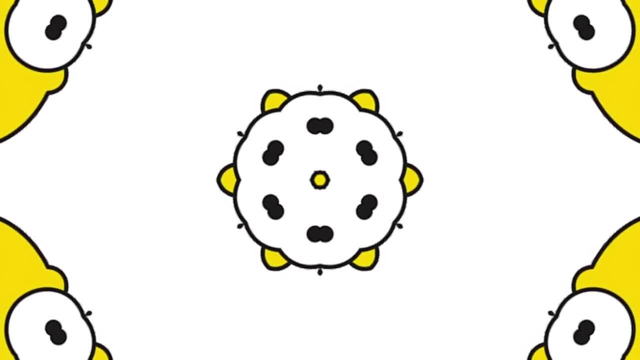 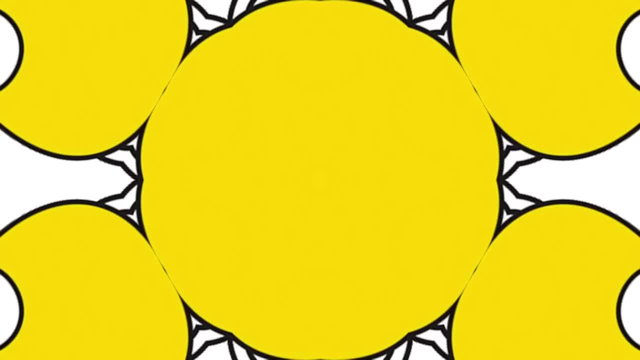 of Futurama. So it is different in that respect, absolutely. But I would also just say the maths in it is. in Fermat's Last Theorem we talk about infinity, but in the Simpsons Futurama maths book we talk about uncountable infinity and 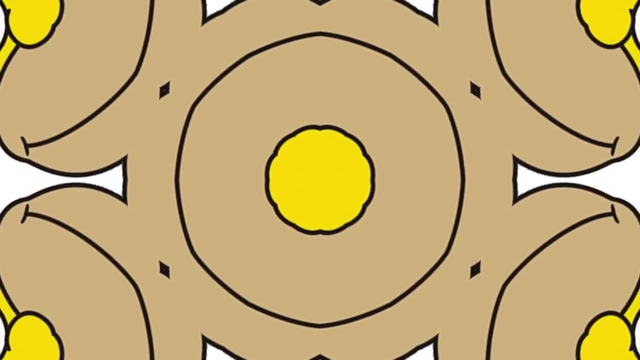 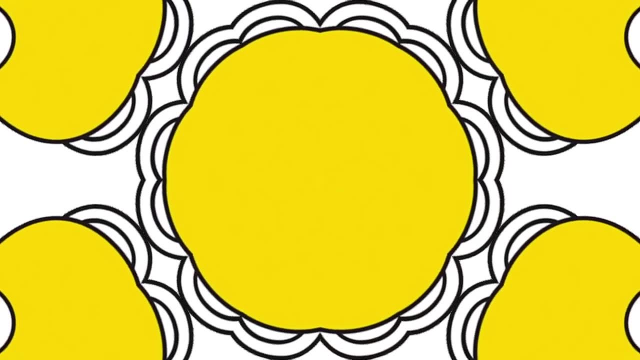 different scales of infinity. So there is some pretty heavy maths in there as well. It's not a trivial maths book, but it's a little bit lighter. What are you doing at the moment? How do we even start with what You've left books behind? 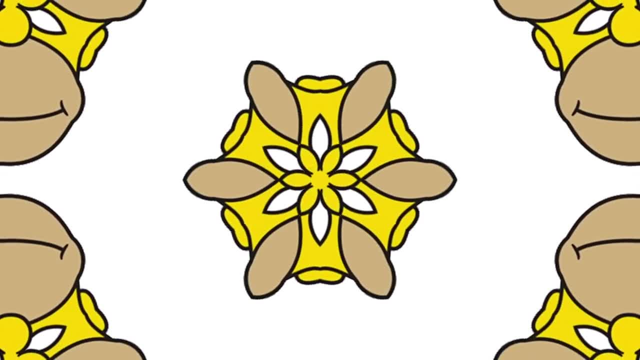 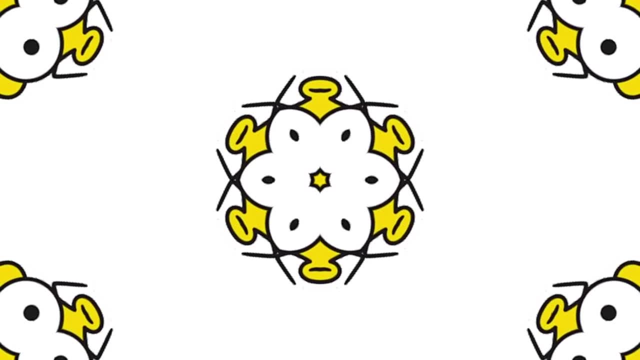 I actually was secretly hoping you were going to reveal to me today the new book you're working on, but you've left books behind. That's it? I'm not sure One. I don't have any ideas. I have not had an idea for a book since 2006.. 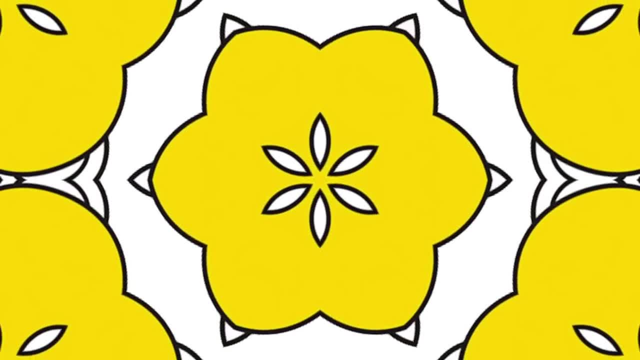 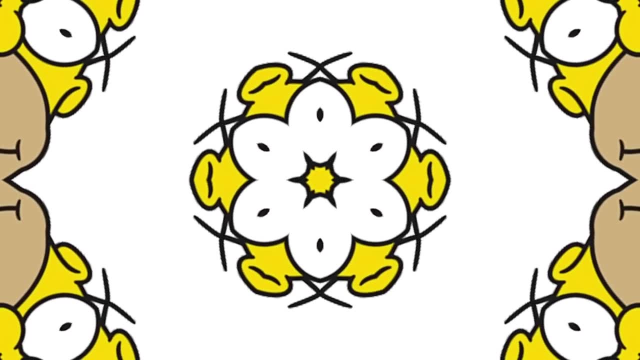 I've not had an idea for a book for 12 years. Is that true, I would have thought. aren't you someone who just walks down the high street and everywhere you look you see a book idea. Is a book idea that different to another idea? 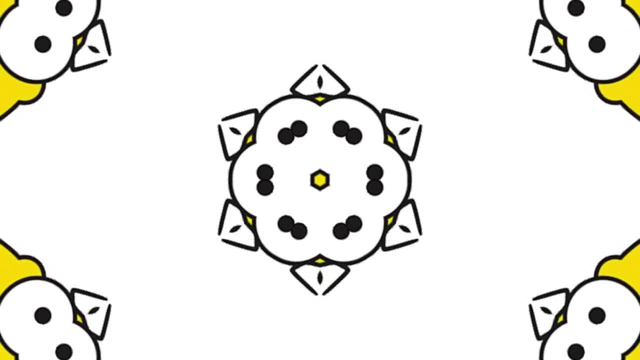 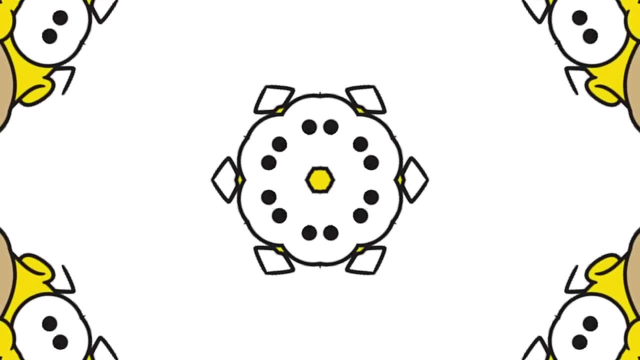 So The Simpsons is the most recent book, But I had the idea a long, long time ago. The last book I had was for Trick or Treatment. That came out in 2008.. So I would have had the idea in 2006,, 2007.. 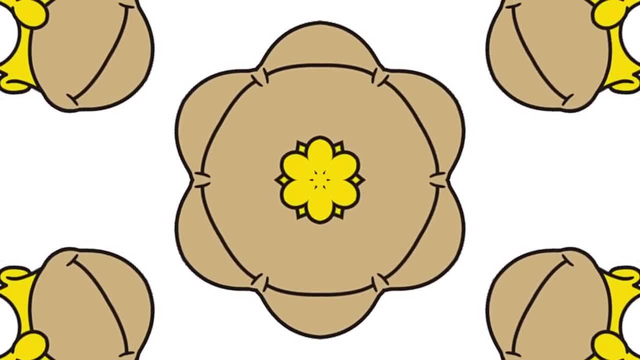 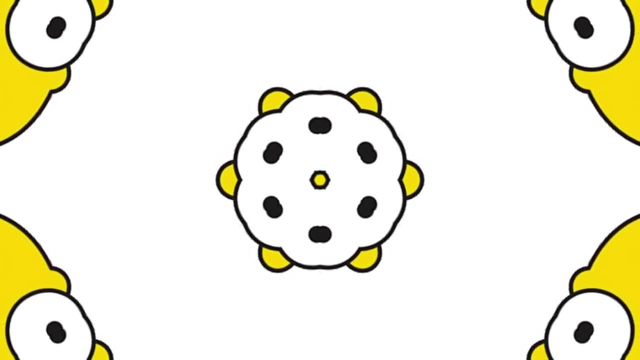 So I haven't had a new idea for a book for 10,, 11,, 12 years. So if I had an idea I might write a book. I probably wouldn't because I'm not sure that I'm ready at the moment to spend two or three. 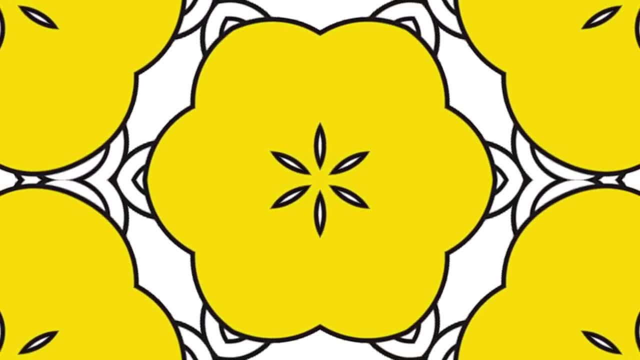 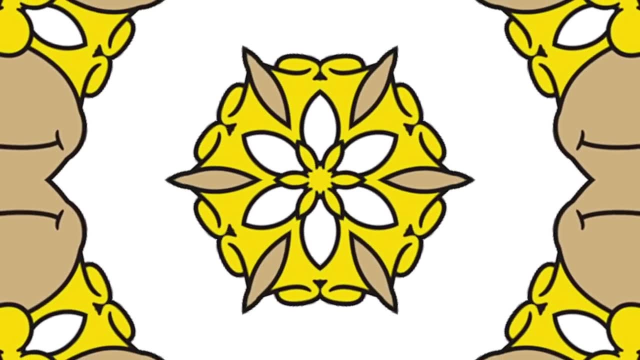 years working on a book that people may not necessarily read. I think the book market is receding. There are amazing things on the internet. There are amazing, Yeah. Long form articles, clever blogs, short blogs, podcasts, funny videos, interesting videos. 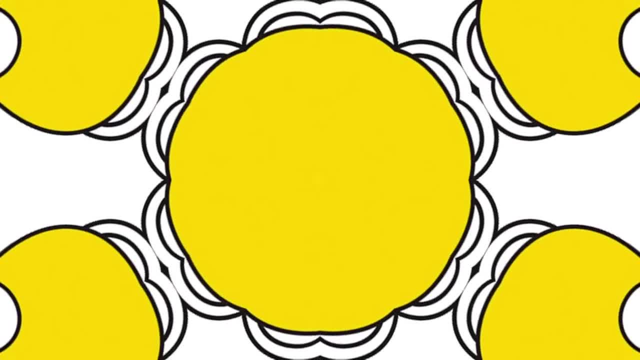 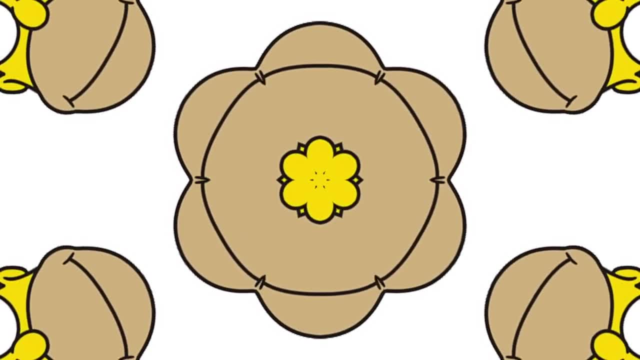 challenging videos. I have no problem with people reading fewer maths books, as long as they're getting their maths in many, many other ways, And I think that's just as enriching. The number five videos you make are every bit as informative and entertaining as any. 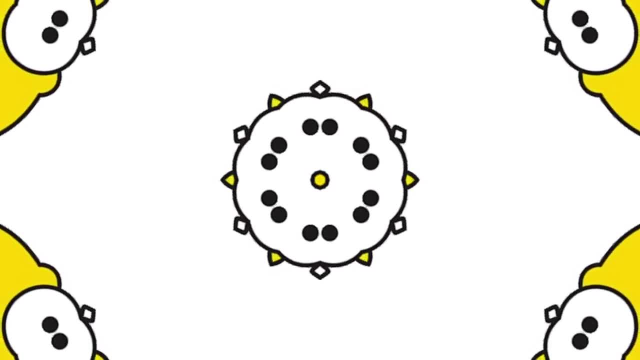 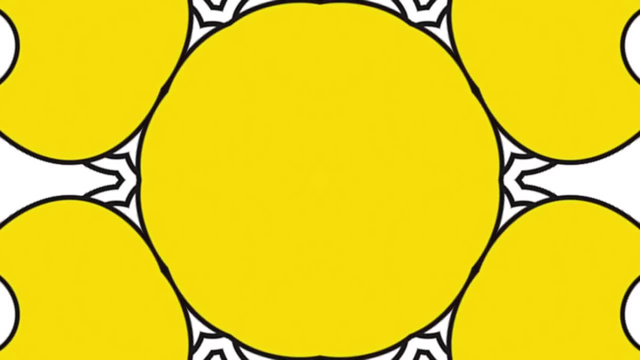 other chapter from any other book. So I have no problem with the book market declining, but it just means it's not what I'm then going to do next, especially if I don't have any ideas Instead, what I'm really, really interested in is education, maths education in particular. 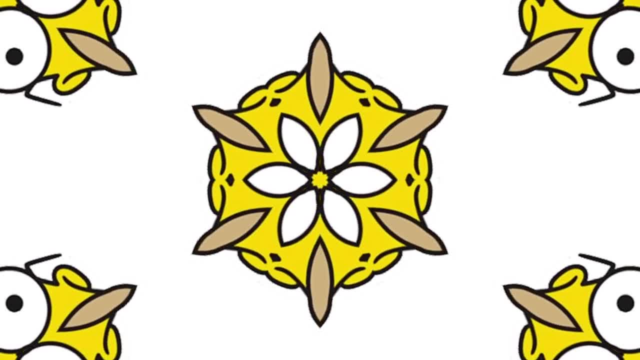 Because I think if you don't get the maths right, you can't do the physics, you can't do the engineering, you can't do any of those other great things. So your interest in the math education that we're about to talk about now doesn't mean. 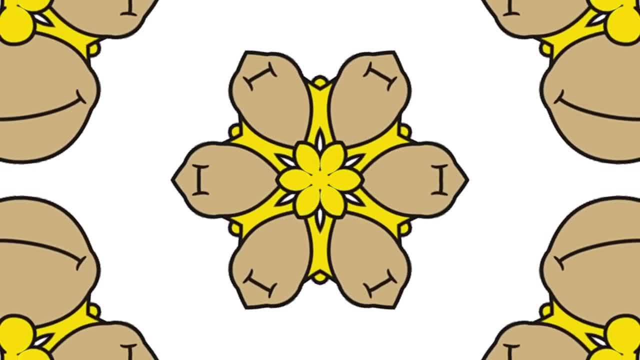 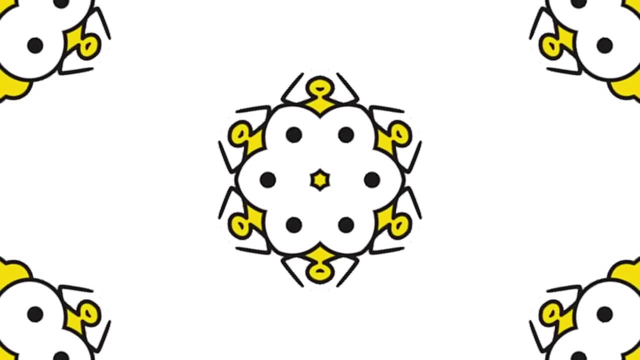 you've like turned your back on physics. it's almost to help the physics. Oh yeah, absolutely. I mean, I think physics A level is not really a good preparation for doing physics at university And that's because they've taken the maths out of it. 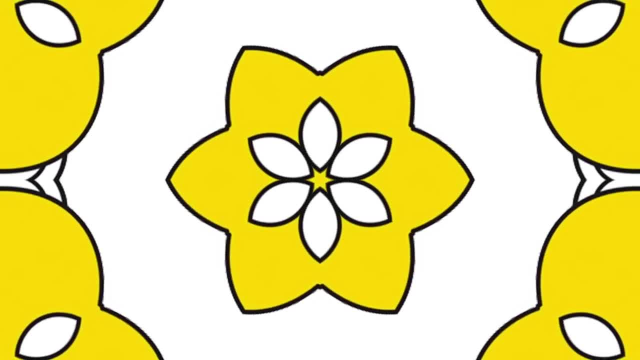 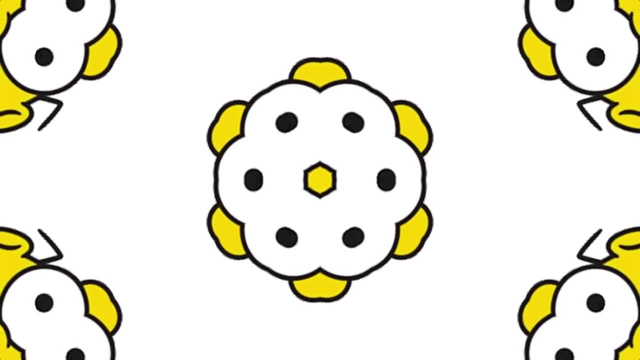 That's why I'm interested in maths. There are many areas that people could look at in terms of math education. You've got kids who are struggling with their basic numeracy. You've got other kids who are okay but who could do much better. 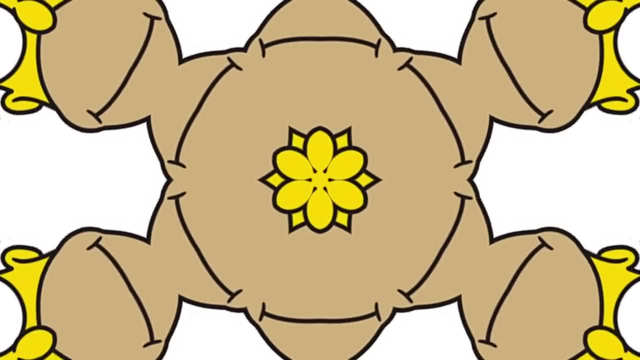 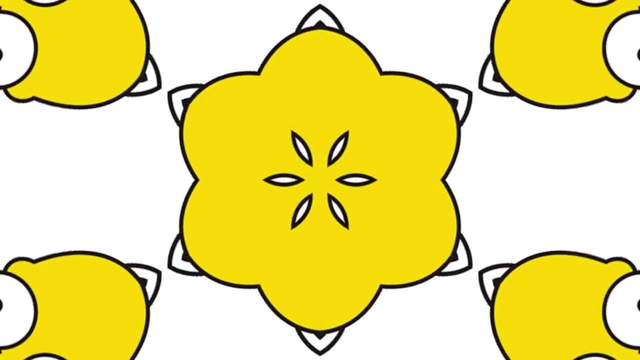 There are many different areas and age groups and people you could focus on. The one that I think gets ignored and the one that I'm really passionate about are kids who are good at maths but who never become excellent. I think in the non-selective state school system, it's almost impossible to become excellent. 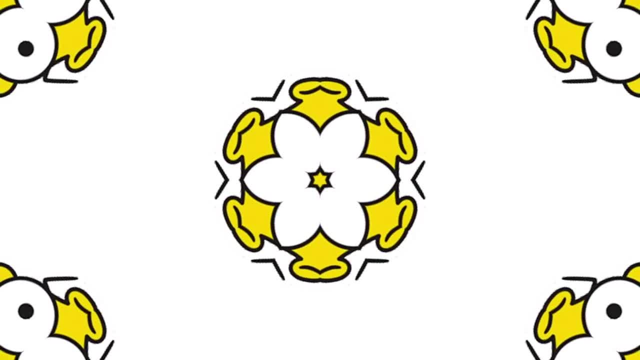 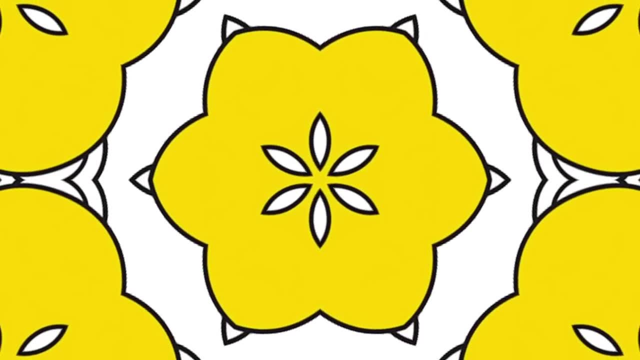 at maths. Yeah, Because GCSE maths is kind of a walk in the park: If you're great at maths, if you're not good it's a bit of a struggle, And if you've got your grade nine you've really earned it. 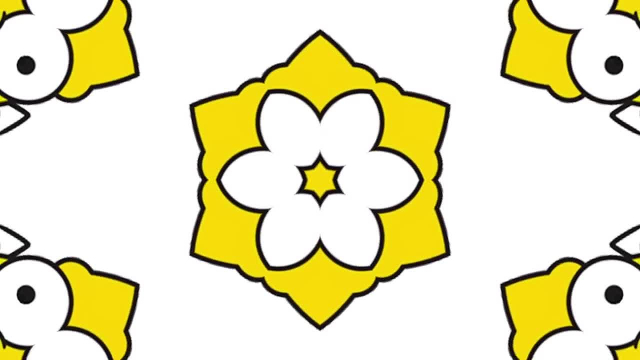 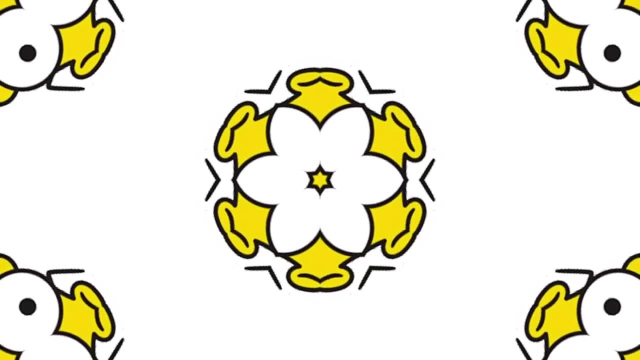 But if you're good at maths, grade nine is not so hard, And so we need to get these kids, preferably when they're quite young, and if they've mastered everything at primary, we need to stretch them and stretch them and show them interesting. 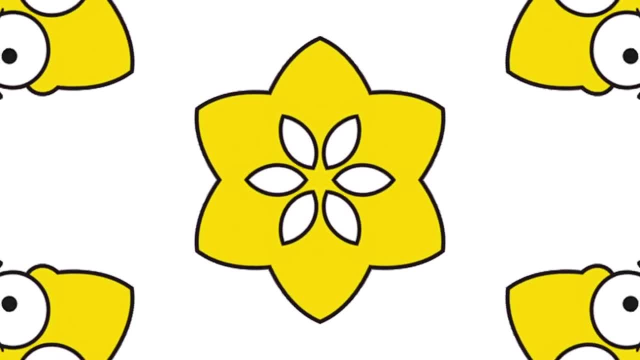 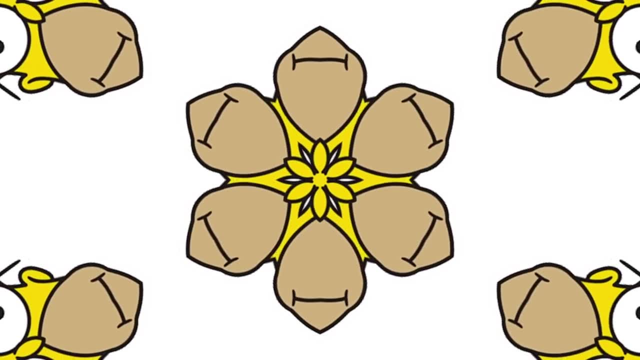 fascinating maths and prepare them for what they could do later in life. So I've been interested in how do you do that. How do you in a non-selective state school environment? how do you encourage good students to become excellent? And I'm only interested in ideas that are cost effective and scalable. 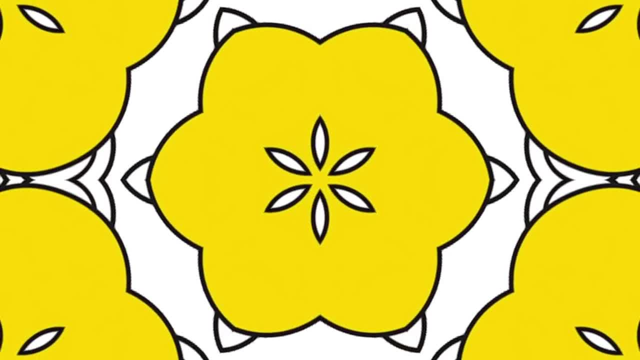 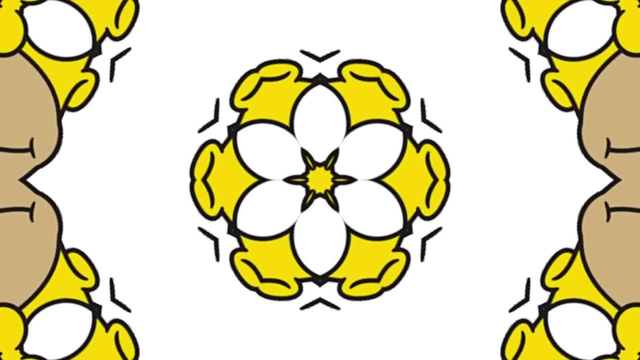 There's no point taking- I don't think there's much point taking- kids away for a week long gifted and talented summer school when in September they'll go back to their old classroom and the mundanity of their classroom- maths- is there for the rest of the year. 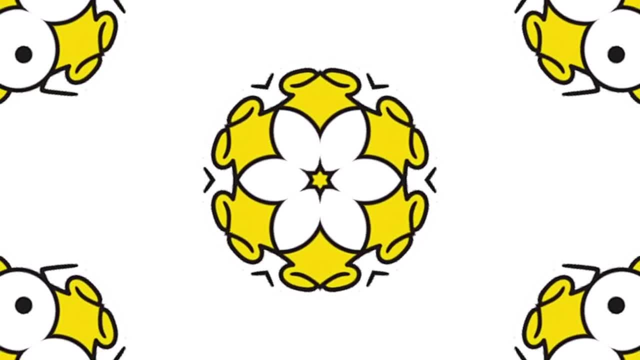 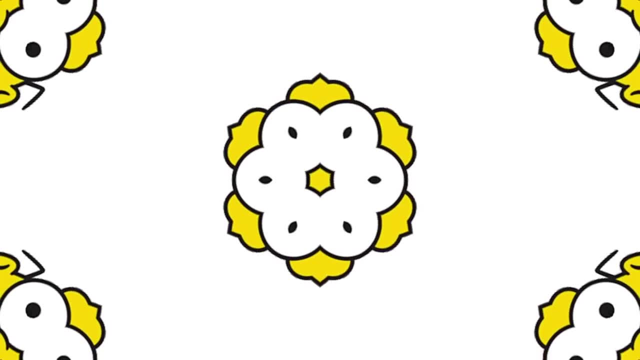 So I'm interested in something that happens day after day after day within a school environment, And so the idea that I've developed is something called top, top-sec, Top-sec maths. Okay, Horrible name, but just bear with it. 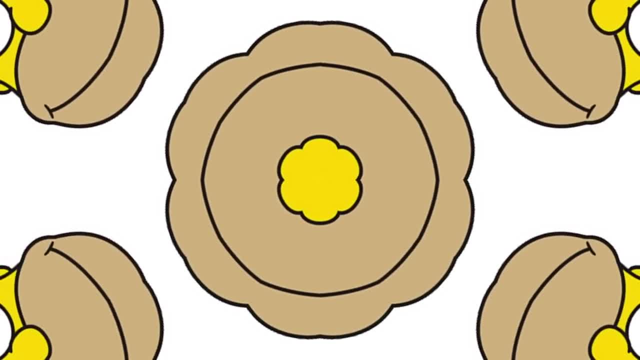 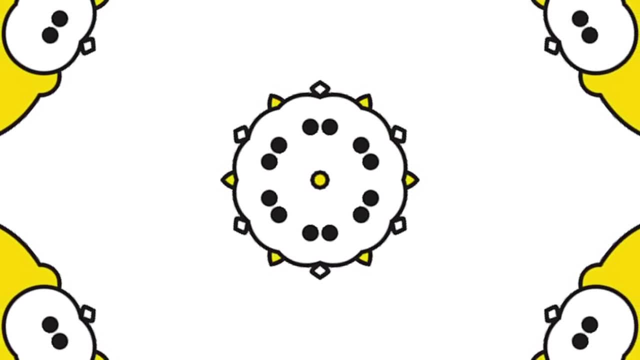 Top top-sec maths Okay, And the argument I've got there is that if you're in a top-sec in maths, you're in the top 25%. The ability range in the top 25% is very broad. If you take 25% of the population, they are not all good good mathematicians. 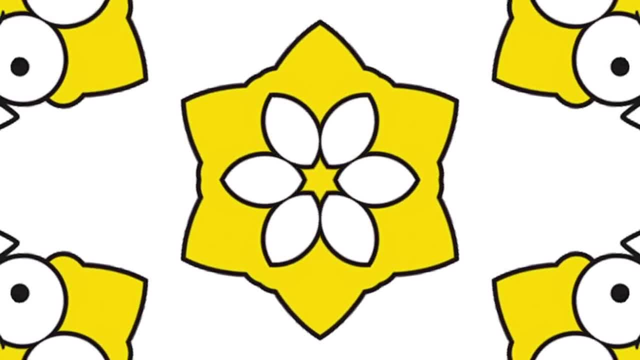 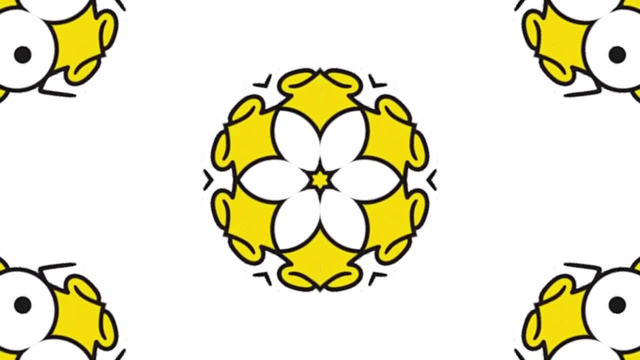 Some of them are a bit better than average. Some of them are brilliant And you tend to have to go at the pace of the weaker students in that top-sec. So the good top-sec students just twiddle their thumbs, So they're still being held back, even though they're supposed to be in the elite group. 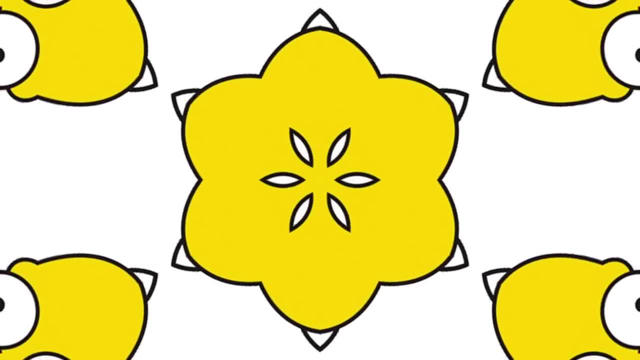 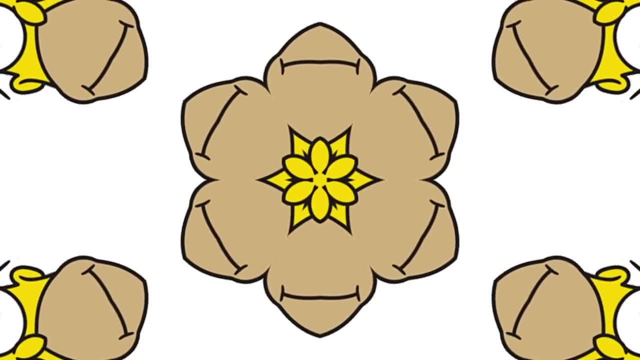 In the top-sec Exactly, And schools often have two top-secs. The schools are very large, so you'll have two top-secs. So I'm saying, refocus it so you've got one top top-sec and then a second top-sec below. 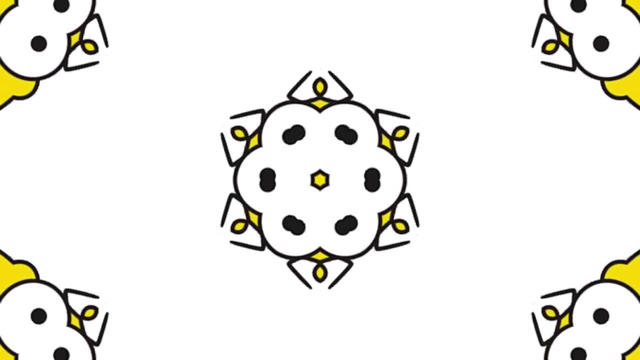 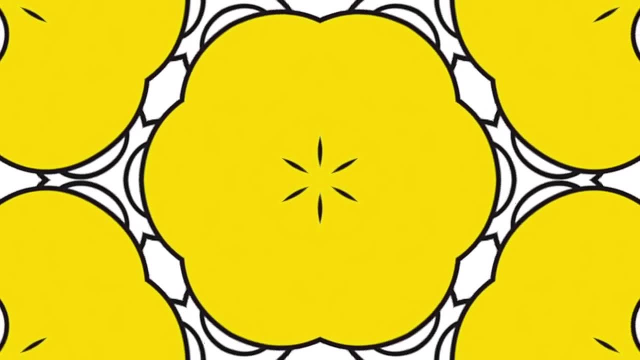 it. And then, with that cohort of students that are quite narrowly ranged in their ability but all confident and they've mastered primary school maths in year seven, when they're 11 or 12 years old, start pushing them up, Start pushing them along in this top, top-sec environment. 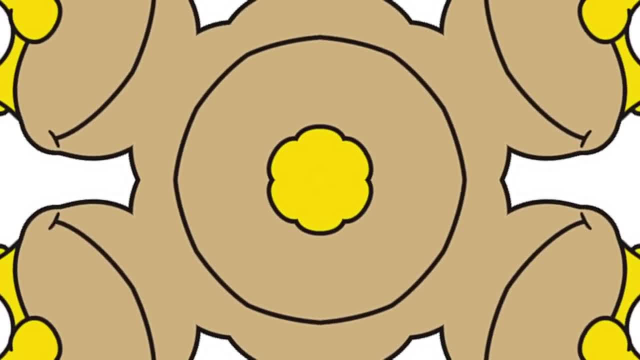 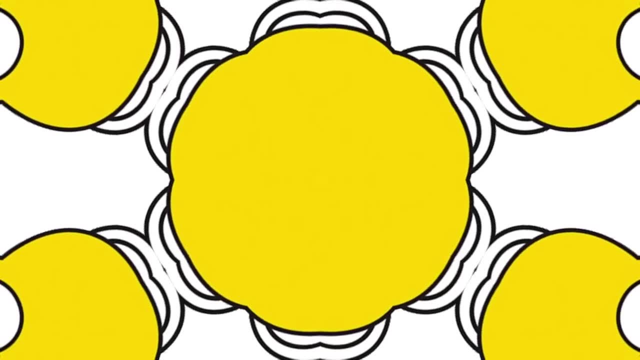 And keep that top, top-sec going right through to GCSE. So those kids don't just get a grade nine, they go beyond grade nine. Their maths is so, so strong at that stage And we're running it now in 13 schools. 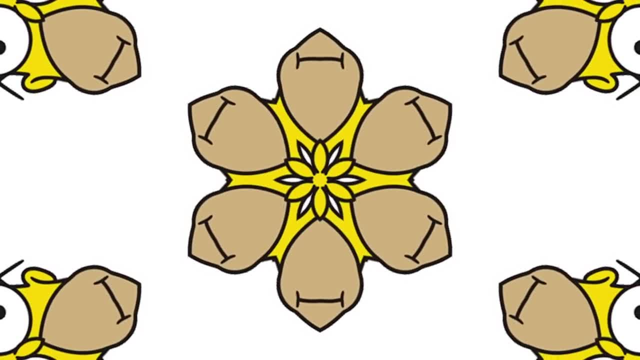 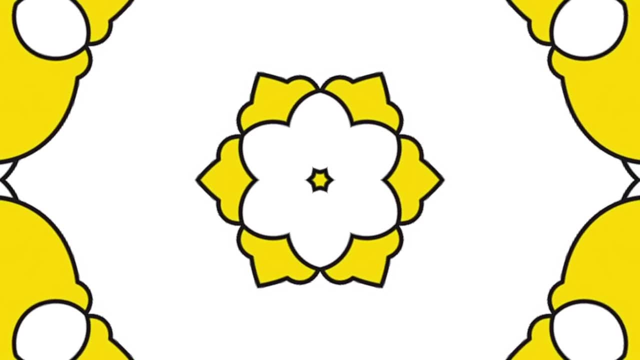 We've only got data from the previous two years when we only had about four schools, But the results, I think, are quite staggering. There's something called the Junior Math Challenge, which kids do when they're in year seven, year eight. 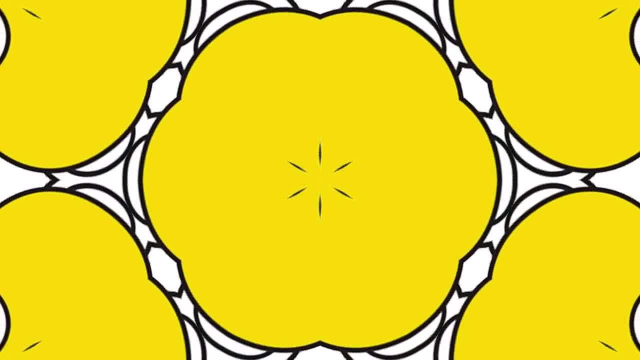 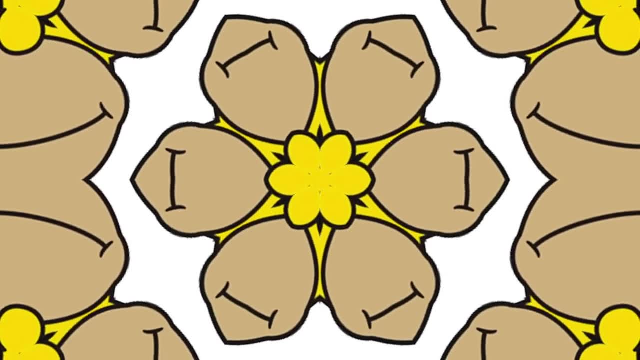 Our four schools doubled the number of certificates they're getting in the Junior Math Challenge, So that's a big difference. Yeah, So they're getting twice as many kids being excellent at maths, And so I think we're making a step change, And this year we'll have a lot more data. 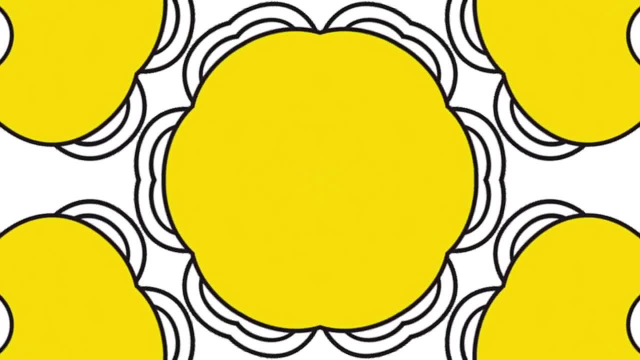 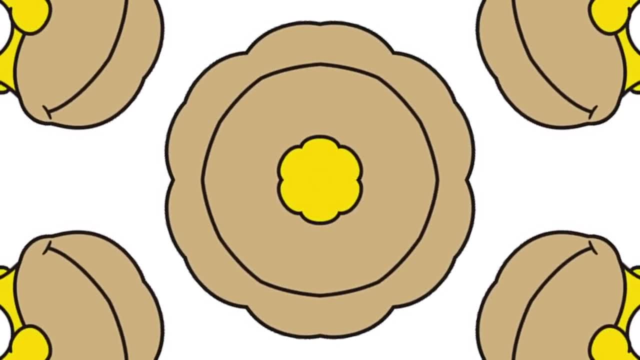 And then the next stage is to say, right, let's not just have it in 13 schools, Let's have it in 100 schools, or 500 schools, or 1,000 schools, So that, wherever you are in the country, if maths is your thing, you can get into a top. 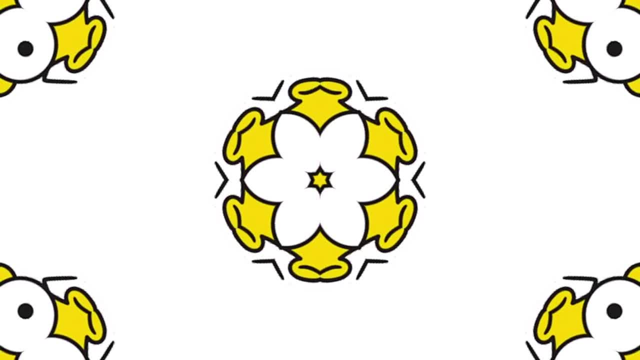 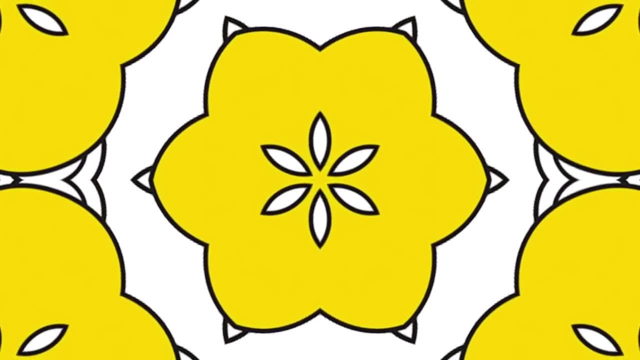 top set and you can continue to build on those skills. Isn't this just like just divvying up the cake even more, though Just more slices? It doesn't sound like a paradigm changing idea to say: let's break them up even more. 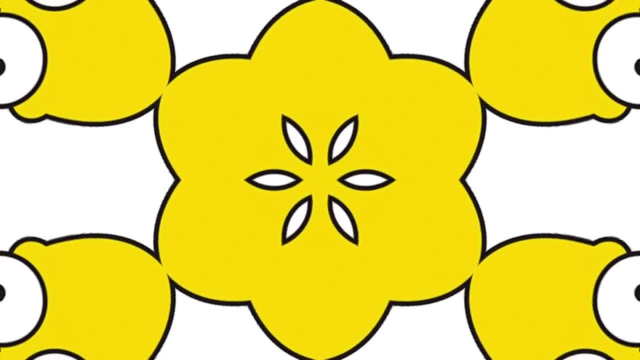 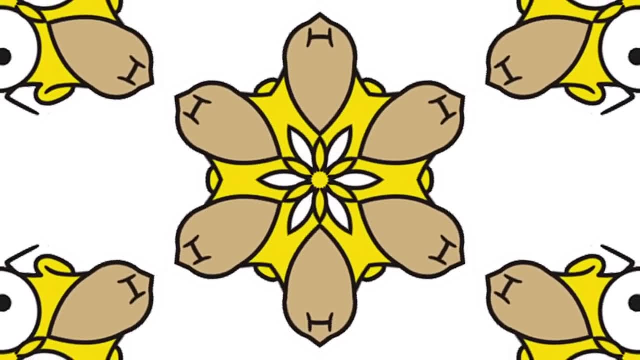 into more specialized groups. It's not a very radical idea, It's quite an old fashioned idea. It's not a new curriculum, It's not a new way of teaching maths, It's not math mastery, It's just saying, if kids are good, let's progress them really, really as far as they. 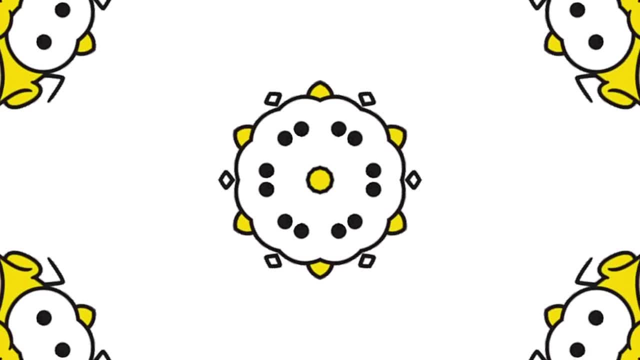 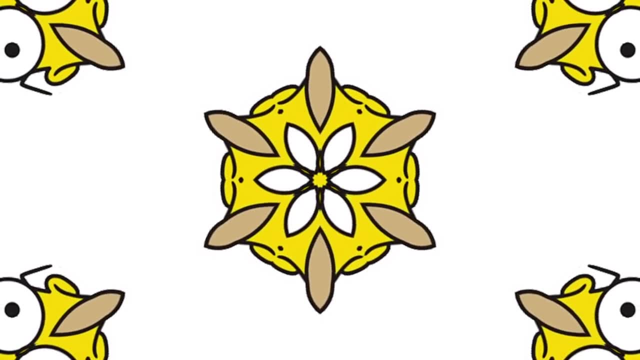 can go. Let's stretch them. Don't you need another class and another teacher? You were talking about cost effective, and isn't this just like creating more work at school? Oh yeah, You do need an extra class. You do need an additional set, effectively, and so you do need an extra person to be teaching. 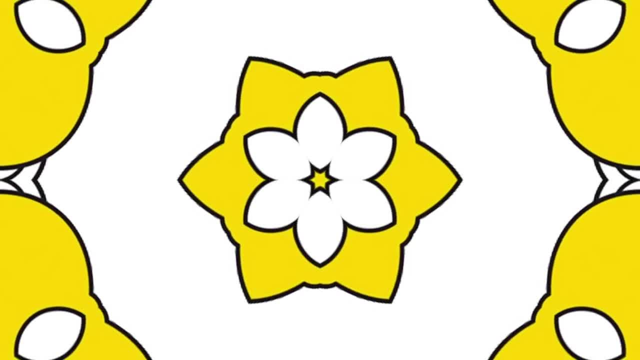 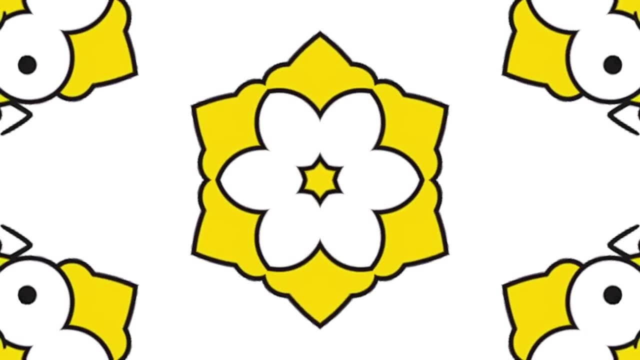 it as well. I still think, pound for pound, this is the best way to teach excellence. I've seen lots of other ideas over the years. I've spoken to 500, 600 school groups over the years. I've been to hundreds of schools. 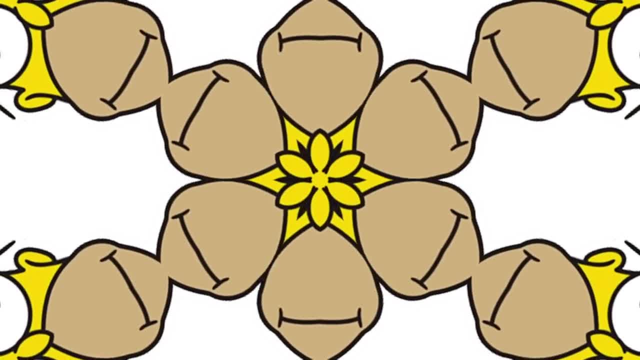 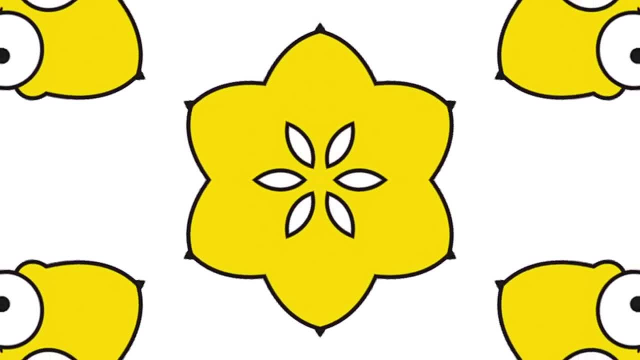 I've heard lots of ideas. This is the one where I'm seeing concrete results and, financially, if you want to make this change, this seems to be the best way to do it. but in a year from now, I'll have more data. 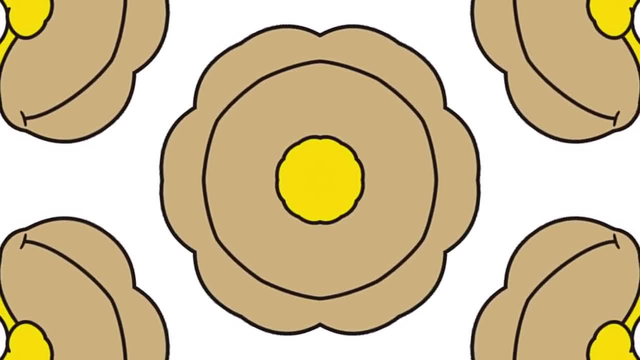 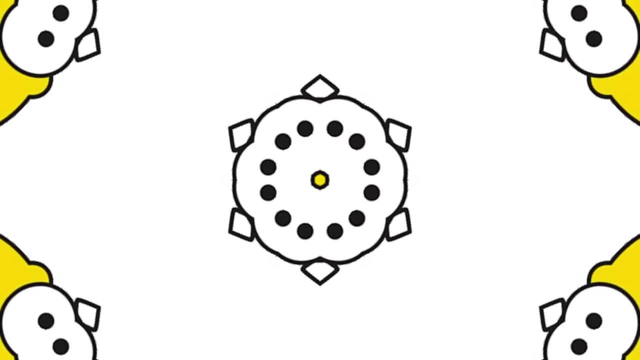 Maybe I'll be wrong, But at the moment it seems to be more effective. The other thing I would say is that it maybe sounds elitist- You're focusing on the good kids and so on- but what I'm seeing is that at the moment, 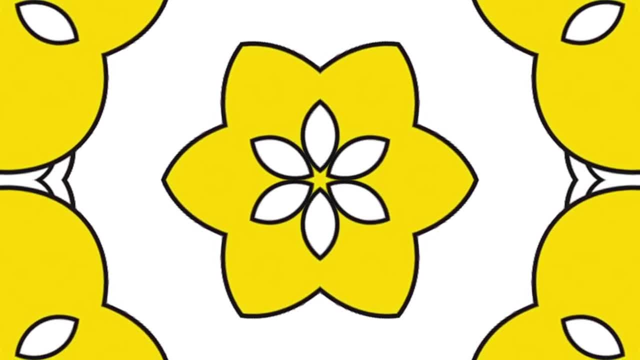 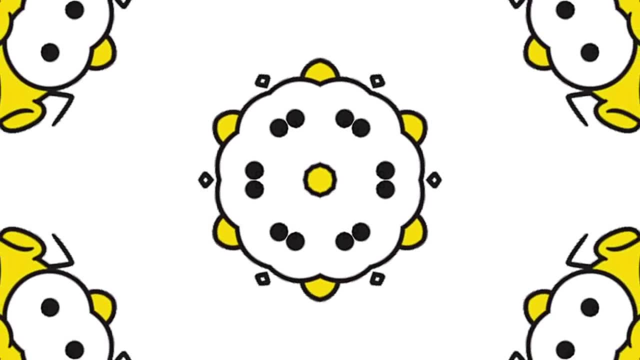 if you want to be excellent at maths, mum needs to be an engineer, or dad's a math teacher, or there's somebody there who mentors you along, because the schools struggle to do it. What I'm hoping is that this will allow far more children from a far wider range of backgrounds. 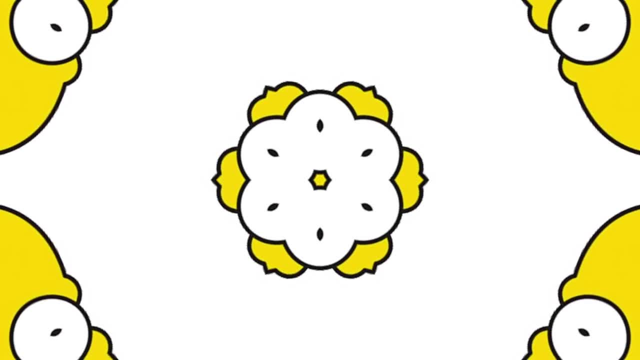 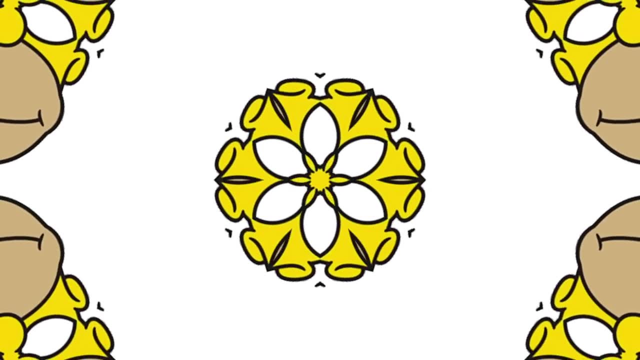 to become excellent at maths, You don't have to have had to go to a private school or had to go to a grammar school. It's less divisive than a grammar school. Everyone's in the same school. Kids can move into the top top set or out of the top top set. 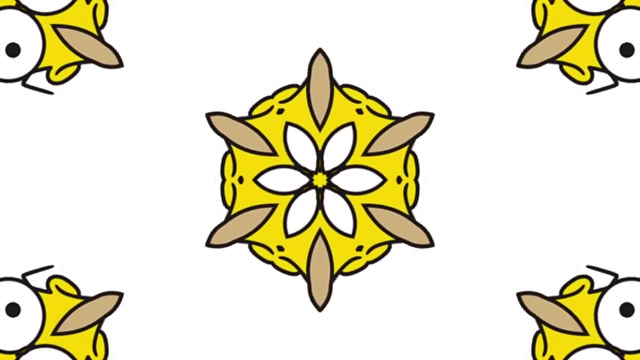 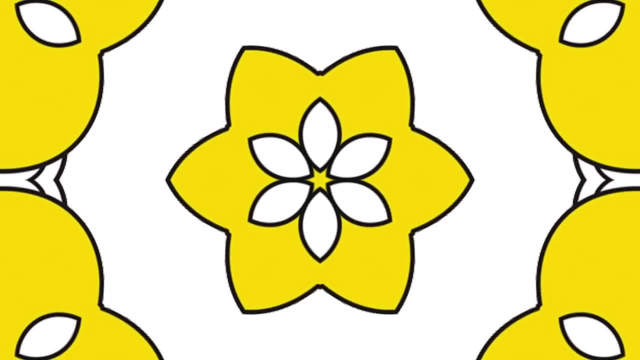 One of our schools is Plashett School in Newham. all-girls school from a huge variety of backgrounds, large Muslim community there. I remember sitting in the back of the class when the project started and these girls are all very bright. 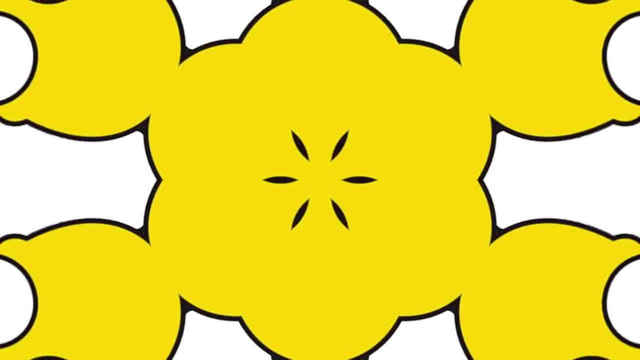 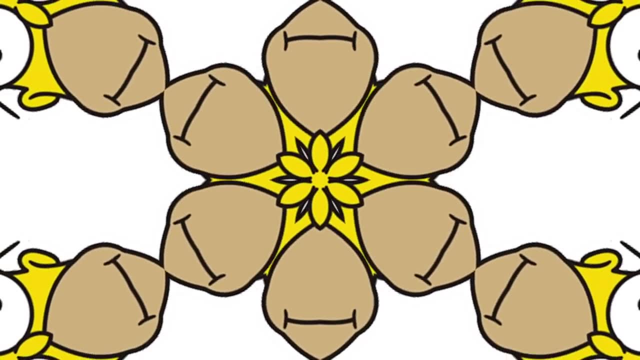 They're in the top top set already. If we did nothing at all, they would all go on and probably do maths A-level. But in our set I think they are going to go on and do maths A-level, Yeah, And do further maths and go beyond further maths and become computer scientists or they're. 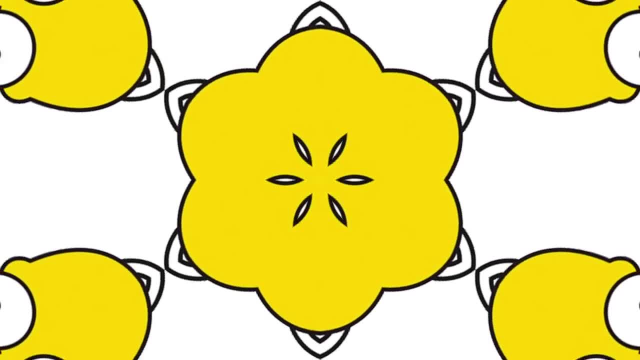 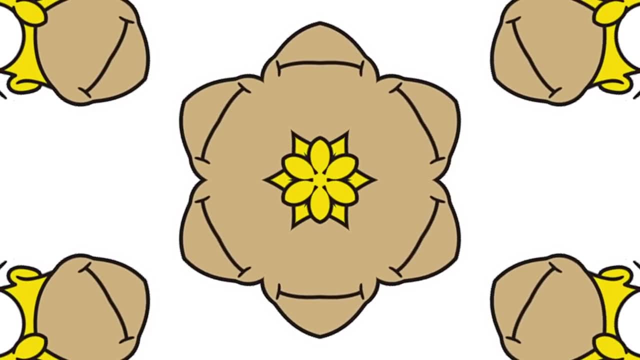 going to become aeronautical engineers or they're going to do something incredible. So I think we're giving those kids a huge opportunity to become brilliant at maths, which is otherwise very hard to achieve. You said you're piloting this in a number of schools at the moment. 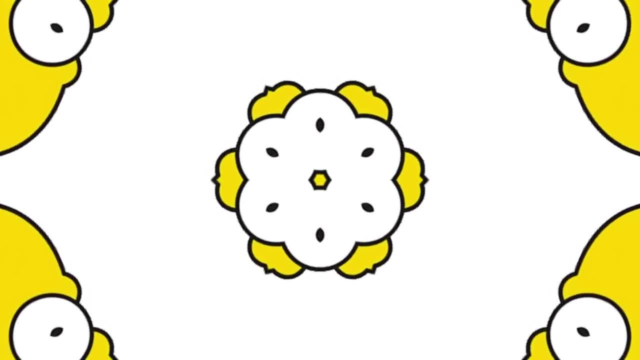 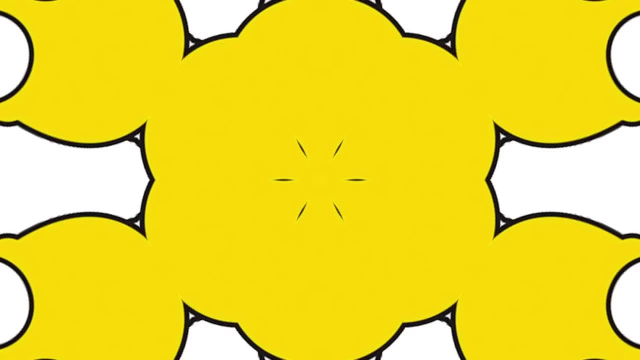 Does that mean you've brought money to the table for them to be able to do it? Yeah, So for the first year I said I'll pay for it because I don't want anybody else interfering with it. So, for example, somebody might say: well, we're going to fund this project. 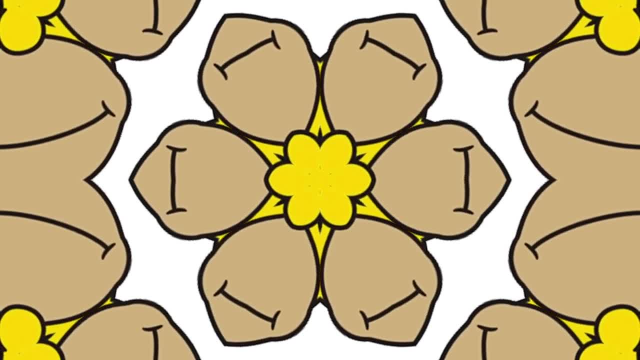 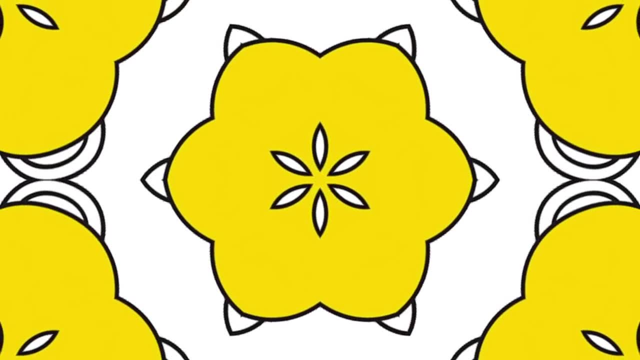 But only if it's developed in such a way that more girls do maths A-level. Now we're not going to get more girls doing maths A-level. As I was saying earlier, the girls that I was talking about are already going to do maths A-level, but they will do much, much better. 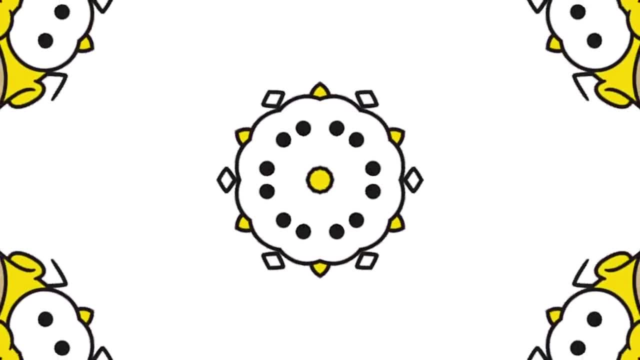 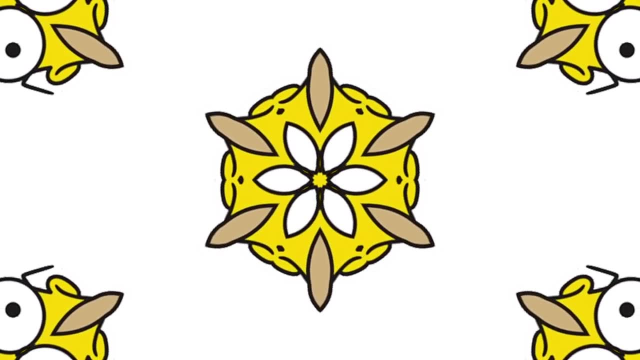 They will become incredible role models. So it's not about getting more girls to do maths A-level, It's about getting those that are doing it to excel even further. But I didn't want that tinkering or tweaking from other people. So the first year I funded it. the second year I funded it. 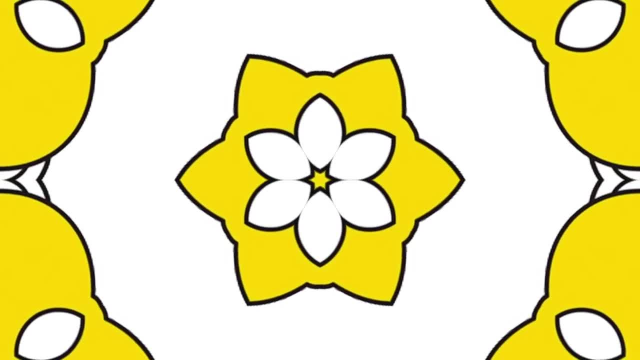 But, as you can imagine, the year seven has become year eight and there's a new year seven cohort. There's no money for that, But all four schools said we don't care, we're going to carry on doing it because we see the benefits. 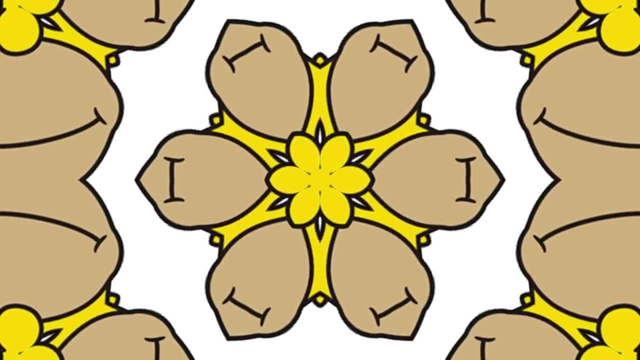 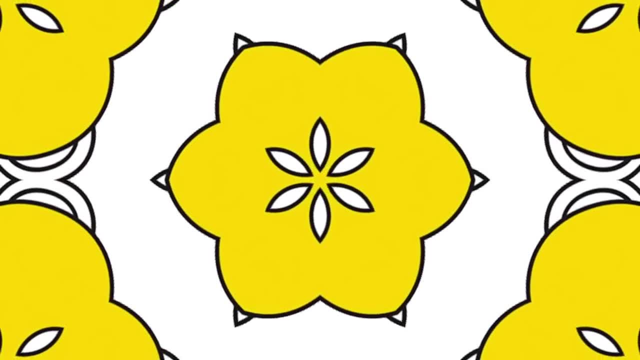 In the third year I'm still putting in some money. but I'm also getting funding from John Lyons Charity, which is kind of the philanthropic arm of Harrow School. They've been tremendously supportive. Emmanuel College, Cambridge have put in some money. 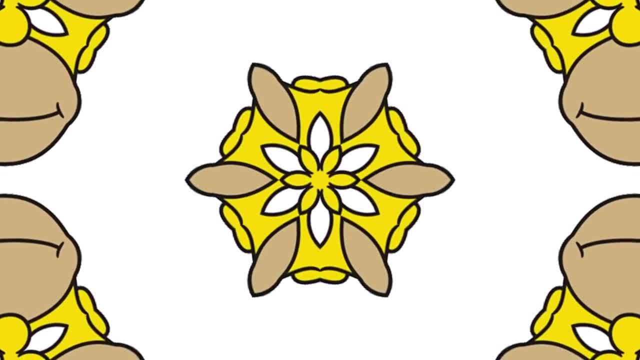 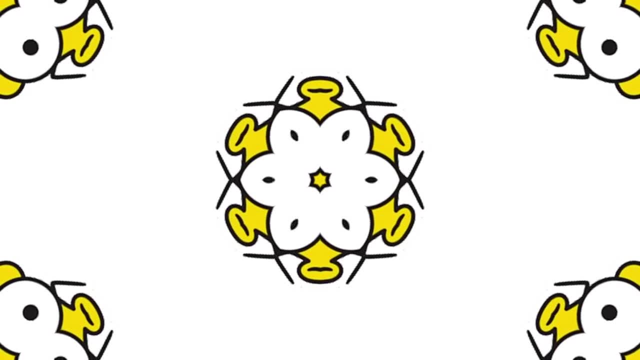 The London Mathematical Society have been fantastic, And the Winton Foundation as well. Winton Philanthropy have also been very supportive, So we're beginning to having shown the proof of concept. I can then go out and say we need some money to support this. 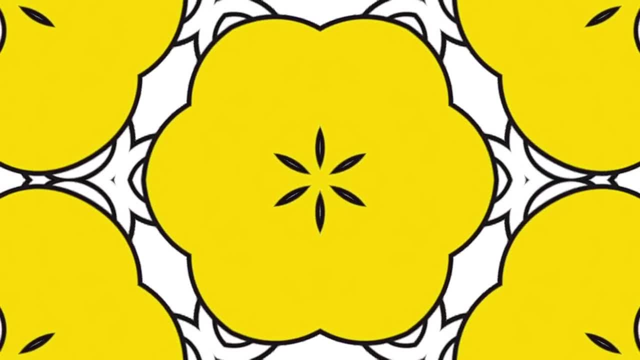 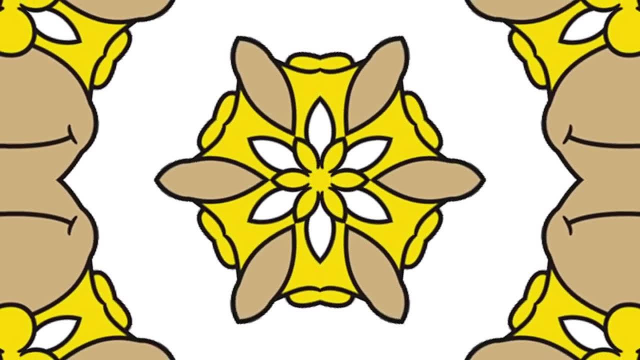 And people have come forward and that's been great. The next step is to get the data show that it works or not. If it does work, get bigger money in and expand it across the country. I mean, it sounds like if your dream was to come true and this was to become standard. 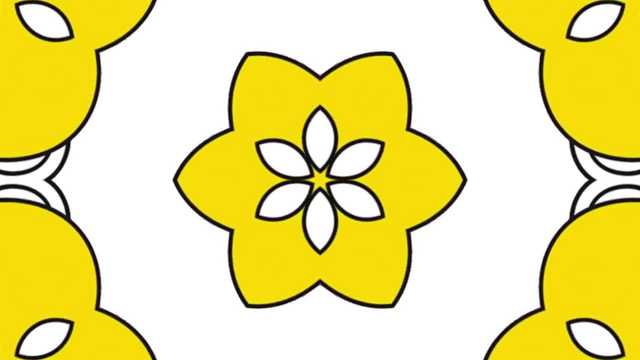 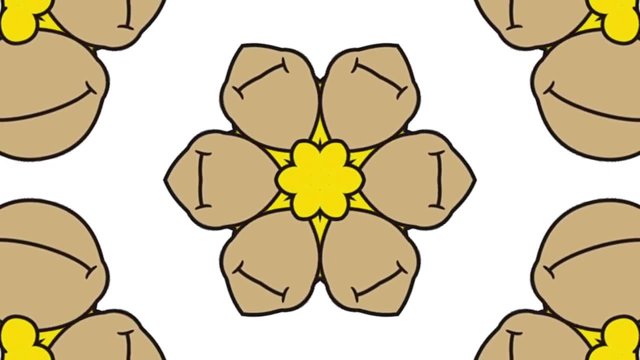 across the country. it'd be enormously expensive, though, to be a whole new bunch of maths classes. The cost would be about 5 million a year. 5 to 10 million a year. What for the whole country? Yeah, Okay. 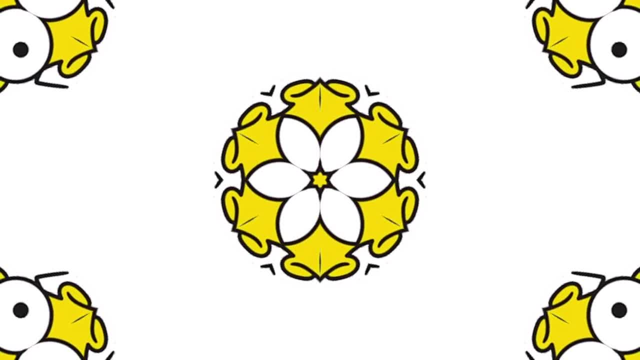 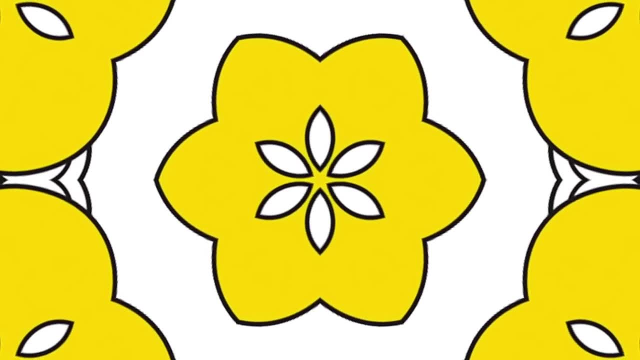 That's a lot of money. On the national education scale of things, it doesn't seem like much. Yeah, You've worked it out more quickly than me. So yeah, you're absolutely right, It's one teacher per school because you've got a top top set in year seven, year eight. year nine, year 10 and 11.. That's five classes. One teacher could teach all those classes. In practice you wouldn't. you'd share it around a bit, but you need one extra math teacher per school. Now, math teachers are like gold dust. 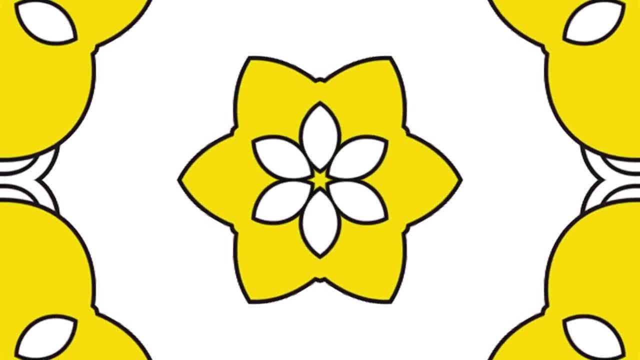 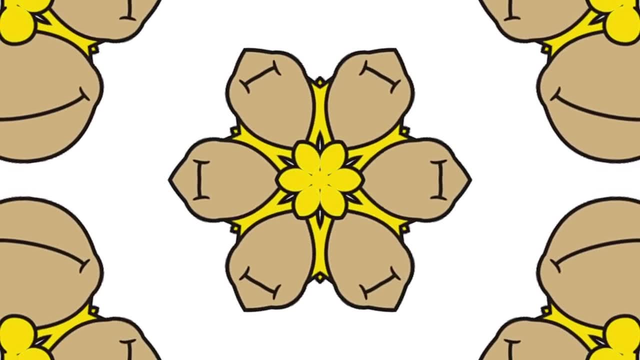 So that could be a limiting factor on how it grows. But if I was retiring as a math teacher I'd be quite happy to come in part-time and teach one of these groups. If I was a school that ran a top top set math project, I think I find it easy to recruit. 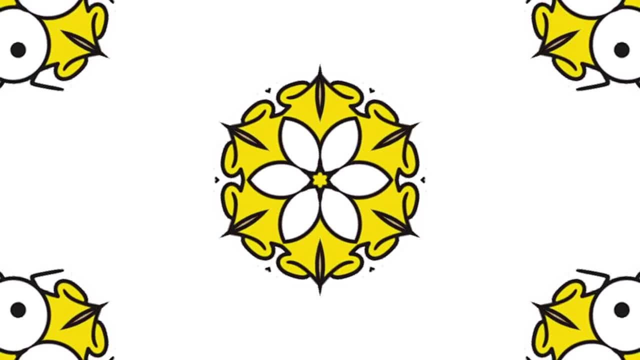 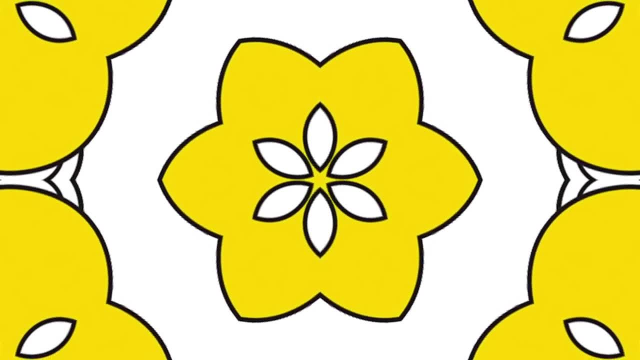 math teachers to my school. So I think there are ways of making it work, And if teachers are the limit, then we'll find out soon enough, But at the moment I think we should definitely have 100,, 200, 300. 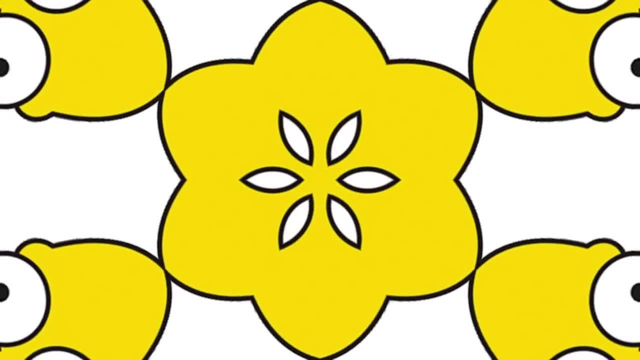 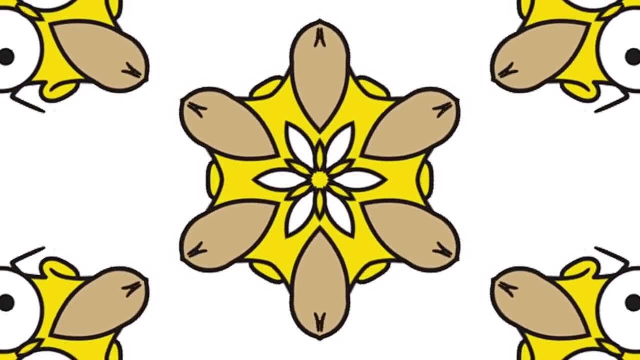 And then that means that's 1,000, 1,500 extra very strong mathematically minded people coming through the system every year. I know you travel around, Simon, and sort of evangelize for this idea, And I've seen you talk about it. 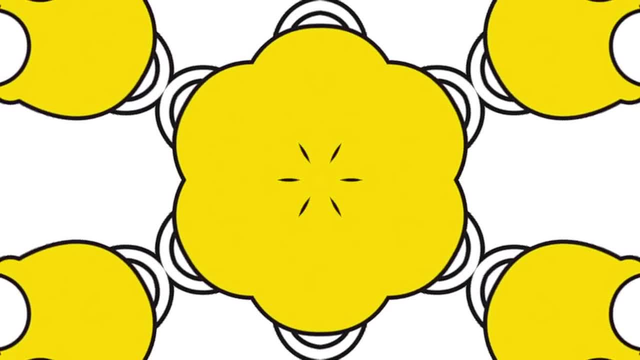 Obviously, a lot of people are going to like what you're saying When you get criticism or when people say: hang on, you haven't thought about this. Can you think of any criticism you've heard so far that you've thought actually that's. 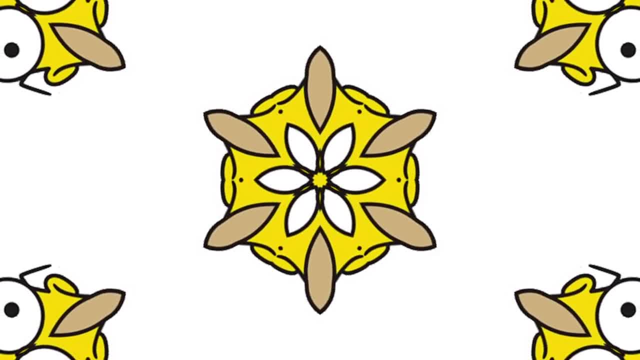 a good point. I hadn't thought of that. The one that came to my head you've already addressed, which was sort of the elitism of it and just like the good get better and that. but you say you can come in and out of the. 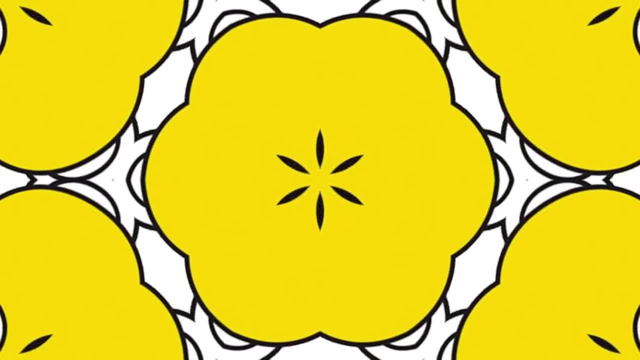 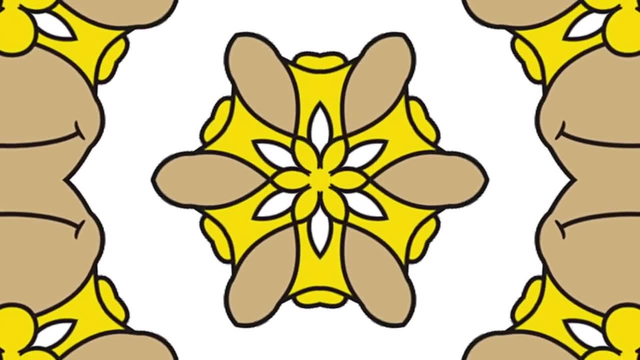 set. But what's the criticism of it? Help me criticize it, because I think it's a good idea. The weird things are things like there are problems with it which you don't see until you actually get to the core. There's a lot of things that you can do. 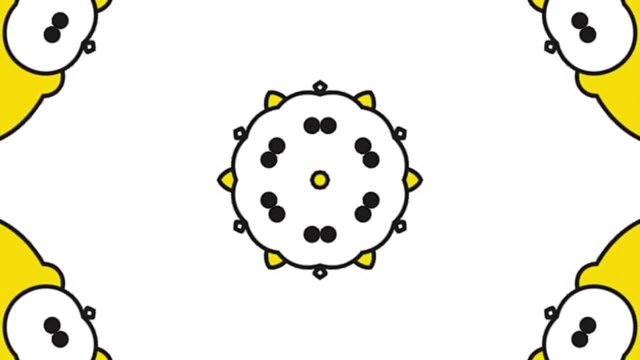 Like you can't even do it in the real world. You can't do it in real life. You can't do it in the real world. You can't do it in real life. You can't do it in the real world. 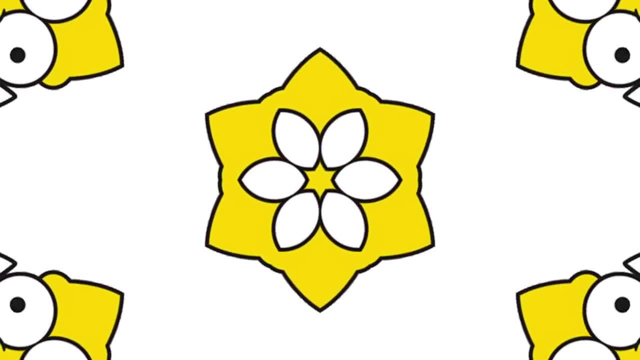 You can't do it in the real world, But there are problems with it. And what I mean by problems with it is that in schools this is the most tedious thing in the world, but it takes up a lot of effort. Some schools are so big. they have a band 1 and a band 2.. 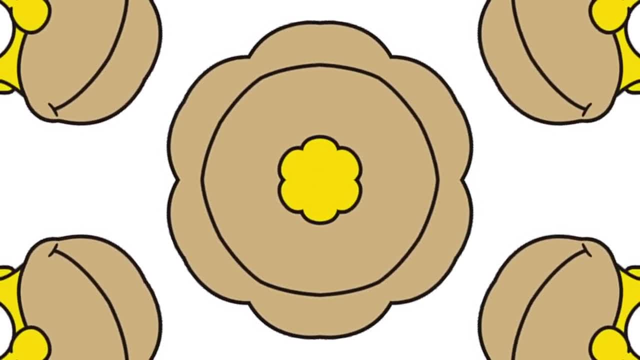 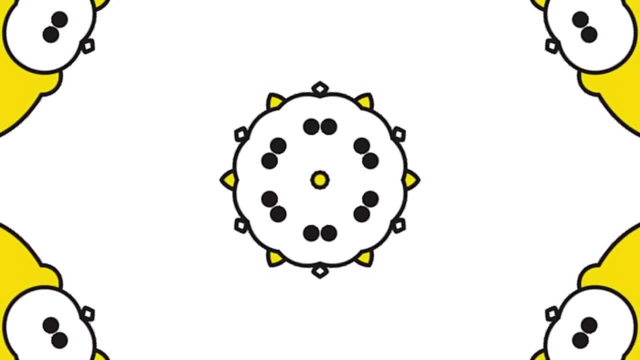 For anybody who can't see this, I'm doing jazz hands. at the moment they've got a band 1 and a band 2. And it's purely so that we don't have enough science labs. So when this band is doing physics, the other band's doing history. 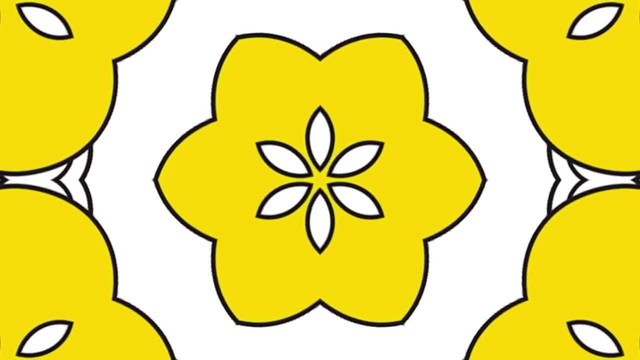 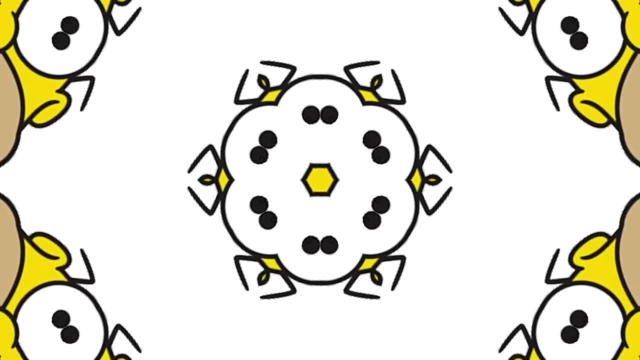 when they do physics and other bands doing history. So that means your top top set has got to sit in one of these two bands. Right, You can't have band one top top set and band two top top set. Well then, you double the cost of the project. 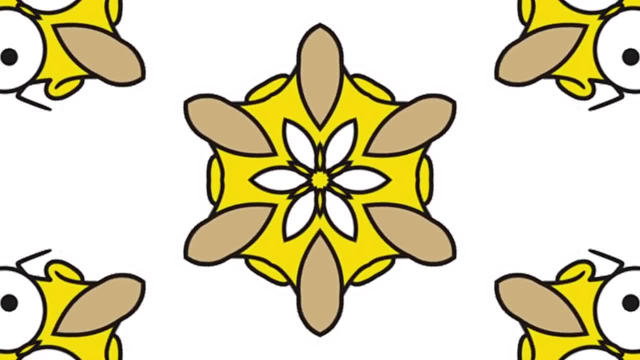 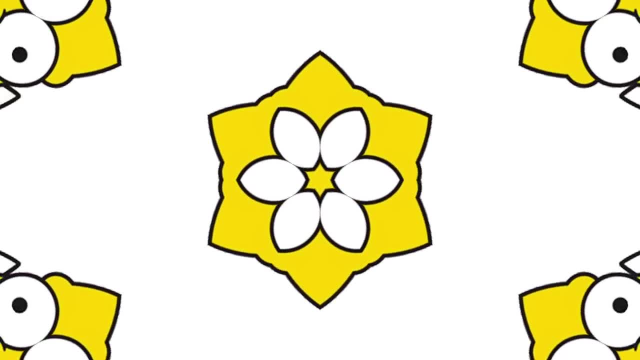 So then, how do you select students and how do you allow for migration between bands, and how do you – so those things are the nitty-gritty of how do you actually make it work? Now, in some schools they do maths across both bands. 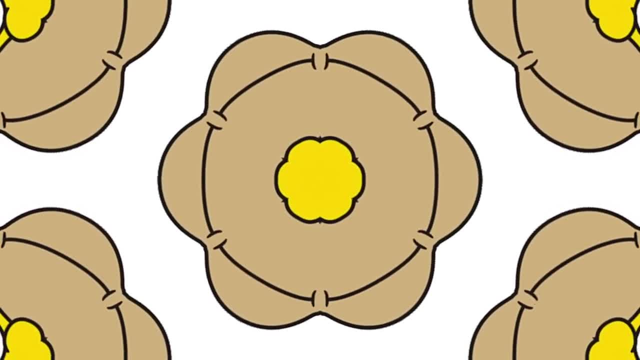 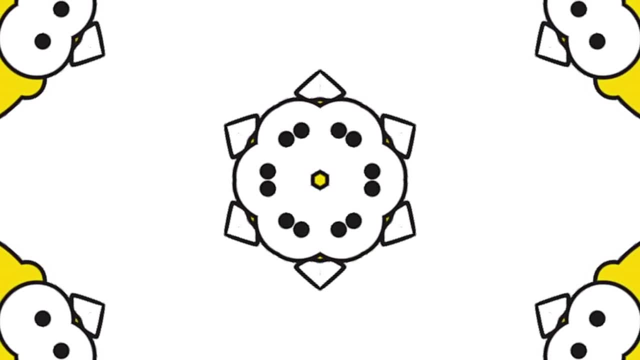 It's not a problem. In some schools they only have one band so they make it work that way. They're more logistical problems than this project is fundamentally flawed or is ethically wrong. Every school I've come across has said: we want to do the best for all of our students. 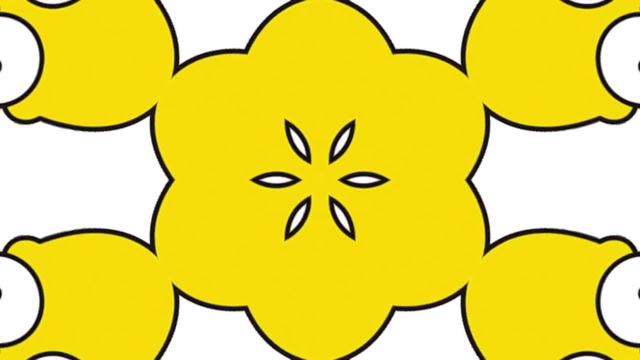 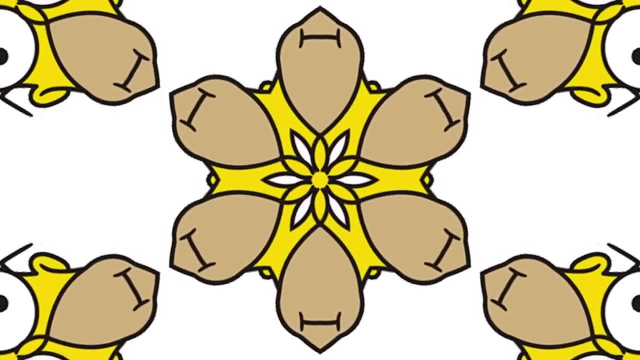 If this student's musically gifted, we want that student to excel. If this student's struggling with their science, we want them to become scientifically more confident. But if this kid's got a maths bug, we want to stretch it as far as it'll go. 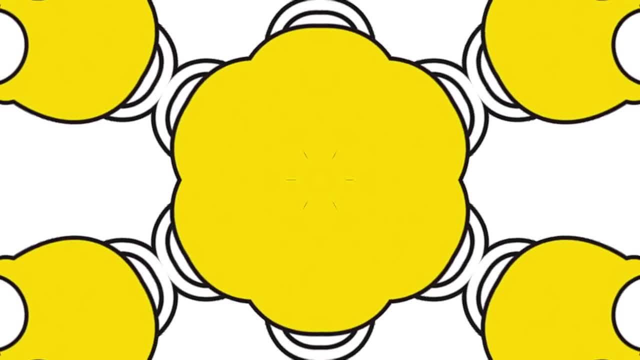 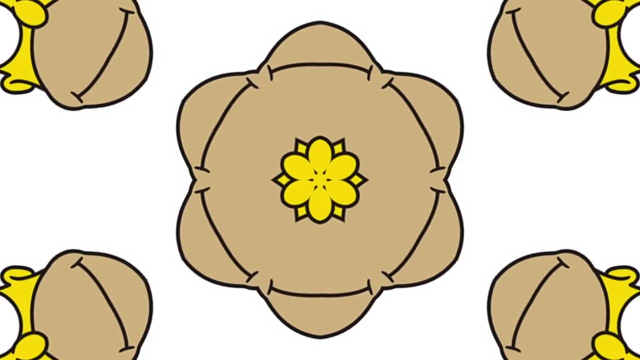 So they want to do the best for every student and they very much see this as being one of those ways of succeeding. Do we not need English top top sets and history top top sets? No, No, No, No, Just maths. 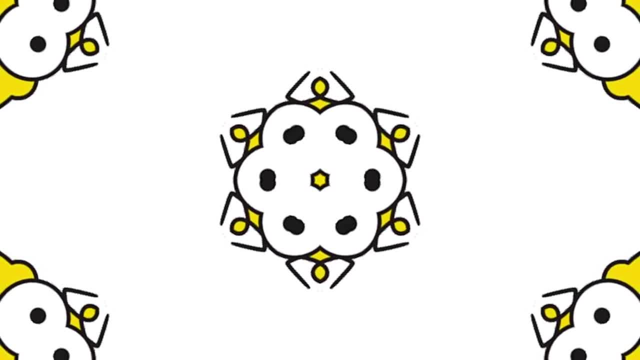 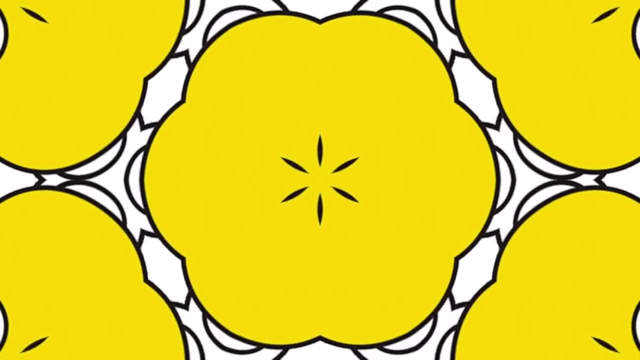 Just maths. yeah, I can explain that. The reason is, my feeling is that if you're interested in history, I think a lot of families can support that. A lot of families can – they'll go to Warwick Castle or the Tower of London. 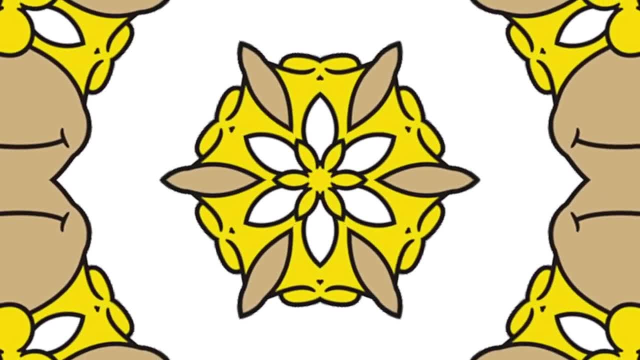 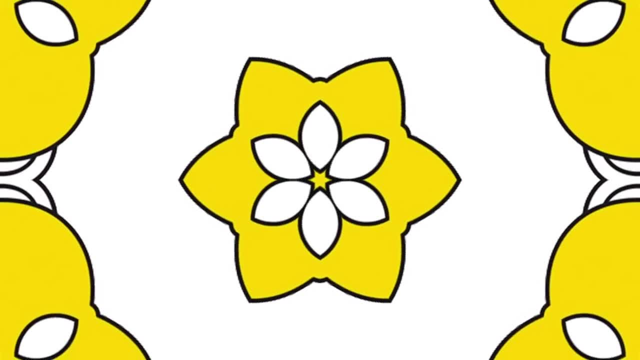 You can watch horrible histories. You can watch more serious documentaries. History is very accessible If English is your thing – I remember our English teachers used to say: oh you know, look, you're good at English. Here's a Dickens book. 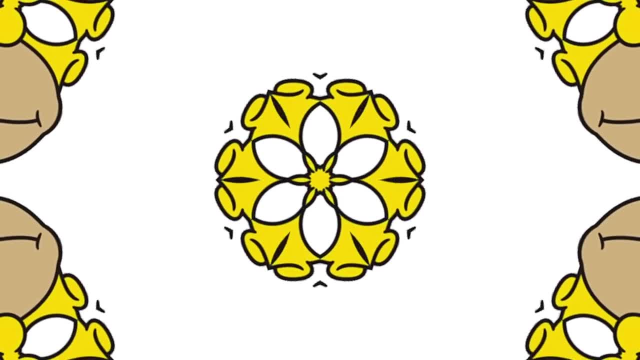 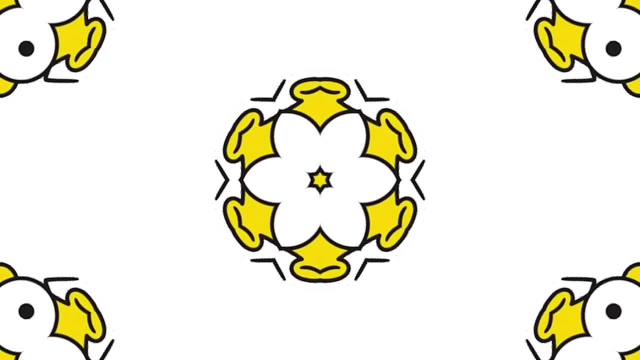 I want you to read this one over the Easter because I know you'll cope with it And you can just be stretched while you're at school. Maths is different. Maths needs mentoring, It needs that guidance. You know you and I can read the same Shakespeare book. 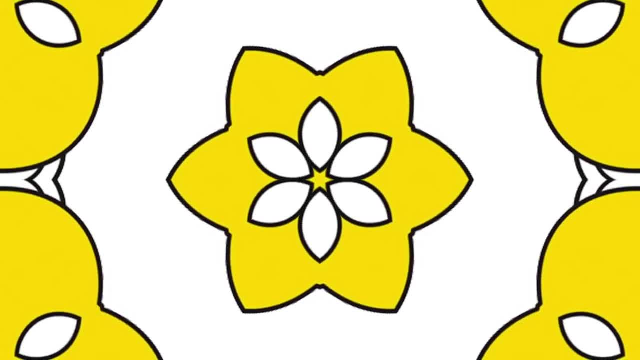 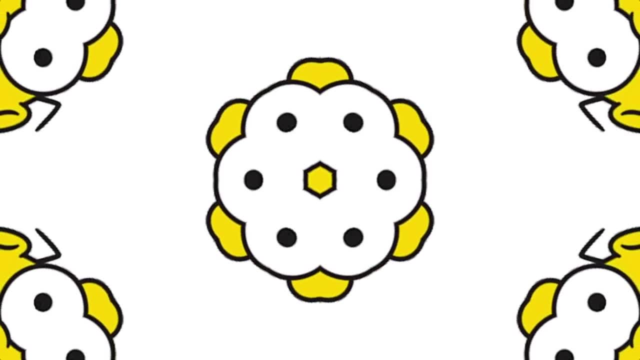 and a load of it will go over my head and you may appreciate it in a much deeper, more meaningful way. But we can look at that same book and read it at the same rate. If we look at a calculus book, then that's not going to work. 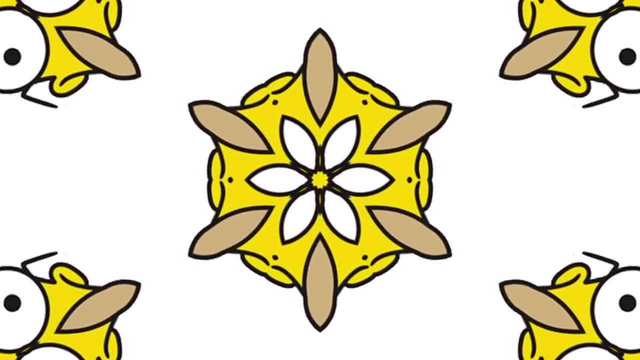 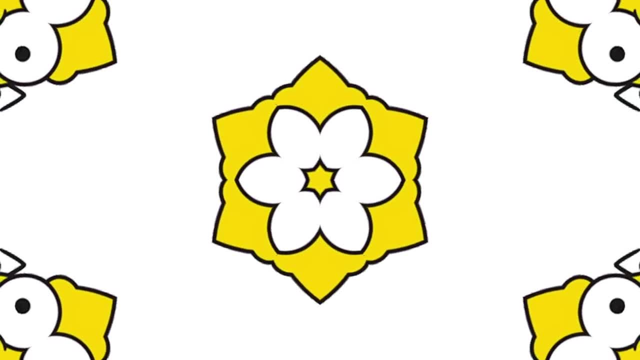 You know, for some people it just means absolutely nothing at all. For others it's meat and drink to them and they'll speed through it. So I think maths needs that mentoring and that careful approach. The data suggests. the international data suggests: 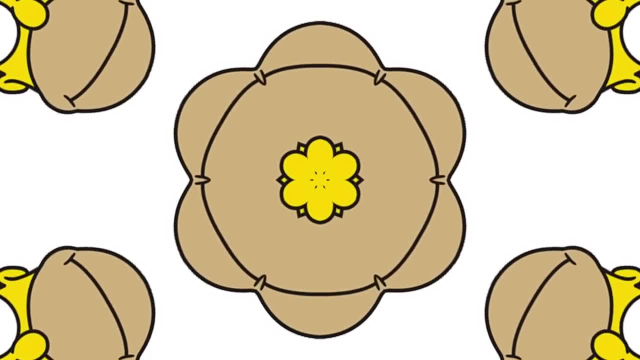 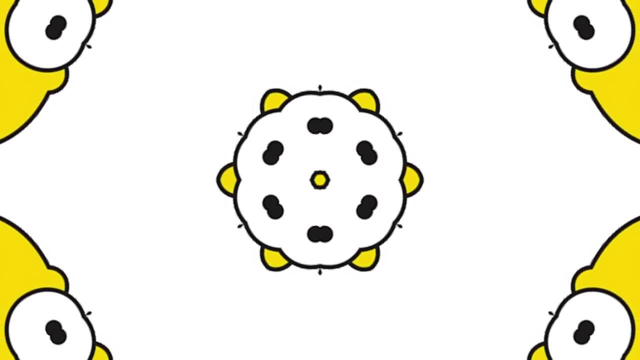 that our students, our average students, are pretty average compared to the rest of the world, And we've got a lot of average students. What we don't have, thankfully, is very much at the bottom tail, but we certainly don't have very much at the top tail either. 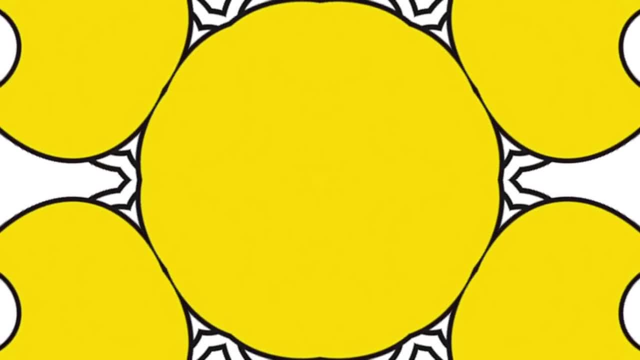 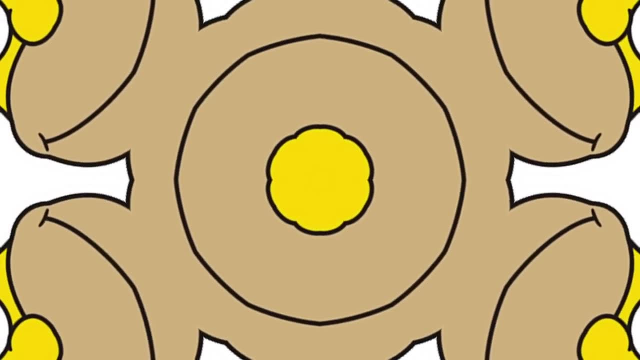 So that's where we're failing, as far as I can see, An argument I've heard that I'm imagining you're going to disagree with quite a strongly, but I wonder what you think about. it is the argument that maybe we place too much importance on math education. now 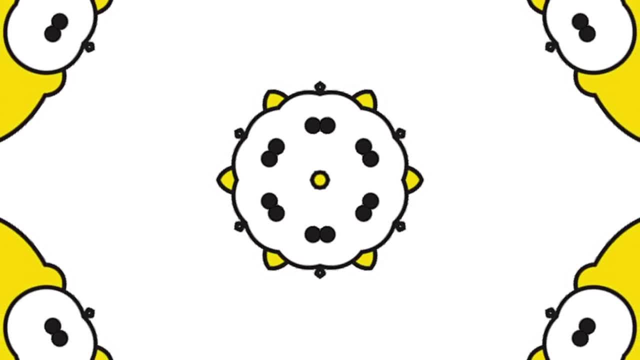 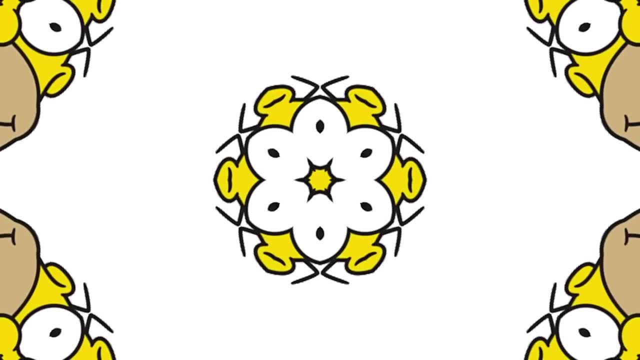 in schools and maybe the times have changed And while there is a place for mathematics, we should be pushing more towards computer science and programming and coding, and we should be turning the math dial down a little bit When I think about maths. 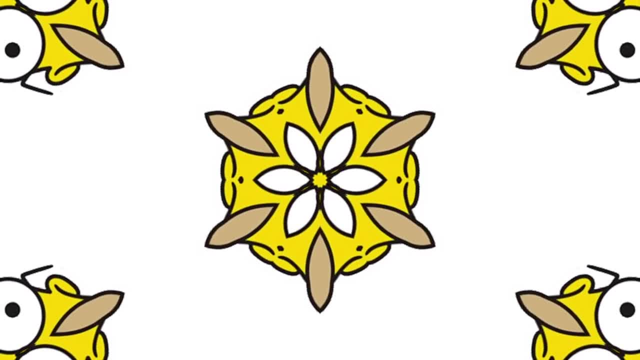 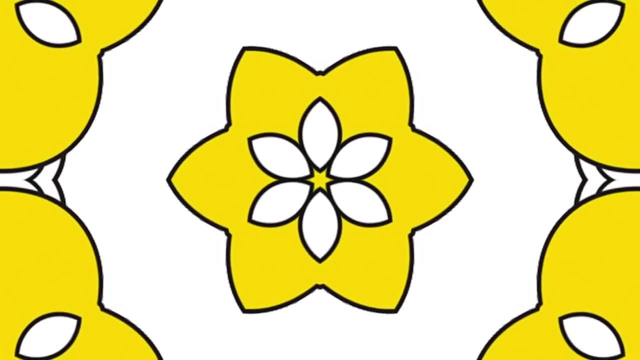 I think math is really just about developing thinking skills and it's just developing problem-solving skills. So those skills can be applied to anything and everything. So if you wanted, say, let's throw out this load of maths and instead put in this coding bit in the maths. 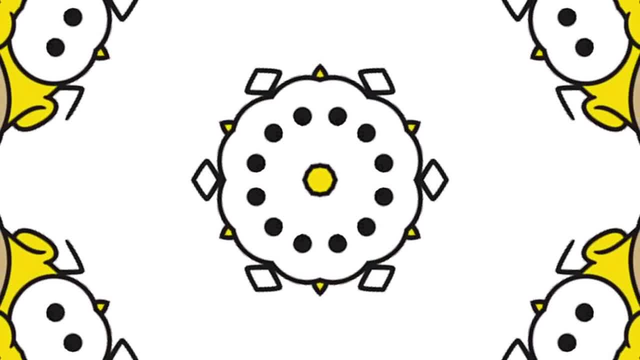 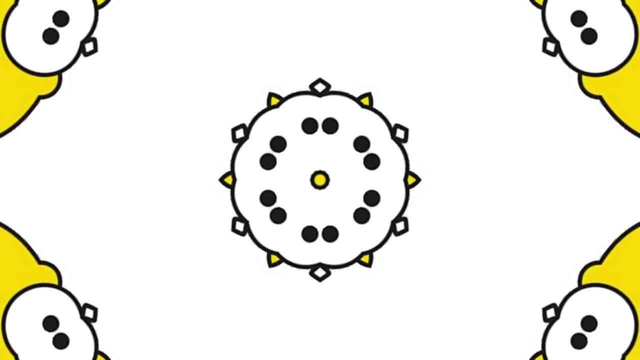 curriculum. very happy with that. if that coding skill is all about math is about problem-solving and so on. It's about giving children problems that they can't necessarily do and showing them how to tackle their problems. approach those problems, develop tenacity. 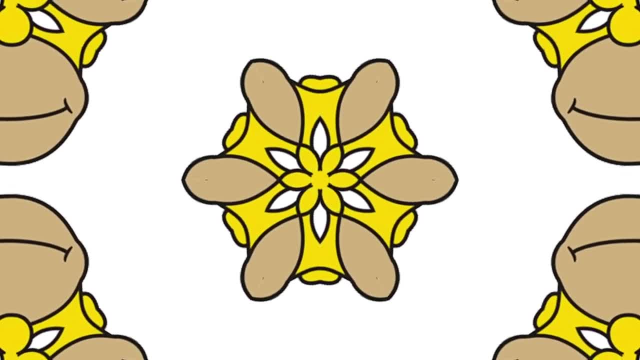 This whole thing about growth mindset. have you come across all these things? Oh, you've not come across growth mindset, Oh right, okay, So I hadn't come across it either, but it's very big in education at the moment. 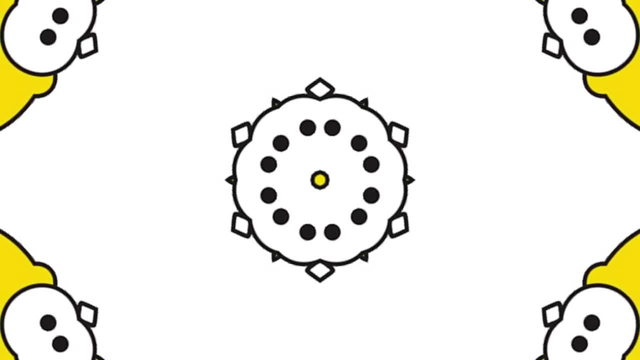 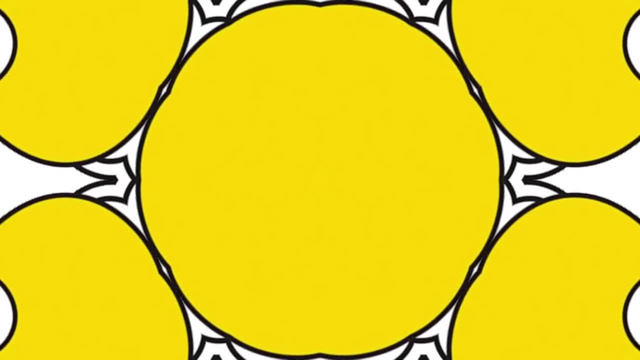 And some people say it's a little bit of twaddle and other people say it's revolutionary. But the idea is that in the past, I think when I was at school- oh, Simon, he's good at maths. that's it and Fred's rubbish. 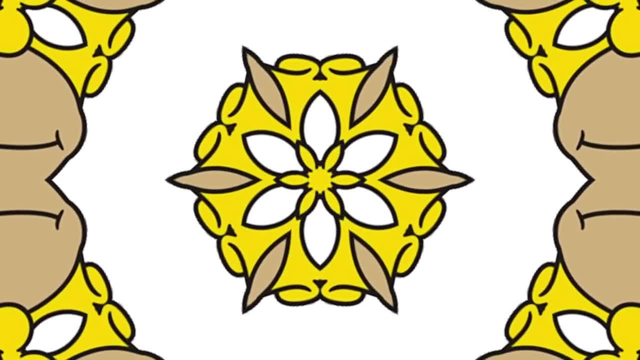 And Fred's always going to be rubbish and Simon's always going to be quite good because he's just somebody who's got the maths gene or whatever. And that's a really unhealthy approach because it means that Fred's just going to give up. 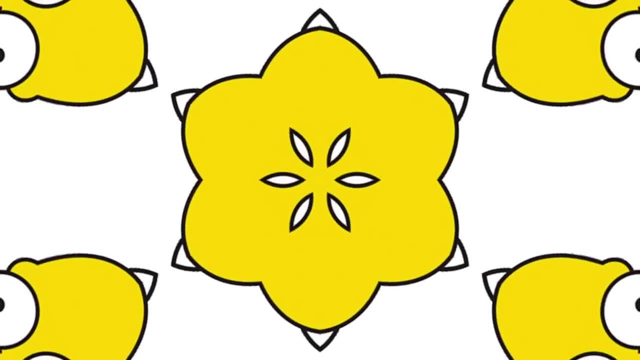 because he just hasn't got that maths thing And Simon's, it's not good for him either, because if he's just good at maths he's not going to try that hard. And also when I reach a point where there's a problem. 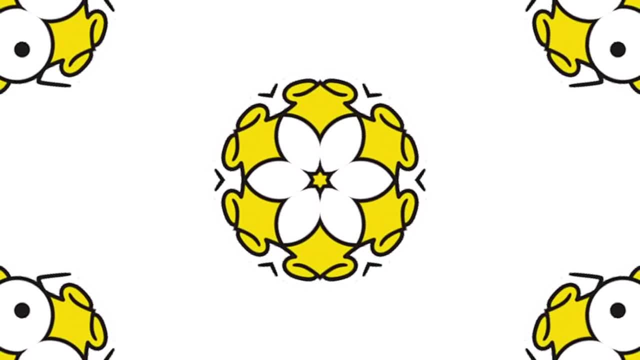 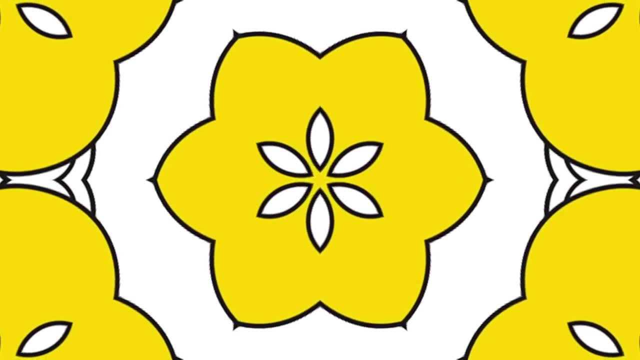 I can't do. that's kind of catastrophic, because I'm supposed to be good at maths and here's something I can't understand And it just destroys kind of your view of who you are, And that's fixed mindset. Growth mindset is the opposite. 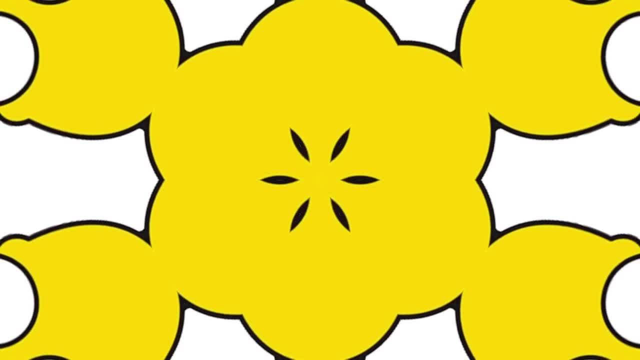 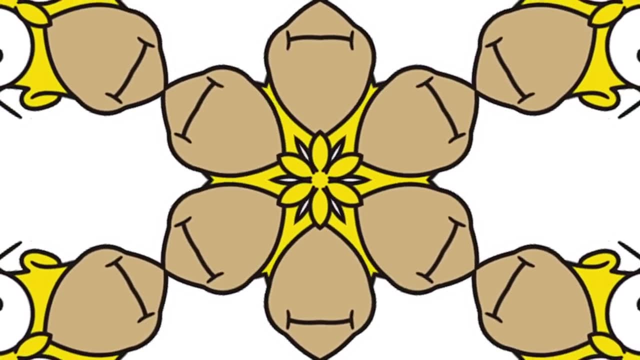 Growth mindset says that, whether you're good or bad, by working harder you can always get better, And, in fact, people who are good have typically been working quite hard previously to get to be good, And so it's not about you failed, it's about you haven't succeeded yet. 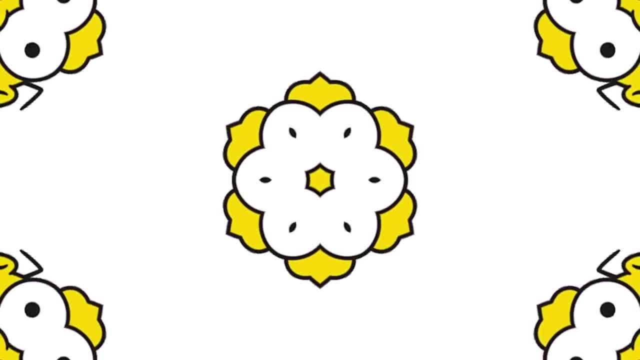 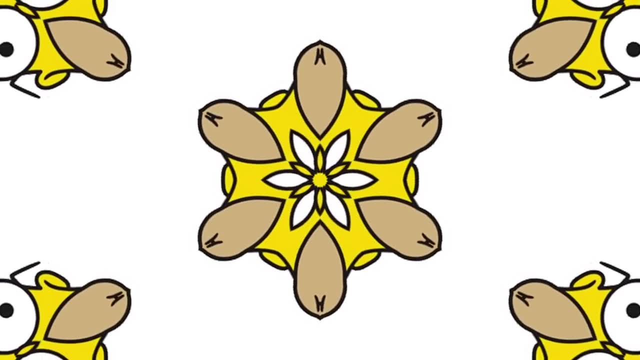 And so you always praise the effort and the work rather than the achievement. And regardless of the achievement, you know you can always do better, And so that's you know when kids in our top, top set should be struggling, because struggling is part of becoming a good mathematician. 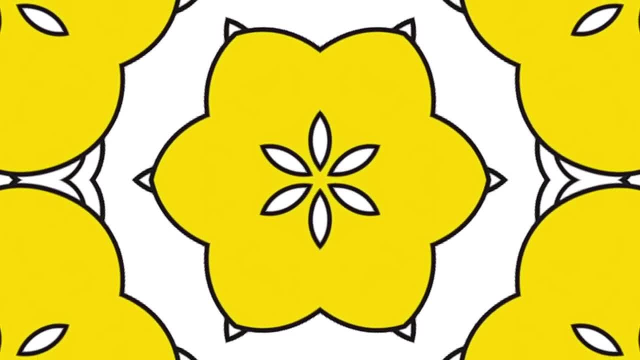 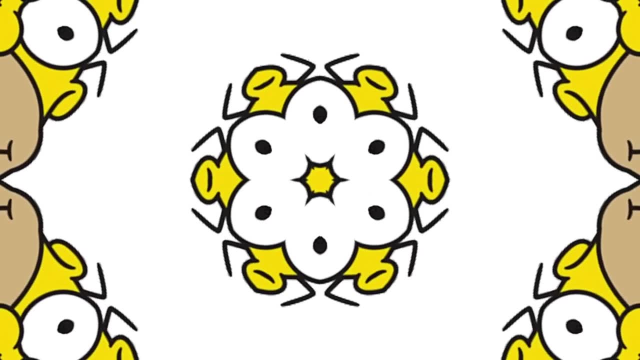 Whereas if they're in a normal top set, they're just good at maths. Gosh, look, they're just. it's just so easy And it makes them complacent and lazy and it just doesn't develop the skills they need. 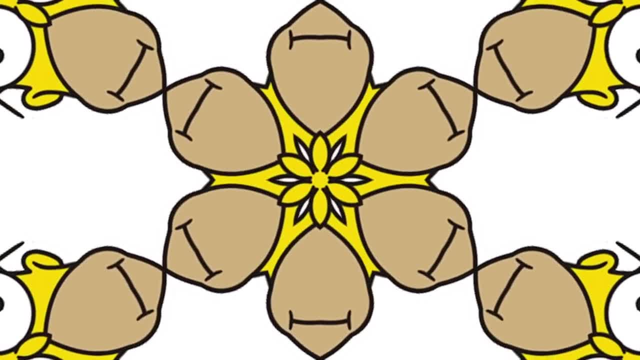 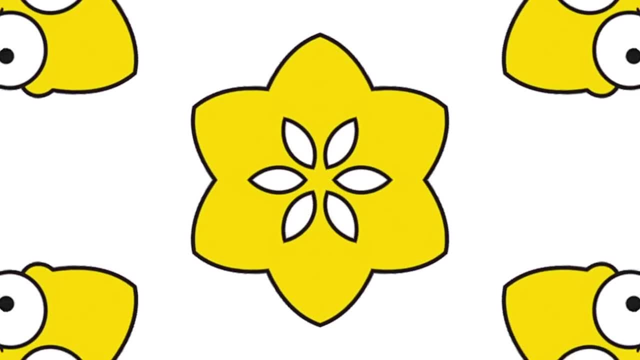 There's an experiment done a few years ago which I think illustrates some of these points, which was that you know, same kids put their hands up to answer certain questions. So you have lollipop sticks with all the names on. you pick them out at random. 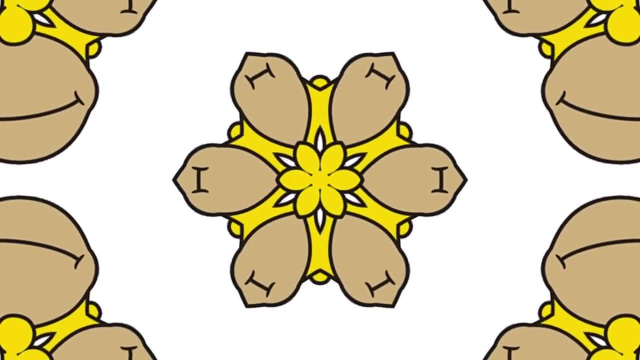 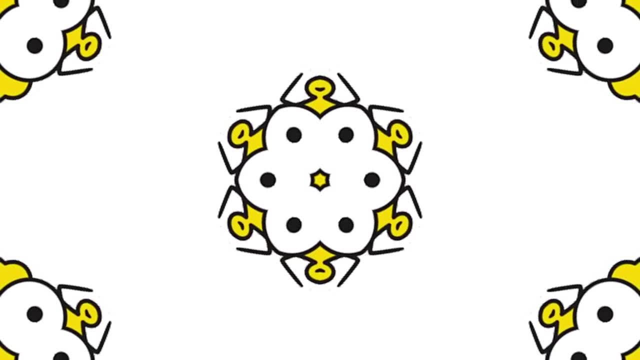 So you have a much broader array of kids answering questions being picked on to answer a question And everybody has to be alert because they may get picked on next. When they moved to this model, some kids started playing truant and not just just not turning up. 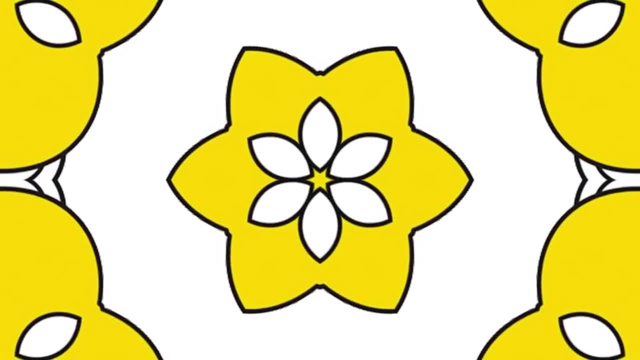 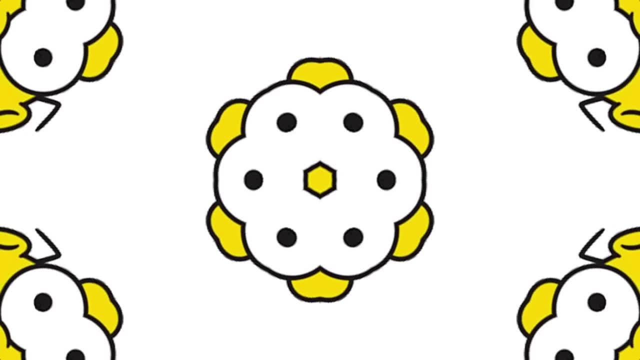 And the kids who were not turning up were the ones who were thought to be very, very bright, Because previously, when they put their hand up, they always got it right. Now there was a chance that they may get picked on for a question that they didn't know the answer to. 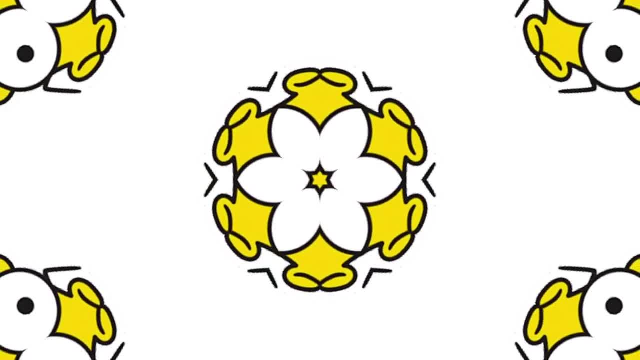 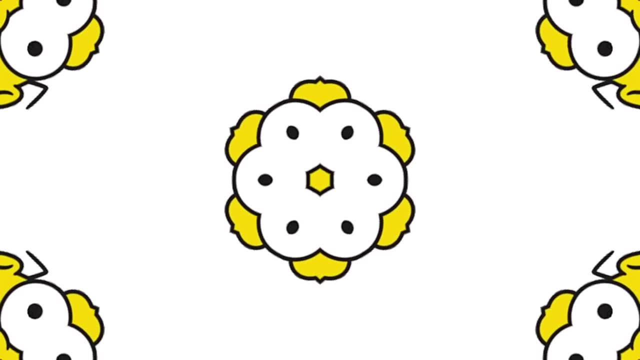 And then they'd be shocked. They'd be shown up as not being as bright as everyone thought they were, And that just destroyed their vision of who they were. So that's part of the top. top set is about developing those skills to apply in engineering or coding or anywhere else. 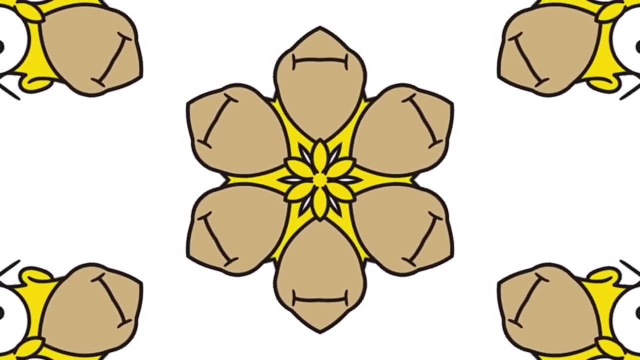 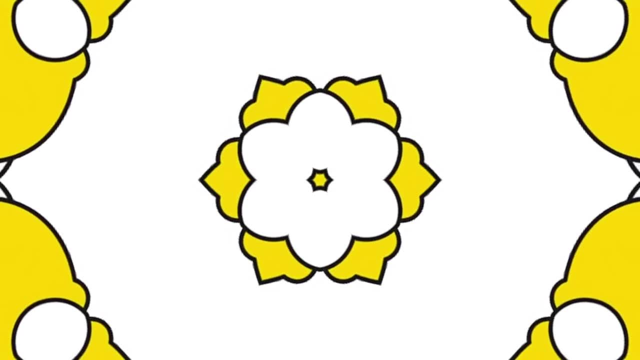 And physics in particular. I can imagine not wanting to go into the top top set for that very reason, though, Like thinking, oh, if I go up there I'm going to get beaten up every day. If I stay here in the, just in the top set, it's all right. 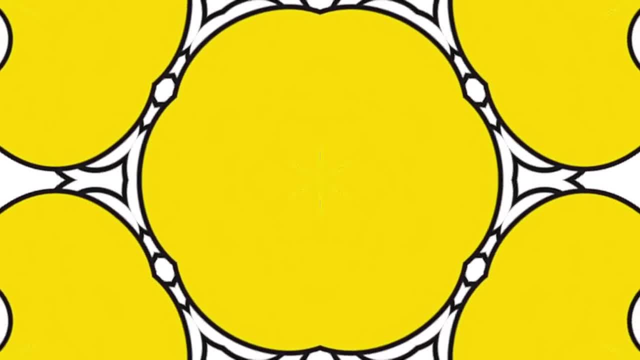 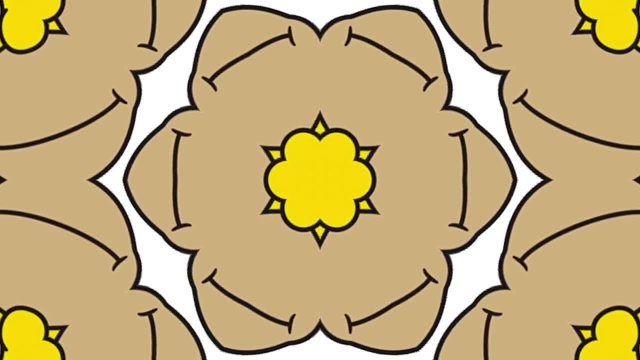 I'm a happy life. Our experience is that it's a leap from primary And I think when they move from primary to secondary kids kind of are open to anything And that's one of the advantages. I know some schools do this sort of top top set approach in the year before GCSE. 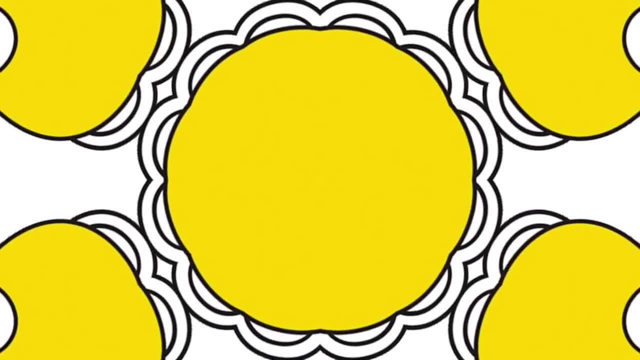 You know these kids are going to do A-level. We'll be better start working them a bit harder because they're going to be the A-level math. That's too late. You've got to start them when they're 11 or 12,. 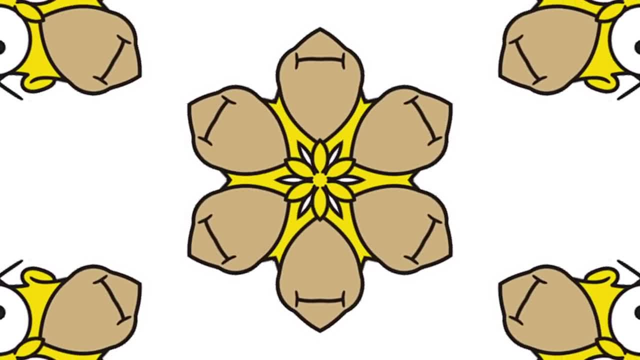 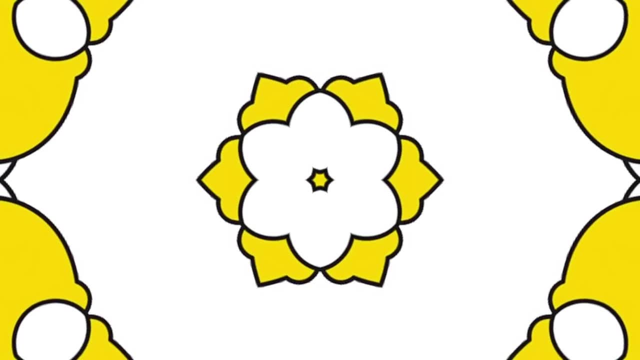 when their attitudes can change and their ambitions can change And they realize they can solve math problems that look apparently impossible to them. I can't remember what it's like to be that age- It was so long ago- But is it a situation where being put in? 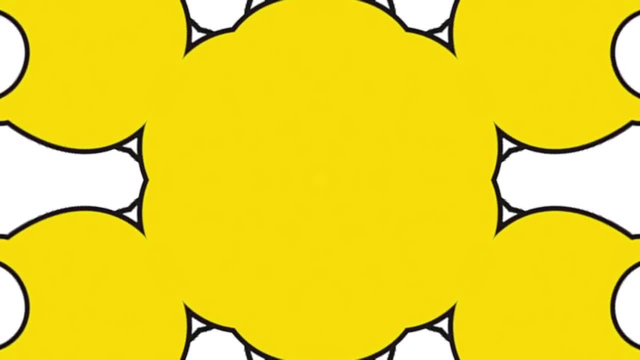 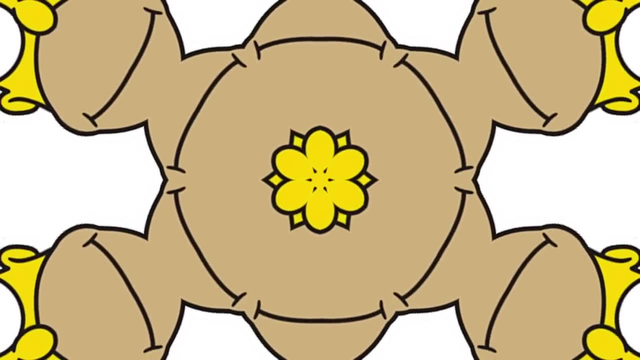 the top? top set is like prestigious, Or is it like being put in the nerd club when you want to be cool with all the cool kids? I think some schools don't make a big deal of it. They just say, look, we have. we've always had a top set. 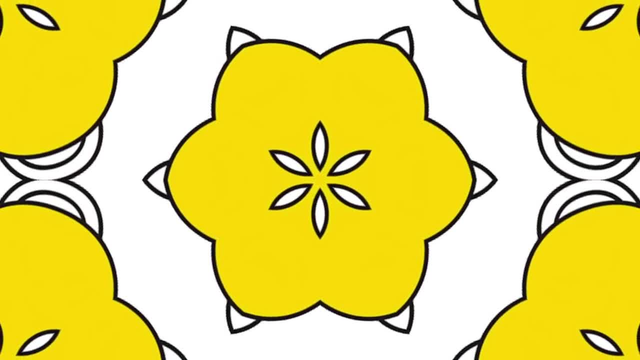 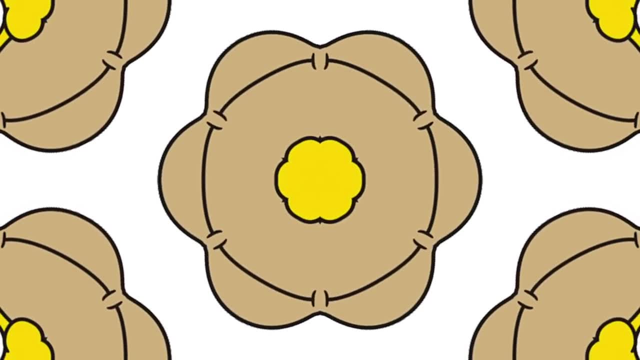 And now we've also got a top set, But the old top set has now just gone down, You know. so it's just the same system as before. Top top sets tend to be a little bit smaller. They tend to be more like 20 rather than 30.. 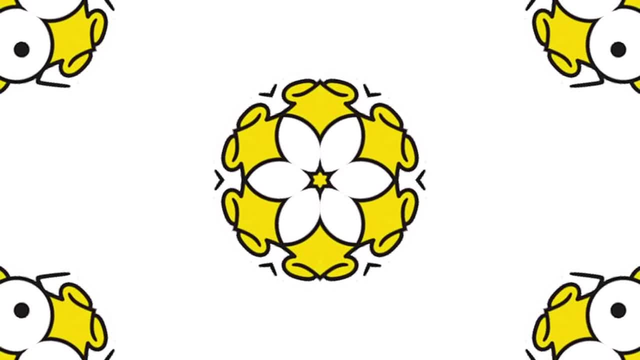 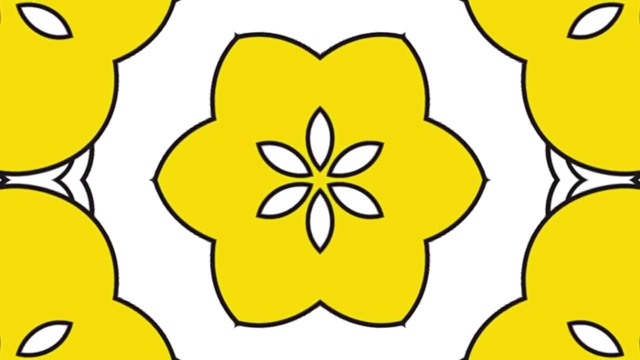 So I think I think in general, the students know that math is now their thing. They're like being in the school football team or the school football team. They're sort of in the school math team. So it's more prestigious. I think it's a bit more prestigious and they take it a bit more seriously. 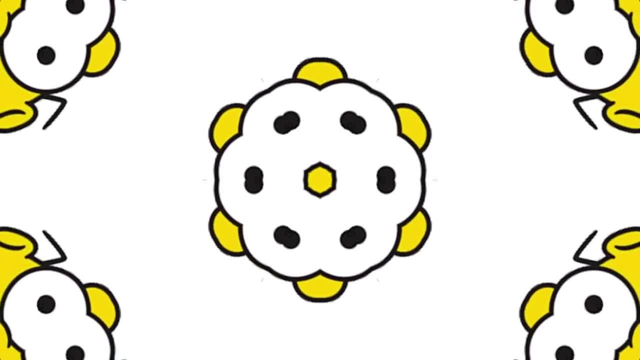 And they do extra work. Again, you know, one argument would be: well, they're good at math, Why do they need to do extra work? And my argument is: well, if they're going to build their future on math, 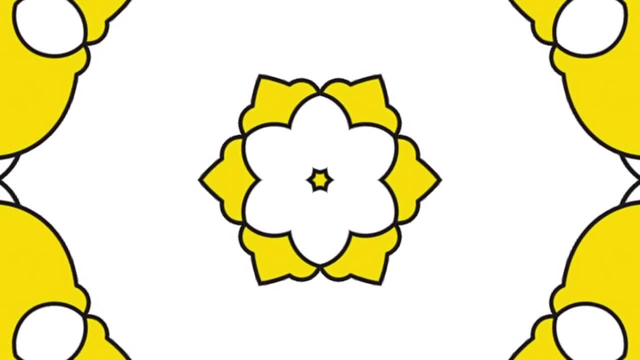 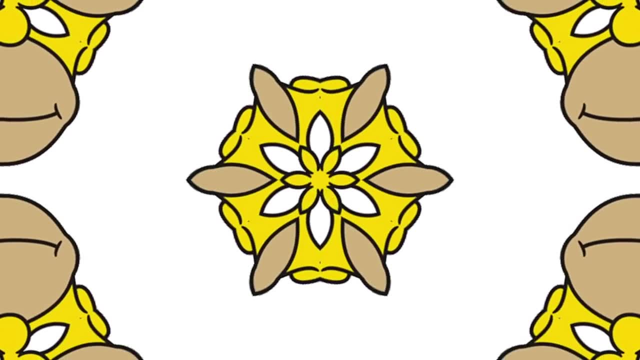 then they do need to do it. If they're going to compete with the grammar school kids, if they're going to compete with the kids in the private schools, they're actually still catching up. And so one of the things we've done, in addition to just having the top 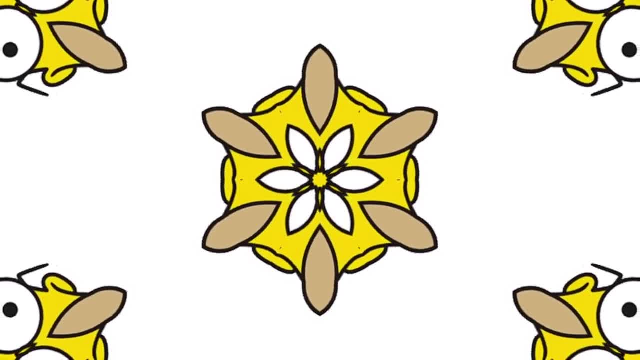 top set project is something called Parallel. So Parallel is a weekly math sheet. It comes out on a Thursday at three o'clock. It's all free. Anyone can sign up. It's like an email list, isn't it? You can sign up. 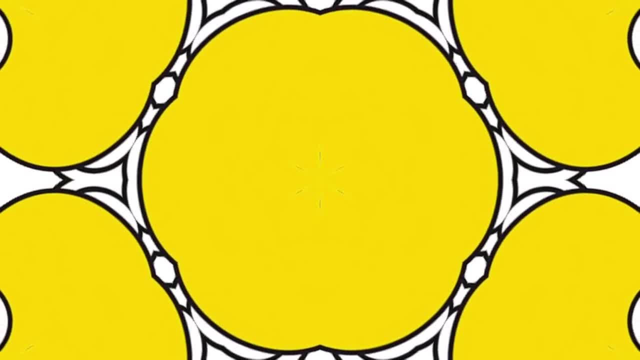 Yeah, that's it, And then you just go onto the Parallel website. It was designed, though, for our top top set students, So they had an extra 20 minutes of math to do over the weekend, But, as I say, anybody can sign up. 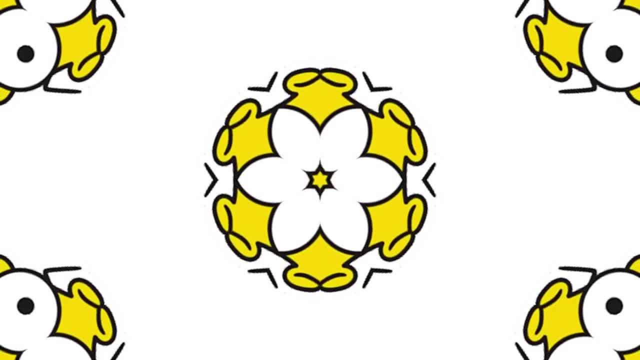 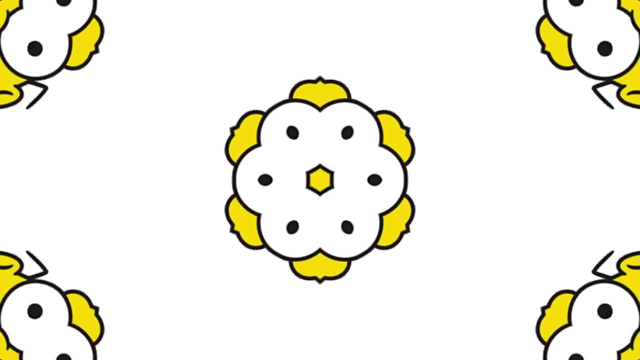 We've got a year seven sheet, a year eight sheet, a year nine sheet. Teachers can sign up their classes, Parents can sign up their kids. The math is interesting. Some of times there's even a Numberphile video there. Oh, excellent, excellent. 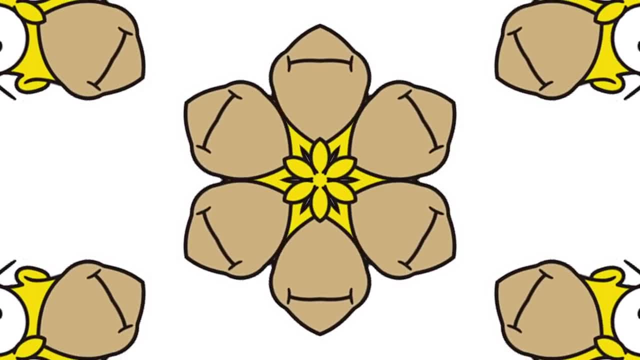 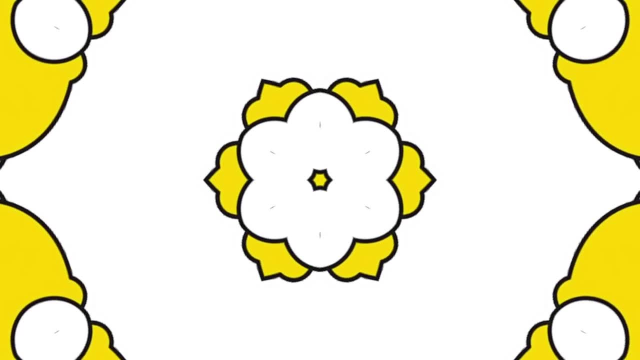 I need to get on more of them. No, they're brilliant because some of them are pitched at just that age group and they're challenging and interesting. And then there are film clips, TV clips, sometimes a video about philosophy, sometimes something about physics. 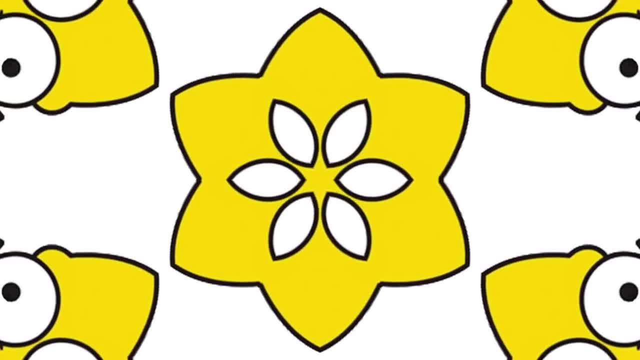 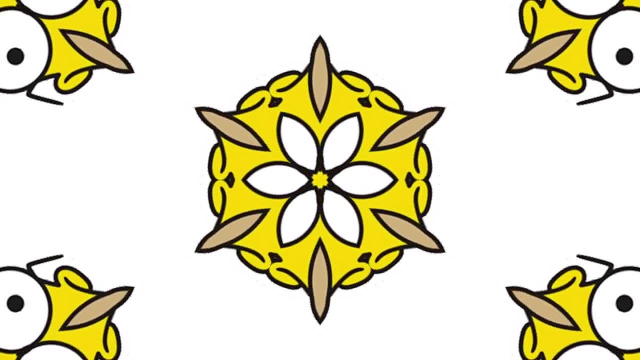 So these weekly – are you still calling them parallelograms? That's right, These weekly missives designed for the students who are in top, top sets, but you let everyone else in the world sign on for them too, if they just want to do them for fun or have some use for them. 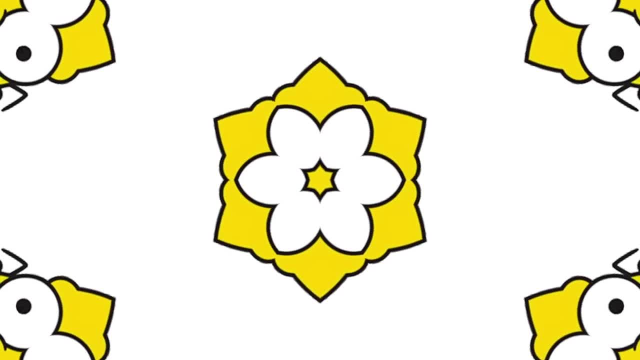 That's it. We've got a lot of them. We've got about 3,000 or 4,000. people do them every week, largely in Britain, but also around the world, And if you teach in a school that doesn't have a top, top set, 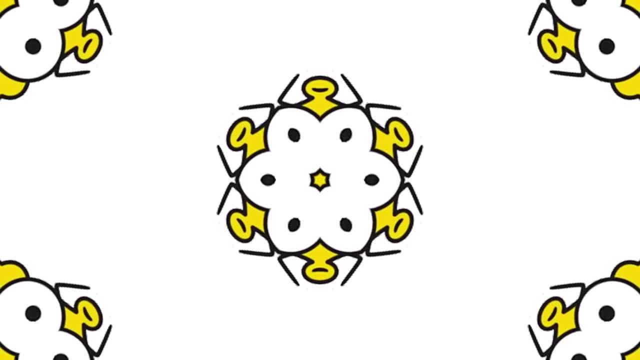 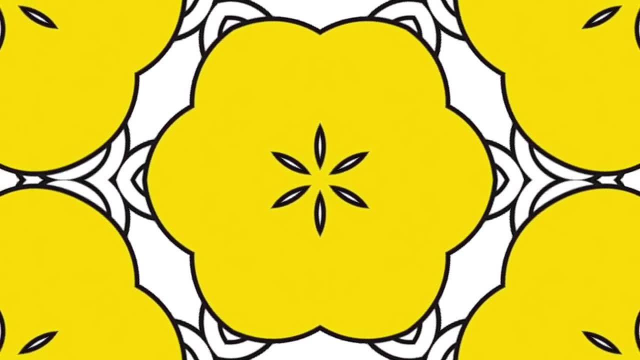 but you've obviously got kids who are strong and you want to stretch them, then this is a really easy way to do it. They can just sign up, They can do it. They get a solutions sheet when they complete it, And I think it's challenging but it's also fun. 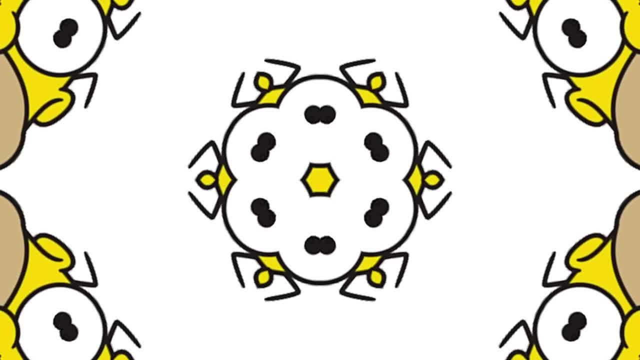 If you're a teacher or a parent or just a kid and you want to sign up to this, just yeah, parallelorguk, And I'll put a link. I'll put a link in the notes as well, for people, Great, great.